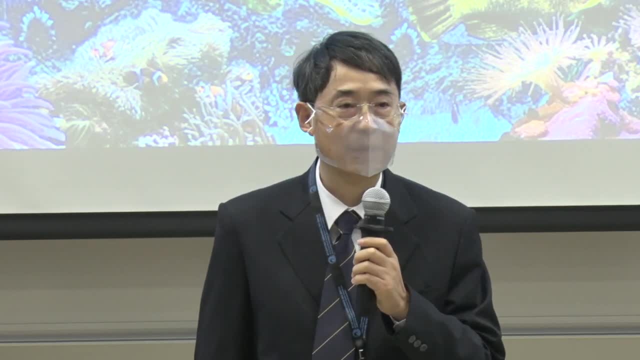 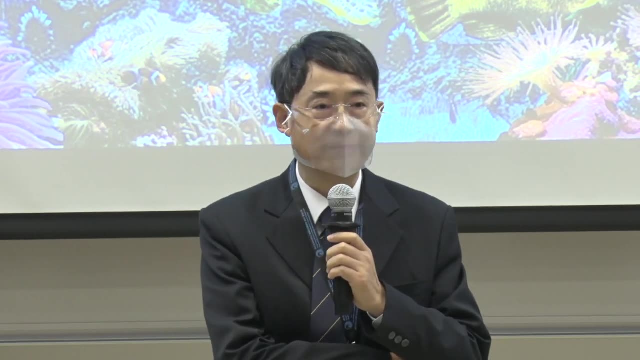 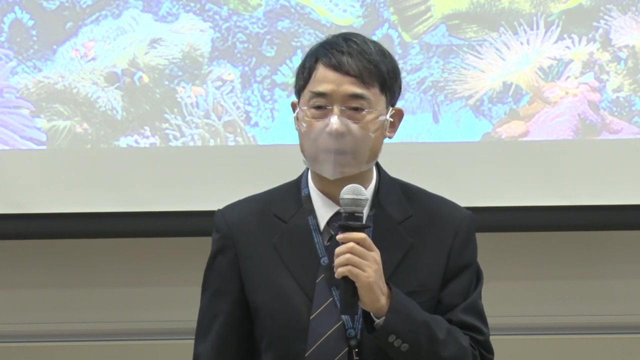 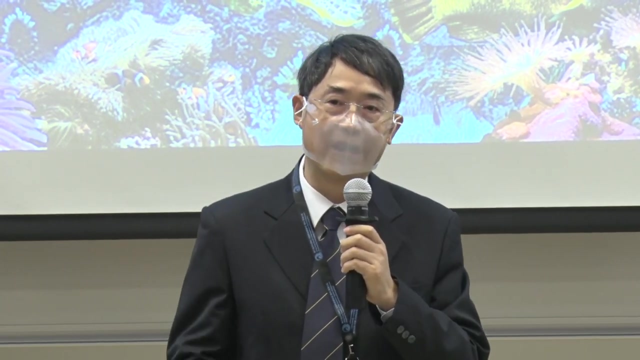 and the ladies and gentlemen, It really gives me great honor to welcome all of you here today and also the people online to attending this public forum on marine biodiversities. This forum is organized by the Hong Kong University, particularly the Department of Ocean Science, and to the Hong Kong branch of the Southern Marine Science Institute of Africa And this is a very special forum and I'm sure the students here are interested옅. I'd like to welcome Mr Wu here. Mr Wu, Thank you very much. 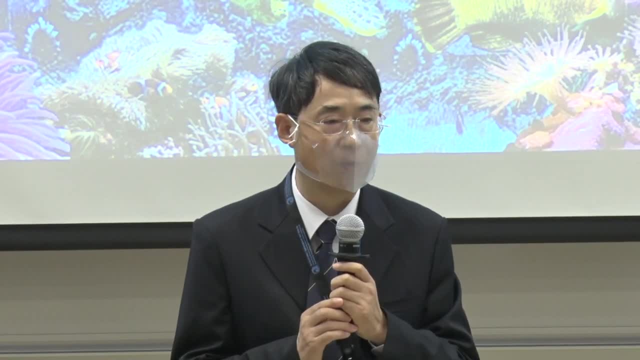 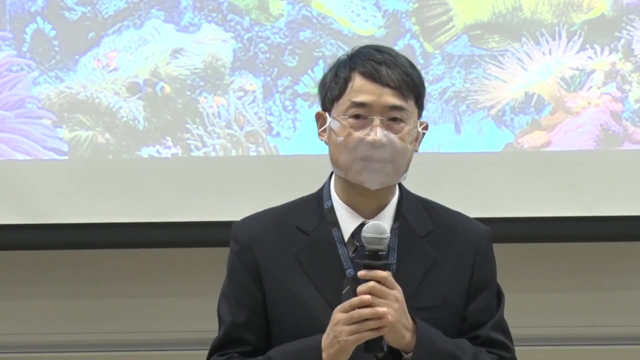 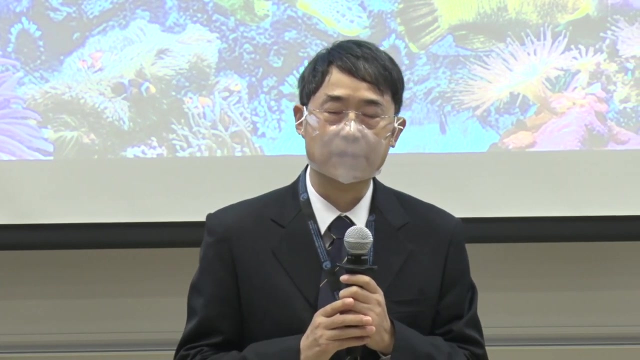 Mr Wu. You are welcome to attend this forum, Mr Wu. Thank you of the Southern Marine Science Engineer Guangdong Laboratory, in collaboration with the UNESCO of Hong Kong. So the professor down here is with us today. This forum is also in conjunction. 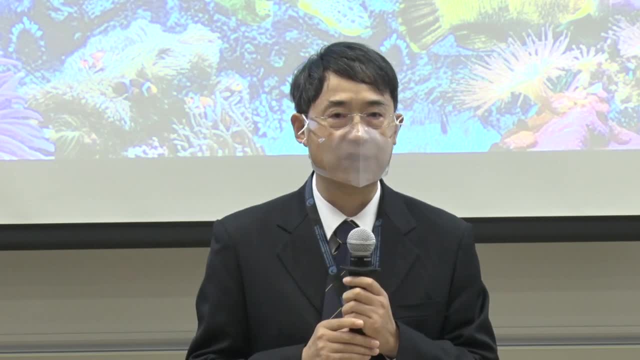 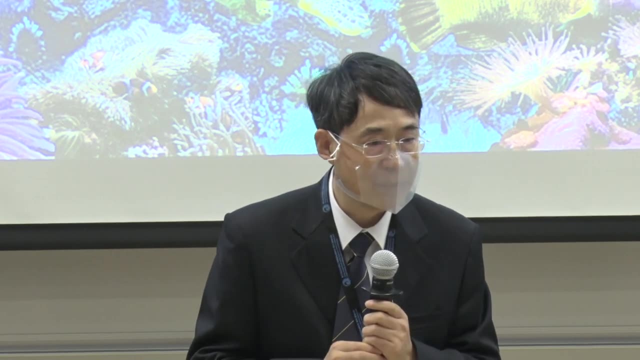 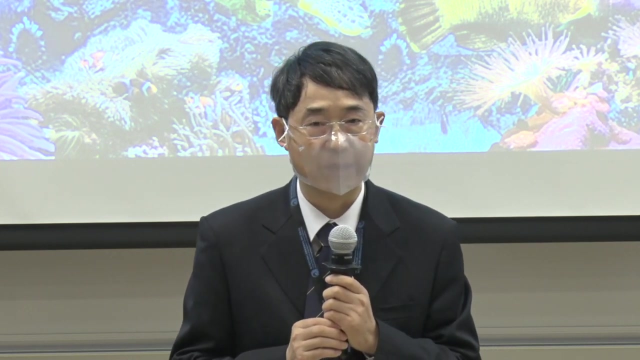 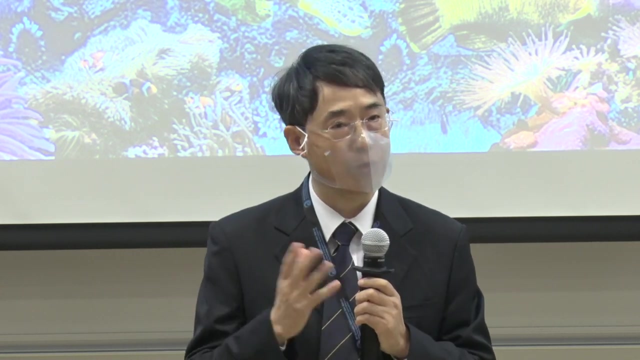 with so-called global climate change a big topic right now under discussion in Glasgow of the UK. It's also in conjunction with the World Biodiversity Conference that held last month in Kunming, So biodiversity is actually part of your and my life. 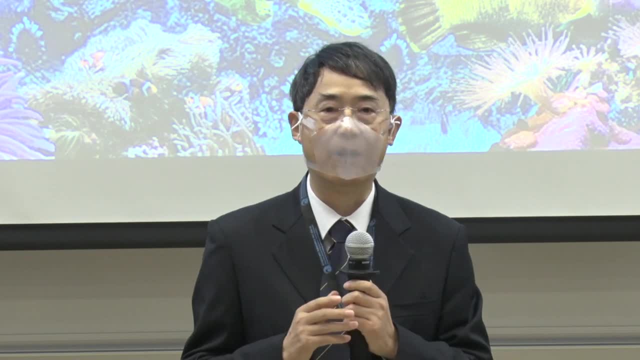 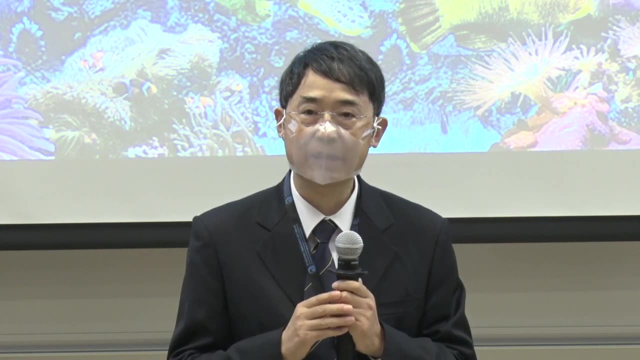 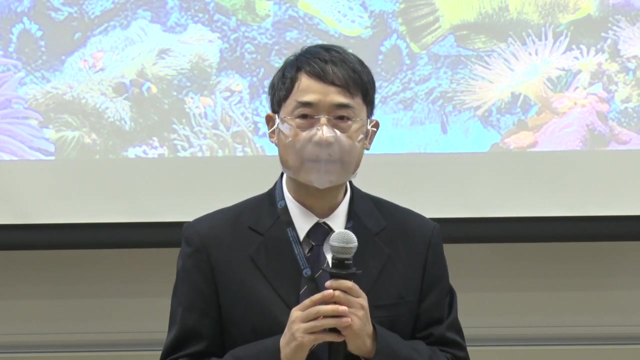 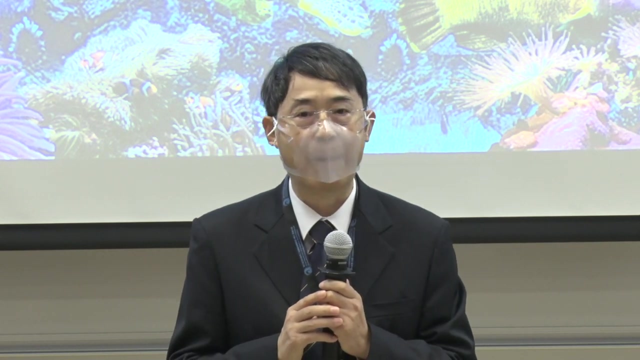 It's also the critical players in our life, supporting system of our planet. The biodiversity is also precious. As estimate and quote by the former Secretary General of the United Nations, Kofi Annan, the biodiversity value alone is about 3.5 trillion. 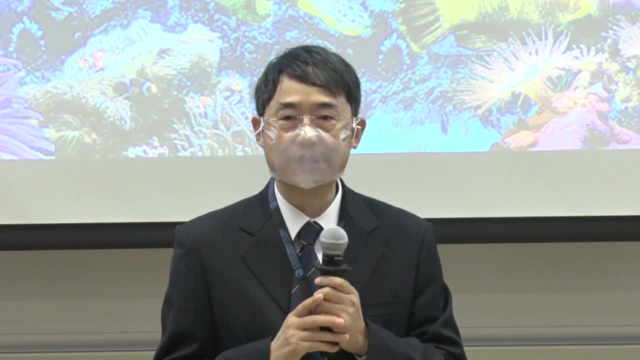 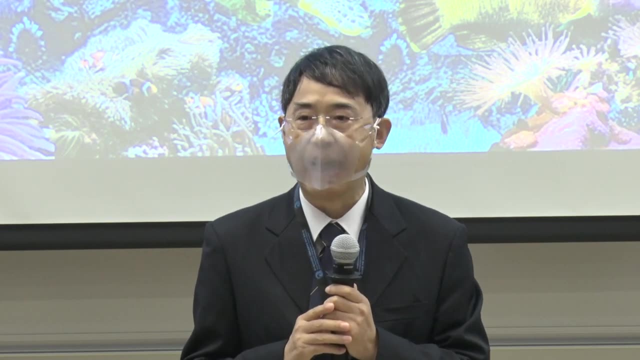 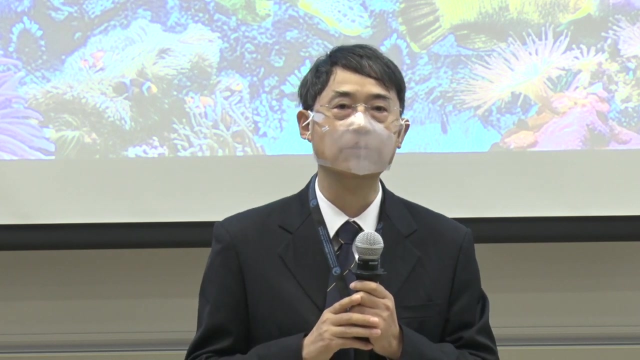 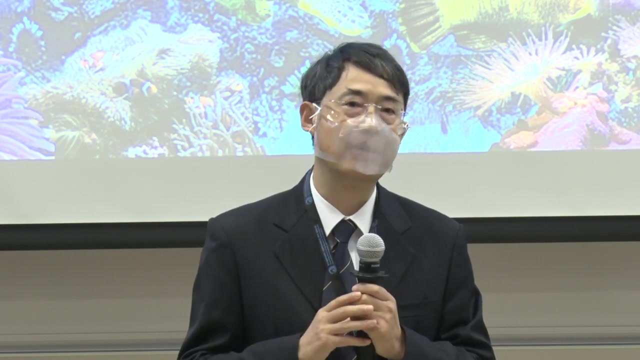 in early 2000.. The ecosystem value related to the biodiversity was of 35 trillion To the family of these two. we are now at some 1.2 trillion dollars in early this century, which is exactly equivalent to the GDP in the year when he delivers his speech. 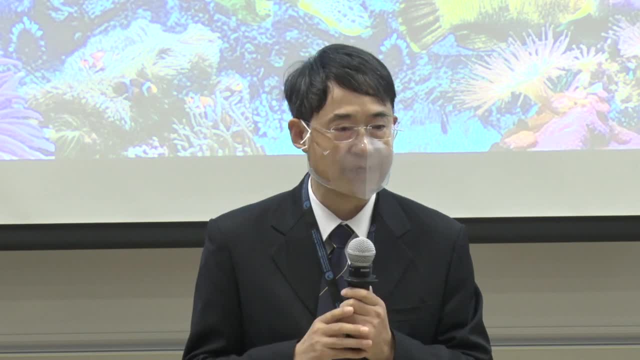 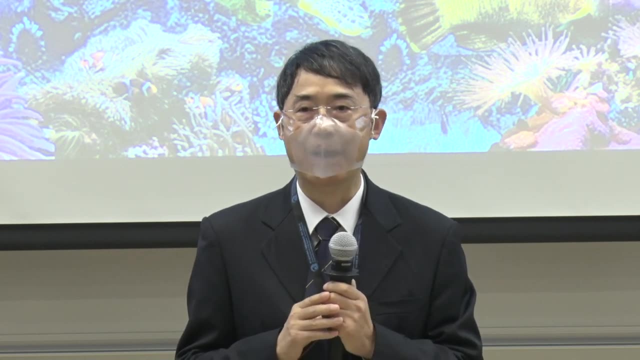 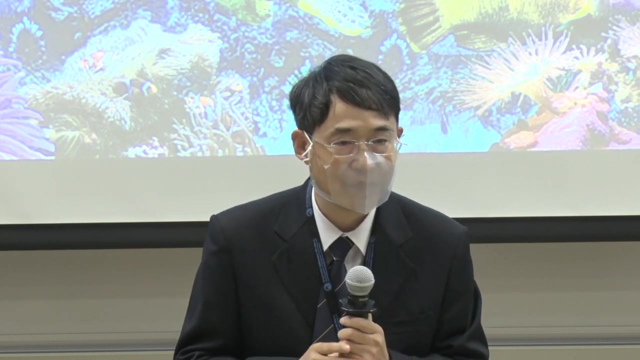 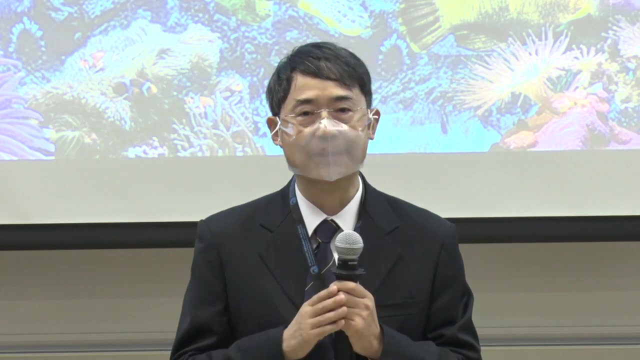 So biodiversity is very, very important. Yet the biodiversity is dropping or decreasing at very, very, you know, to the high speed: 140 to 140 species per day. Over the last 30 years, we lost somewhere between 15,000 to 50,000 species per year. 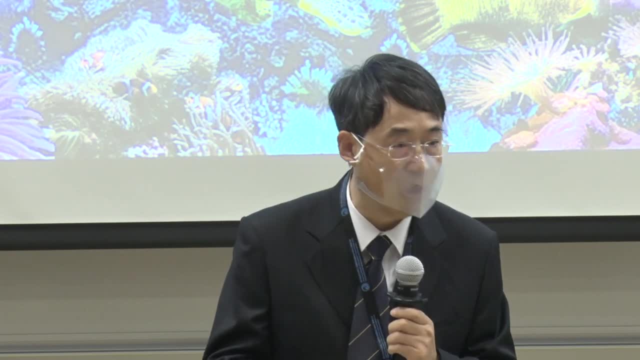 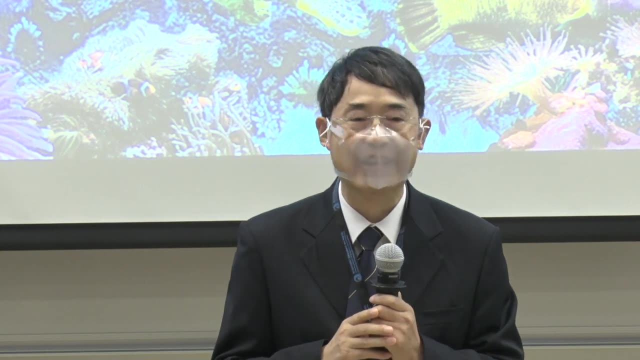 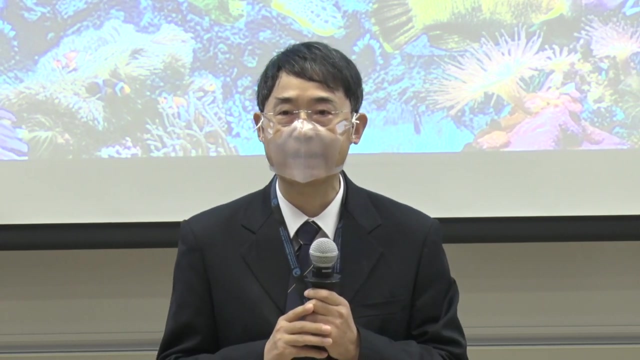 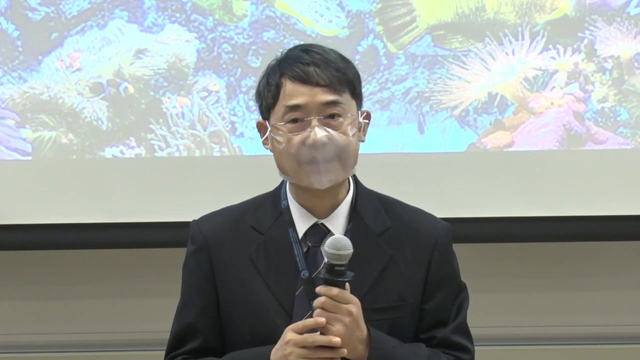 due to deforestation alone, So many of the species disappeared before we even got to know them. How many species actually we have? when we're talking about biodiversity, The honest answer is we do not know The estimated biodiversity of the number of species on our planet. 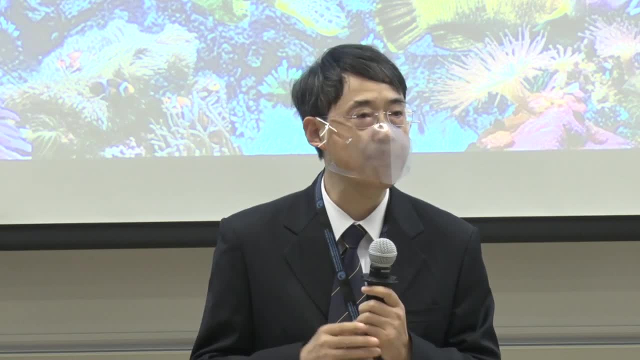 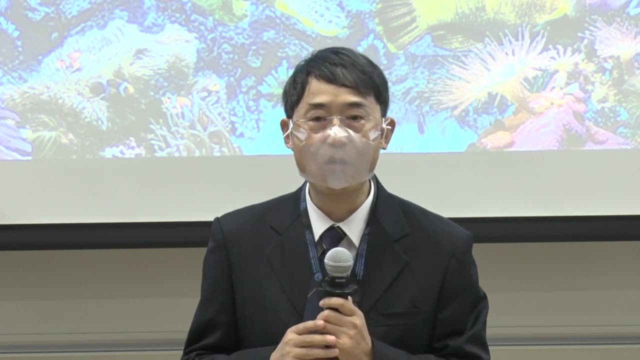 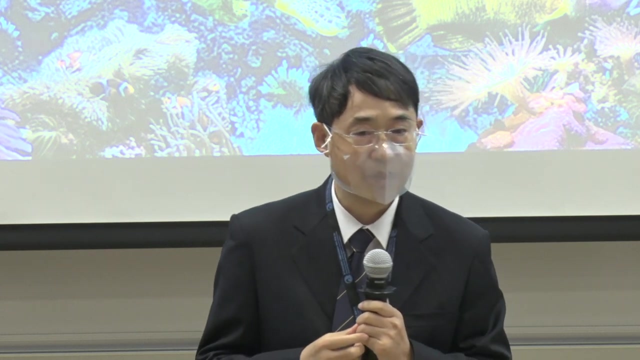 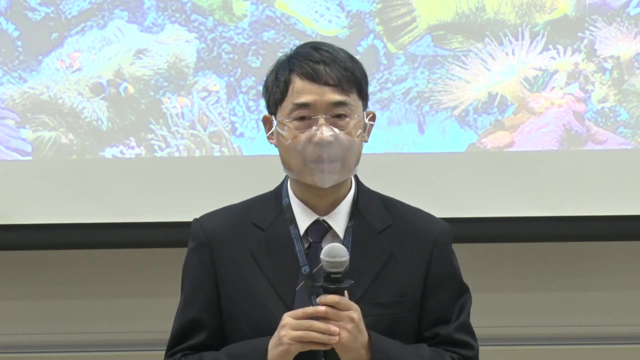 is about 8.5 billion plants and animals, without counting microbes. Only about 15% of those species has been described so far, And most of them is unknown to us for simple reasons. Most of those species we know also caused the described species. 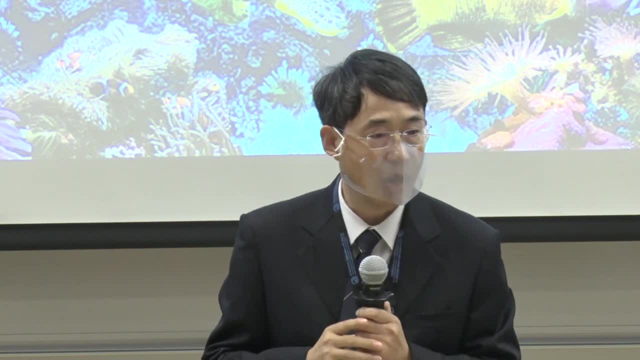 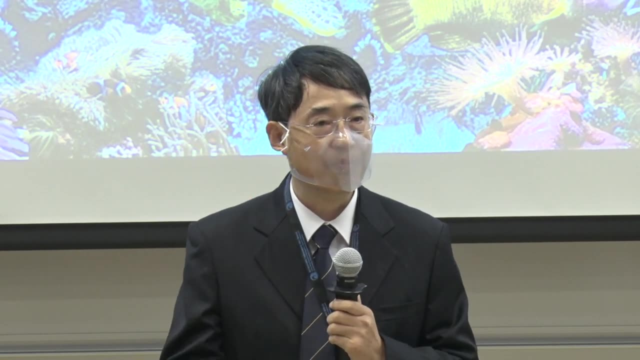 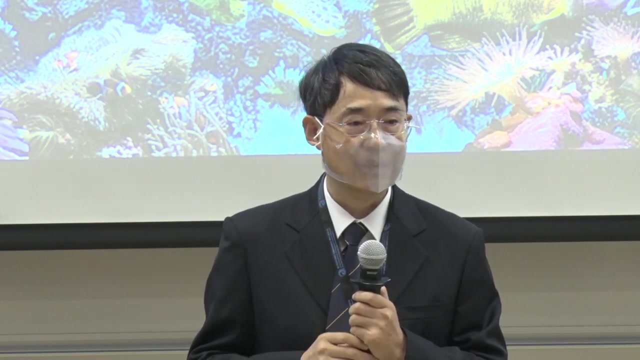 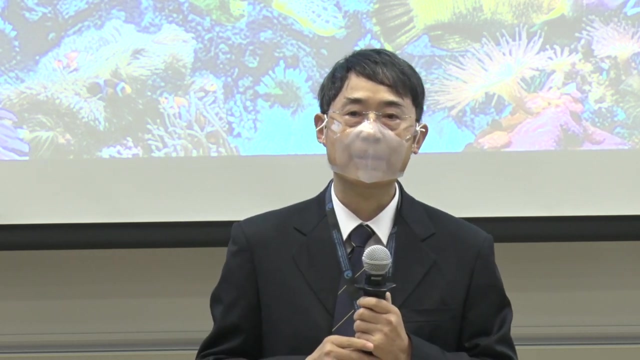 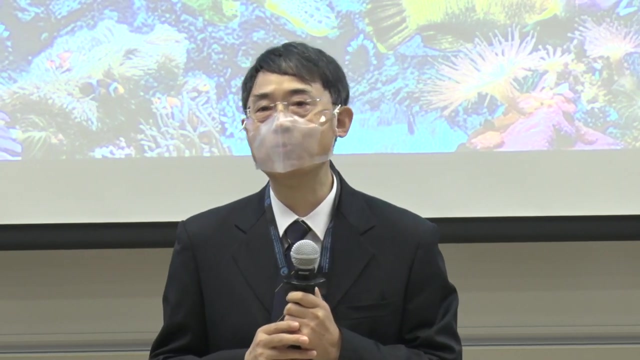 are primarily from land, also the coastal waters, Yet 90% of the hours open, the open oceans, also the ocean environment, remained unexplored to us. The reason is very simple: The vast volume of the ocean environment, which is about over 300 times. 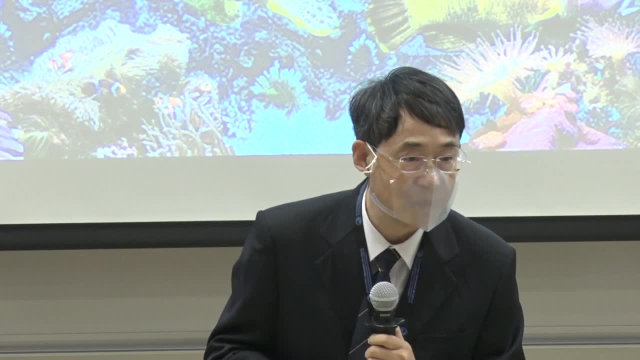 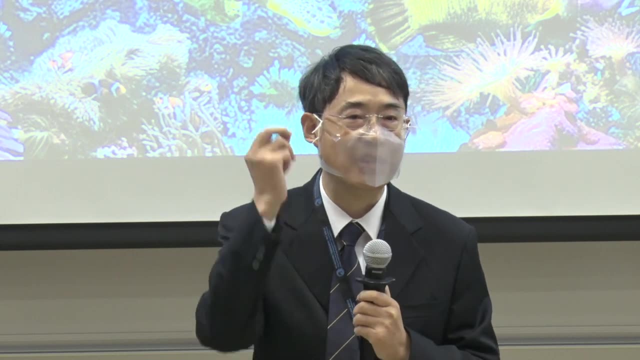 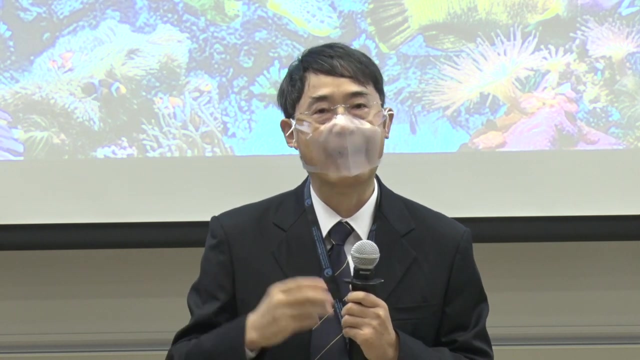 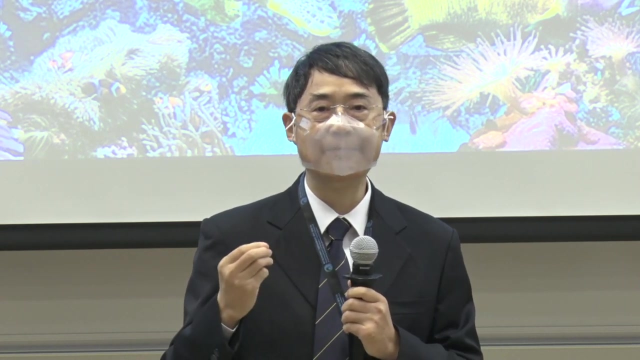 of the volume of the terrestrial ecosystem When we do not know about 90% of it, meaning that we really know no very tiny fraction of our planet. This is really call for great effort for studies, marine biodiversity. UN urged each of the country to develop. 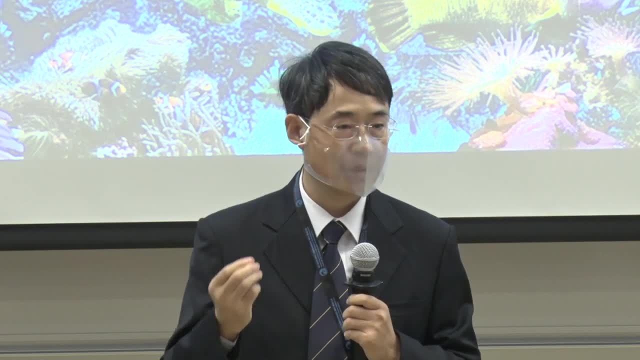 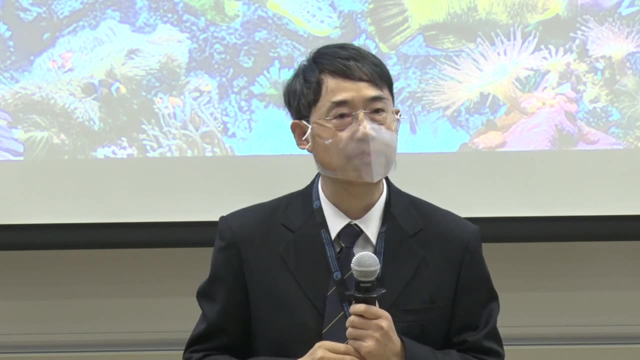 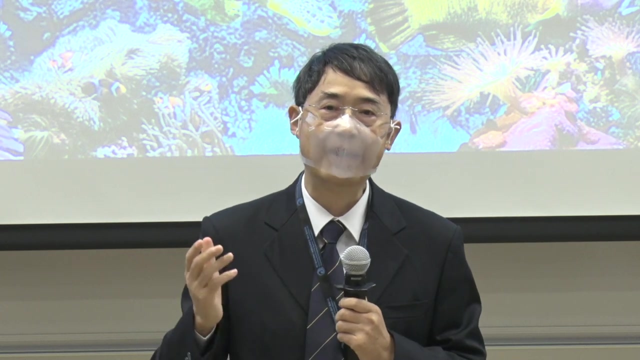 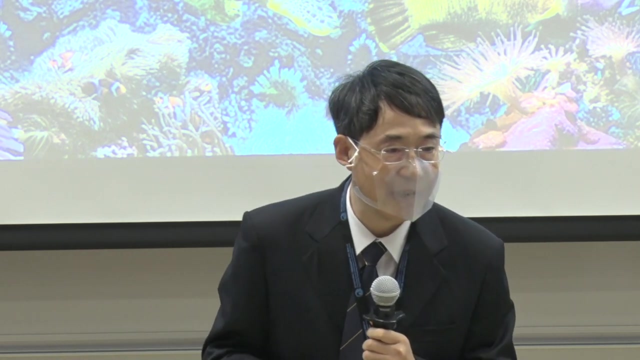 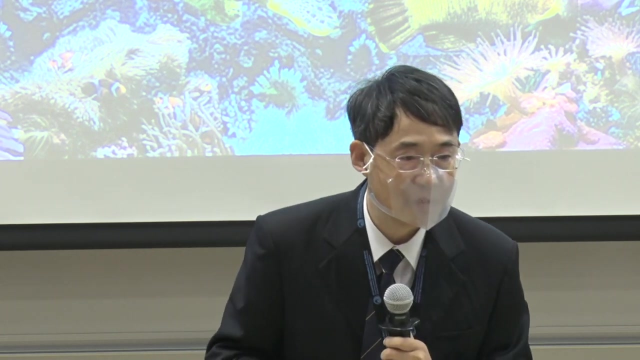 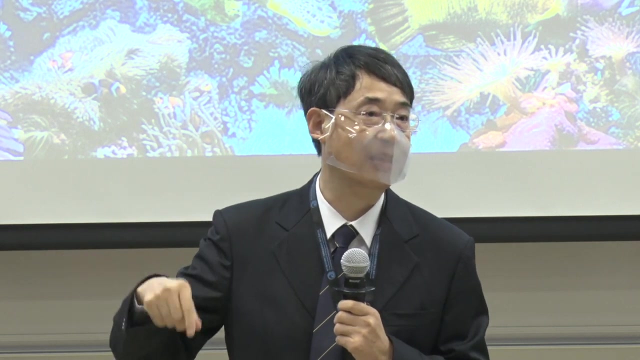 their own strategies and plan to protect their biodiversity, And UN also urged countries of the economy to protect the biodiversity by designating certain area as a protected area. So their goal is 30% of the land or oceans you know for the protection in the next 10 to 15 years. 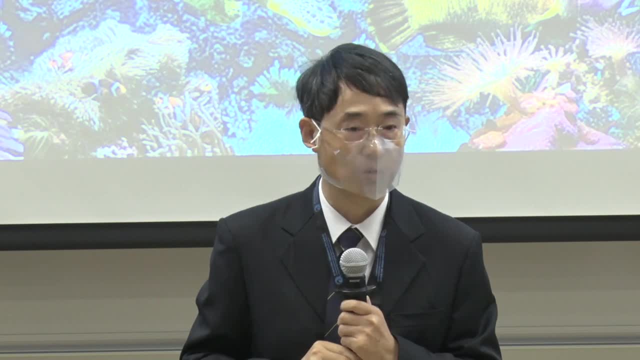 So their goal is 30% of the land or oceans you know for the protection in the next 10 to 15 years. So their goal is 30% of the land or oceans you know for the protection in the next 10 to 15 years, Which is really tough goal to achieve for. 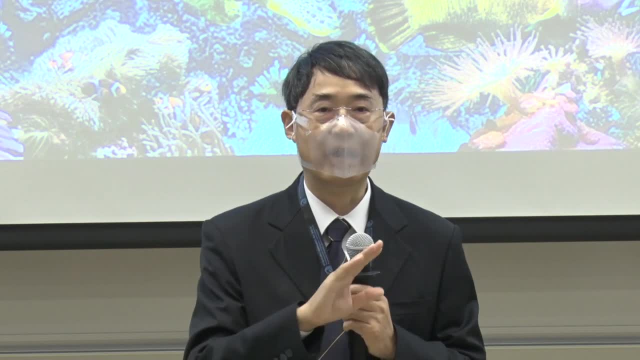 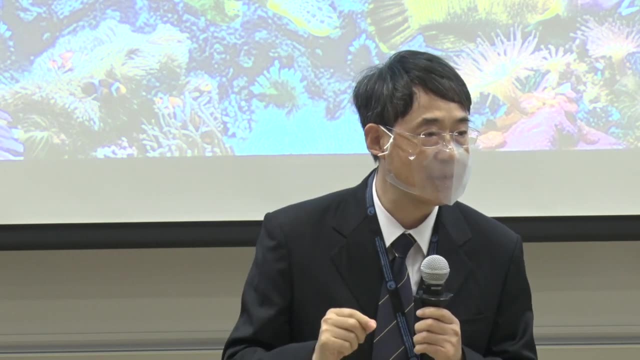 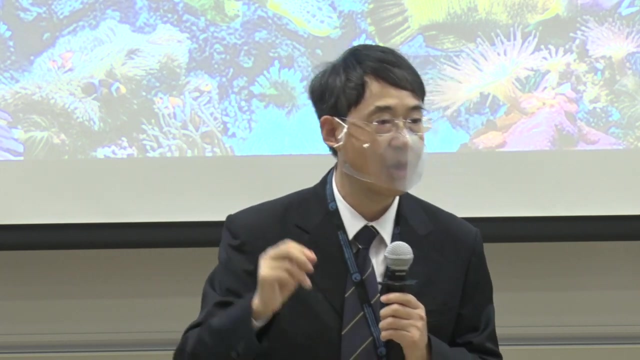 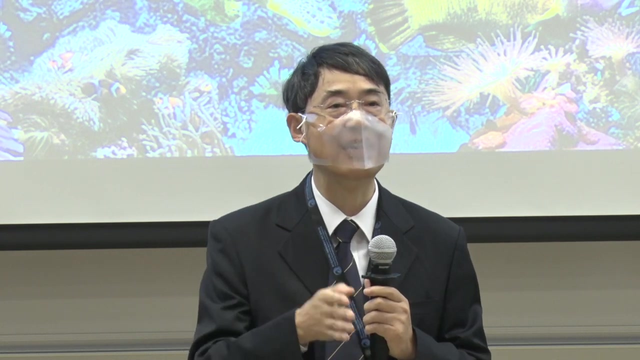 simple reason: Up to this moment, at global skills, on the 17% of land, 7% of the ocean have been served, reserved as the so-called parks, All that are reserved with some sort of the protections. So from 17 or 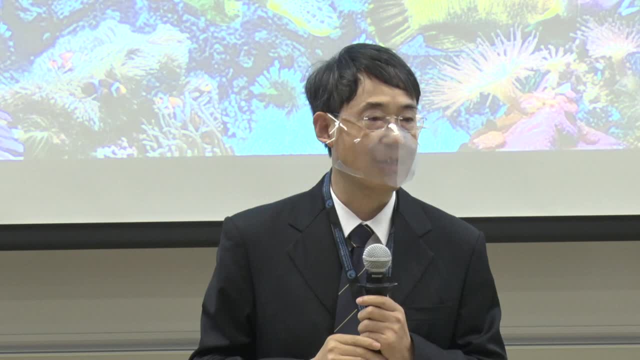 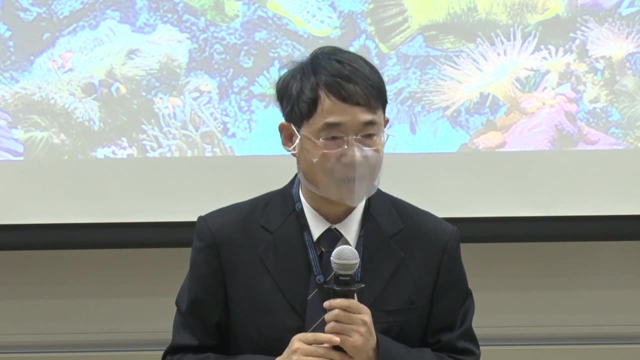 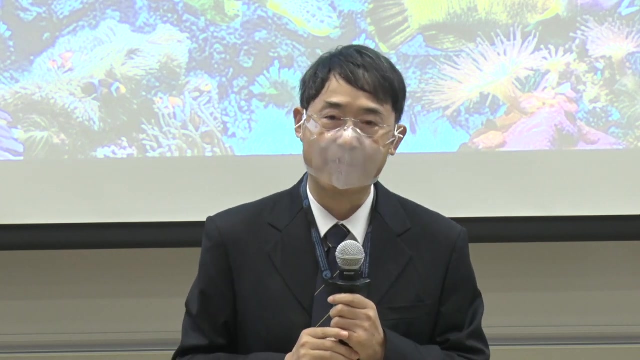 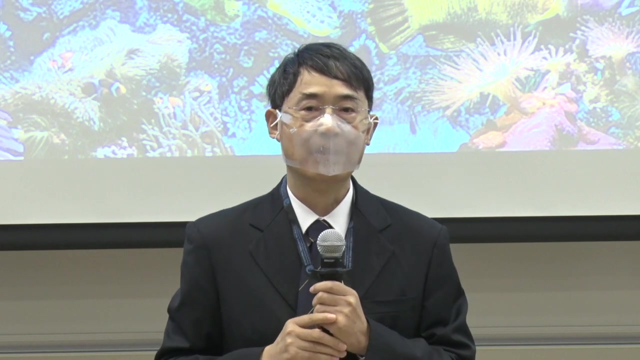 7% to the 30% is a long way to go. This is why we are here to talk about marine biodiversities. So I'm really excited about the talks from our distinguished speakers, all the guests for this afternoon. So welcome you all to this. 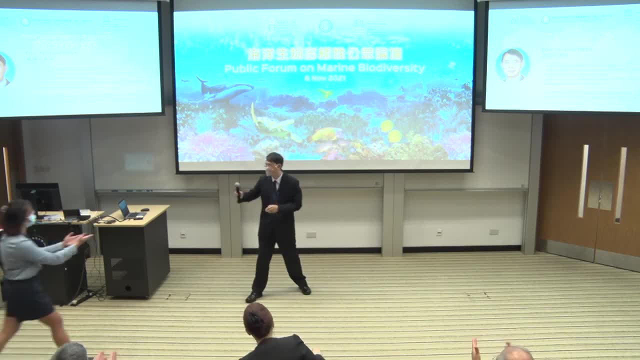 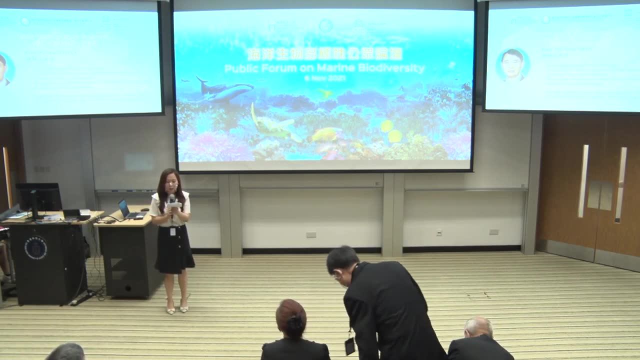 forum. Thank you very much. Thank you, Professor Chen, for a wonderful remarks. As the co-organizer, let's welcome Professor Karen Chen, the Executive President and Secretary General of UNESCO Hong Kong Association, to deliver a welcome message as well. Welcome, Professor Chen. 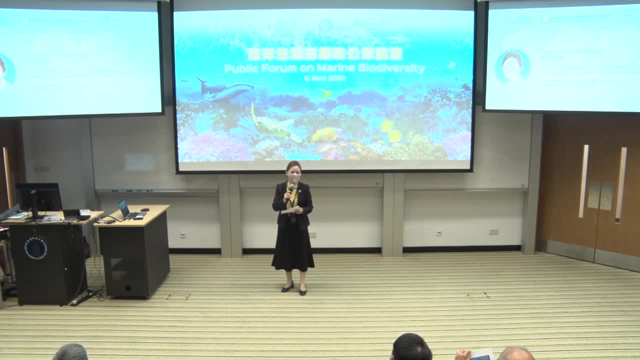 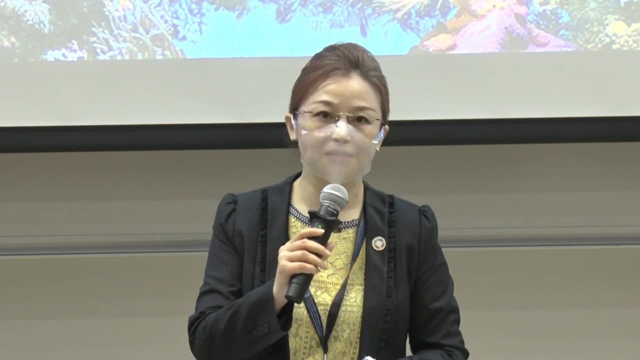 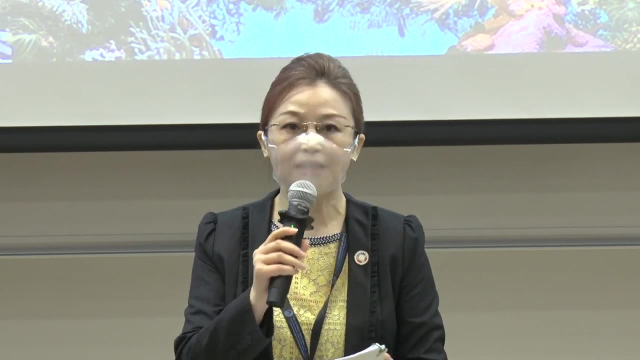 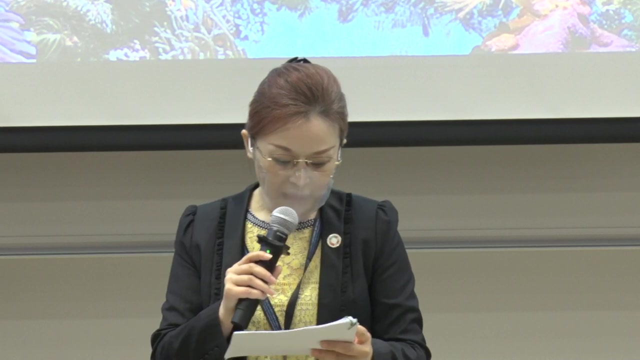 Good afternoon Mr Chairman, Professor Chen, dear speakers, guests, teachers and students. It's my pleasure to deliver the opening address and have to join us this Saturday for the public forum on marine biodiversity. We have invited experts on marine related issues from the 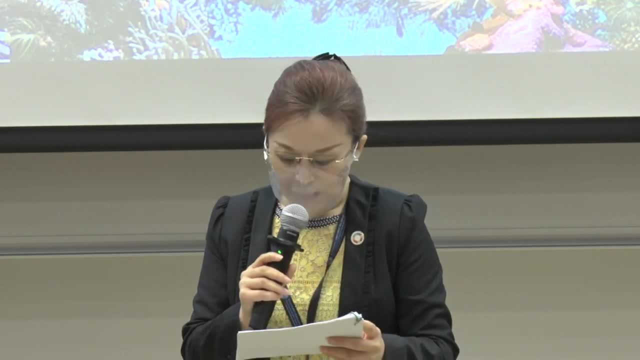 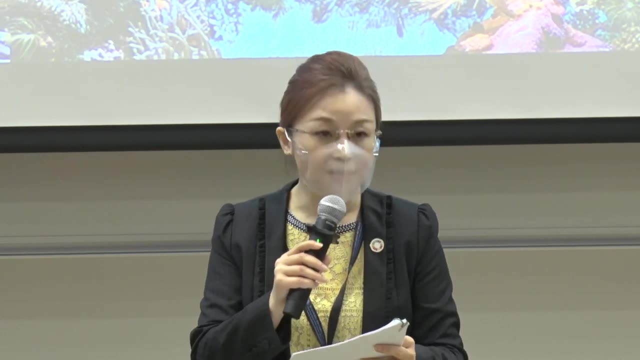 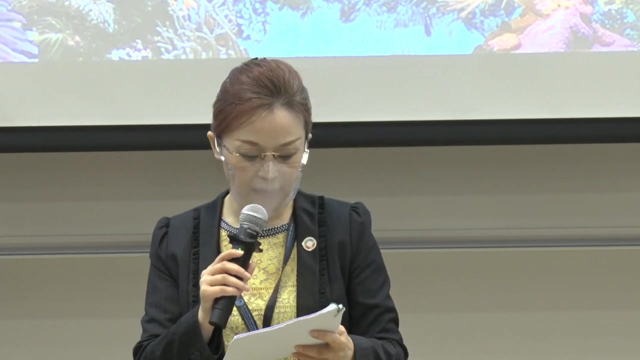 government, business leaders, the education sector and expert researchers and peers to discuss with us the topic of marine biodiversity. There has been increasing discussion surrounding marine biodiversity. as it is directly related to the biggest current concern for all researchers and researchers, please be seated. 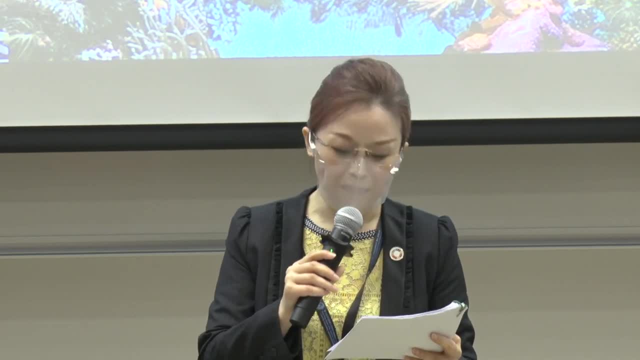 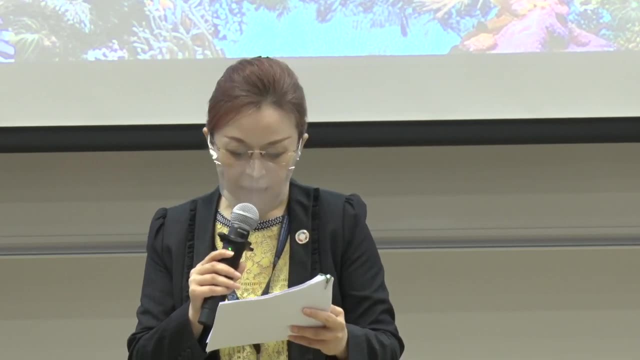 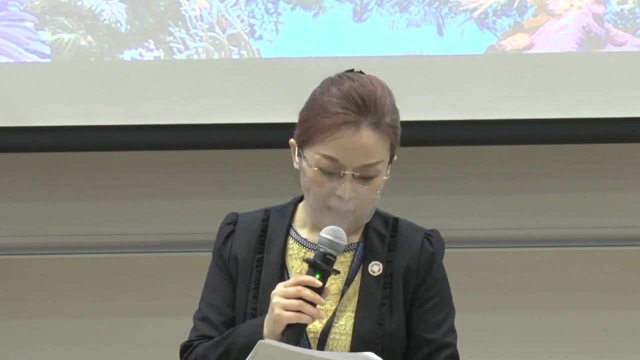 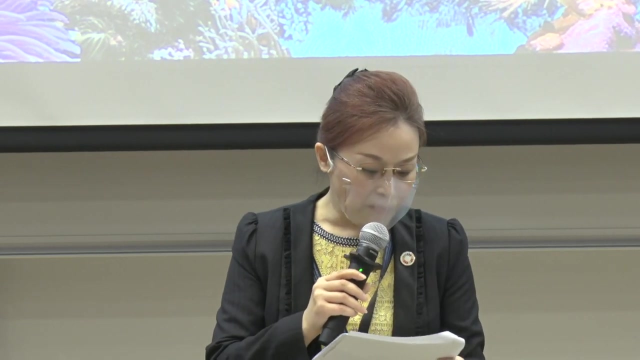 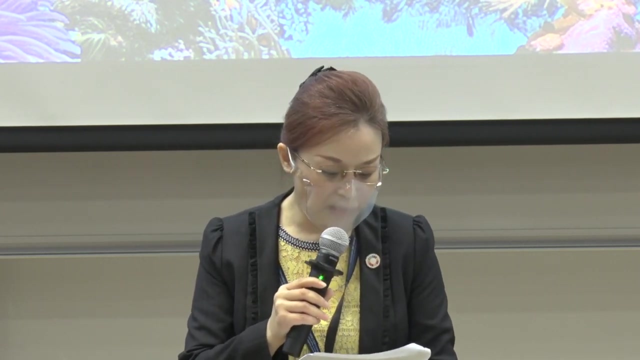 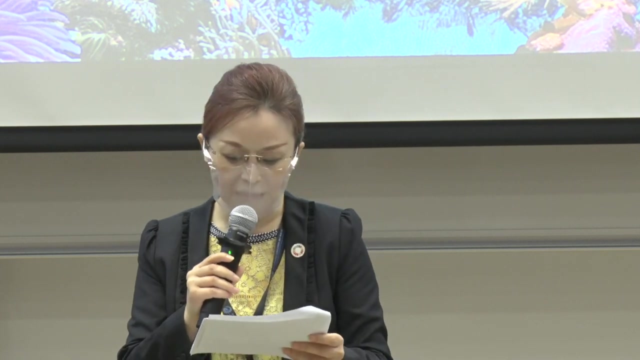 Thank you very much. Thank you. current concern for all nations around the global at present: climate change and sustainable development. the cup 26 is current running on the other side of the planet, from Copenhagen to Glasgow. over the 10 years, our mother earth has experienced huge changes, especially under uncertain, as uncertainties caused. 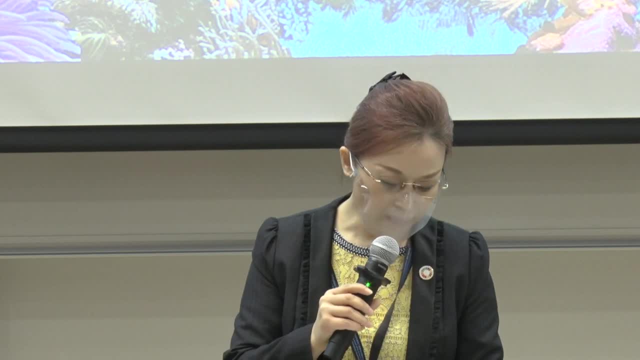 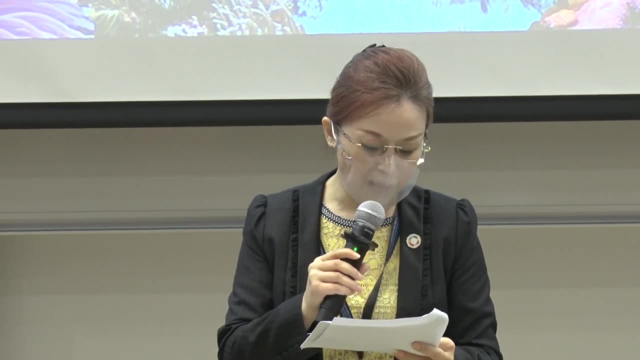 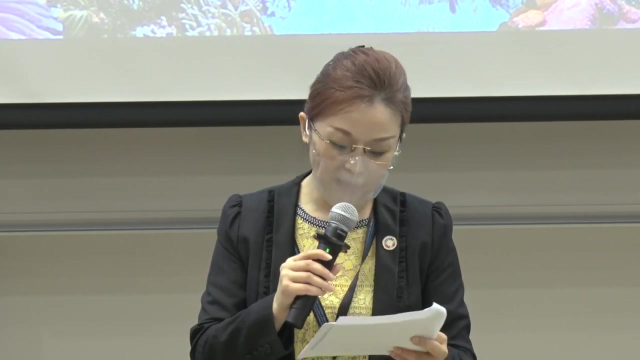 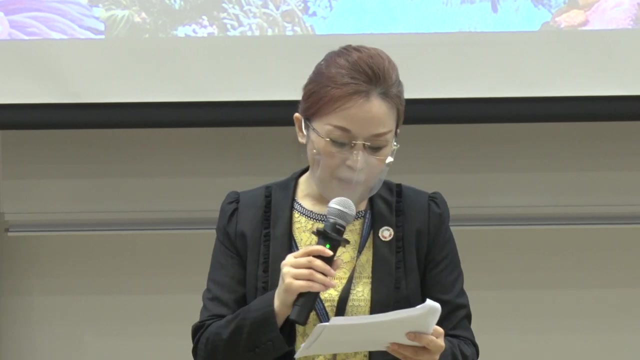 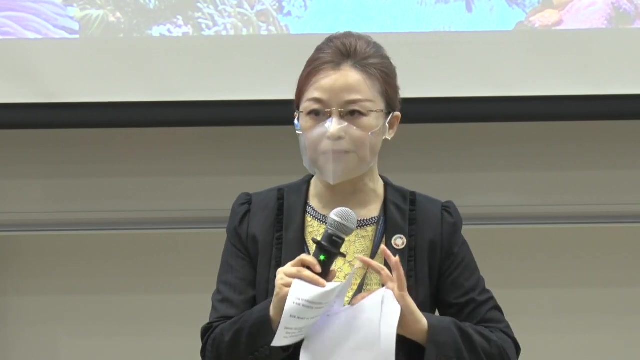 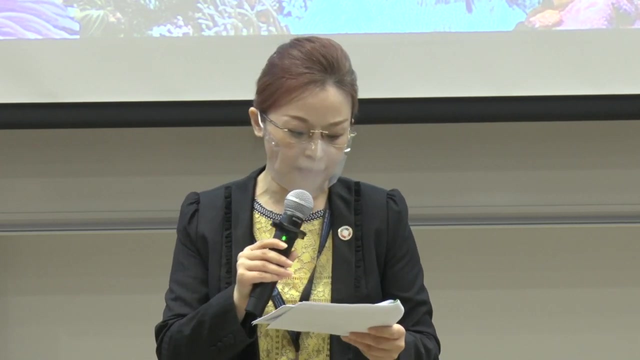 by the cover 19 pandemic. we need to recognize our relationship with the planet and the make systematic transformations. every one of us- government, business, academic, students- are a part of the transformation and ought to take our responsibility in global movement. According to the United Nations, the ocean covers more than 19% of the habitable space. of our planet, and is estimated that there could be as much as 10 million different marine spaces sharing the marine ecosystem with us. However, we have not treated them with care. Climate change and increased temperature has made ocean water more acidic, which disrupted the living environment for marine life. 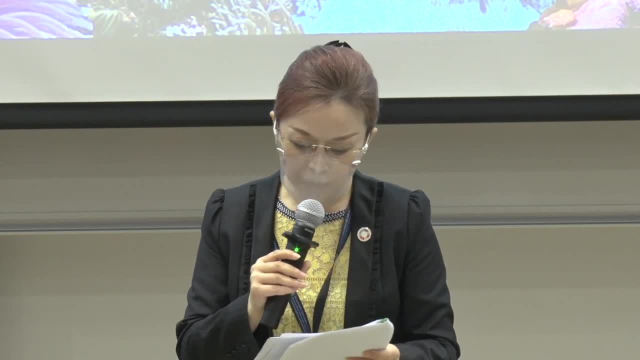 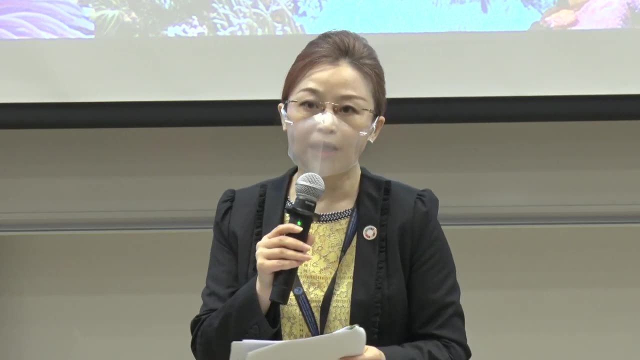 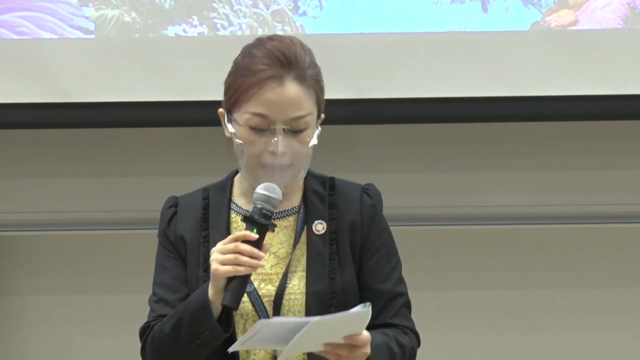 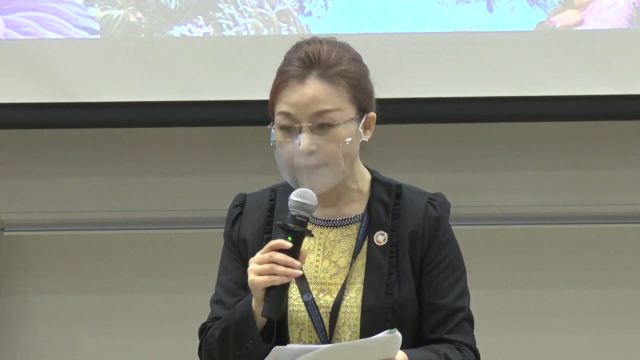 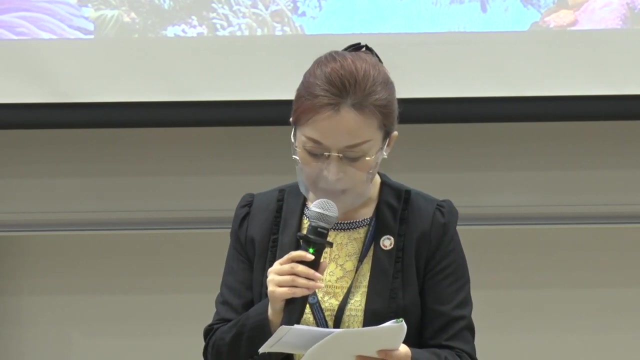 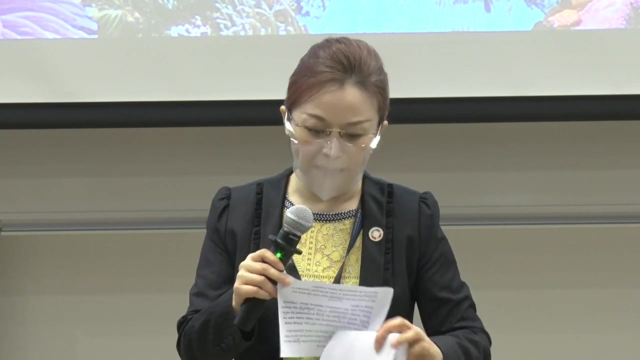 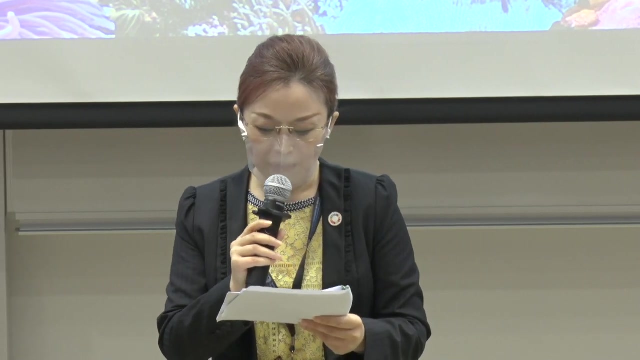 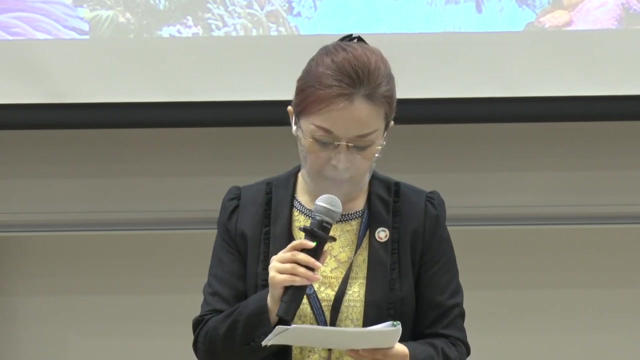 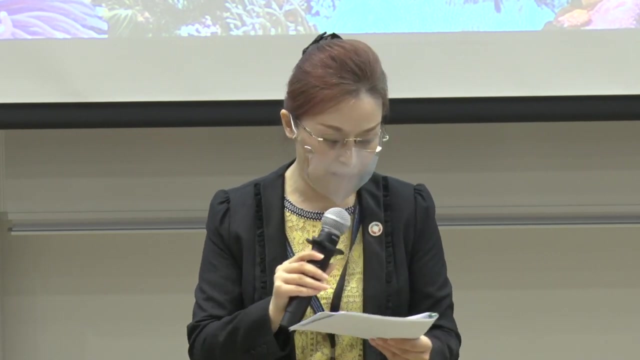 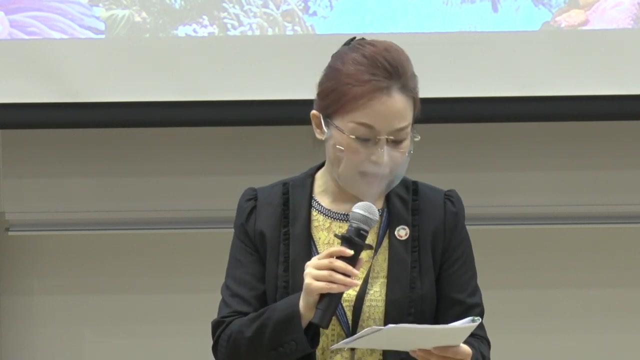 Human consumption of fish prospered the fisheries industry, with fish production reaching about 179 million tons in 2018.. As a result, tourism has also distracted the marine life. The preservation of marine diversity is especially critical for Hong Kong. Hundreds of years ago, Hong Kong was just a small fishing village, but by having the 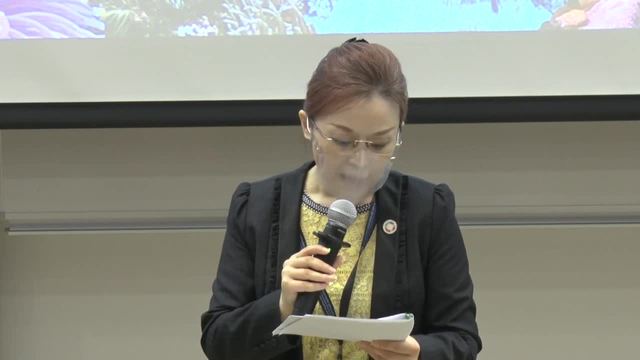 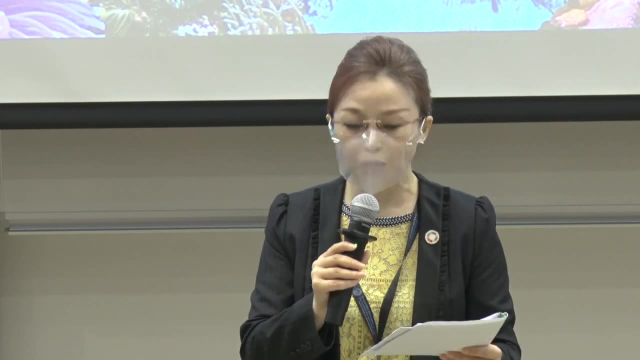 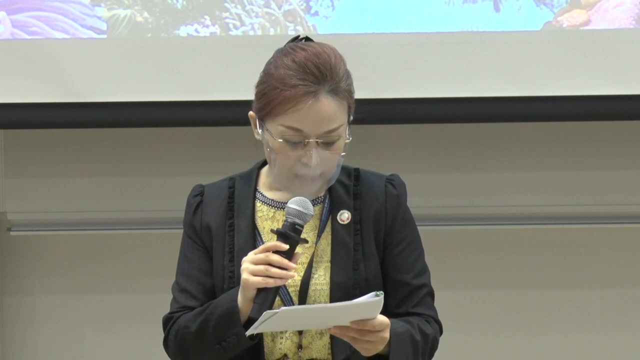 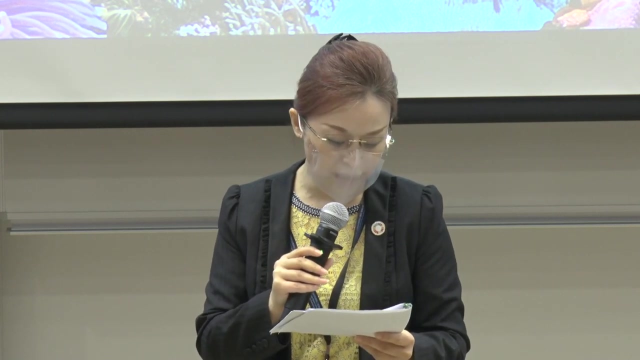 ocean beside us. our economy has grown rapidly from its access to international trade, becoming the global trading and trade hub of the world. The ocean is now the financial center of today. The ocean also provides us with food on our planet- household water used every day. 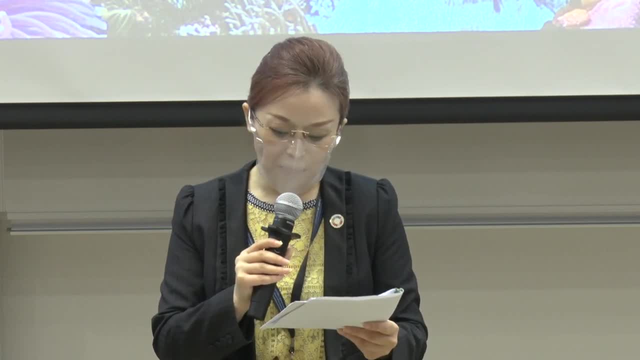 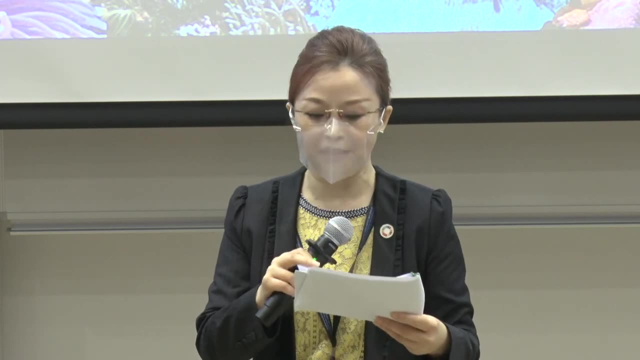 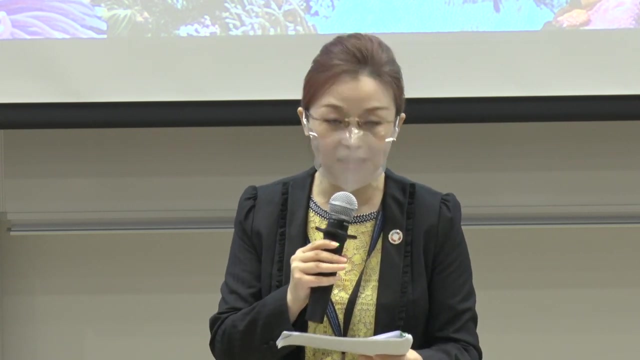 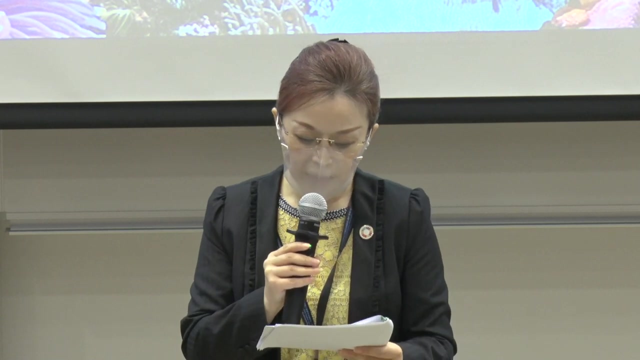 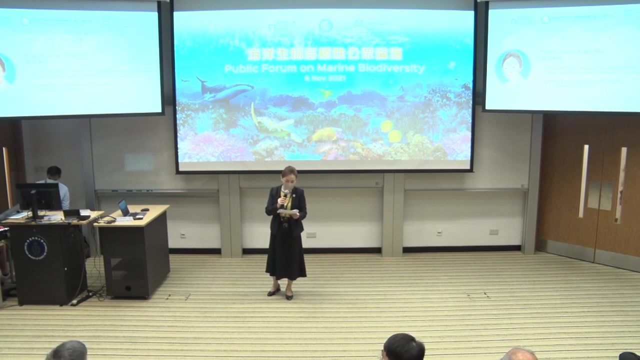 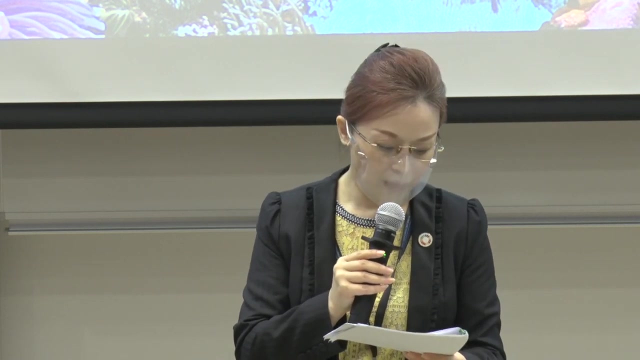 The precious learning resources and marine life are doing a remarkable job of supporting our daily activities. In fact, according to the WWF, Hong Kong waters has very high coral diversity. The Ha Hoi Wan Marine Park alone hosts more than 17% of our local pieces. 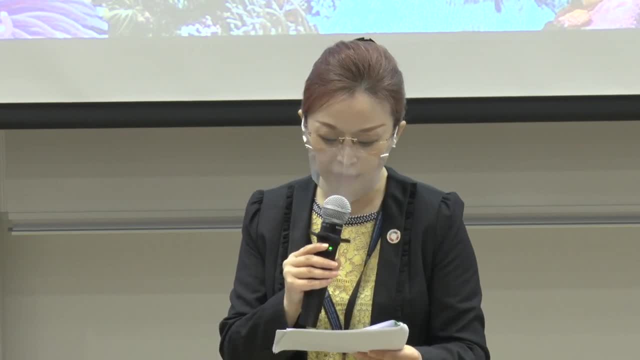 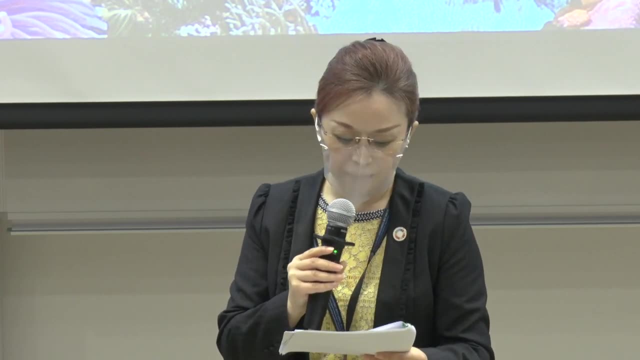 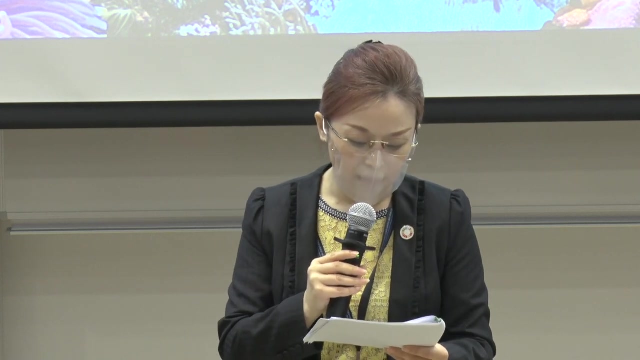 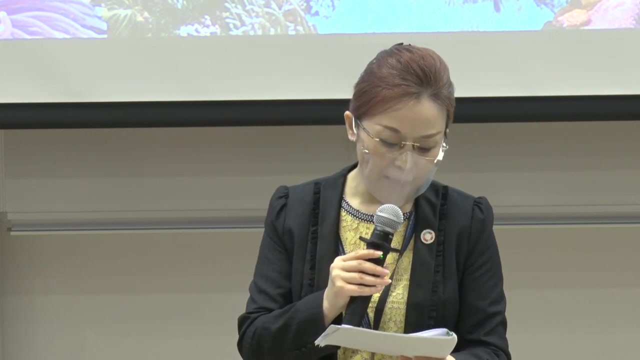 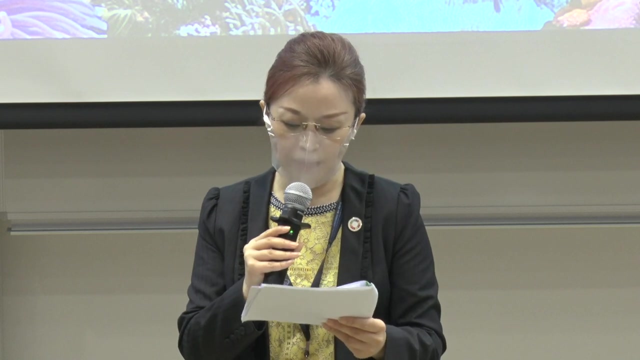 Nevertheless, reclamation of large tracts of marine life is also an important part of the? a due to land shortage and a sustainable lifestyle, filling the ocean up with a mass-practice leader's fashion of ocean and marine biodiversity in Hong Kong. On an international level, UNESCO has established inter-governmental ocean and maritime freedom. 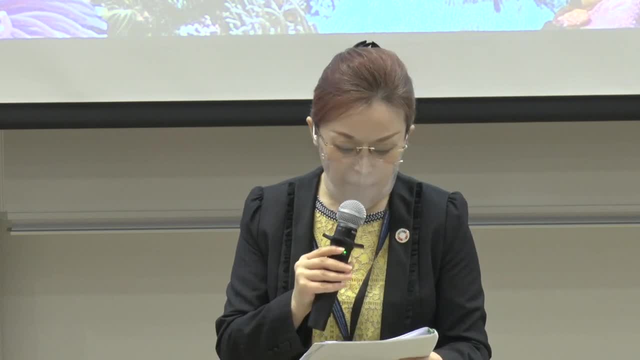 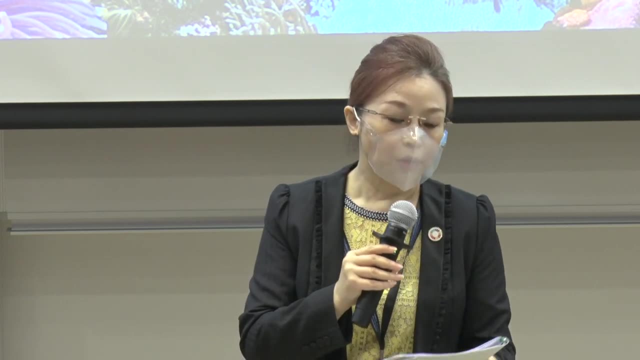 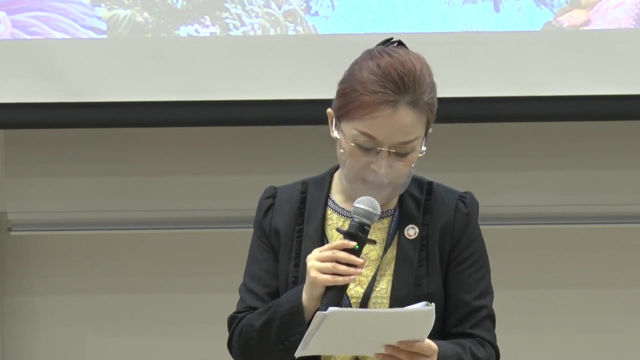 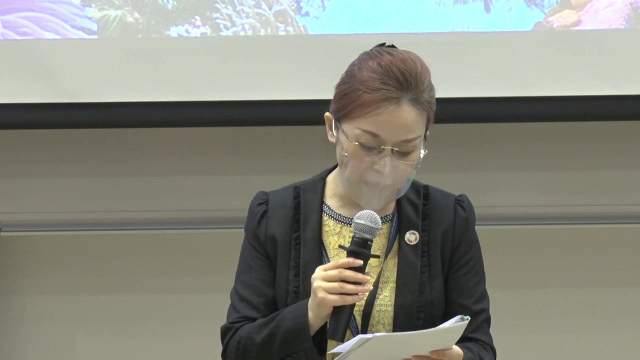 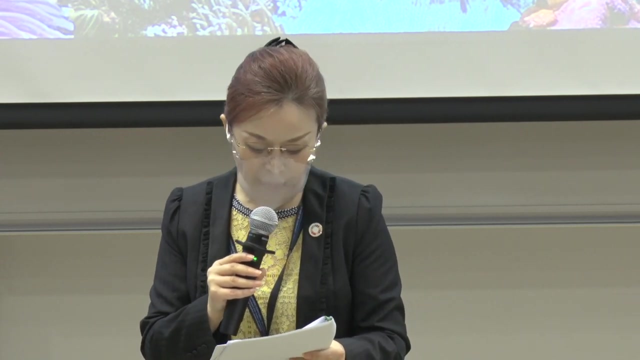 in Hong Kong Ocean Graphic Commission to support research and service on ocean science Regionally. the UNESCO Hong Kong Association, working hand-in-hand with the Hong Kong Institute of Education for Sustainable Development, has followed the five action priorities highlighted in the Berlin Declaration on Education for Sustainable Development. 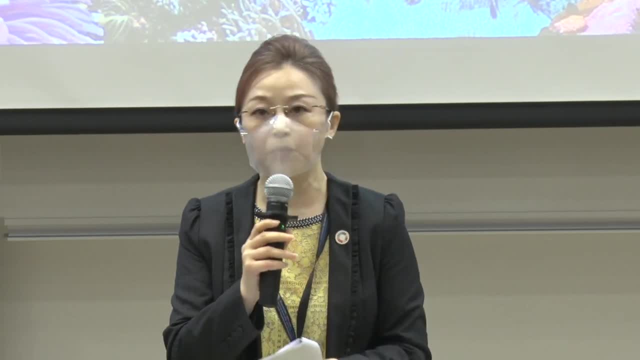 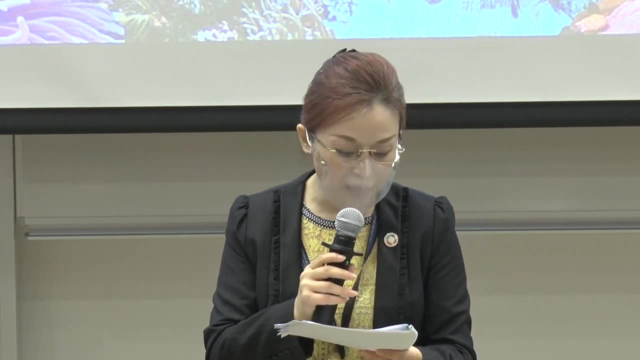 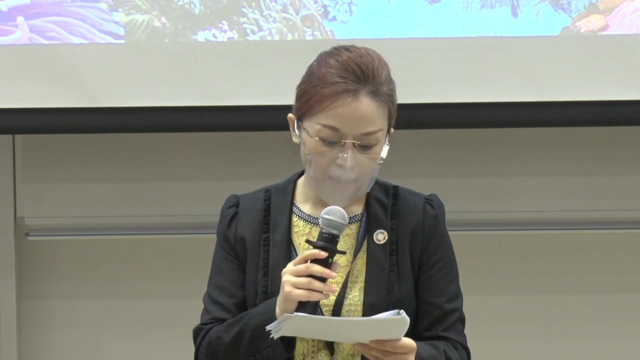 Adopted in May 2021, during the UNESCO World Conference on Education for Sustainable Development, including policy advancement, changing the learning environment, cultivating the capacity of the environment and the development of the environment. The UNESCO World Conference on Education for Sustainable Development has followed the five action priorities highlighted in the UNESCO World Conference on Education for Sustainable Development. 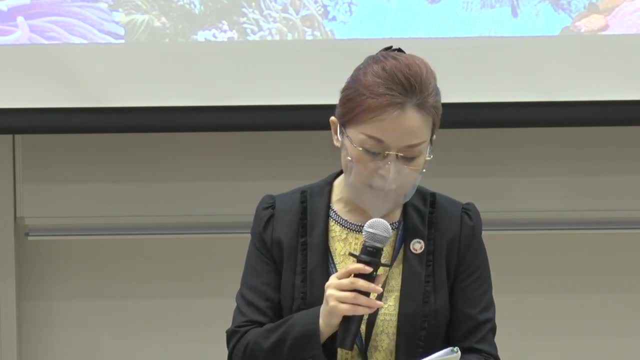 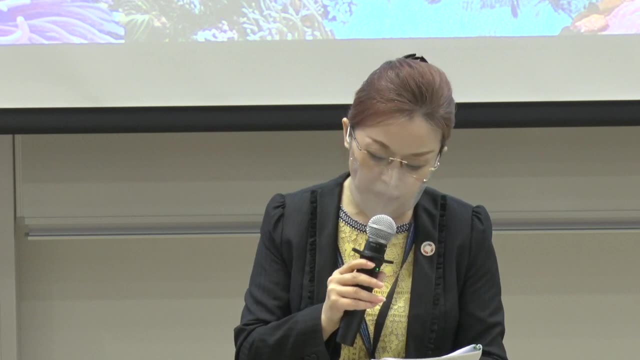 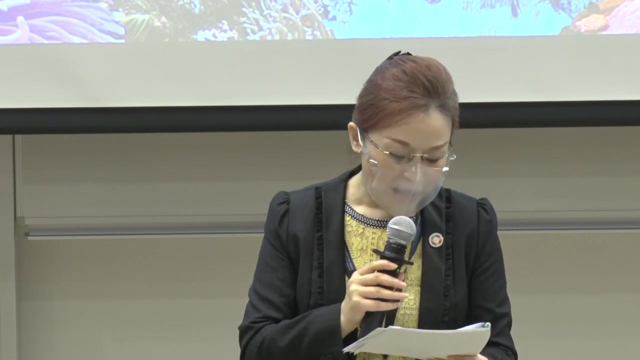 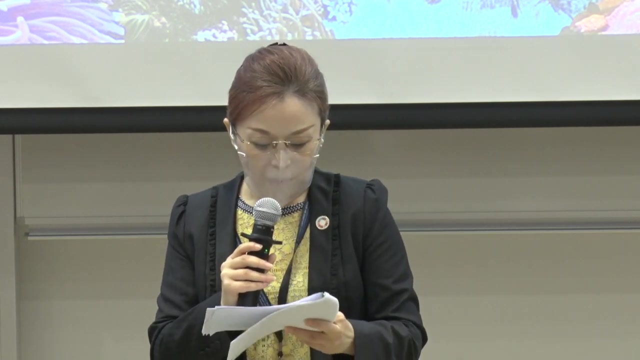 including policy advancement, changing the learning environment, cultivating the capacity of educators, empowering youth and accelerating local actions to promote sustainable development and the achievement of Goal 14 of the UNSDGs- Life Underwater. in Hong Kong, We have worked to engage business leaders and government actors. 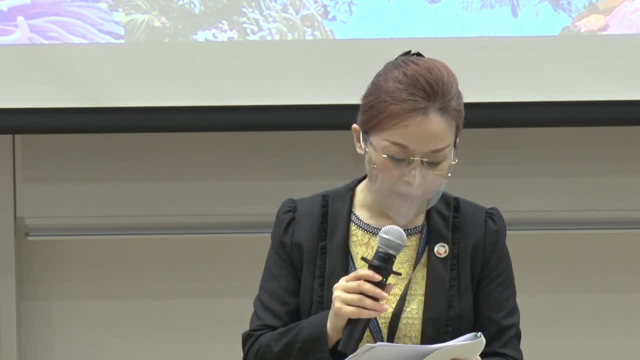 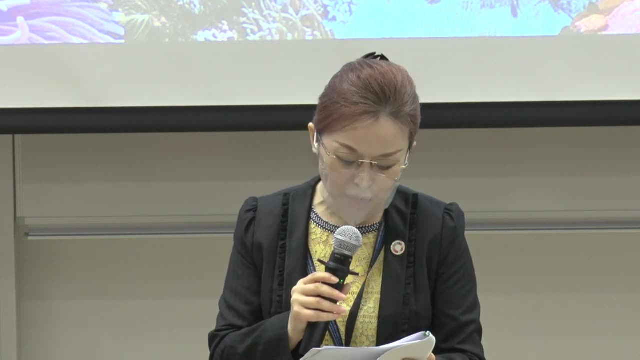 We have also increased the perspective of local and international leaders in the world. For example, the purpose of UNESCO World Conference on Education for Sustainable Development is to promote sustainable development and the universal opportunity for innovation and innovation. This is not an easy task and we would like to encourage all members of the UNESCO World Congress. 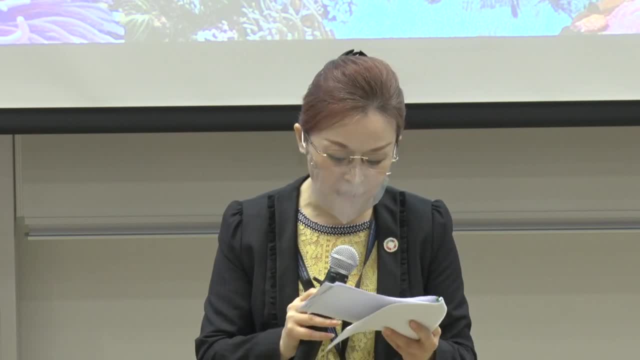 to do so in the future. I would also like to hold a press conference this weekend to discuss the future performance of the UNESCO World Conference on Education for Sustainable Development and the participation and development of modal bins, which is a common demand component in public transportation. 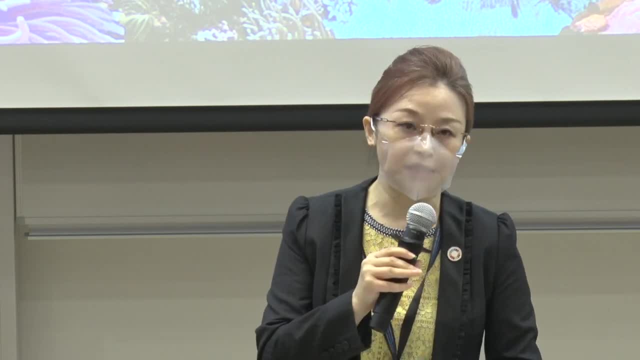 and transportation. We will also share the gedaan work and look forward to the future of the UNESCO World Conference on Education for Sustainable Development, which will grapple with the management and development of the basic skills required to be a people-centered organization. The UNESCO World Conference on Education for Sustainable Development is a public who can share. 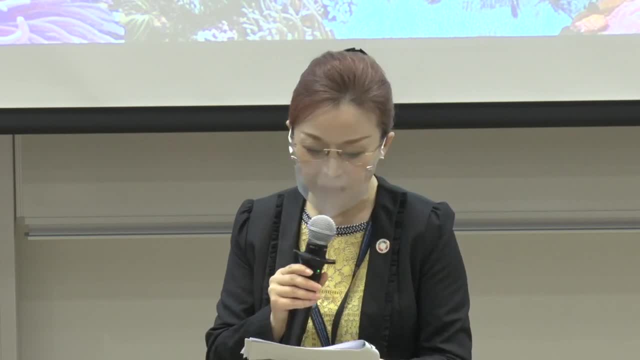 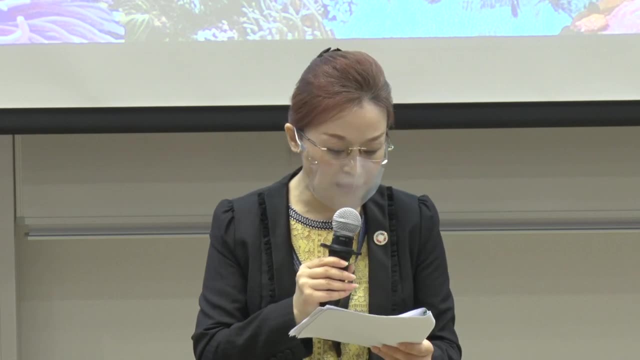 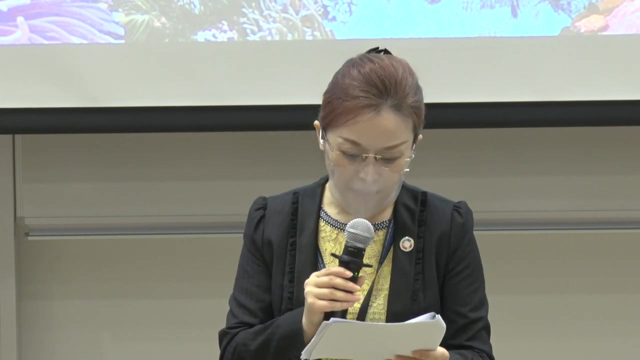 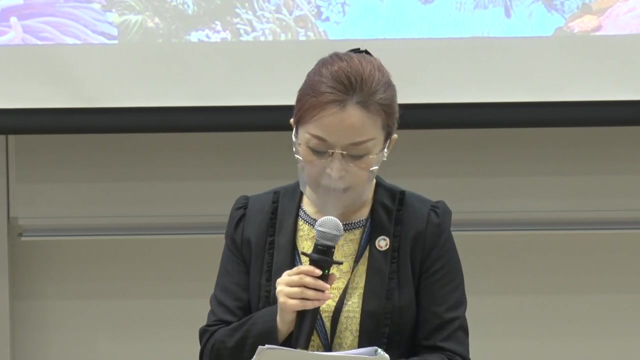 Hong Kong Green Citizen Youth Ambassador Program to give opportunity to youth in Hong Kong to share their perspective on sustainable development on the global platform. Our FreshESD learning program has been running over 10 years. It corresponds to improving learning environment and one of the theme this year. 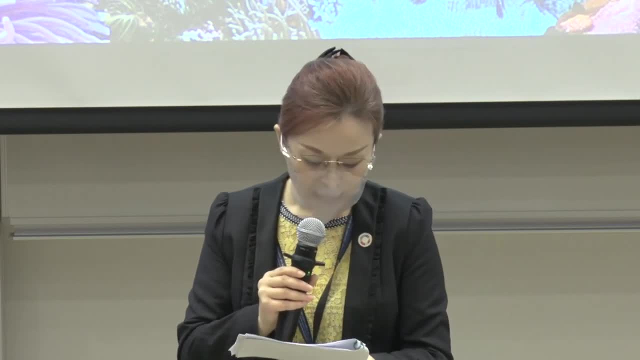 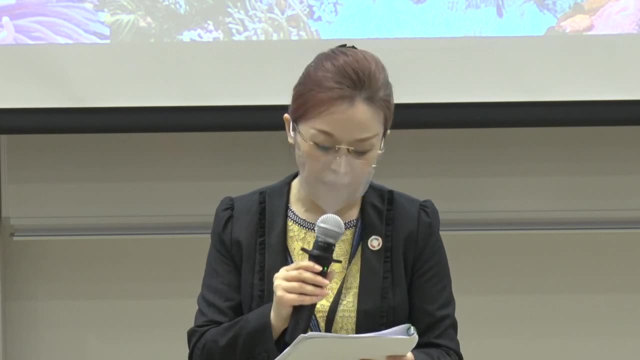 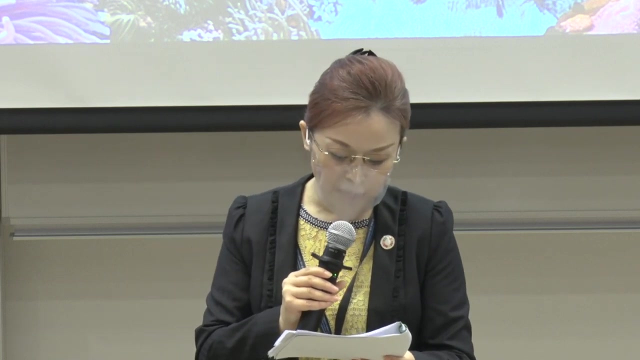 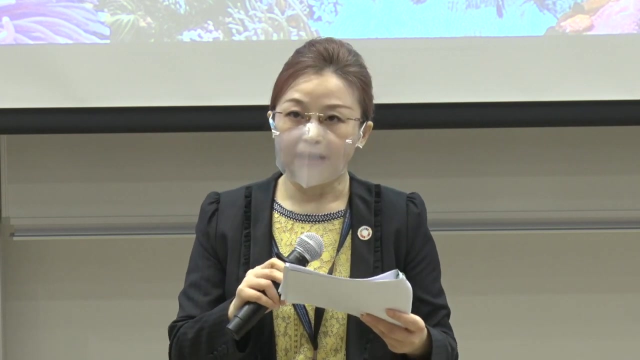 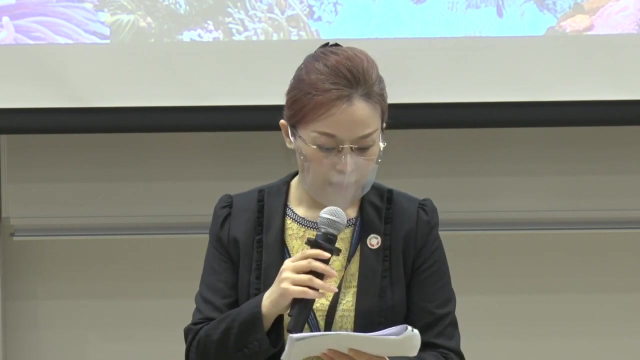 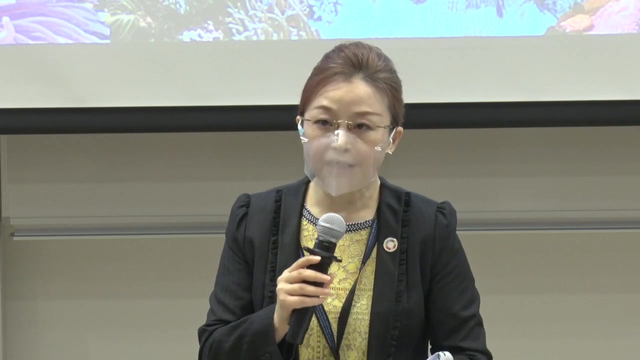 is on marine biodiversity. Students will get a brand of experiential learning and the research-based learning. increasing students' awareness surrounding marine biodiversity issues is one critical part of promoting marine biodiversity. To cultivate the capacity of educators, we provide various training and courses for teachers. 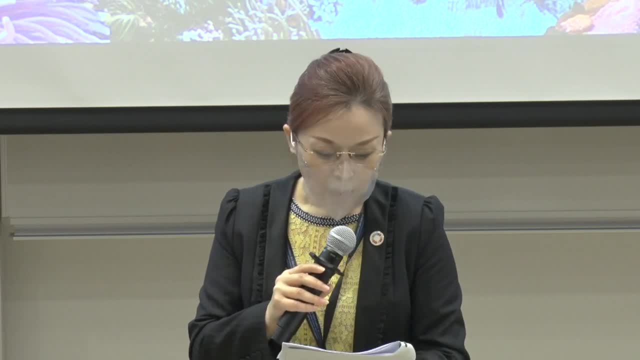 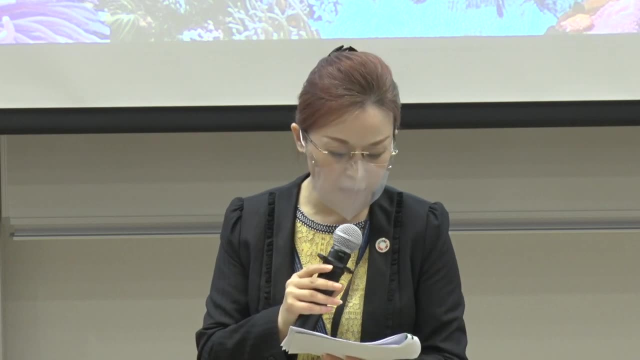 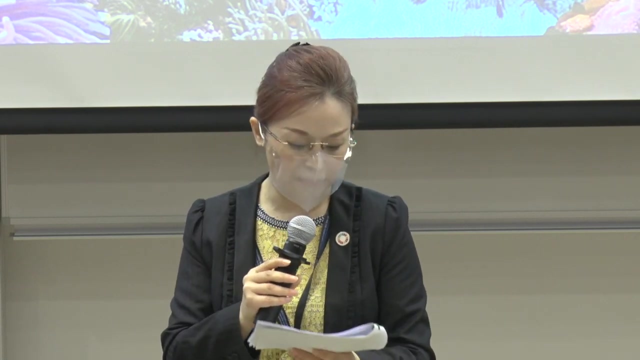 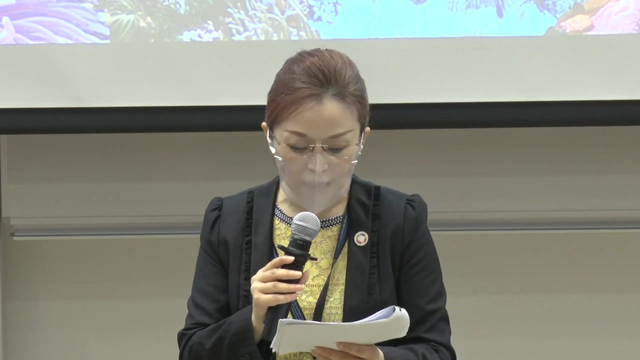 on the sustainable development goals, hoping to educate the educators, to allow them to use SDG content in their teaching and in integrated ESD into school curriculums. Finally, our High-17 SDGs podcast, in which a certified sustainable development planner 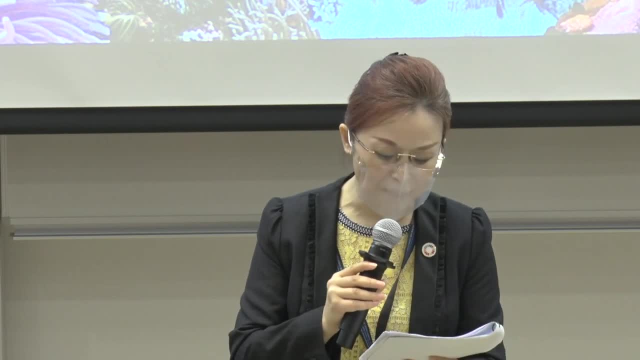 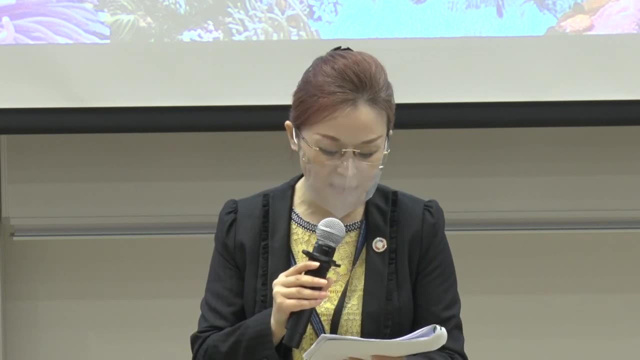 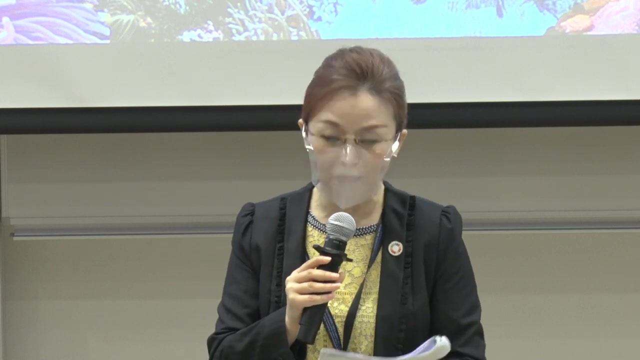 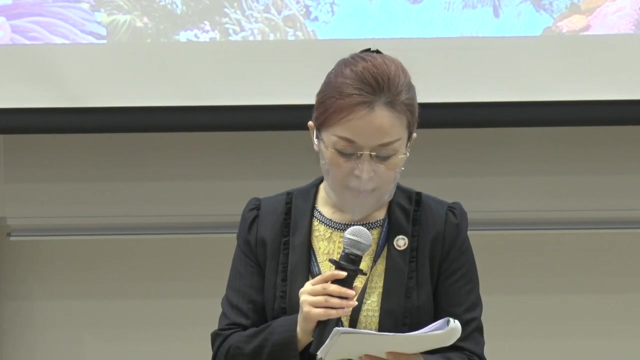 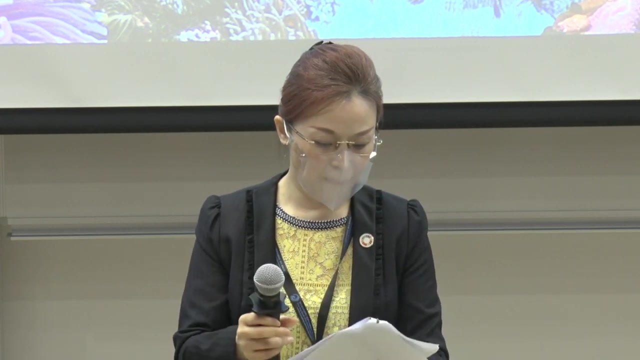 will explain one of the SDGs to the public, each to improve SDG awareness of Hong Kong citizens. Today's public forum is yet another example for our effort to engage communities in Hong Kong in discussion surrounding sustainable development and marine biodiversity With COP26 and COP15,. 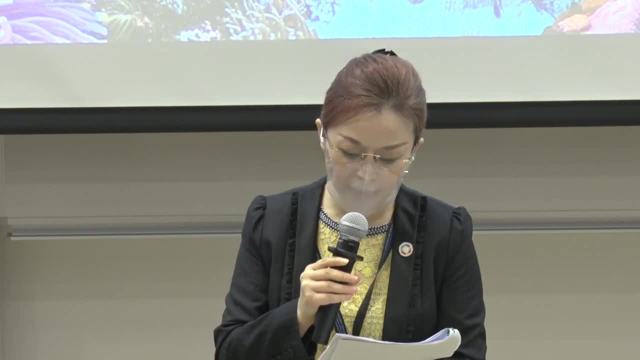 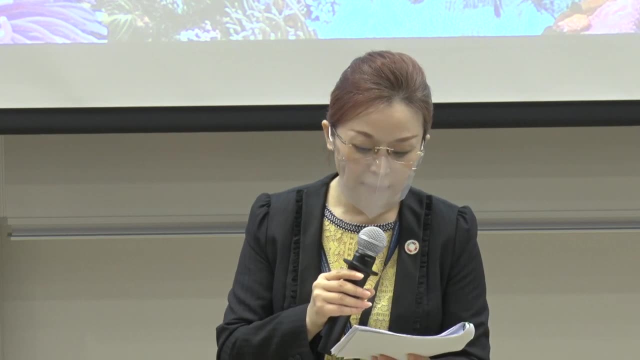 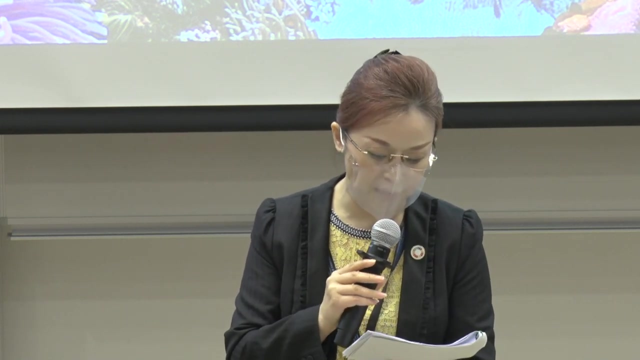 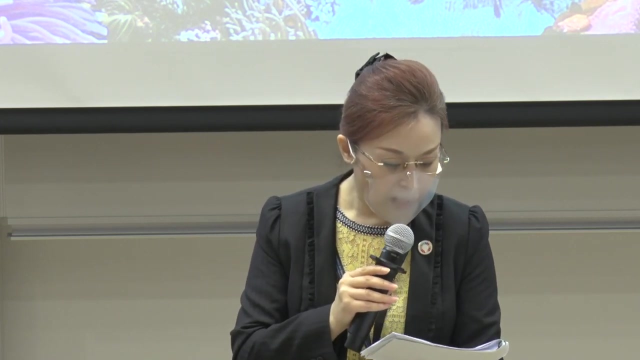 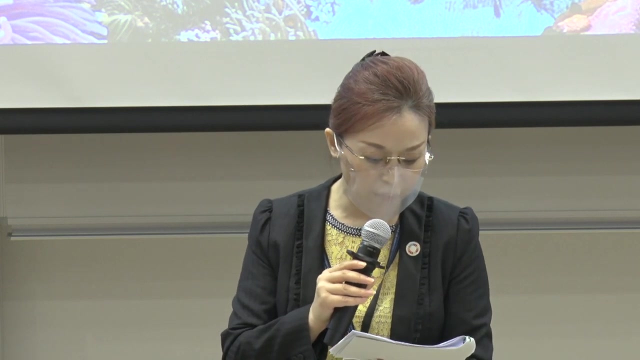 we must realize that the negative impact of human activities on marine biodiversity is pushing the planetary boundary more than ever, Different parties of the societies and professions in different industries needed to work collaboratively to increase marine biodiversity and to transform the current status to a more sustainable future. 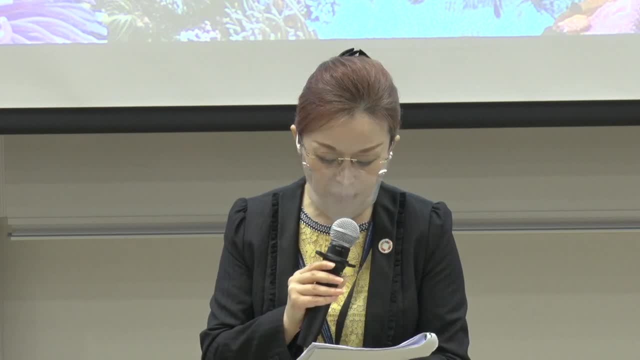 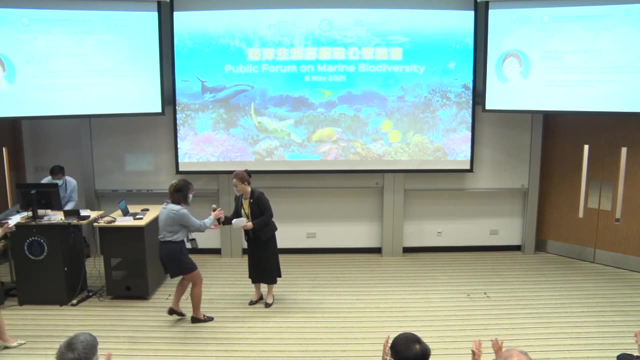 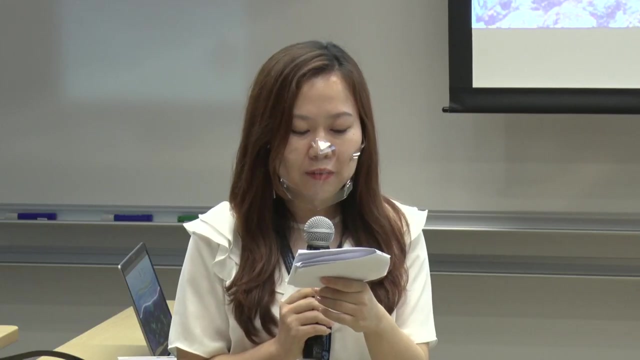 I wish the forum a great success And please look forward to exciting talks. that follows, Thank you. Thank you, Professor Chen. Thank you. Today we are also honored to invite the former secretary for the education of the Hong Kong government and also the honorary president of GHK-MGBA. 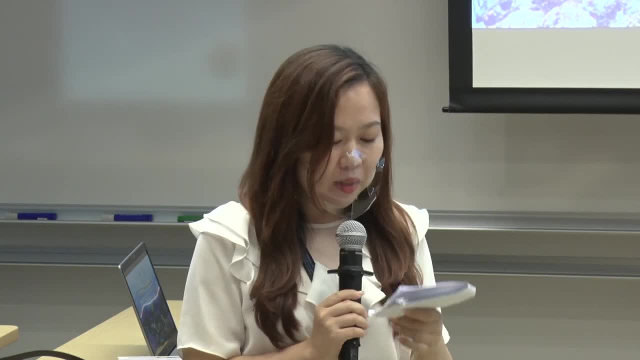 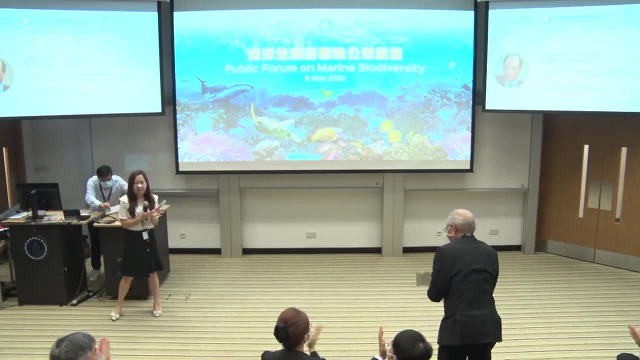 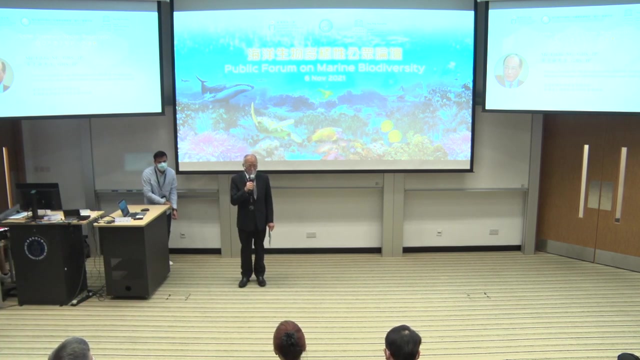 Economic and Trade Institute, Mr Eddie Ng, GBSJP, to deliver a keynote speech first. Please join me in welcoming him. Thank you, Please join me in welcoming Mr Ng. Thank you, Professor Chen. should I call you Madam Cheung? 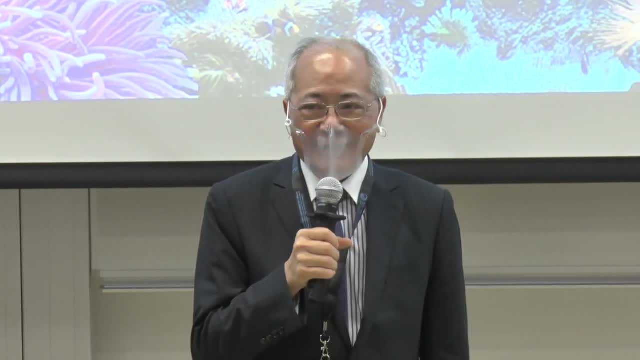 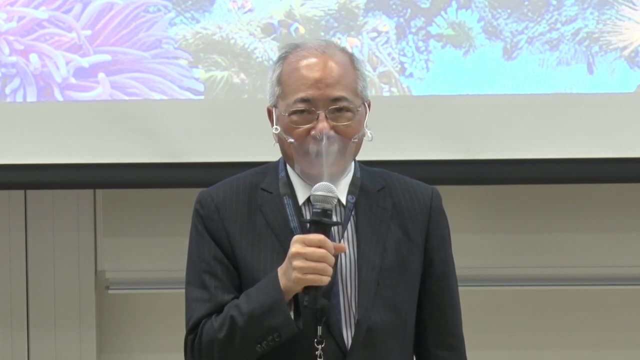 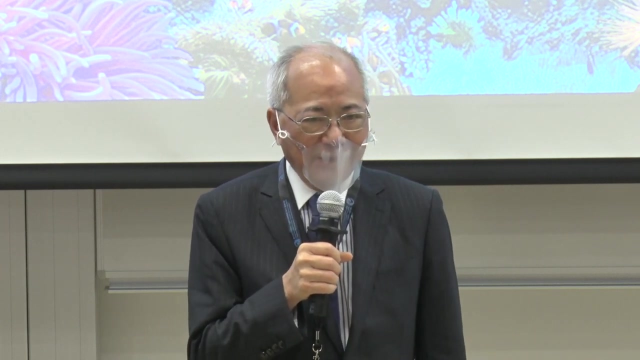 or Professor Cheung And our distinguished speakers, gentlemen, all the attendants, good afternoon. You can sense that my sound, my noise, is picking a little bit shaky because in front of all the experts, I'm not sure what I would be talking about. 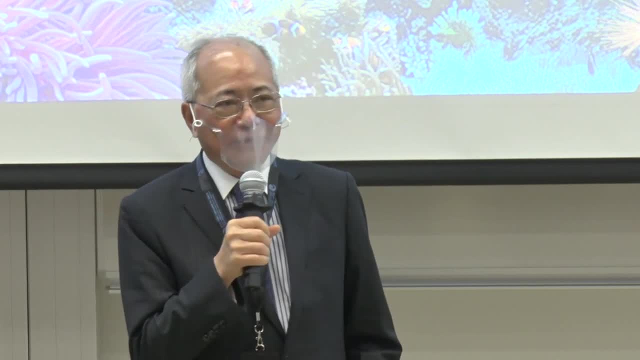 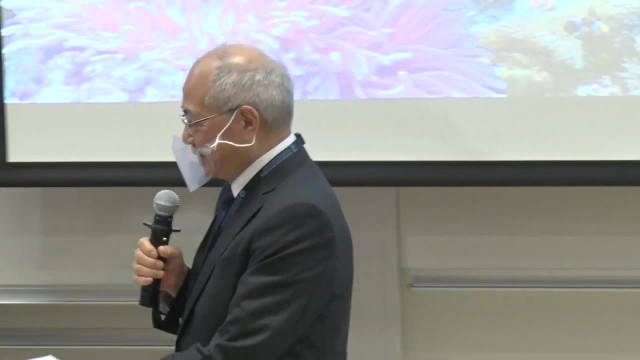 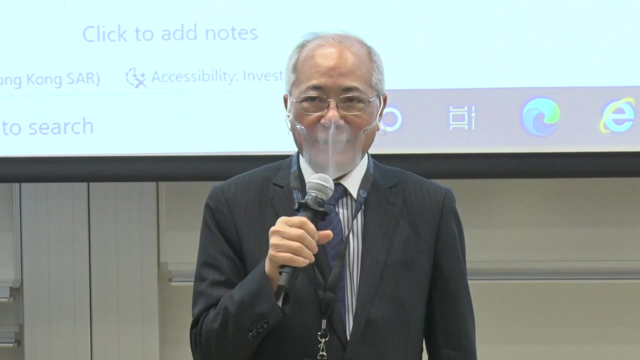 Yet better preparation is always helpful. That's why I have prepared about two hours PowerPoint. So with this one I think I will be able to address that. So I'll run through that very quickly. The idea I really want to say is: a week ago. 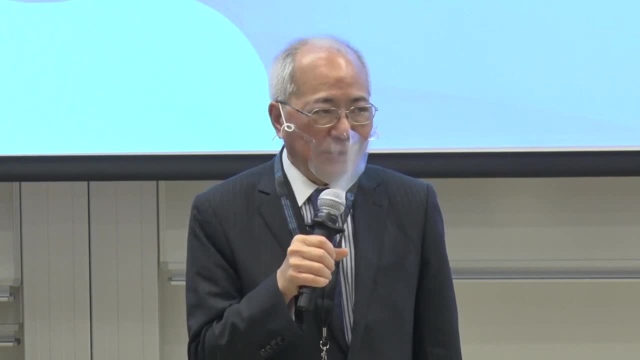 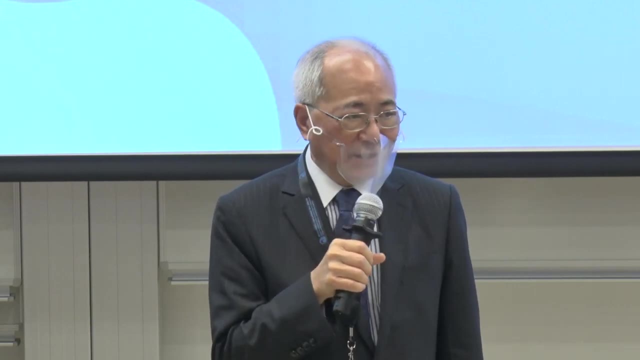 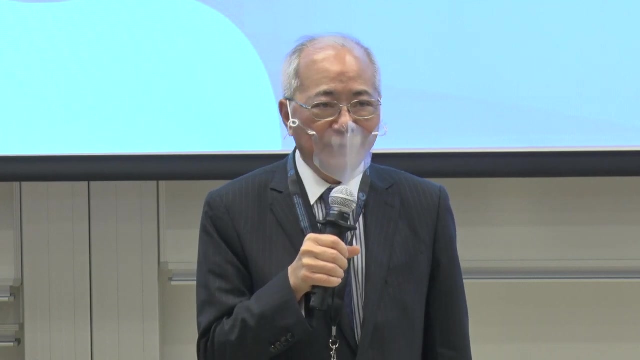 a week ago. I have not much knowledge, idea about what is the marine biodiversity is, But now I think I have some idea what it is, When I have the guts to relay that to our environment, to our focus. Hong Kong- greater Bay areas. 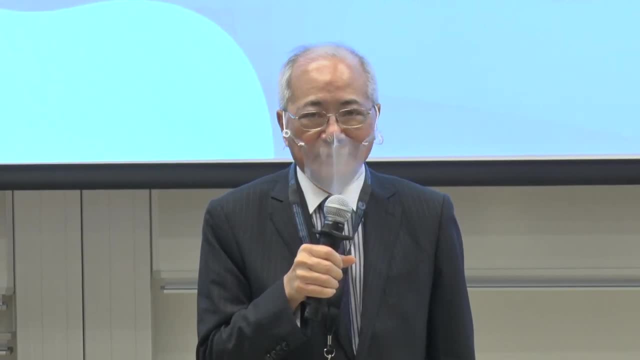 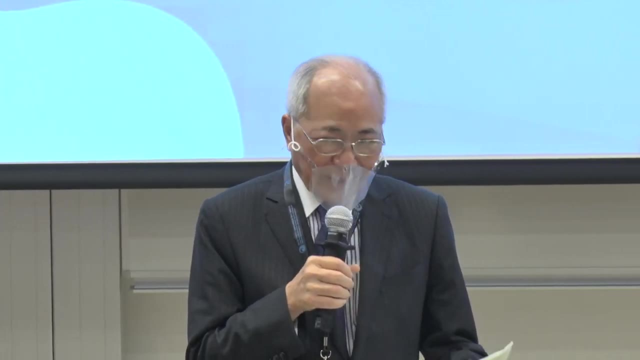 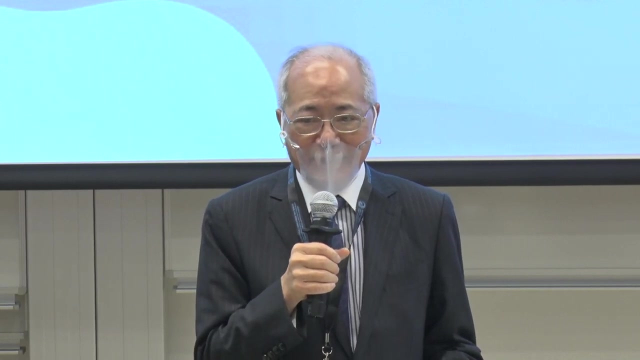 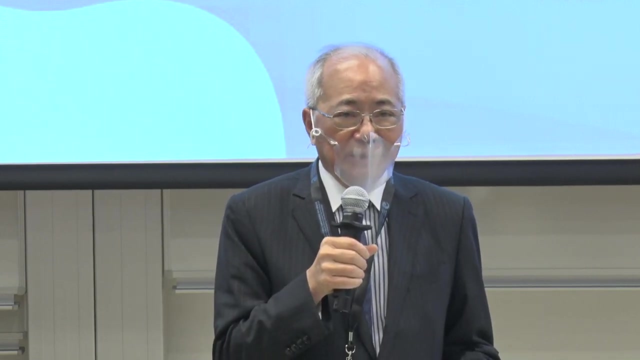 mainland region internationally. I think I have better confidence to talk about the subject Again. we really want to congratulate the UNESCO Office and UST for great work done together with the Southern China Institute. COP 15 is the number we need to remember. 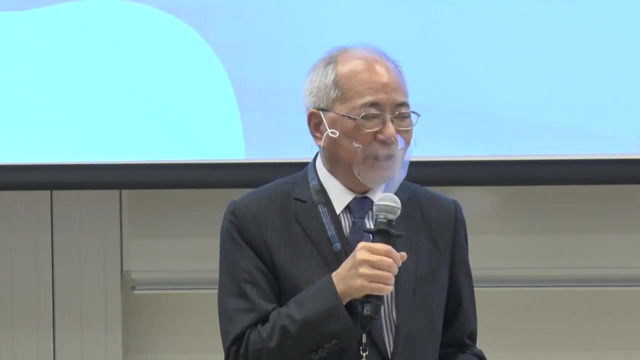 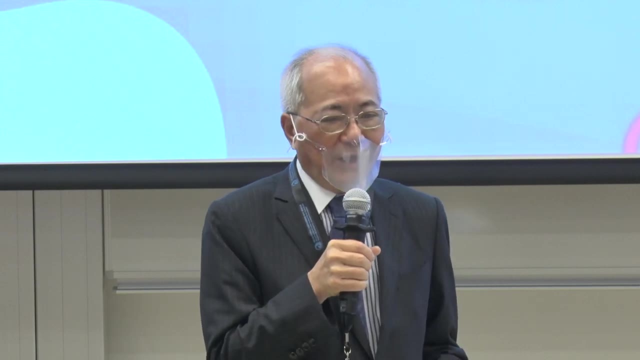 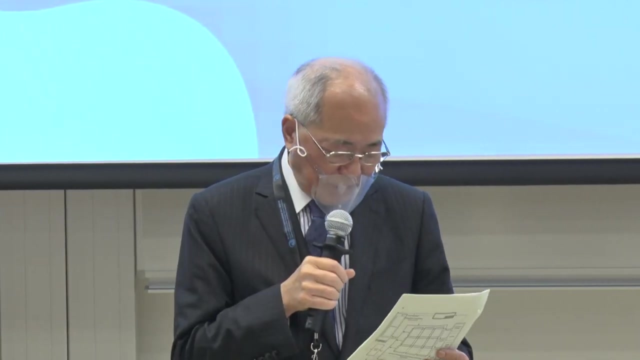 It embodies a lot of things. If you want to have a good reading, try this topic. It will consume you at least two weeks of the Google reading. at least two weeks, 24 hours per day. I do remember on the COP Conming in China. 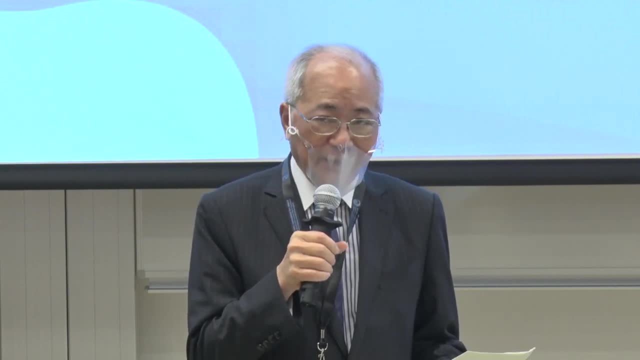 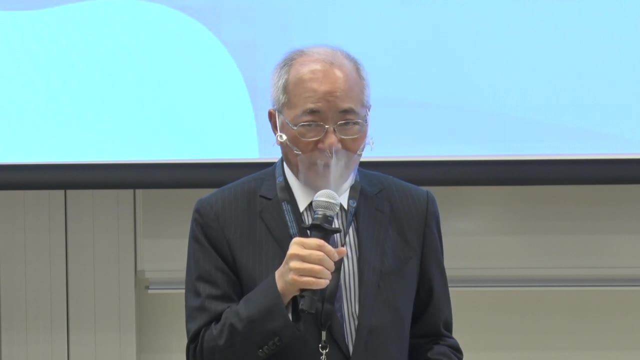 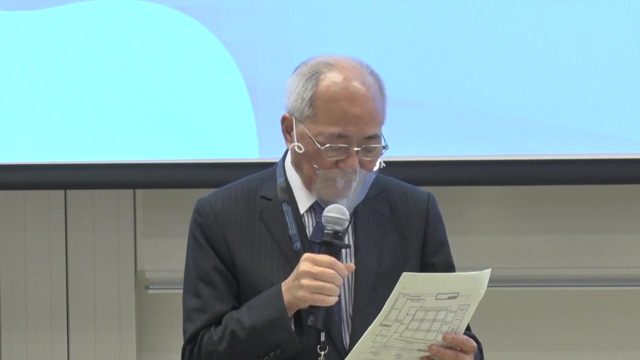 that was, I believe, October last year, and then the President ceased talking about that one. Initially, he just said: well, let's start the conversation with one simple thing. This is important, So I put up the COP Conming Biodiversity Fund. 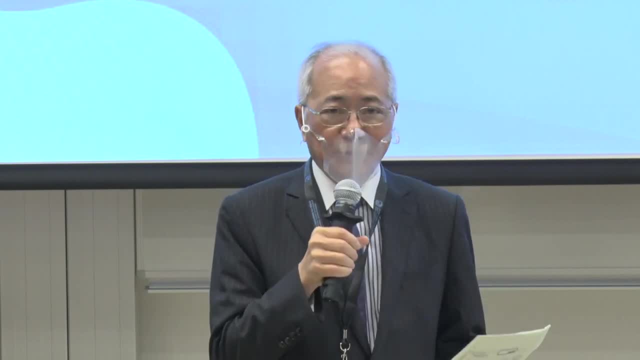 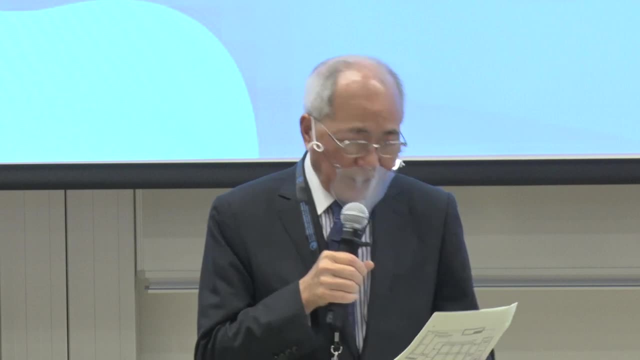 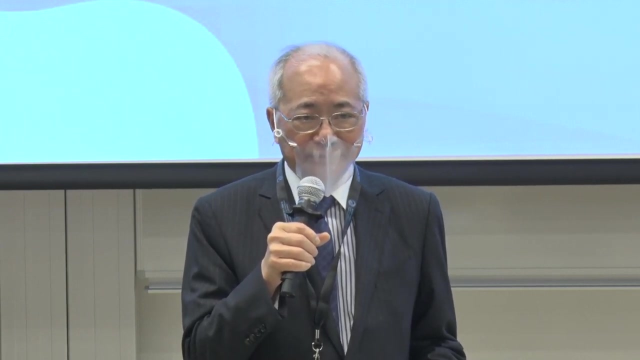 Of USD, US dollars- $230 million to begin with, I understand Japan follows by $17 million. Another message we need to remember: we are not just talking about what's happening in the ocean. We are talking about the interaction between men and the nature. 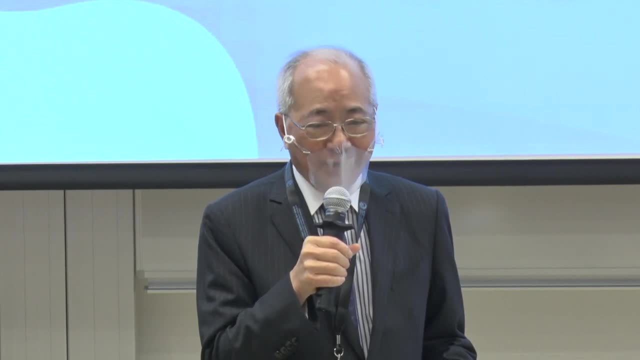 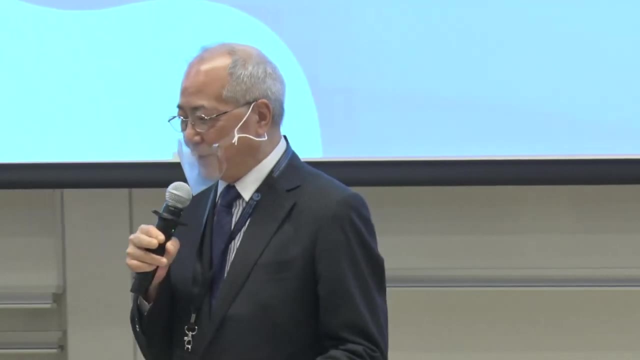 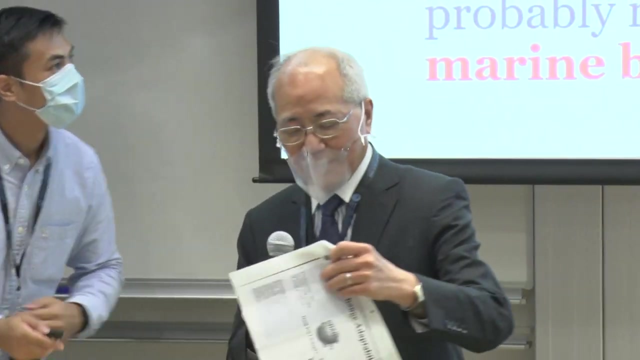 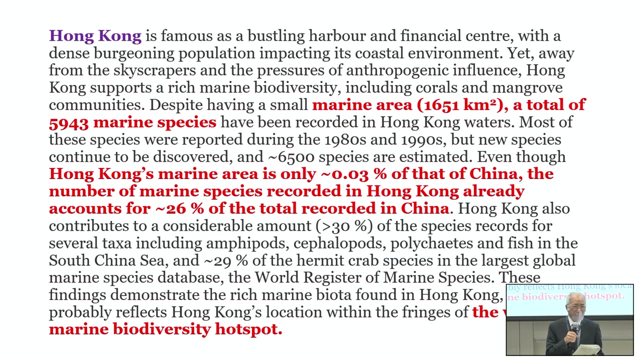 or women and the nature to be politically right. It is relevant to Hong Kong. It is relevant to everyone in Hong Kong. On this chart, just remember three things: Our ocean is at risk. Our ocean is at risk If you've been enjoying seafood every day, every week. 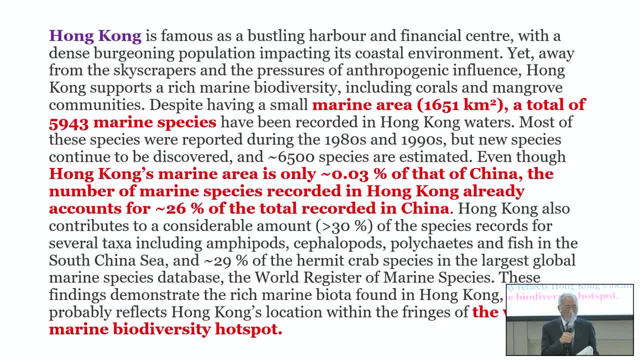 your seafood dishes are at risk. So let's put it this way to get it closer to you. And second ocean is important. It occupies 70% of our usable space on Earth. So 70% If the latest COP26, talking about everything in the air. 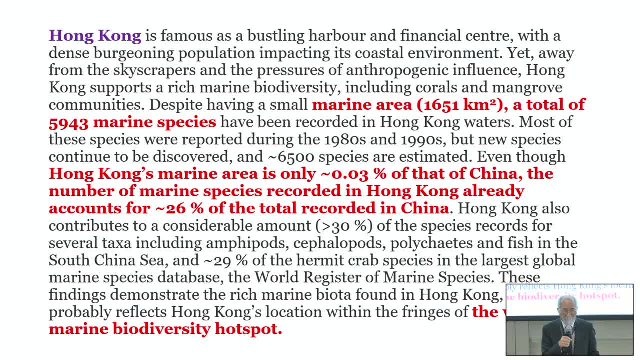 everything on Earth, on land, but not much talking about the ocean. We are ignoring the 70% areas that we are in. Another thing, equally important in threatening our seafood dishes is that 34.2% of the global fisheries are overstocked. 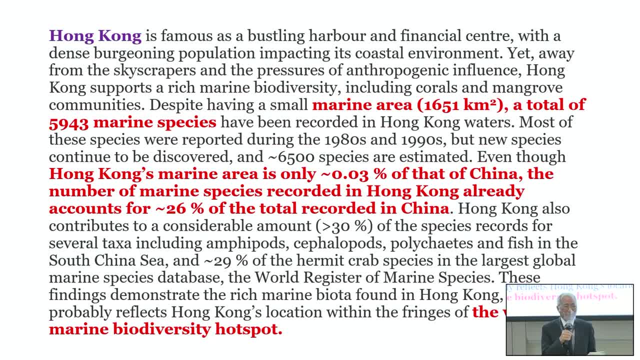 Over, over, Over, sort of stock-taking Meaning. it is overfishing, overconsuming. So if you translate that 34% for one year, how many years you consume the 100% wastage? That easily counts In the case of Hong Kong. 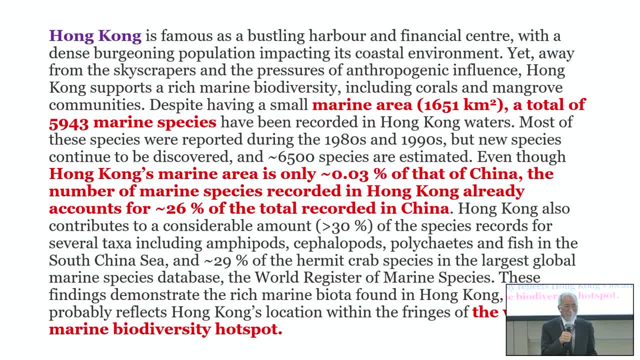 we have very, very interesting gifted land in front of us. We set a lot of people to fill land available. More importantly, actually, we have a lot of space, but not sort of on solid soil, but together with the ocean We have a very long and spacious marine area. 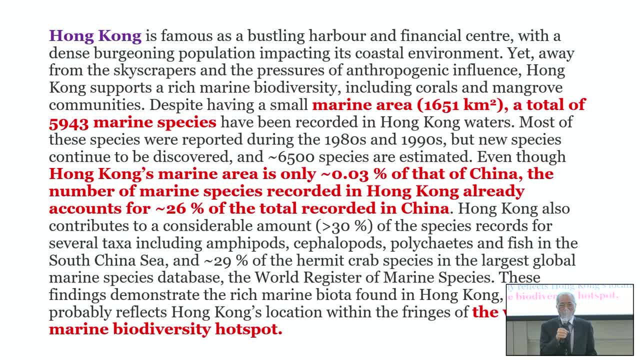 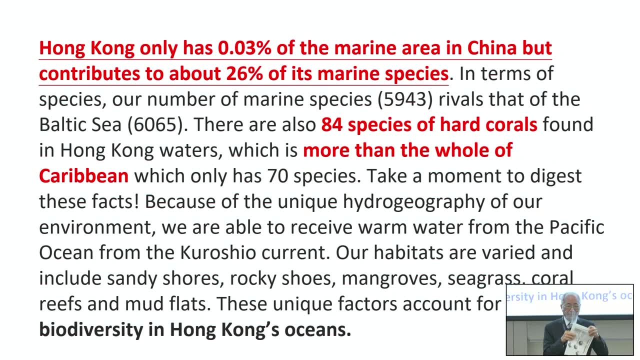 While it is only 0.03% of our mainland's total area in terms of the species. actually, we occupy over 26% of them. Now, this is a very, very interesting mix. That means what? Actually? we are quite important. 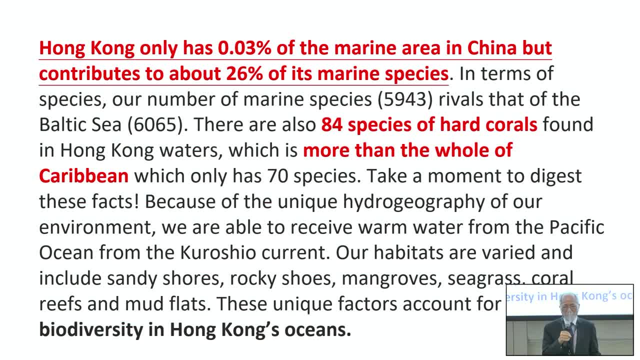 but how important do we know? Actually, we don't know much about it, We just live on what we have been able to touch. As Professor Chin mentioned, we actually have 90% of them. we have no idea at all. Not knowing it is not good. 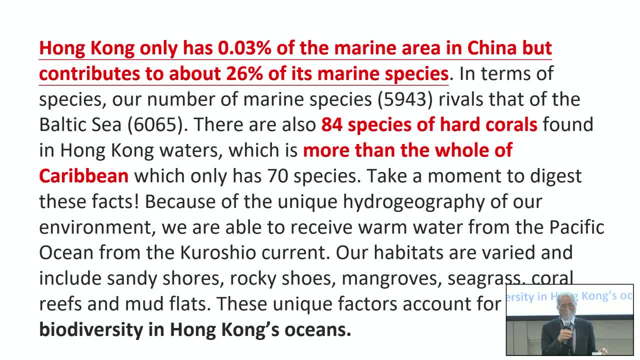 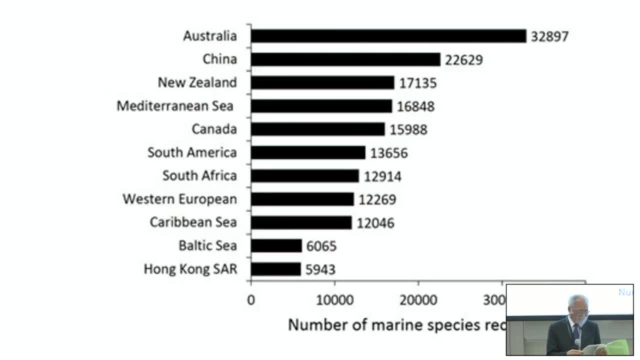 but not knowing it and trying to avoid it is guilty. If I may look at the issue in front of us, two layman points. we need to understand The marine populations, meaning the species and so on, actually not just disappearing but indeed it is a total decline in abundance. 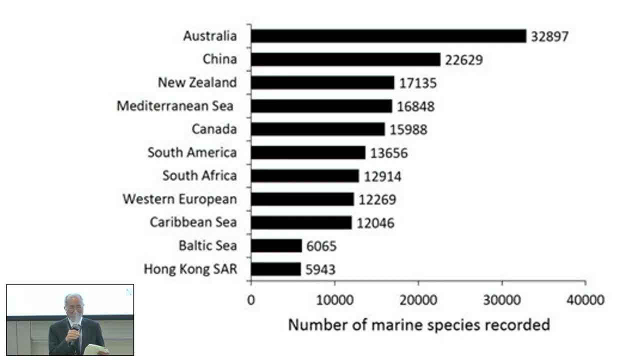 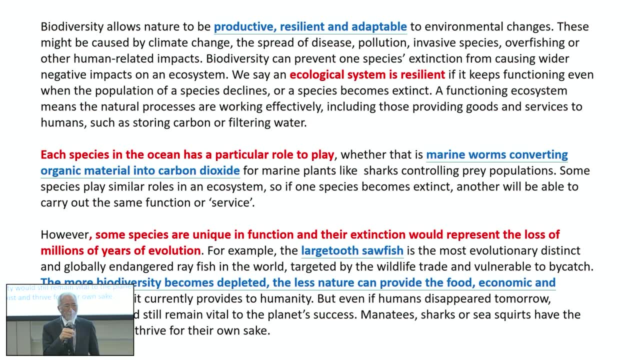 Total decline in abundance, Disappear, Extinct. This is what we are after. If the 10%- we know some of them- are disappearing, you have no idea what is the associated disappearance of the 90%. Therefore, Jane Goodall did say one thing which I like. 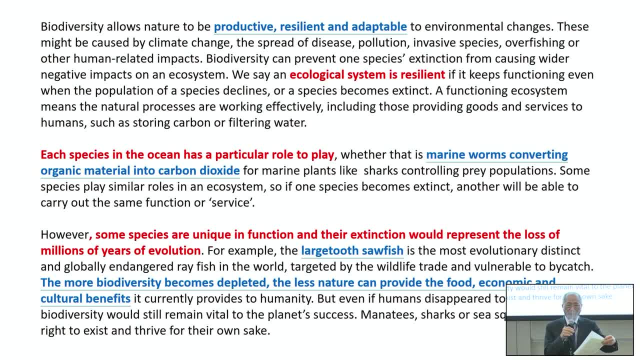 and that is only when we understand, we start knowing we can be caring. Only when we care we will be able to offer the help And only when we really take action to help we may be able to save ourselves. I read a book. 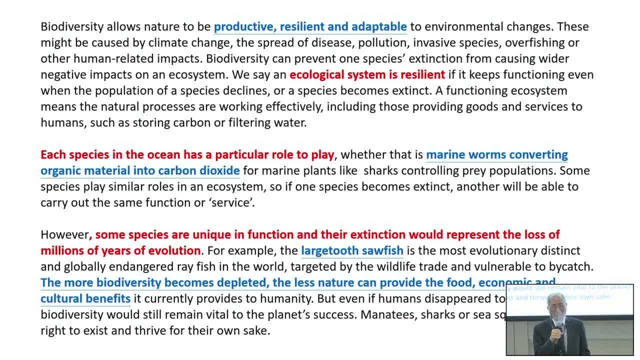 several years back, but that is one of the best practice books, particularly for the business world. that is the Knowing-Doing Gap. This is a very good book. When I was with Motorola and AT&T, this is a must-read book for all the managers. 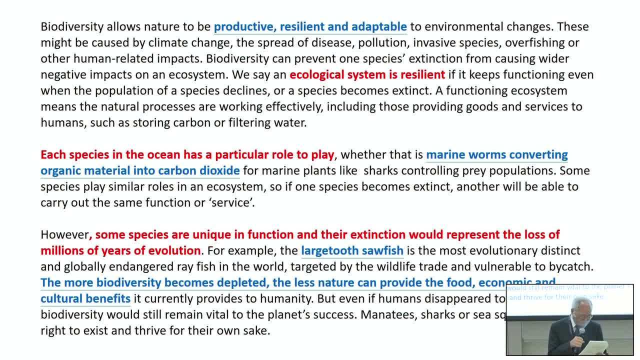 If you haven't read this book, try not to be promoted. First of all, do I know? Everybody heard about it every day on TV news: COP26.. What is it? You know it? Do you understand it? So the author arguing: 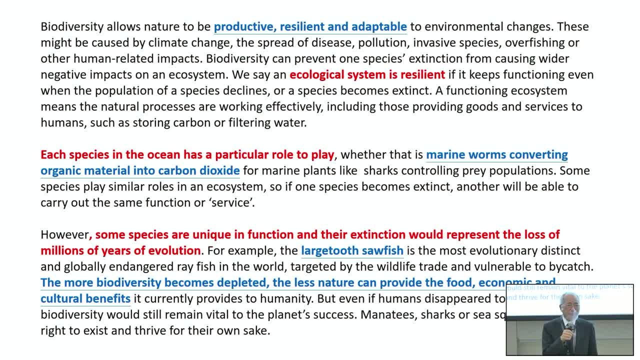 try to understand it. Marine, I know Bio, I know Diversity, I know. When you put the three together, do you understand? This is what that means. If I know it and I understand it, do I know how to address it? 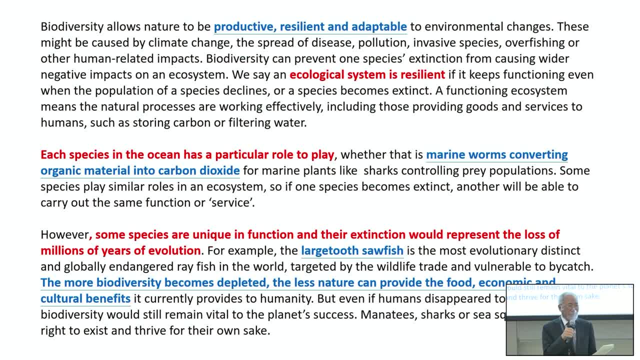 by acting on it. Do I know how to do it? I would say I know it, I have a bit better understanding. I have no idea how to do it, So picking up how in order to act on it. So if you don't know the how, 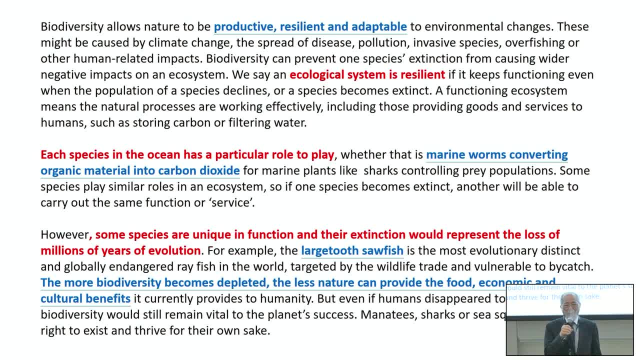 know how, you will never be able to address it, Even though you know how to do it, are you going to do it And everybody will be saying: well, the government should do this, the professors should do this, the world should do this. 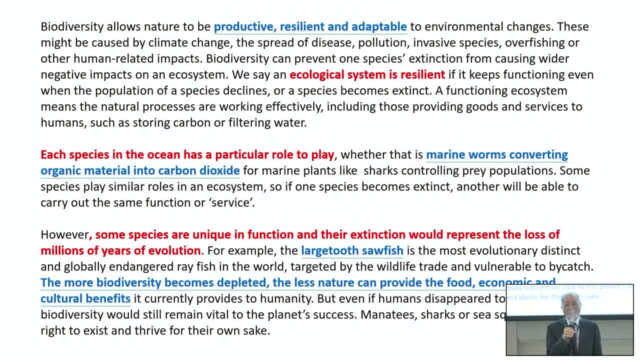 but how about yourself? I believe in more about ourselves. I start doing it. When I start doing it, then I expect I will have the right to ask other people to do it. If I haven't even done it, then I keep on asking other people doing it. 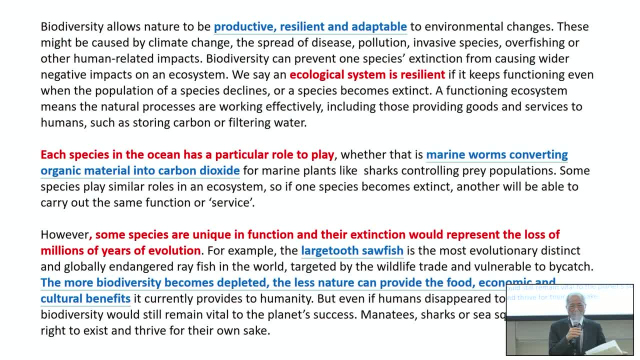 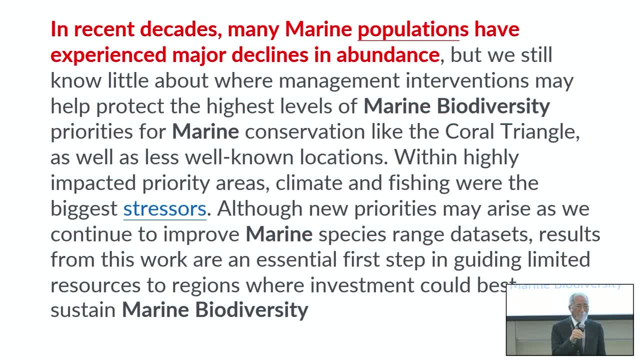 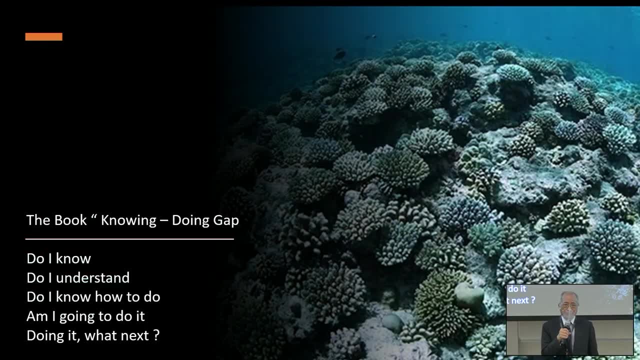 And doing it, practising it right now. then the next question is: what next? This is the best book I ever had All my 35 corporate experience. I rely a lot on this, This particular book: How to make sure our people. 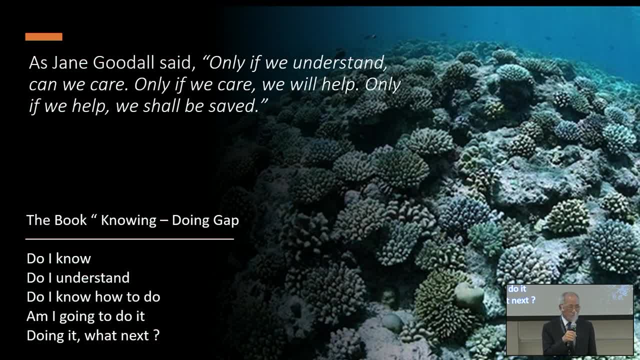 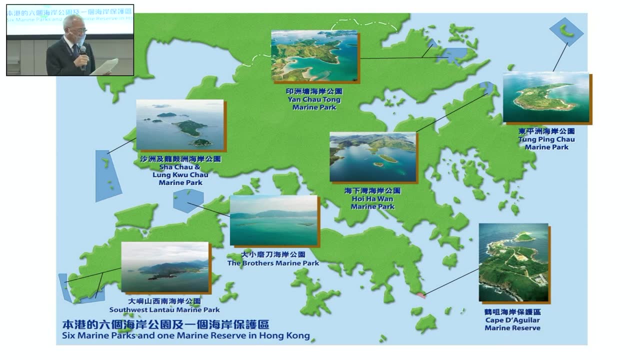 particularly young people, to know this issue. Actually, Hong Kong is not short of action on this one. For example, we do have six marine parks and a marine reserve, and these are functioning every day and fully booked and occupied, But that's not enough. 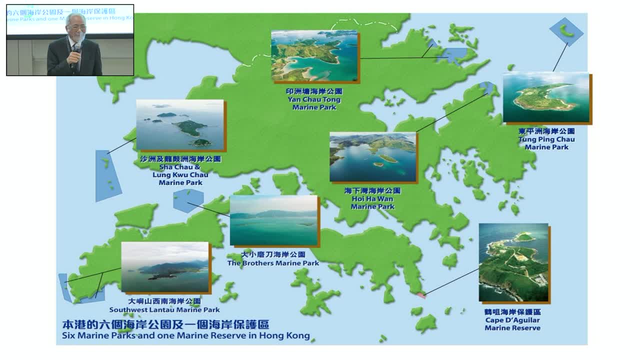 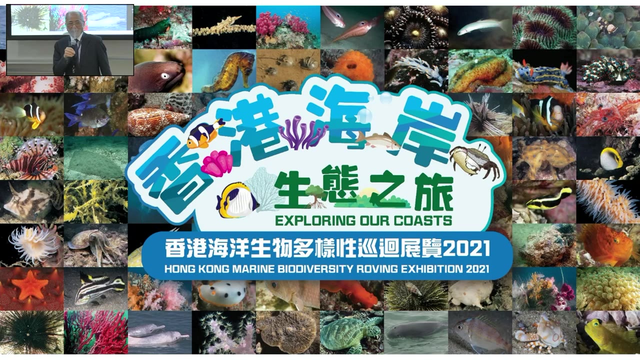 This would help. do I know it? Do I understand it, But I'm not getting into the how to do it. I know it, but I didn't practise it. Is it better I'm back? This is a very interesting programme. 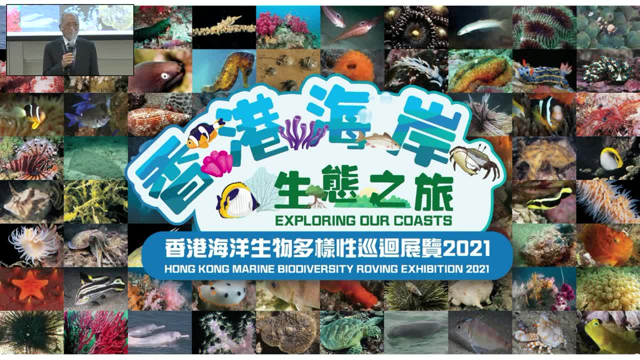 the sea front. There are a lot of programmes taking place. I personally engage in around three of them and I physically went to Pak Lai, Pak Lai village And I noticed that two things impressed me upon. There are quite a lot of the. 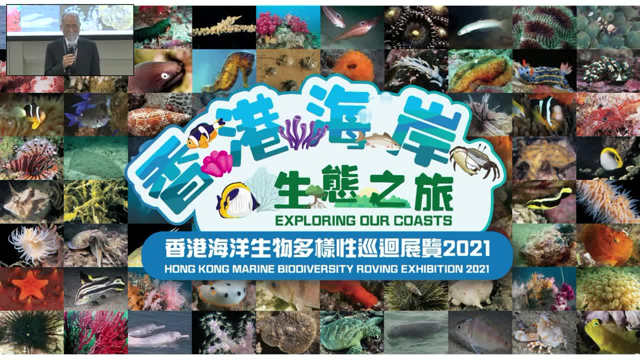 sea food targets I have been able to touch physically. The other one is I found out there were some of the aged historic stones, like the stone age type of the tools, actually over 10,000 years. One actually is 50,000 years. 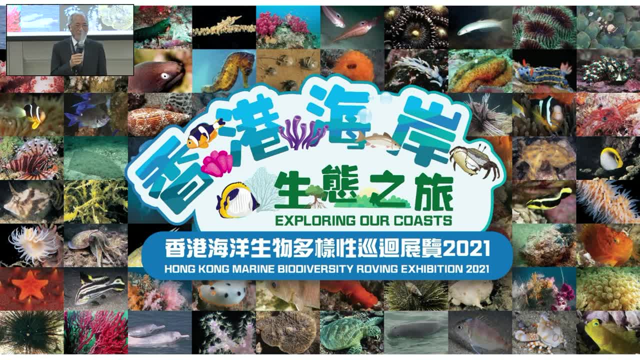 I physically touch it, Then I have a different sense when I look at it again in terms of sentiment. So government is never, never coming late, even though it's a little bit late If you look at the Hong Kong Climate Action Plan 2050,. 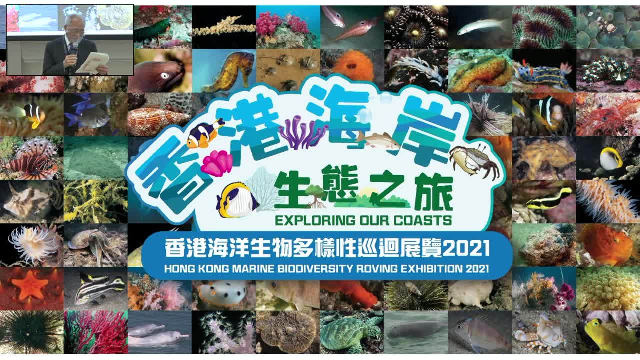 you'll be able to see that a lot of things coming And carbon neutrality hopefully on in or before 2050.. That's what it said. It embraced a lot of actions, including net zero electricity generation, energy saving and green building. 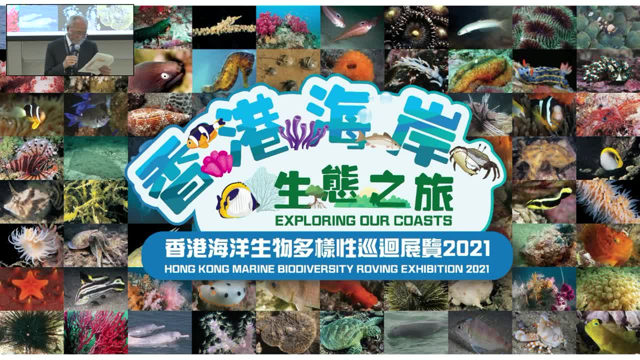 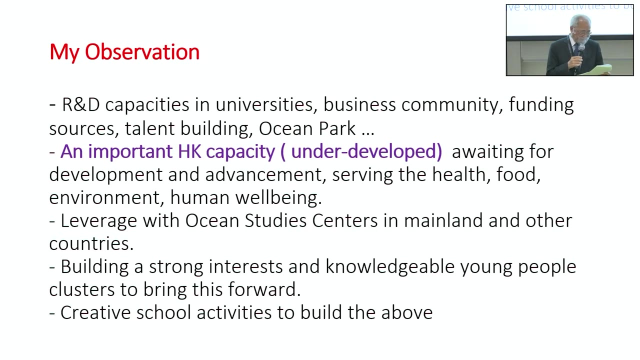 green transport waste reduction. There's a Council of Sustainable Development overseeing that. Where's the 70% ocean area that we are in? What's happening to my future supply of sea food chain or the? Therefore, I do want to share. 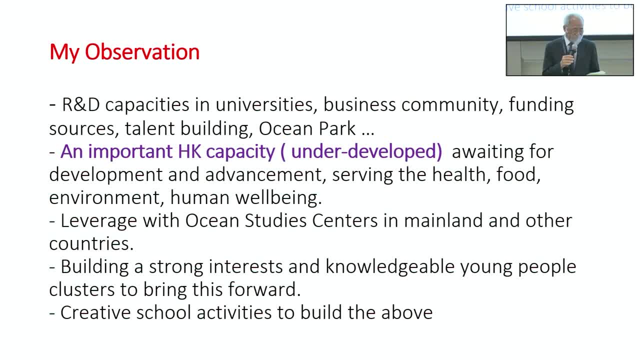 as the last two, second page, my observations. There's a reason for me being here. I would like to see the research and development capacities existing in universities. this is particularly UST. I realise it today, the real, the only programme so far. 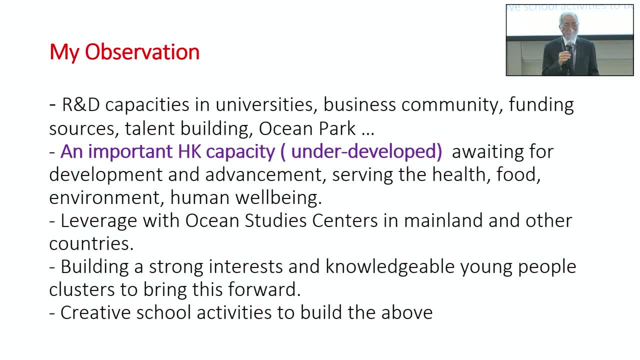 for the undergrad. It's actually only a few years back. The first cohort has been in place and they are starting it Right on time, right after the COP26.. The business community: we do have a representative in the Legislative Council on Fishery and Agriculture. 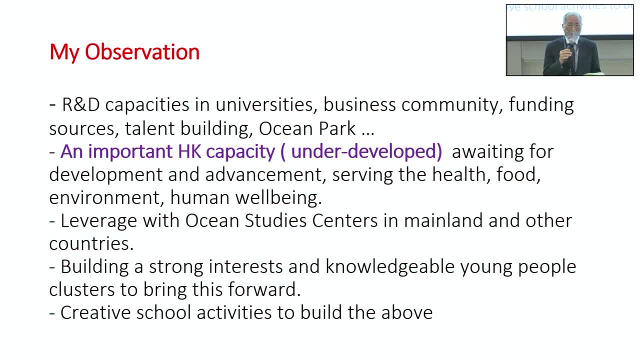 We are the funding sources other than the ROTC and then the UGC. There must be a lot of others. There are a lot of corporations actually engaging in this particular sector Have been able to align the sector with the ROTC. I would like to say that 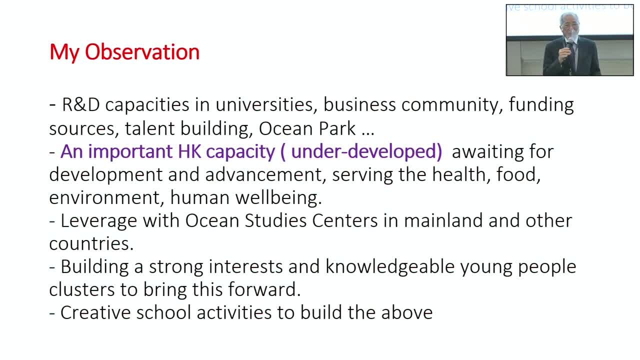 I think the sector, those who are aligned with them, how many people actually are able to get engaged into that, particularly how many young people have the chance to understand and to get engaged? That is the key. How many I actually couldn't find. 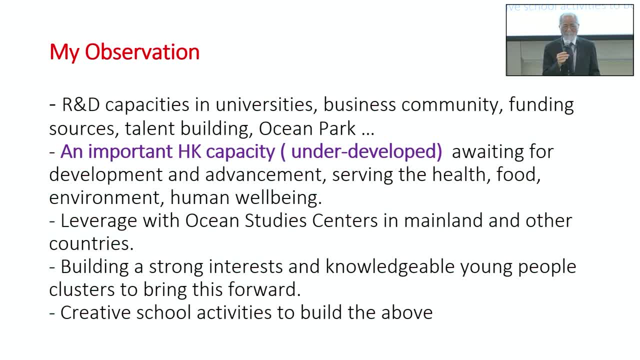 particular evidence yet other than try to understand it and know it. One area which we forgot underplay a lot, actually a lot of expertise: Ocean Park. I have seen a lot of Ocean Parks around the world doing a lot of labs. 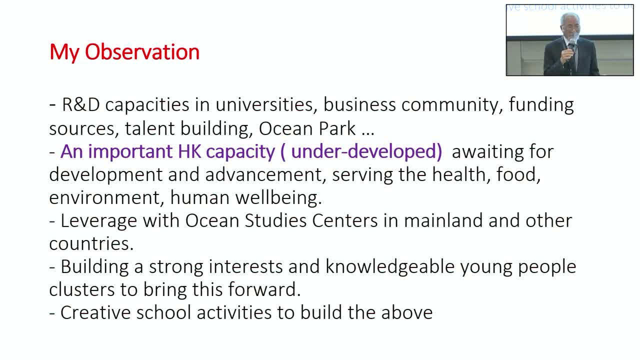 doing a lot of research work. They have the business direct link capacity to address that. The second one is: I do believe this is a very, very top strength area and strong area for Hong Kong, but so much underdeveloped Underdeveloped. 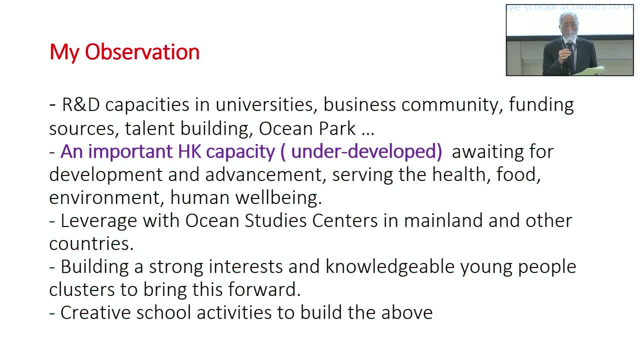 Therefore, everyone here in the room, hopefully we will be able to do something right after today. Go back and see what you can do, to do something about it, because it's going to touch our health, our food chain, our environment and our human wellbeing. 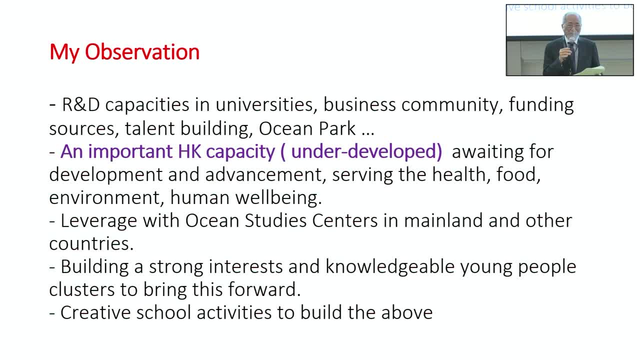 all together We need to leverage. Hong Kong is a small space, 7.5 million people, small city, but we have a lot of strength. Therefore we need to leverage with other strength together in the southern part of China, in the whole China. 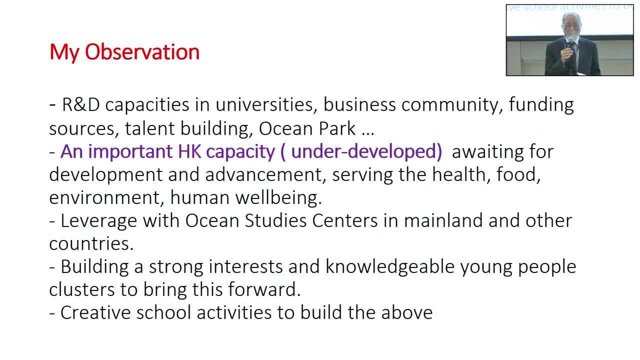 and in Hainan Island, in Qingdao, Qingdao, one of the earliest sort of a research centre, and particularly in, say, Australia. Australia is the largest species around the world and need to do a lot of the work to motivate our young people. 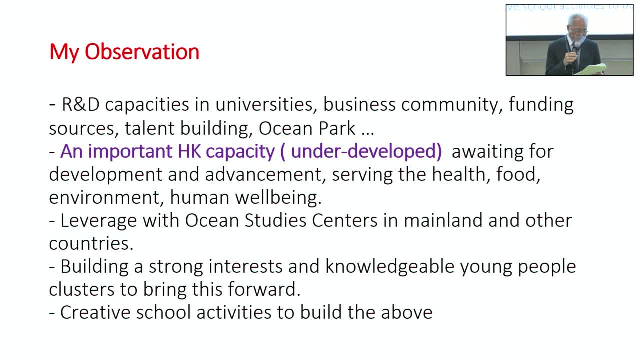 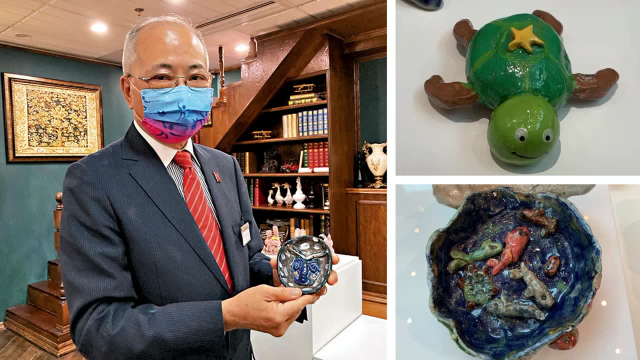 to get them interested in and be able to get their actions together, particularly create school activities to build all this. This is a very interesting picture. I just got engaged recently. This is my dream. I start with the kindergarten kids. There are about 150,000. 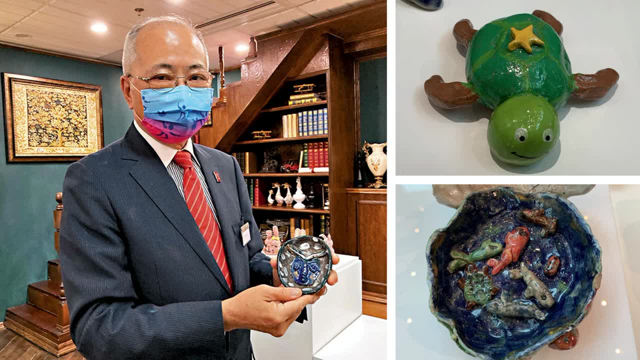 kindergarten kids in Hong Kong, We said: well, they are too young to do anything. I'm telling you this pottery arts particularly designed for the kindergartens: these turtles, these fishes were produced by them And when they produce it. 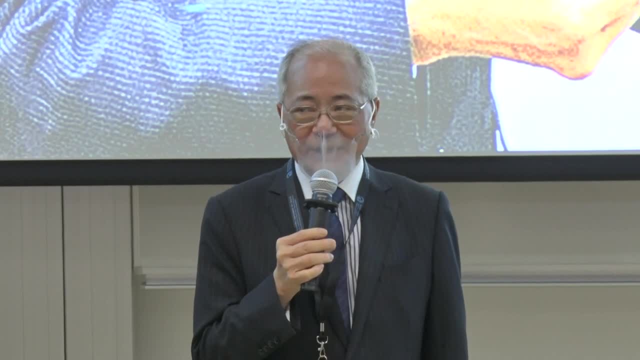 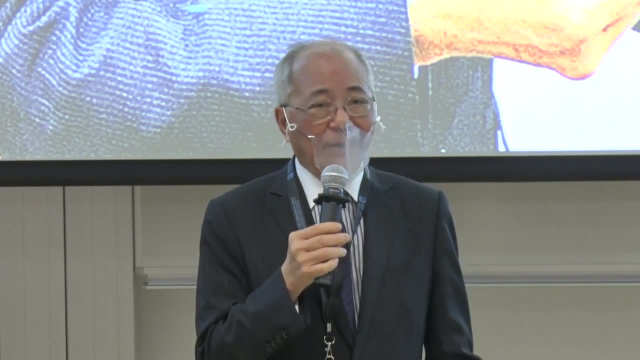 they realise it, What is it? What difficulties the turtle actually had faced with all along? The environmental, the fish nets, sort of cutting the neck, all these things. they start to realise it. And as they realise it, the plastic materials. 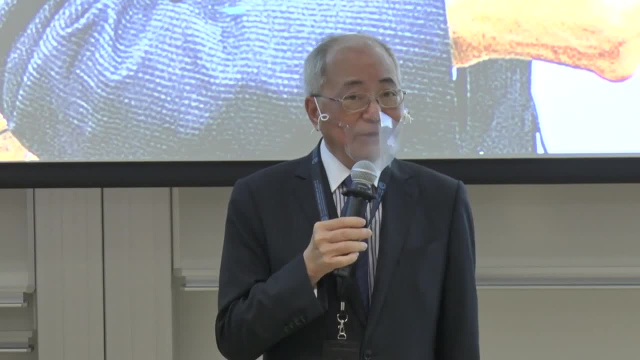 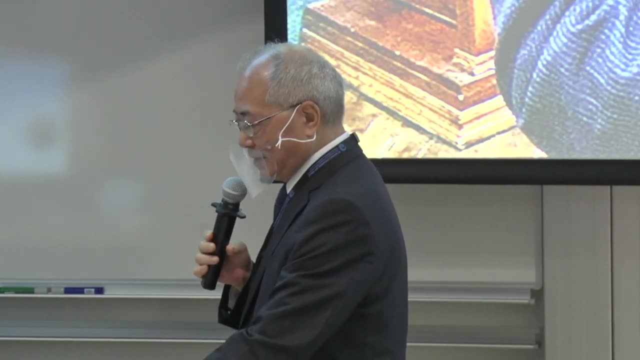 inside the deep ocean. what does that mean? Actually, they are able to teach their parents, KG students teaching the kids. So, if you look at it from that angle, this is the key. Therefore, I hope this is just a few points. 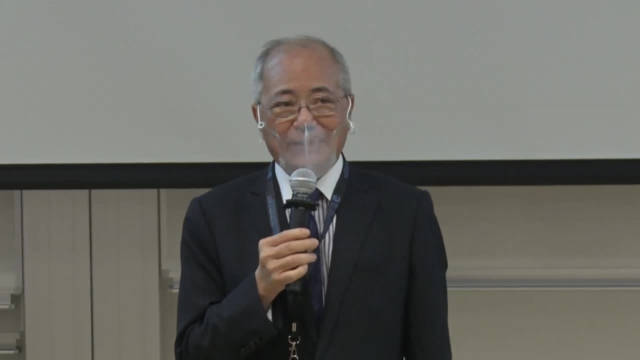 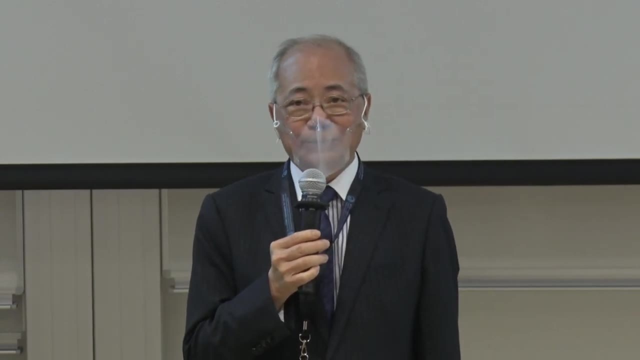 of reminder and be able to just get a bit more of your attention. The key thing is: let's start understanding more, Let's try to do something about it and we act on our own first before we ask other people to act on. Thank you so much. 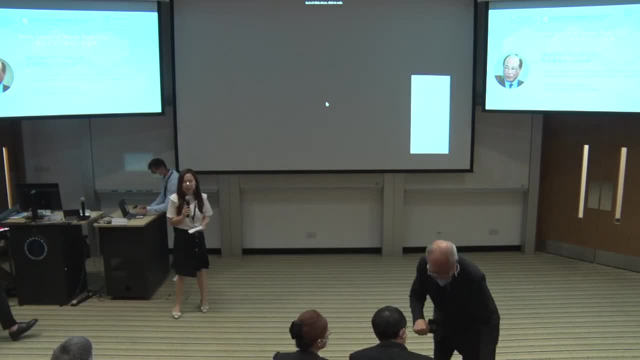 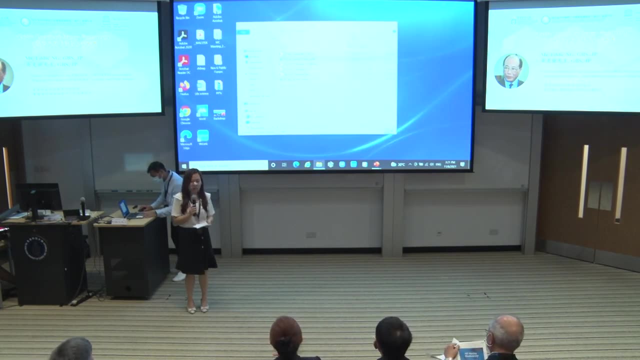 Thank you. Thank you, Mr Ng, for his remarkable presentation. Other than Mr Ng, we have also invited another keynote speaker, but he can join us in person today. He is Dr Chen Shang, who delivered a keynote speech, and he is the Vice Chair. 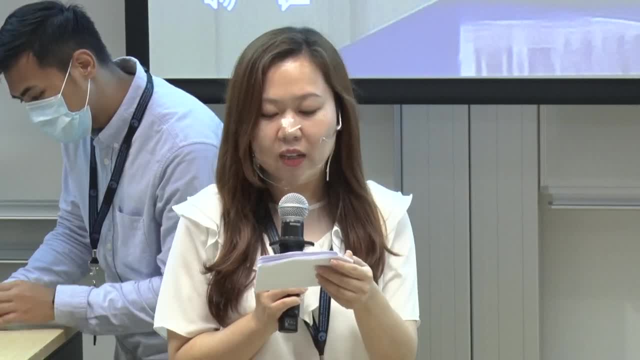 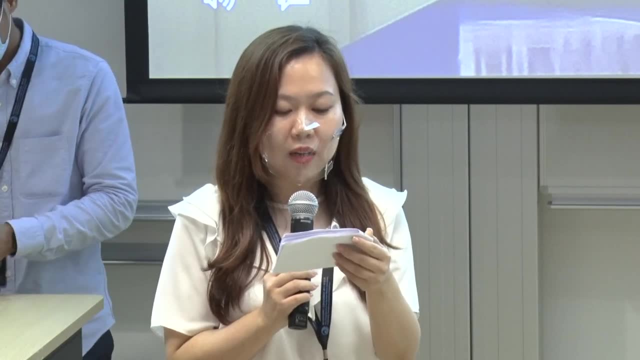 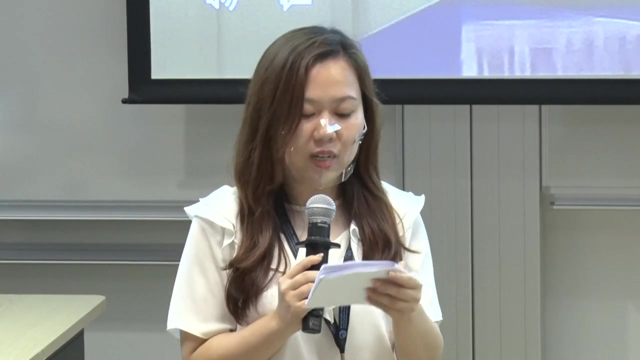 of Marine Committees Council. Member of Chinese Ecological Economies Society. Co-Chair of Working Group for Ecosystem Services. Member of Committee on Human Dimensions of Marine Systems- North Pacific Marine Science Organization. So let's watch his pre-recorded speech and presentation together. 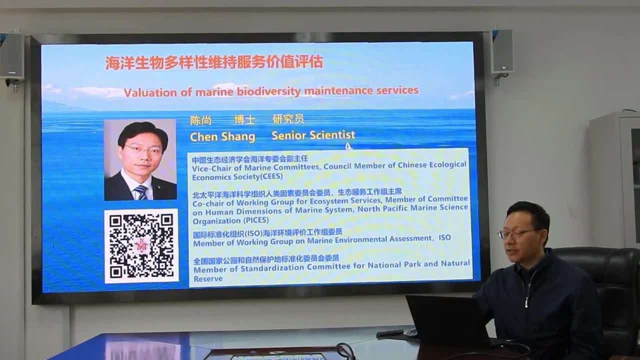 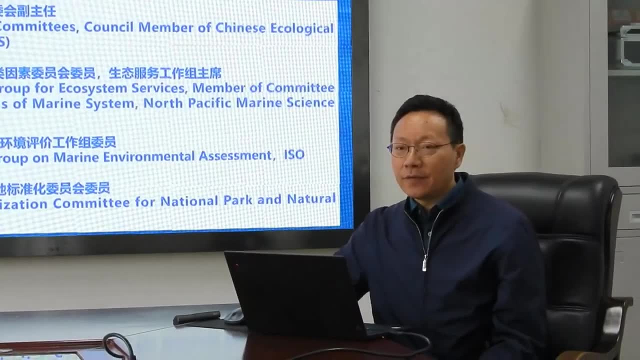 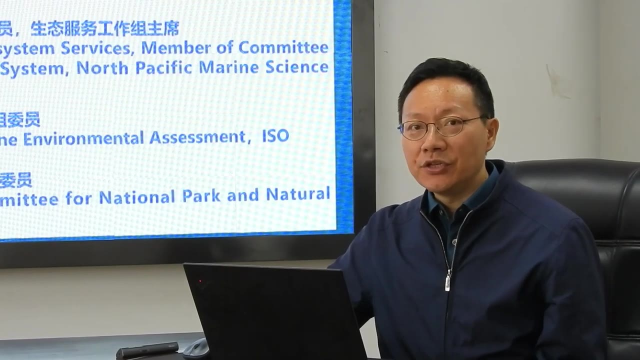 Dear Chen Li-Yen, Professor Zhang Qing, Professor Wu Kejie, Professor, ladies and gentlemen, good afternoon. Many thanks for inviting me to give a talk during the Public Forum on Marine Biodiversity and in Qingdao City, Shandong Province. 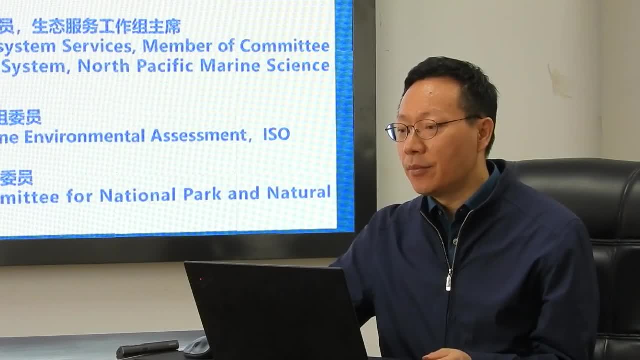 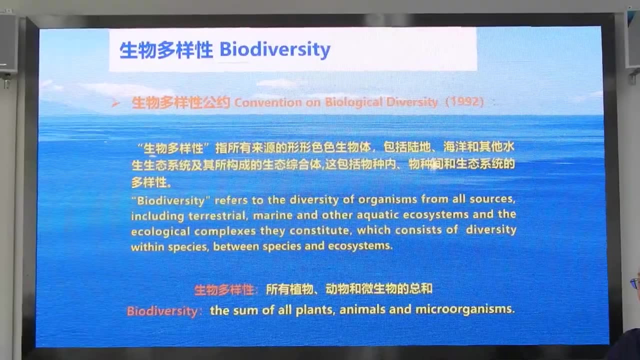 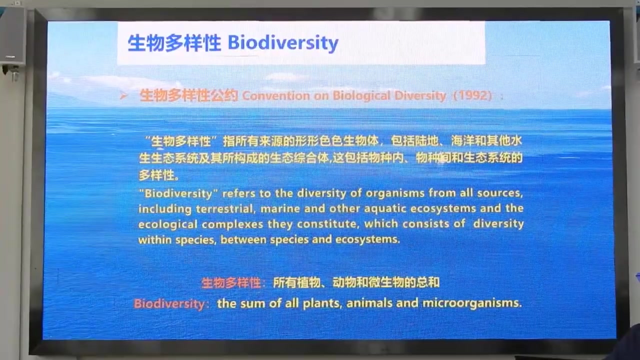 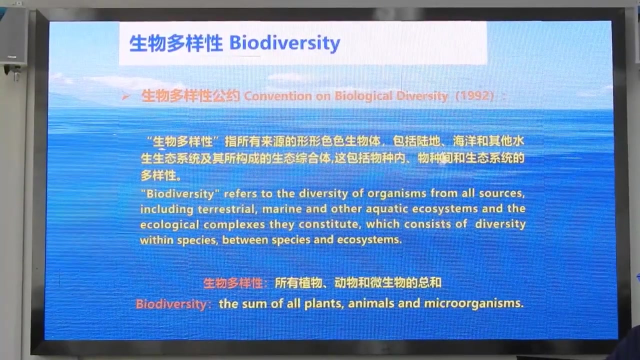 Today, my talk is on how to assess the monetary value of marine biodiversity maintenance services Under the United Nations System. the Convention on Biological Diversity defines the biodiversity as the diversity of organisms from all sorts of sources, including terrestrial, marine and other aquatic ecosystems. 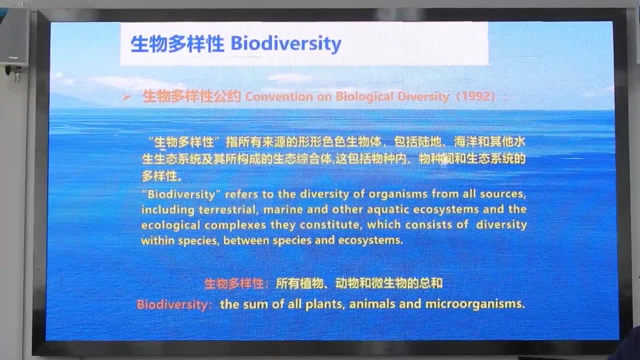 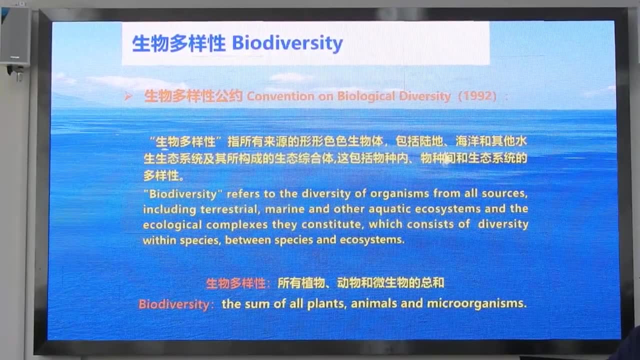 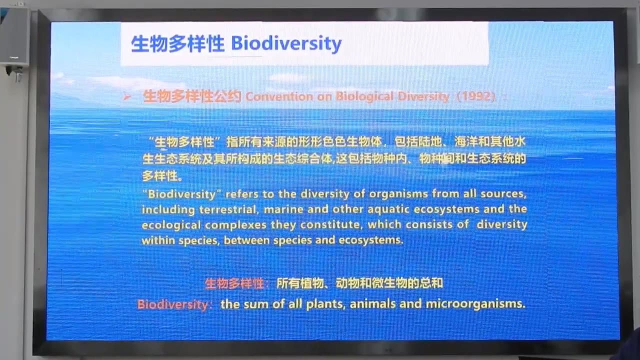 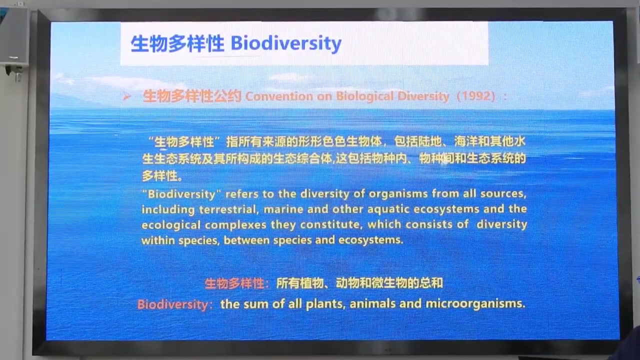 and the ecological complexes they constitute, which consists of diversity-based species, between species and between ecosystems. In short, biodiversity is the sum of all plants, animals and microorganisms. This concept is accepted by most of the people. Biodiversity has three levels. 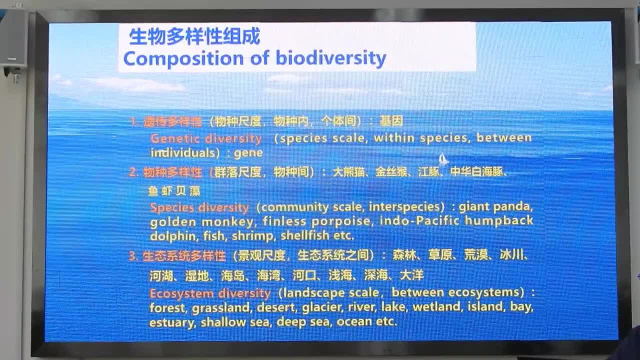 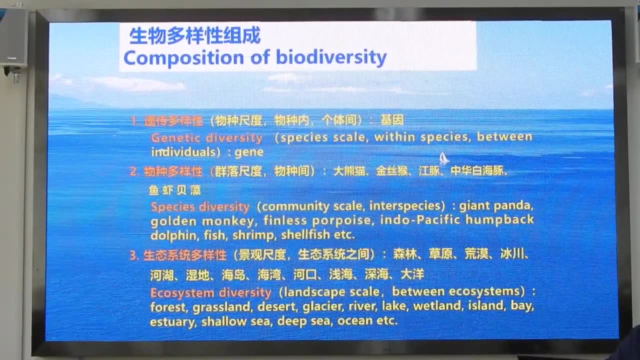 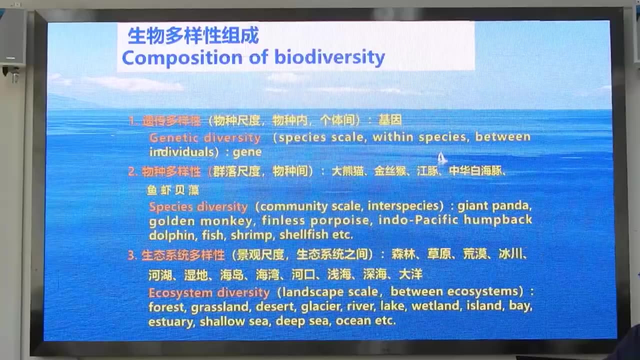 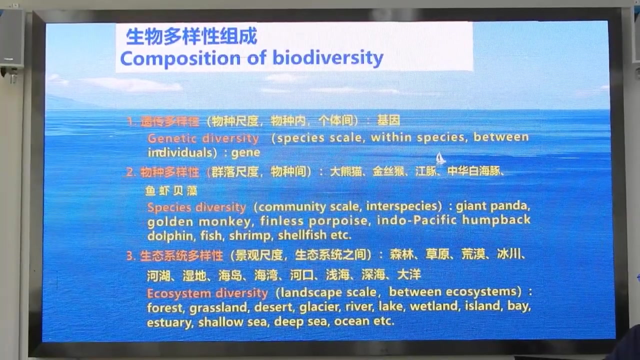 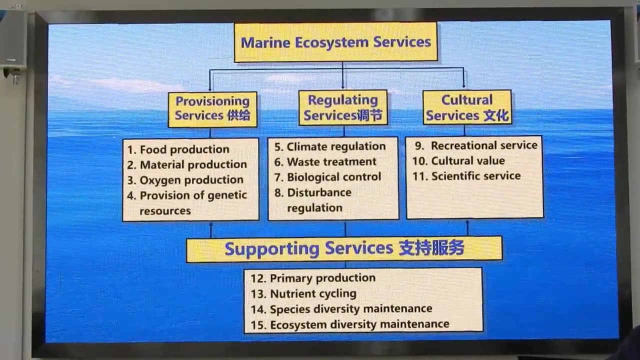 The first level is the genetic diversity among different individuals within one species. The second level is the species diversity among different species and biological community level. The third level is the ecosystem diversity among different ecosystem at landscape level, Marine biological community plus their habitat, sea water. 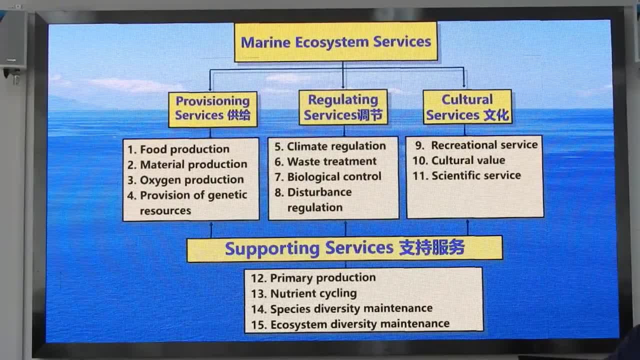 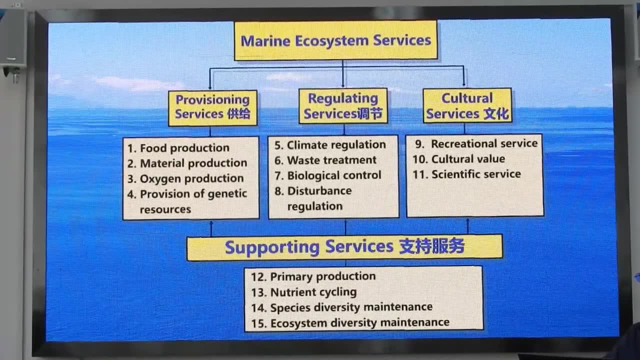 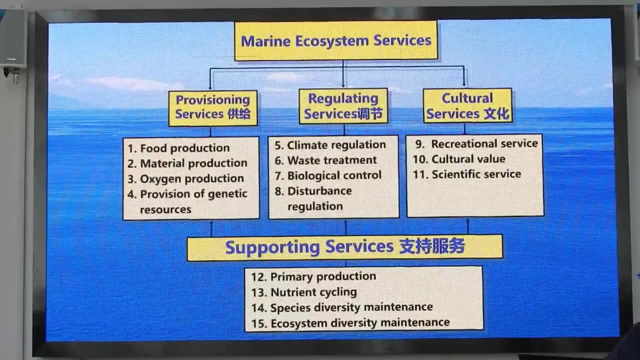 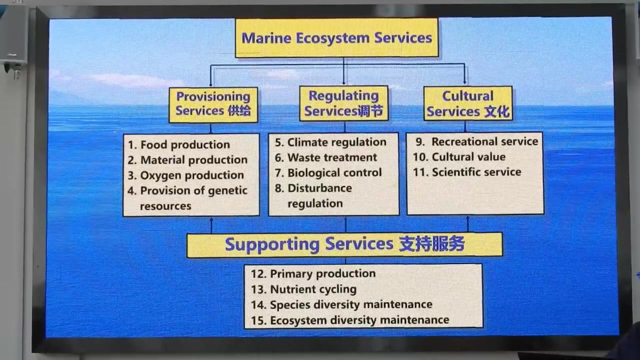 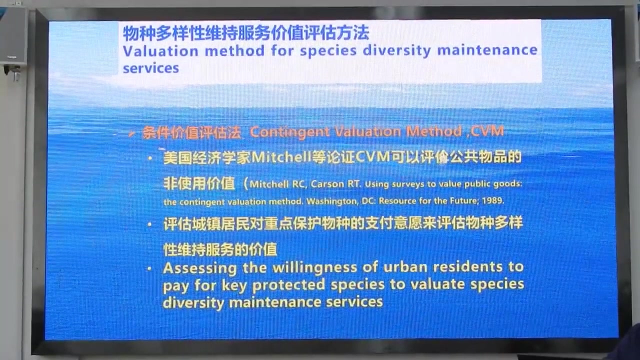 and surface sacred form into one ecosystem. Marine ecosystem provides us four groups of services and 13 kinds of services. for example, record seafood production, climate regulation, nature and recreation, species diversity maintenance from the sea, Two species- biodiversity maintenance services are mainly contributed. 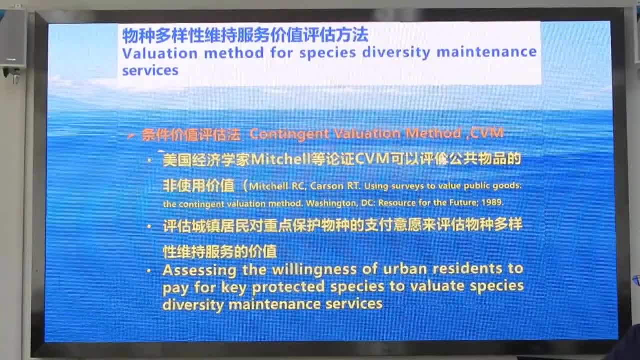 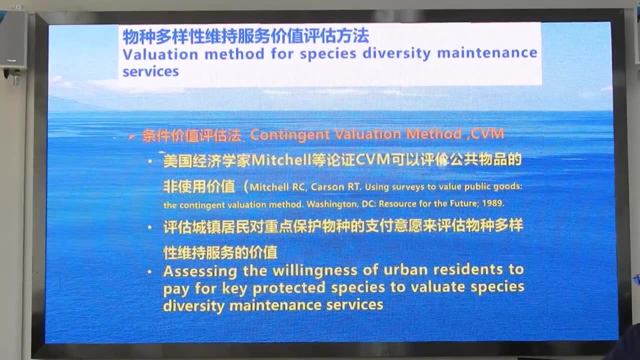 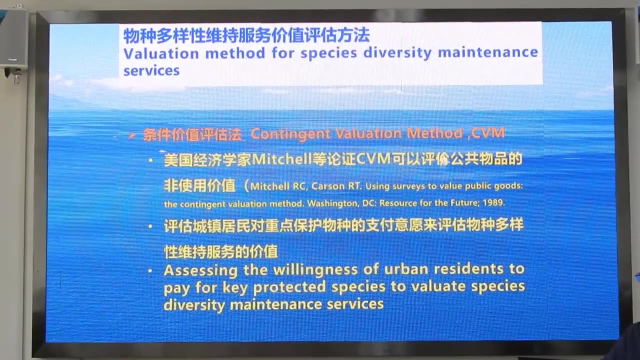 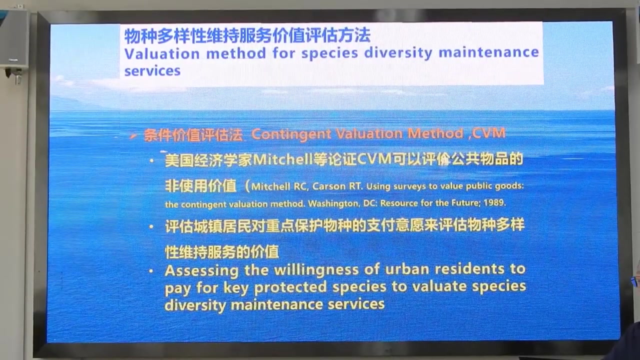 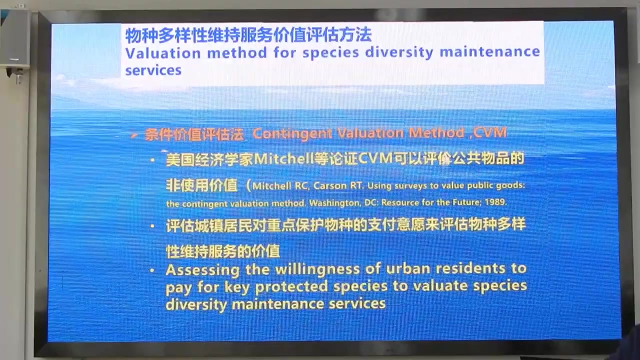 by the rare and endangered species, especially contributed by the register species in the National Key Protection Land List And its value attribute belong to the non-use value or existence value, intrinsic value. They are not market price for this species. The US economists 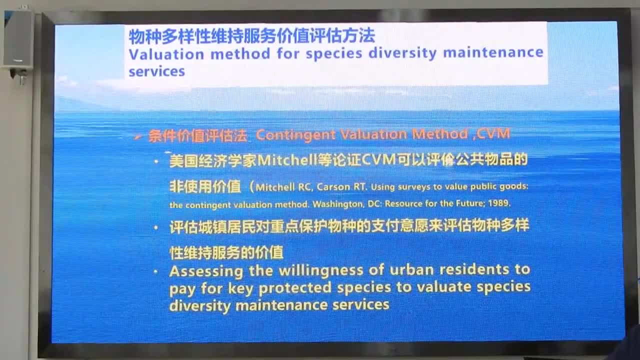 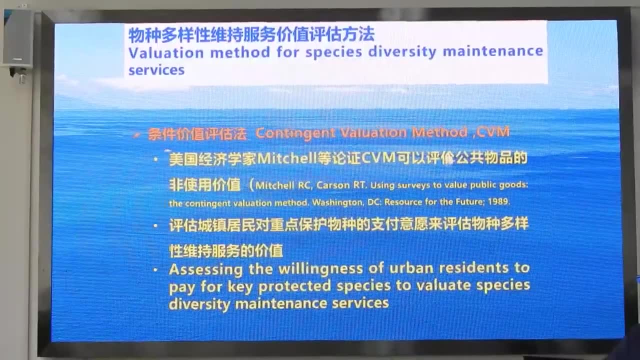 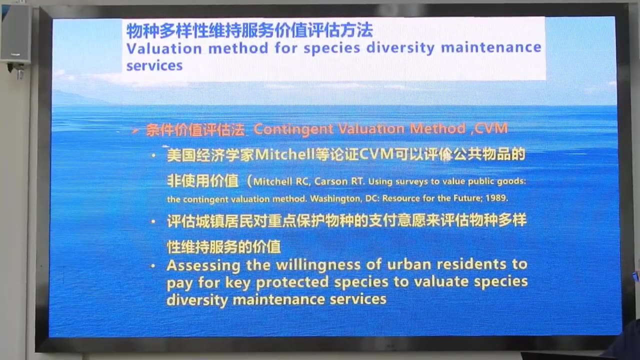 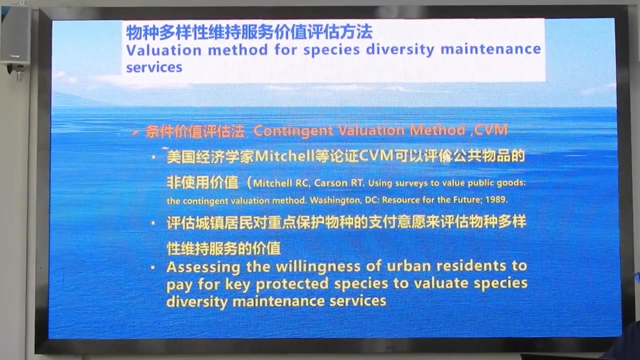 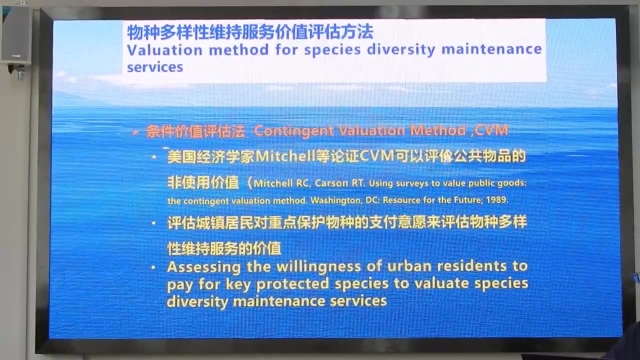 The US economists have developed one method to assess the value of public goods without market price, That is, continuing the valuation measure. This survey has been widely accepted. Here we use the NASA survey arm to assess the willingness of urban residents to pay. 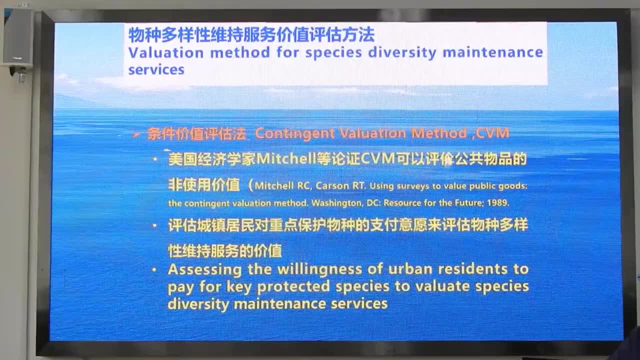 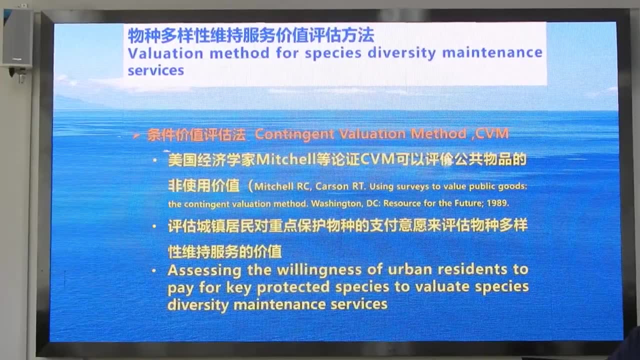 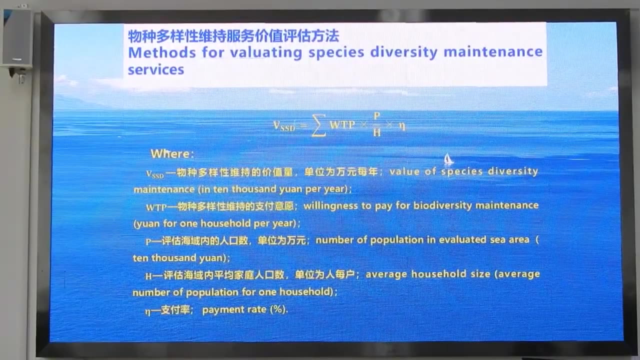 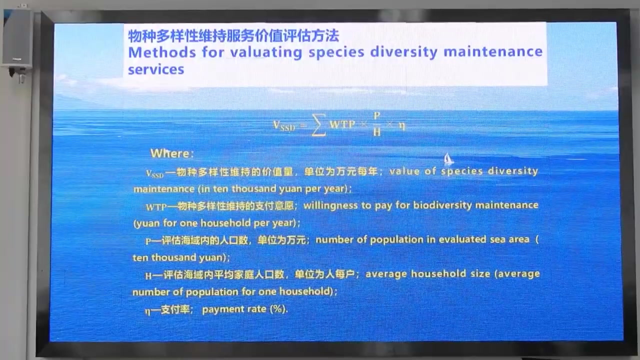 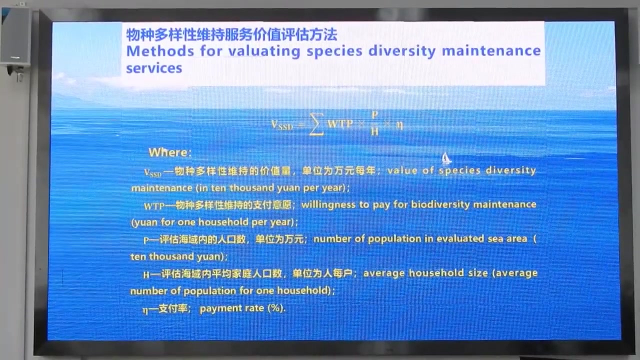 for national key protected species, then calculate the monetary value of the species' diversity maintenance services. This formula is to calculate the monetary value of the species' diversity maintenance. This is the monetary value of species' diversity maintenance. This WTP is the willing to pay. 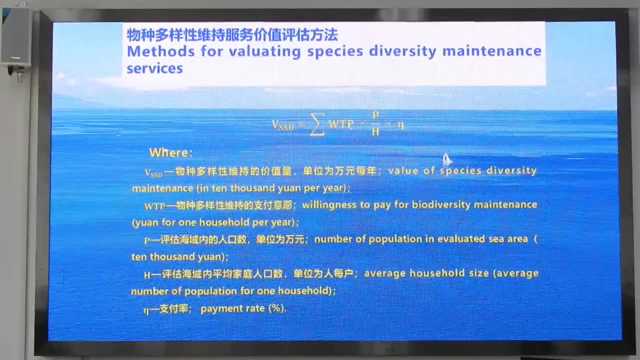 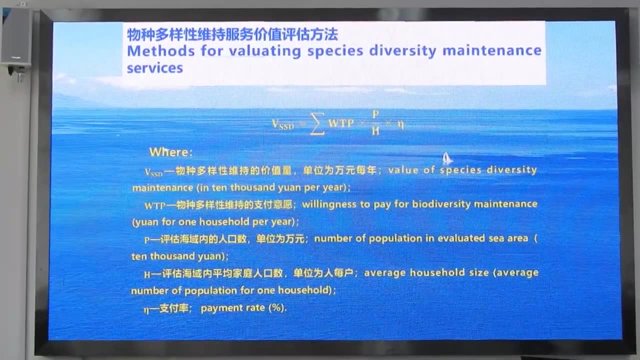 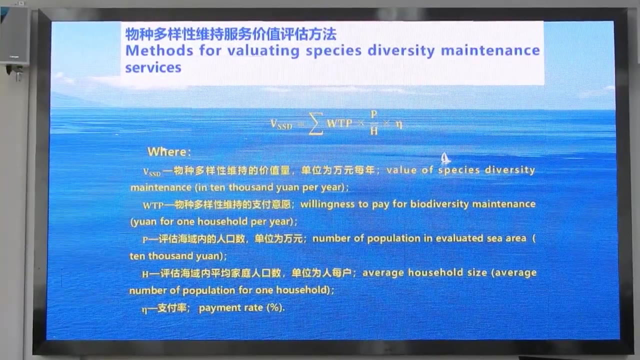 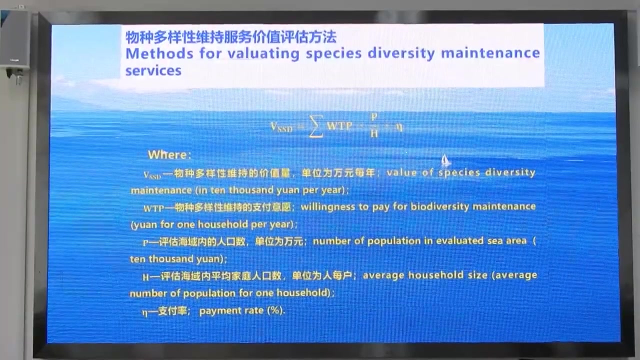 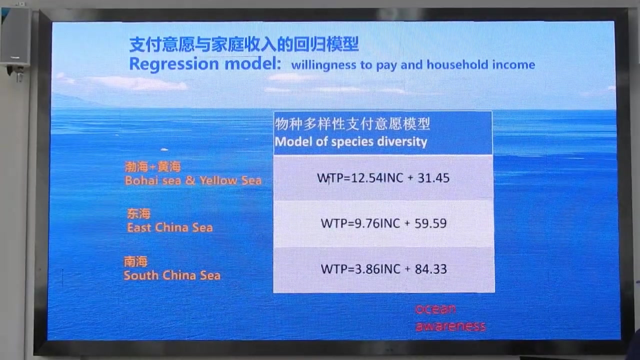 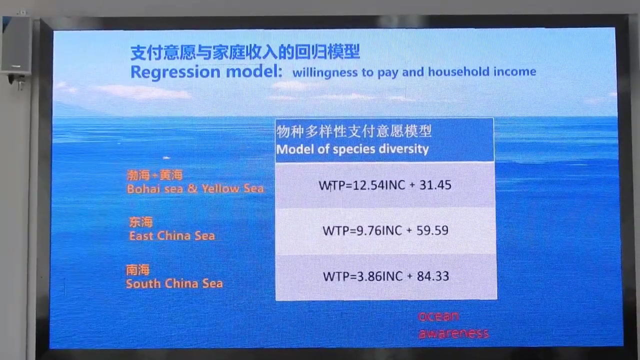 for biodiversity maintenance services. The P means the total number of population, H is the average household size. That means the number of population for one household. Eta is the payment rate of several populations. We got the WTP regulation model, This form. 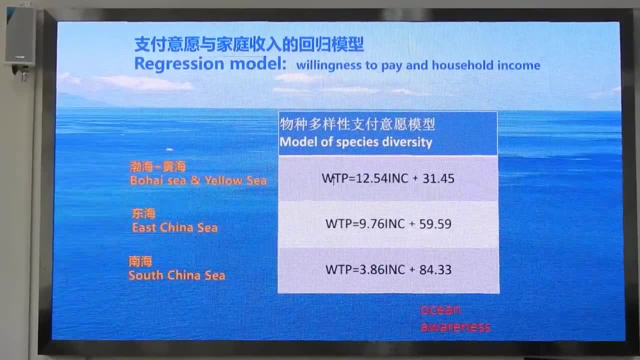 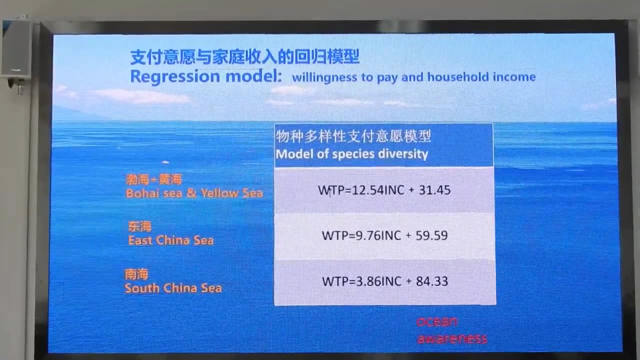 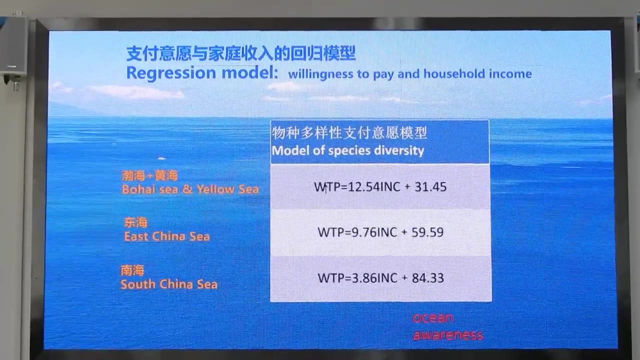 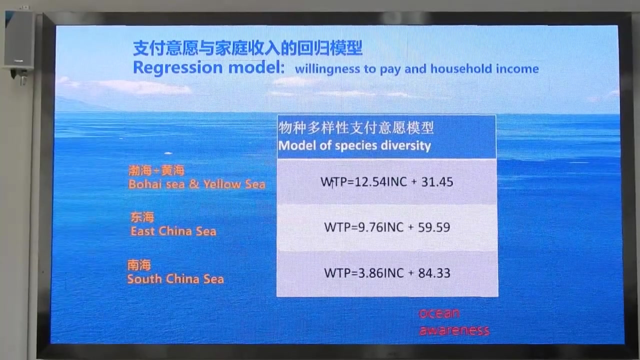 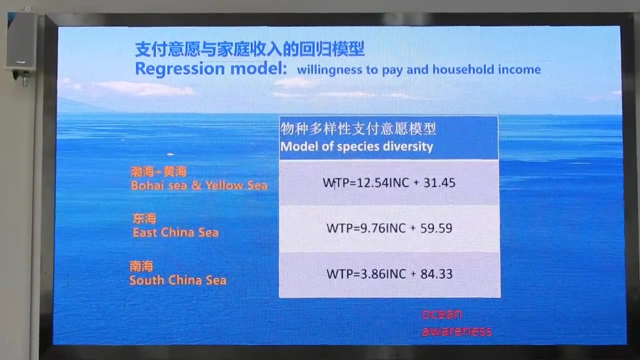 is for the safety of the coastal residents around the West Sea and the Yellow Sea. The WTP is held in the WTP that highly depends on the household income level. This value is reflected on the portion of the residents. This is for East China Sea. 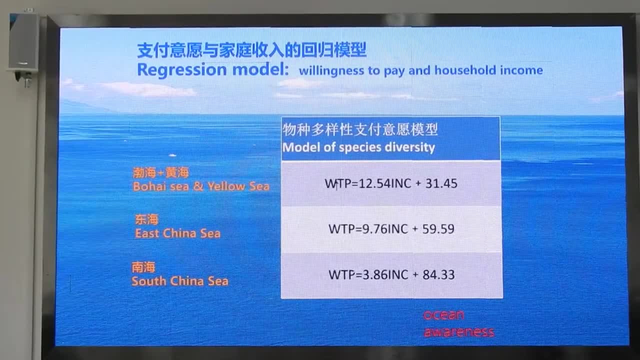 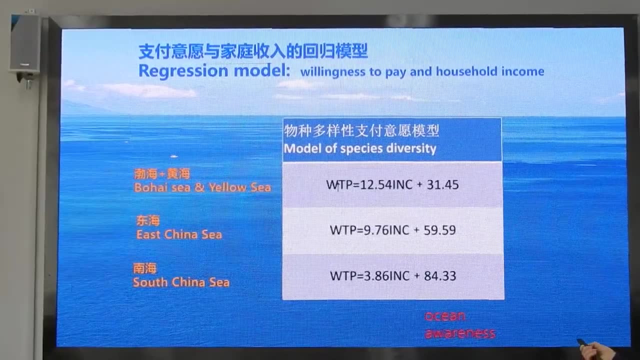 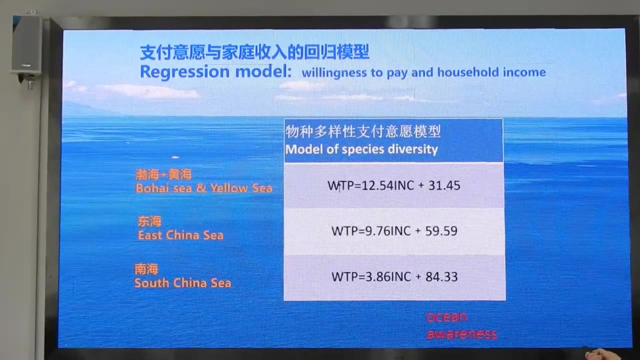 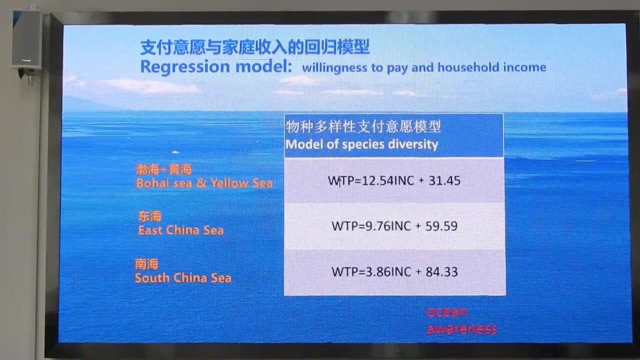 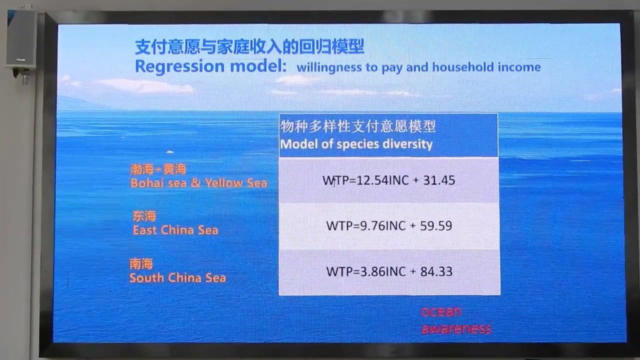 This one is for the South China Sea residents. From the Bo Hai Sea and Huang Hai Sea to East China Sea and South China Sea, the values decrease. This number reflects the portion of values in the South China Sea Around the South China Sea. 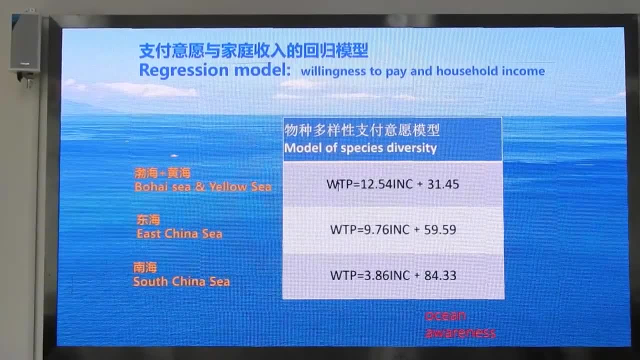 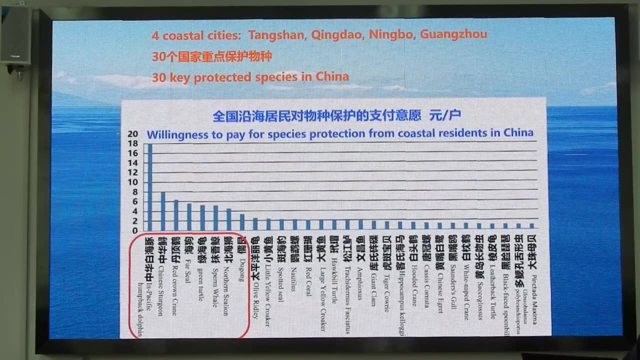 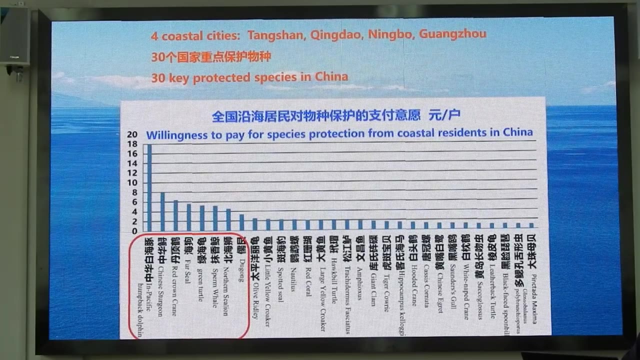 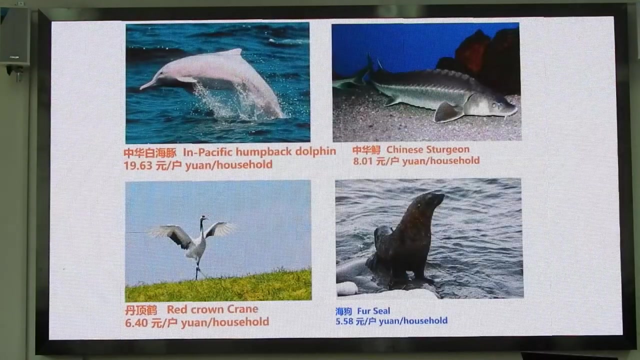 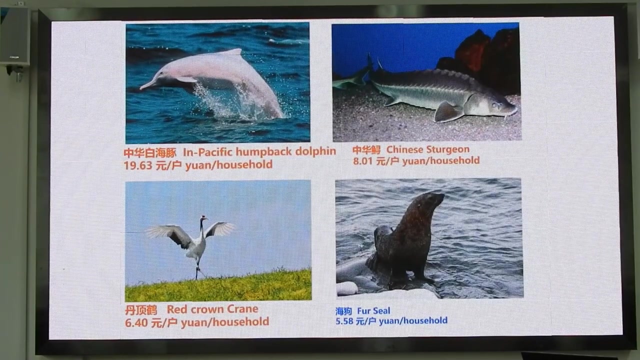 the range of the ocean values is higher than East China Sea, Yellow Sea, East China Sea and South China Sea. The four services are conducted face-to-face to get the valuable pay of urban residents. for certain national practical species, This is a species Chinese. 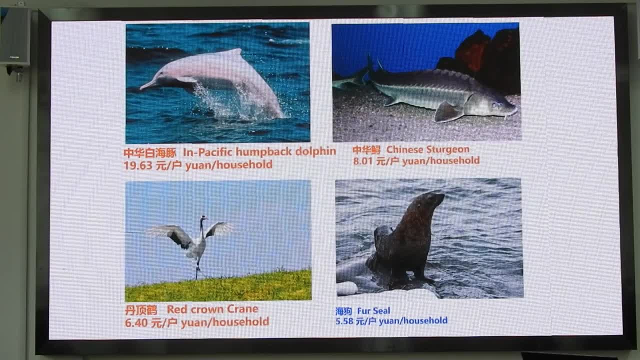 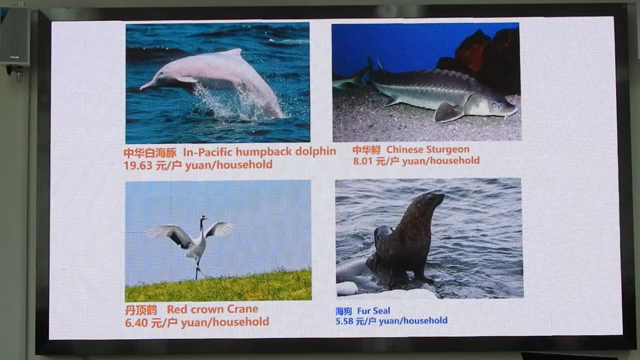 dolphin. This species is distributed in Hong Kong waters. The valuable pay is the highest, about 20 per household per year. The second is the Chinese statue: 8 Chinese per household per year. The third is the red coral crane: 6.4. 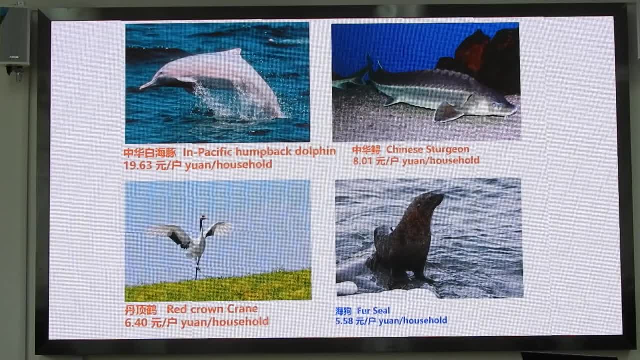 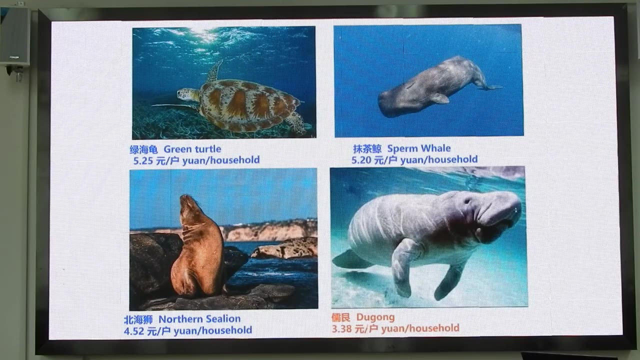 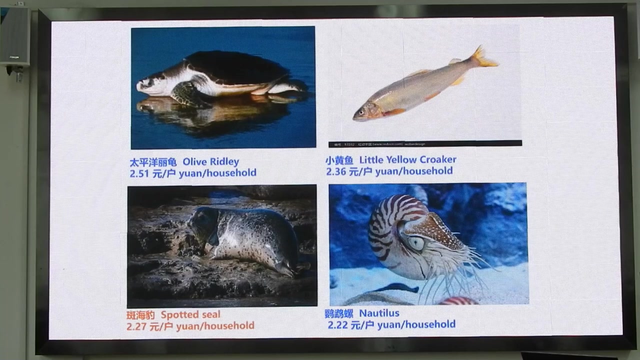 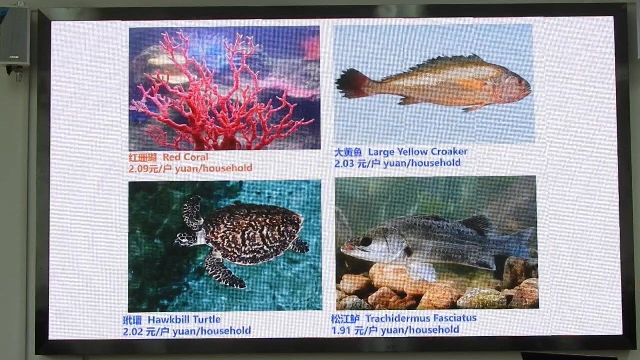 Chinese Yen. The fourth one is the first sale: 5.6 Chinese Yen. The token is 3.4 Chinese Yen. The fourth is the second sale: 2.3 Chinese Yen For red coral: 2. 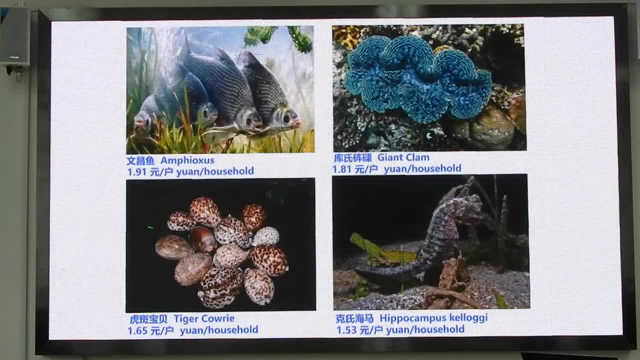 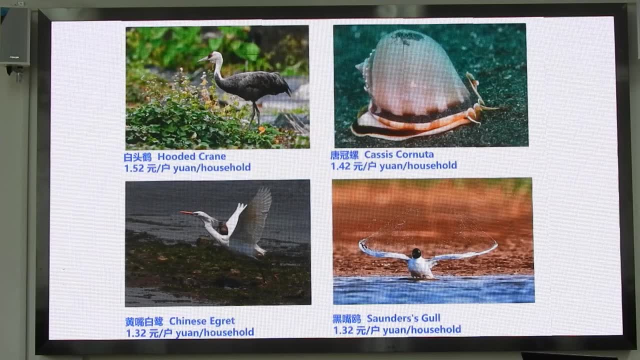 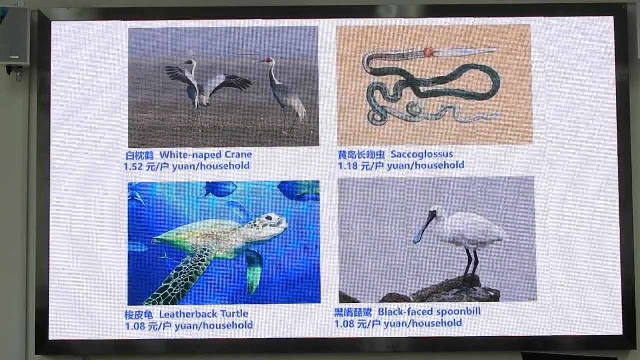 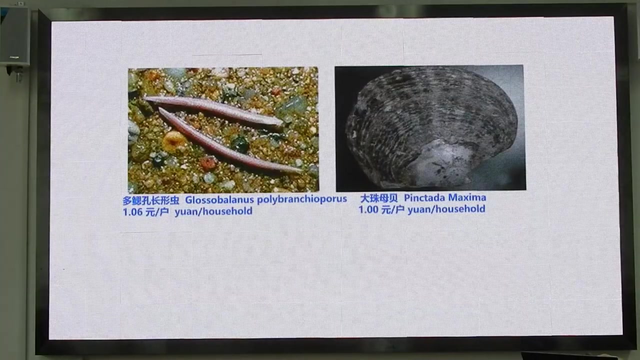 Chinese Yen For Chinese ivory. 1.3 Chinese Yen For red coral. 2 Chinese Yen For red coral. 2 Chinese Yen For red coral. 1.3 Chinese Yen For red coral. 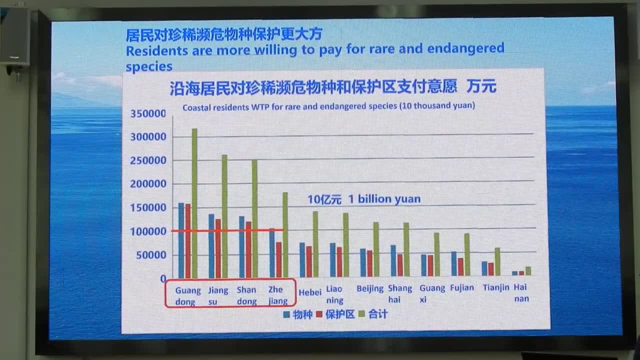 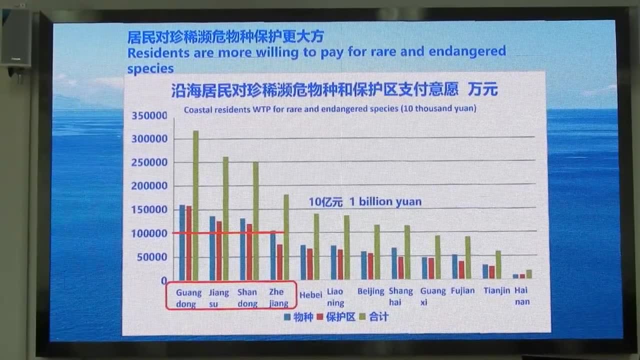 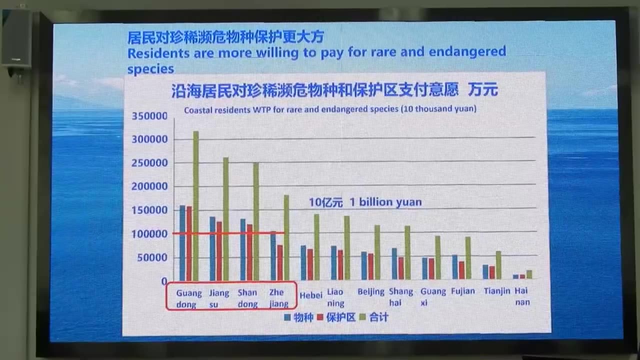 2 Chinese Yen. For red coral: 3 Chinese Yen. The third is the fourth sale total willing to pay is from Jiangsu. the third one is from Shandong province. the fourth is from Zhejiang province. 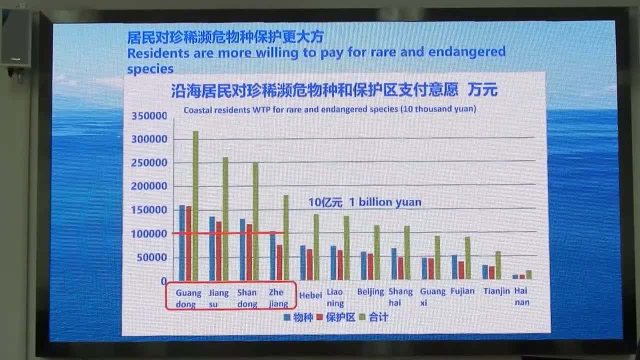 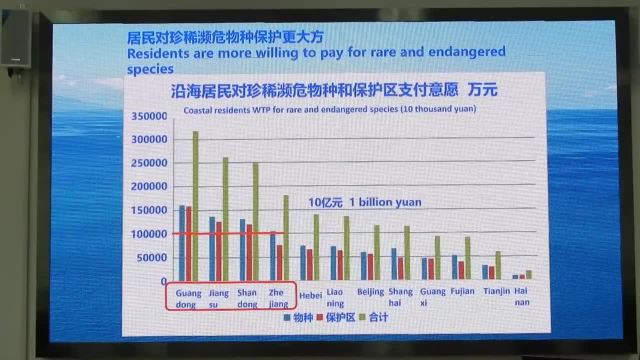 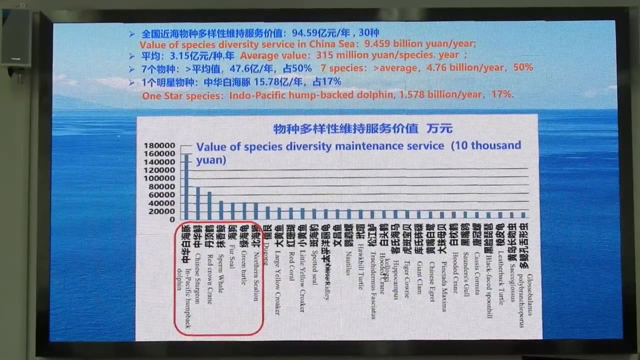 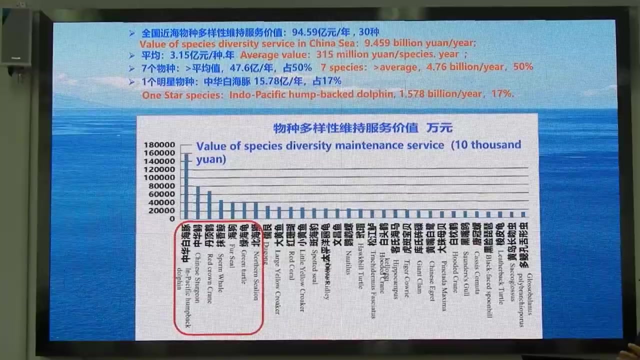 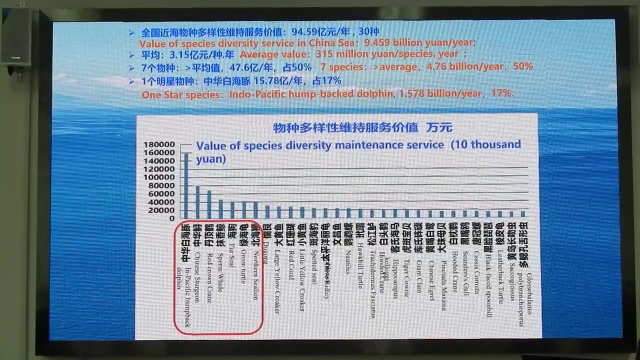 The willing to pay depends on the income level and person's ocean awareness. The value of species divestment financial services is the total willing to pay From 12 costa province. the total value of 30 species is 9.459 million CNY. 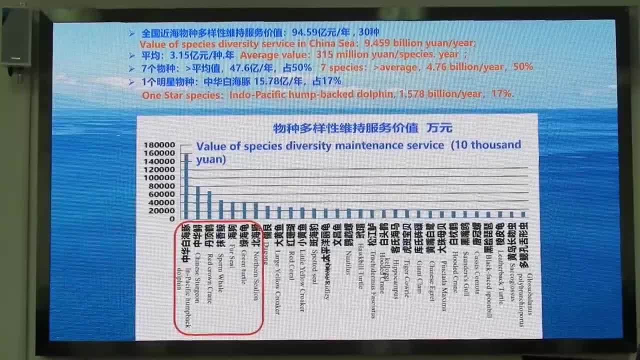 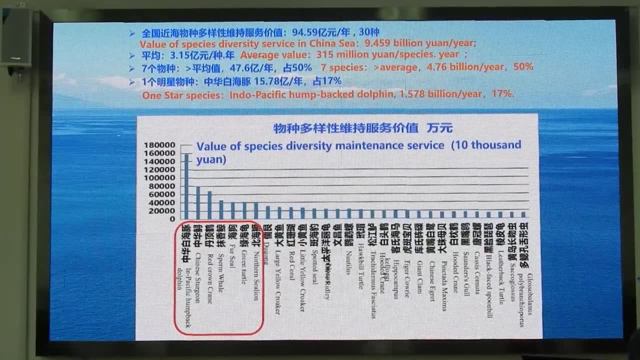 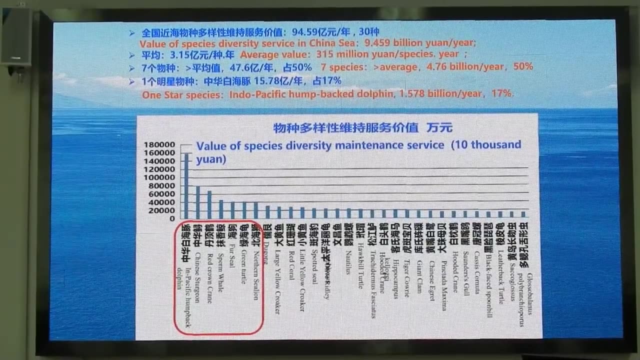 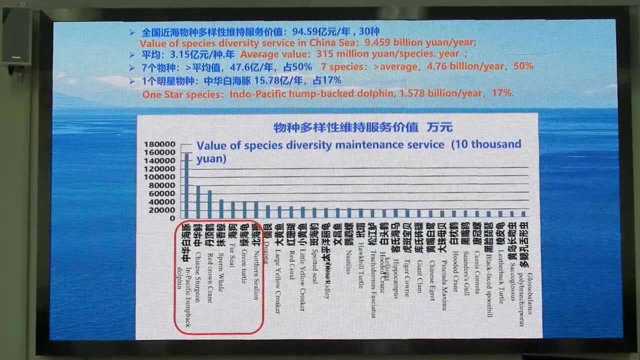 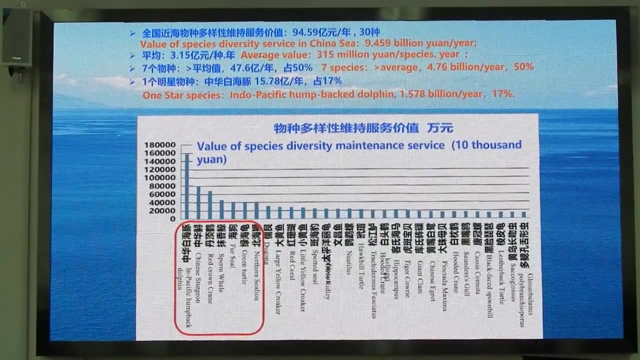 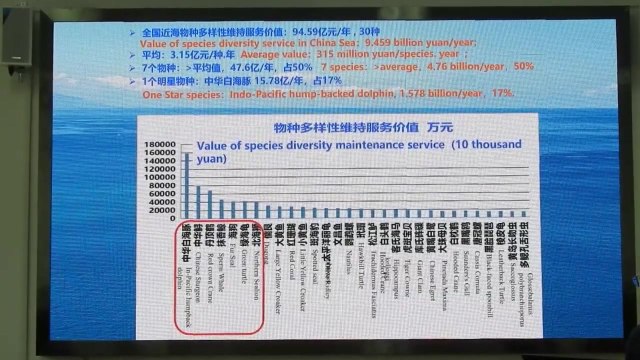 The average value is 350 million CNY per species in one year. These seven species' value is more than the average. The total value accounts for 50% of the total value. The Chinese Dolphin is a famous star species. Its value reached 1.578 billion CNY per year. 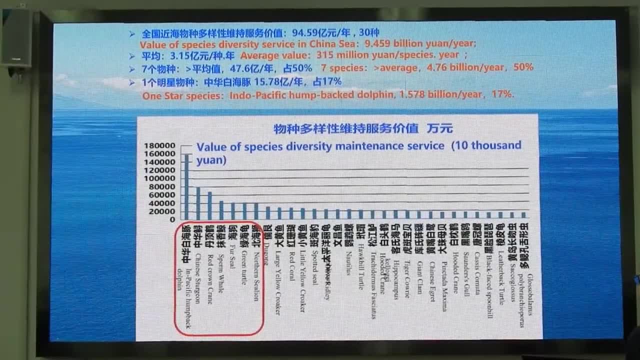 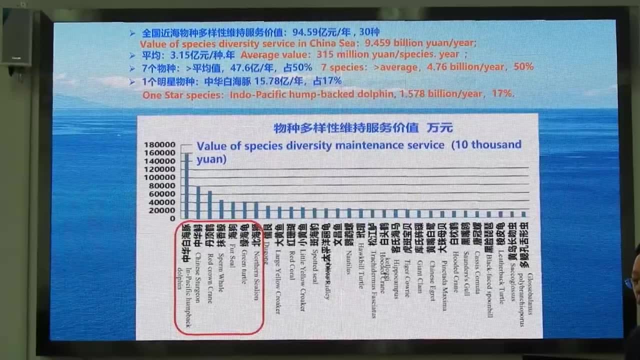 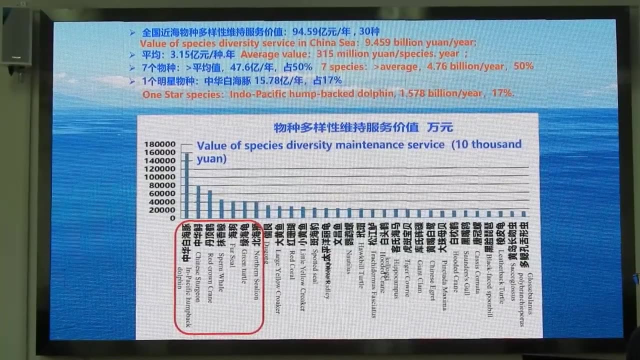 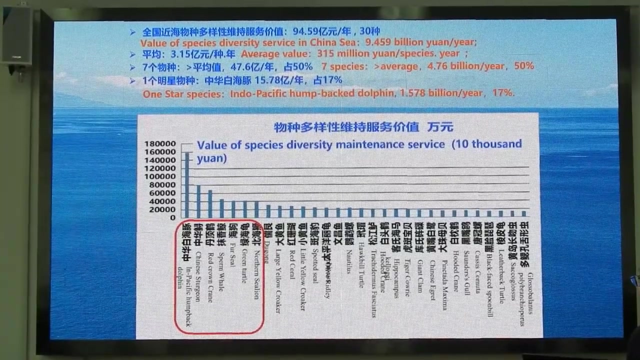 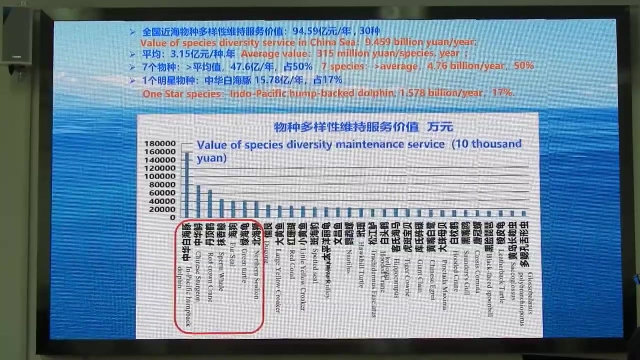 It accounts for 17% of the total value. Each individual Chinese Dolphin is worth 394,000 CNY per year, about half a million CNY. The price of this Chinese Dolphin decided by the Agricultural Ministry is 2 million CNY. If we consider that in all of the urban residences willing to pay, the total value of this Chinese Dolphin is very rich. The total value of this Chinese Dolphin is about 2 million CNY If we consider together the species divestment maintenance services. 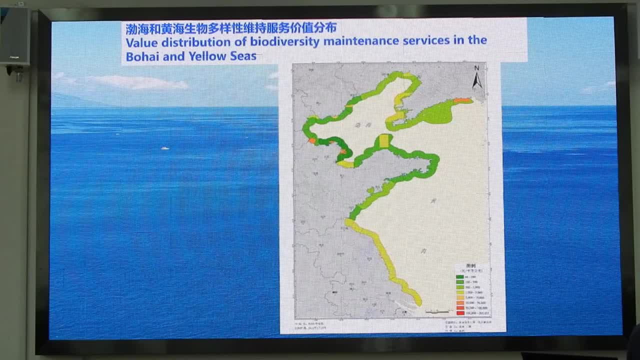 and the ecosystem divestment maintenance services. together we get the following: The value means the highest value, The yellow is the median, The green is the low value. In the Bo'ai Sea, the highest value is in the Yellow River Delta. 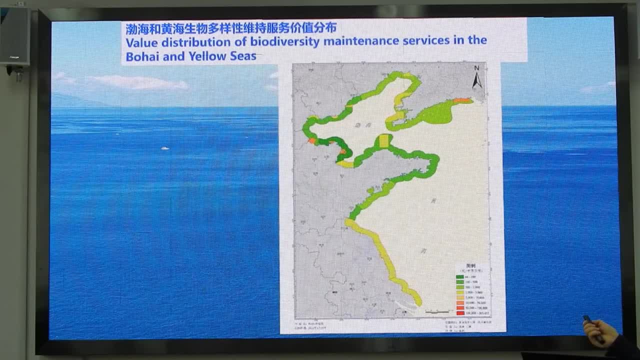 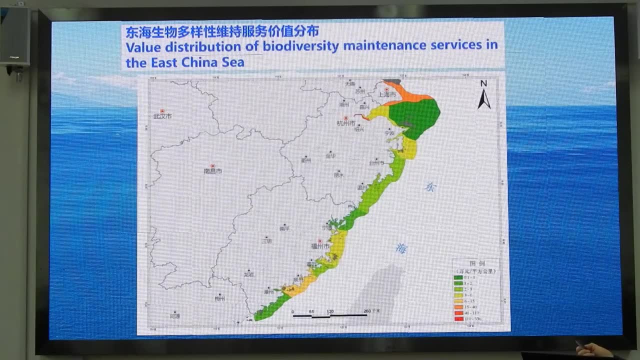 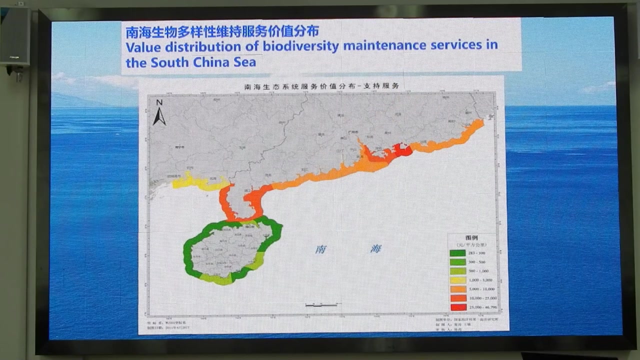 What else is there Also in Yangtze River Delta In East China Sea, the highest value is in the Sun High Coastal Waters. The red is the Yangtze River Earth Stream. In South China Sea, the highest value is around the Hong Kong waters. 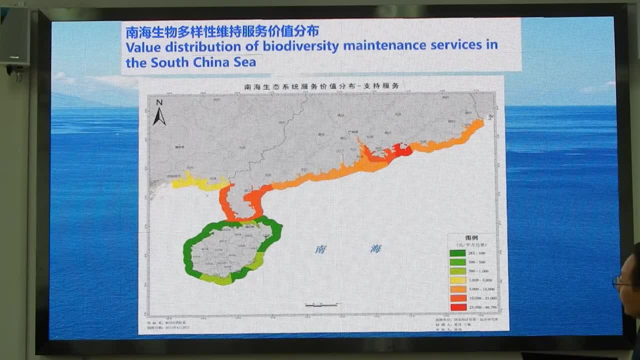 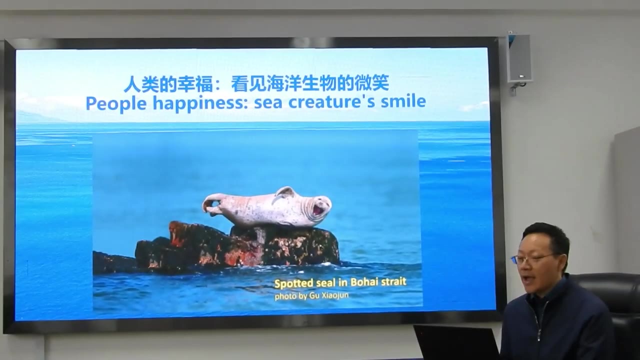 Shenzhen waters, Also in Zhangjiang. the highest value is in the Central China waters. The same is the life support system of us. We need to save, not save in us. I expect to see the same creatures smile In history. 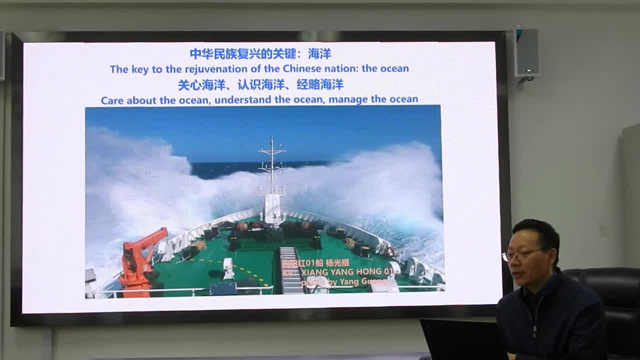 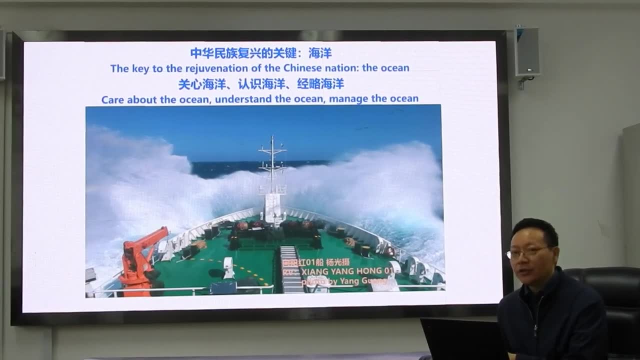 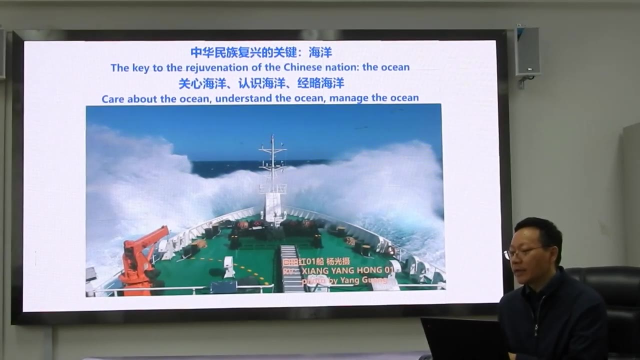 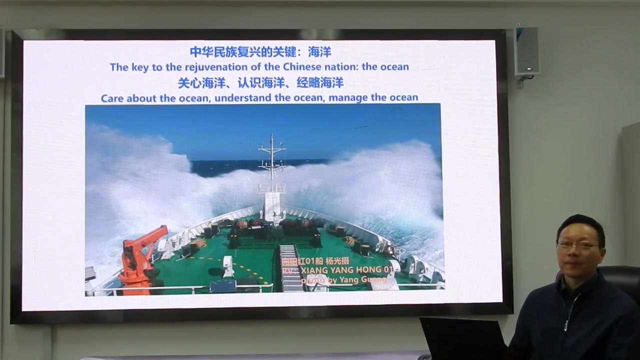 the Chinese nation lost the ocean. to realize the regeneration of the Chinese nation, The point is still in the ocean. I sincerely invite everyone to hear about the ocean more. understand the ocean. Let's manage the ocean for our shared future. Thank you. 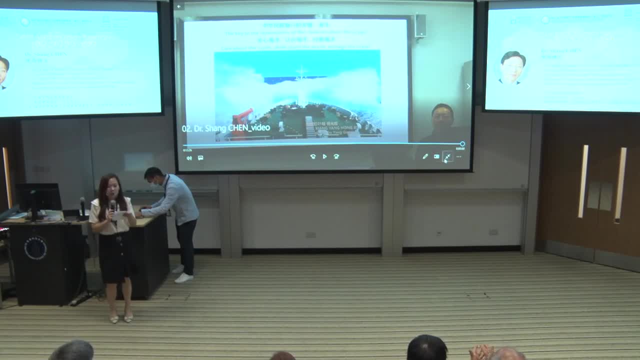 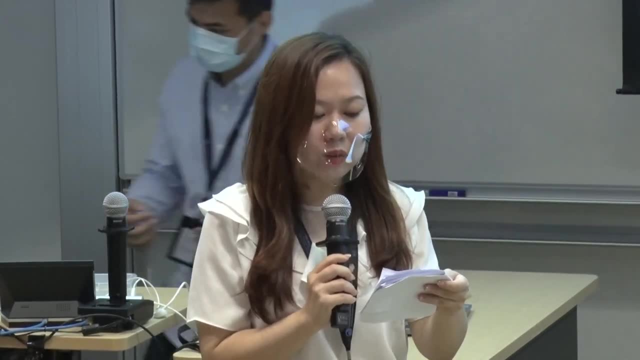 A very informative and detailed sharing. So we'd like to express our gratitude to the keynote speaker first. So may I now invite Professor Qian Peiyuan and also Professor Kevin Chang to present the thank you certificate and also souvenir to Mr Eddie Ng first. 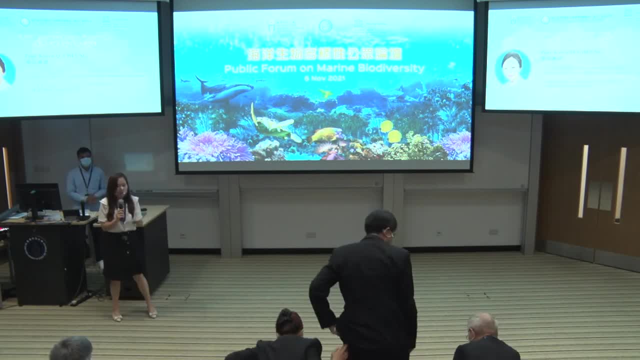 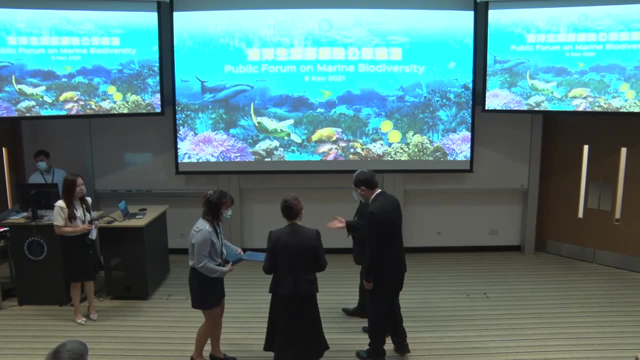 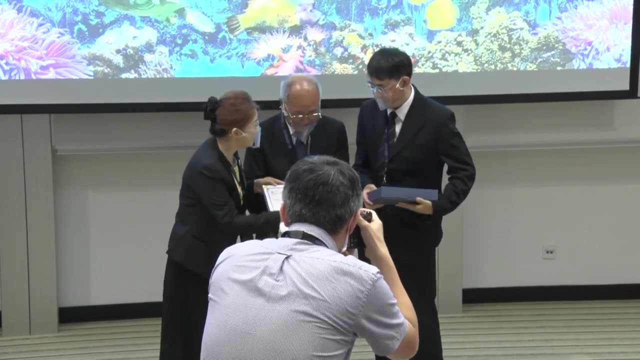 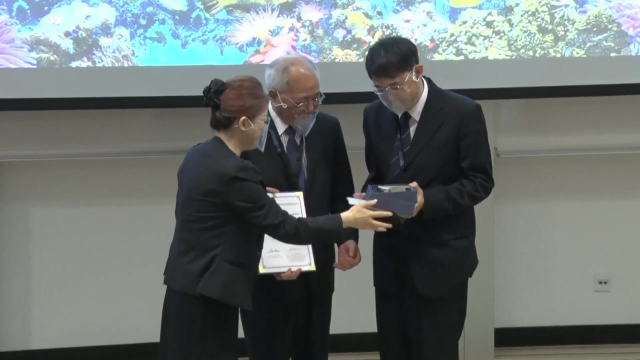 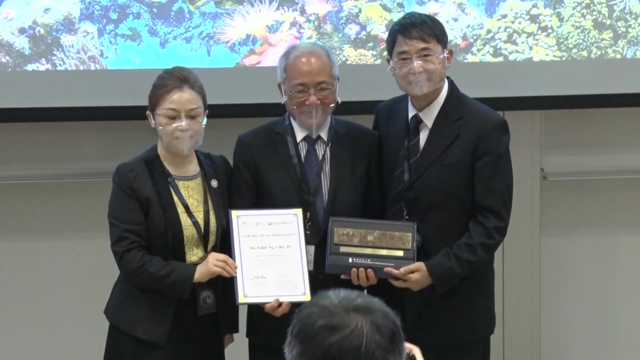 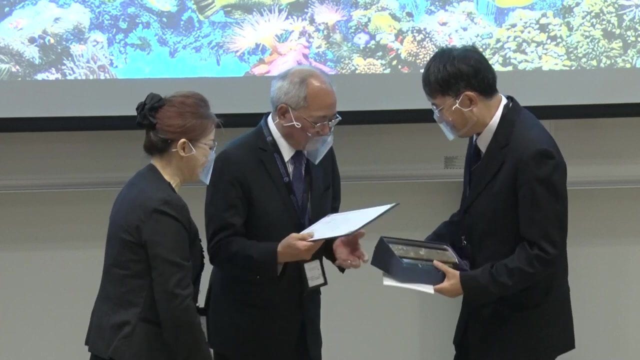 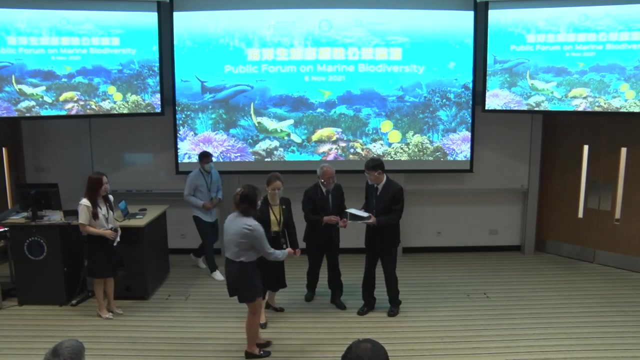 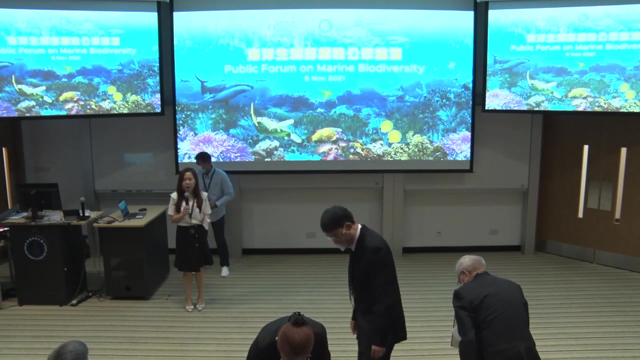 Professor Qian, Professor John and Mr Ng. please come forward. Okay, thank you. Please be seated. Before our break time, we wish to have a group photo with all the participants And the first group photo we will take right here. 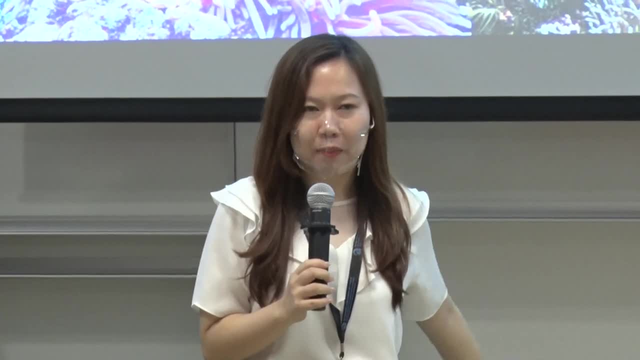 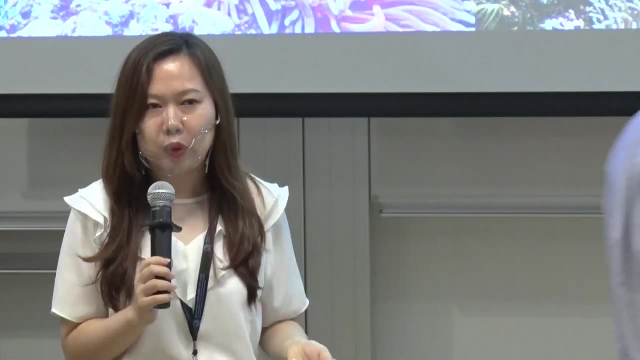 and our photographer will shoot the photo from our side, And you can just remain on seat first. After that, we wish to invite all of you to go outside in front of the backdrop for another group photo. Then we'll have an around 15 minutes break. 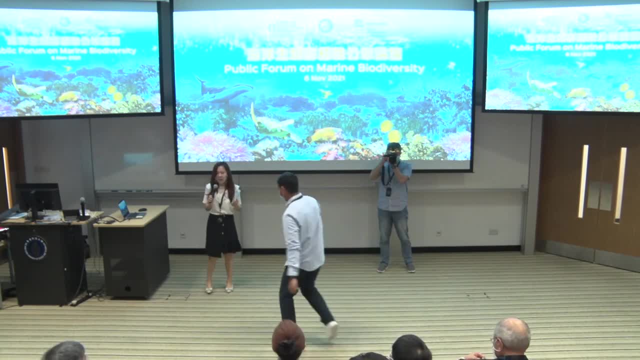 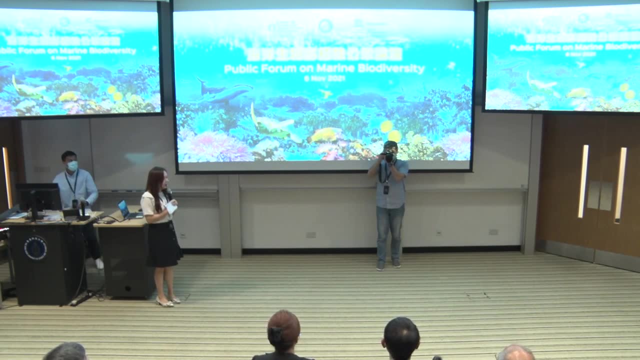 and come back at 3.50.. Okay, Three, two, one. Okay, another photo. Three two, one. Okay, thank you. Let's go out for another group photo in front of the backdrop first. Okay, may I have your kind attention please? 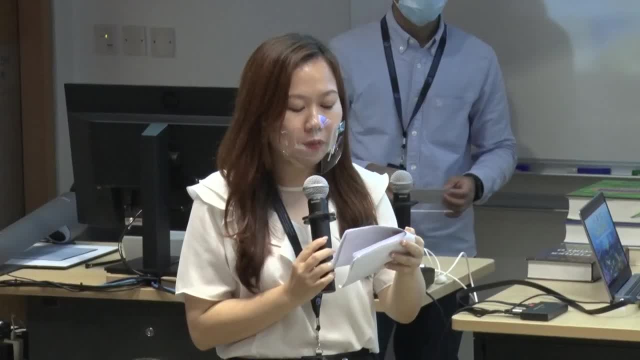 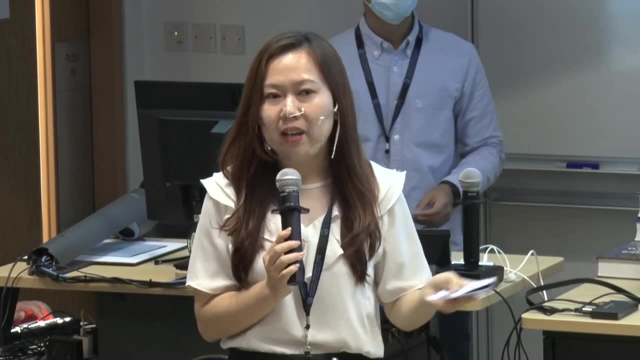 We are about to begin the next session. First of all, you are all invited to scan the QR code on the screen anytime to ask speakers questions, And our staff will select some of the questions which will be discussed during the panel discussion and Q&A section. 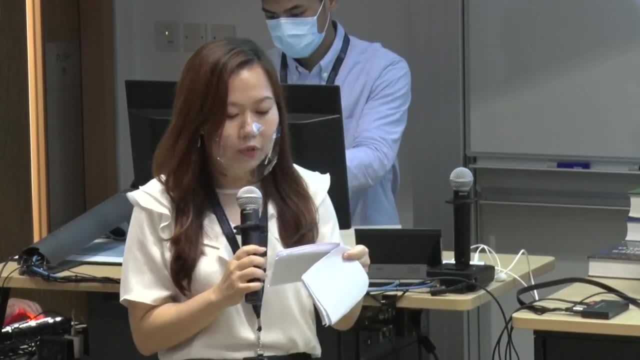 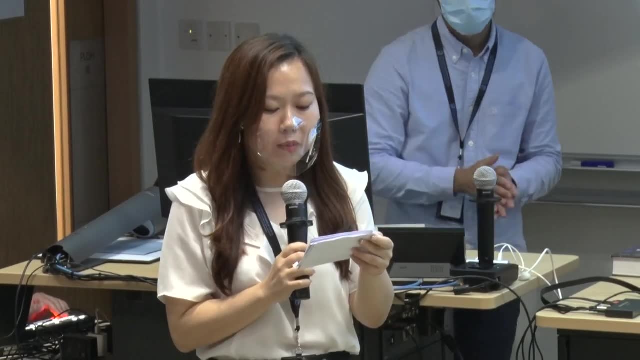 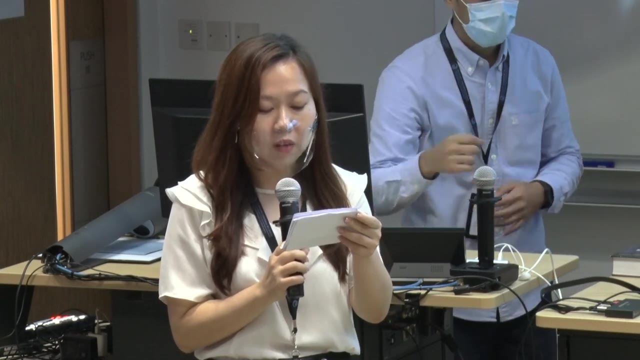 Okay, First of all, let me introduce our first guest speaker, Professor Thomas CC Wong, Executive Committee Member and Chairman of Sustainable Development Committee of the Chinese Manufacturers Association of Hong Kong, and also the former advisor of Endangered Animal and Plant Office. 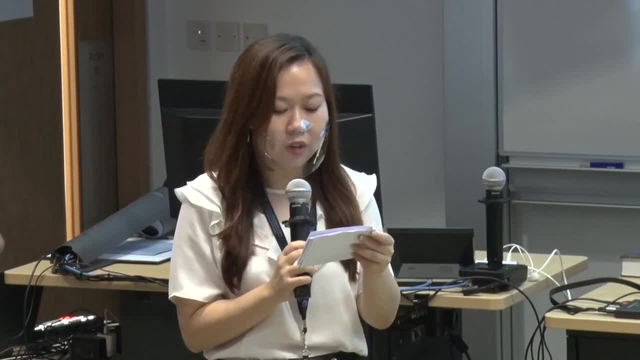 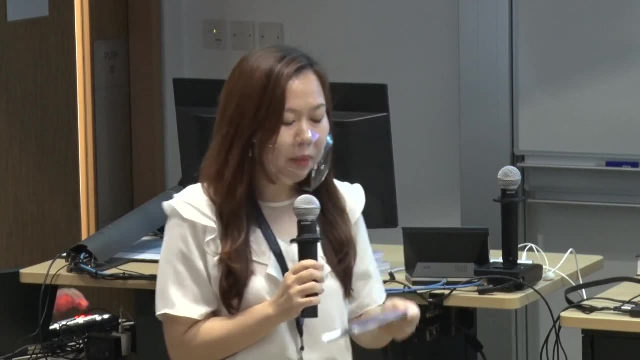 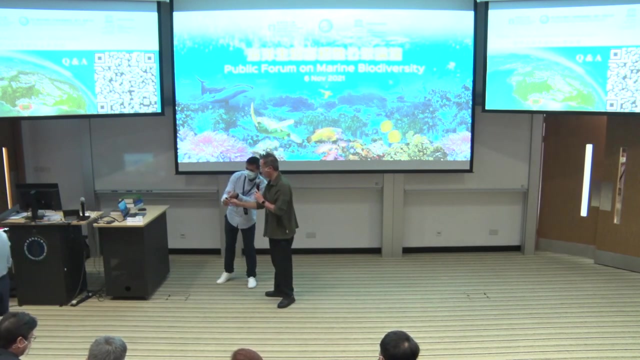 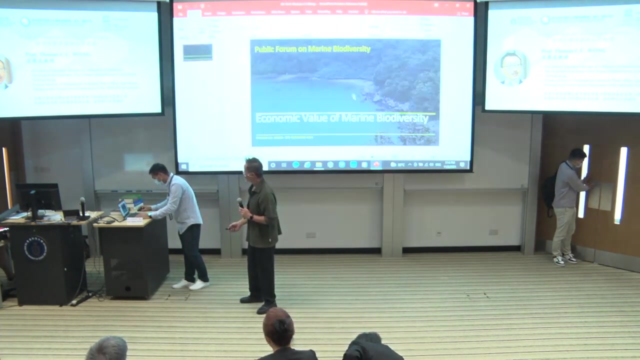 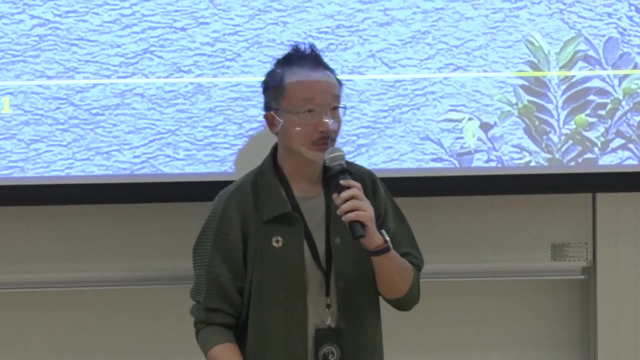 Agriculture, Fisheries and Conservation Department of the Hong Kong Government to share with us the economic value of marine biodiversity. Please join me in welcoming Professor Thomas Wong: Hello, hello, Hello. Ladies and gentlemen, distinguished guests, good afternoon. My topic today is economic value. 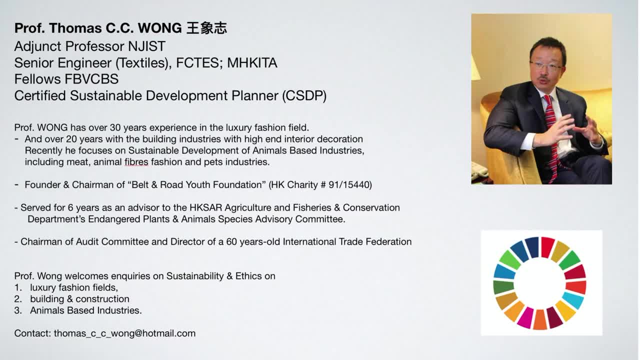 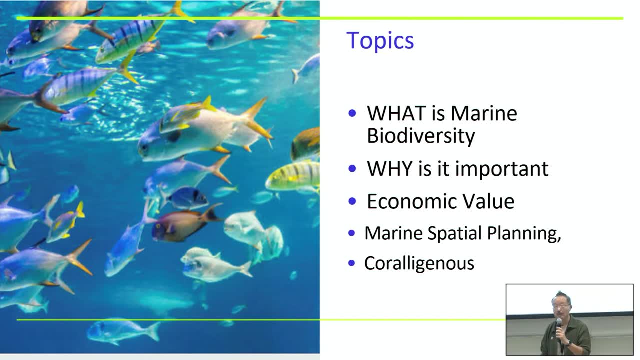 of marine biodiversity. This is me. Okay. I was thinking how should I go about talking about this. Maybe I will start with what is marine biodiversity, And then what is important, And then economic value, Things like marine spatial planning and all this. 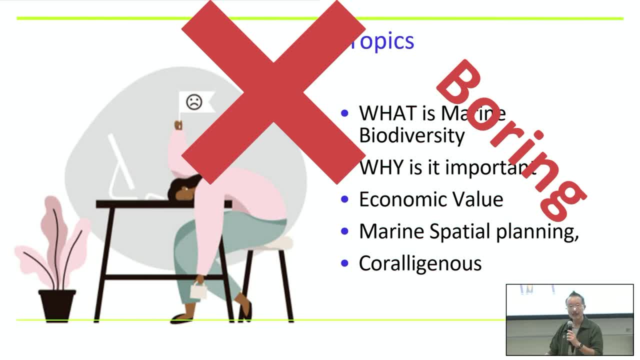 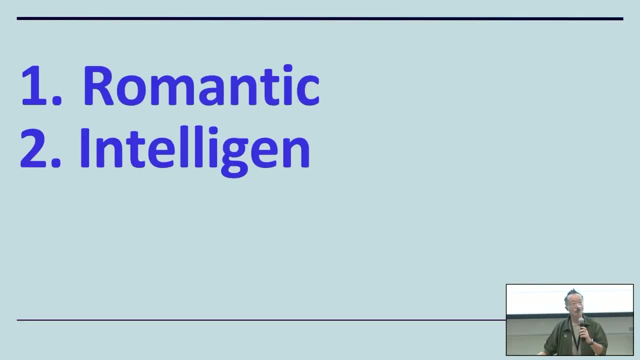 But I thought that would be boring, wouldn't it? So I said, no, I'm not going to do this. So what am I going to do? I'm going to start with some romantic stories, And since all our audience are intelligent people, 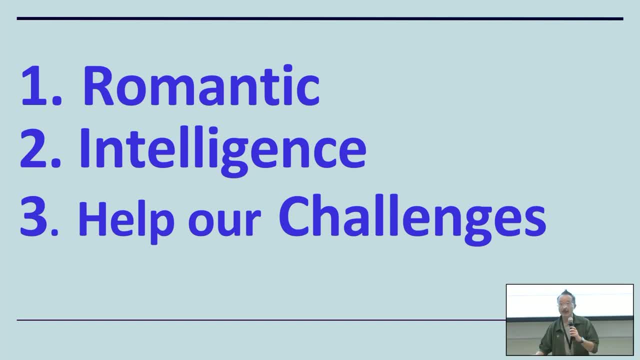 so we'll be talking about intelligence And then, at the end of the day, of course, we have to come back to how this would help our challenges. How would they help us to face our challenges? Romantic, Don't? we all love romantic stories? 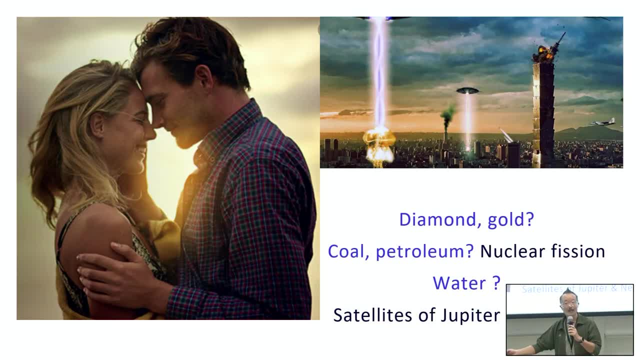 Let's start with this one. John loved his wife, Community, Nation And planet Earth. But one day, planet Earth received warnings from aliens Said that: hey, human beings, we are on our way. We are coming to destroy you. 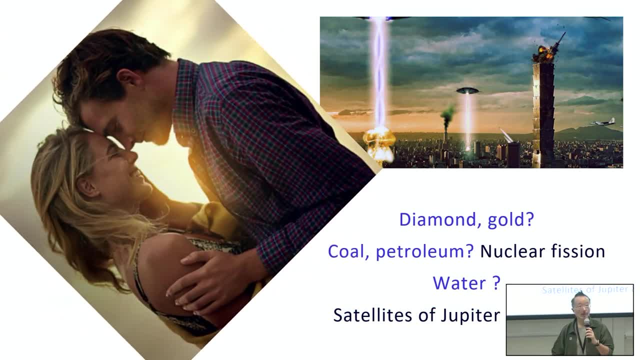 to conquer you. So John said to himself: I want to save my family, I want to save the world. So first of all John had to find out: why would the aliens come and conquer us? When you start a war, there must be something you want to get. 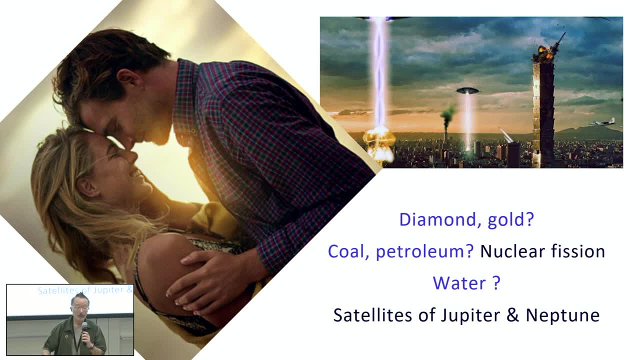 from the other people. That's why you would start a war, right? So what would these aliens possibly want from the Earth? He looked at himself. he said: what is of most value to me- Diamonds, Gold. But he know. 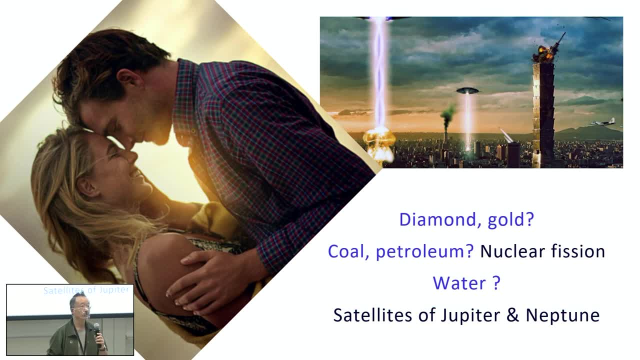 aliens are not interested in this, because diamonds and gold are symbolic values for humans. Critical value, Very small. Maybe they're looking for anything. they're looking for energy, Petroleum, But then they think. but then John thinks with aliens. 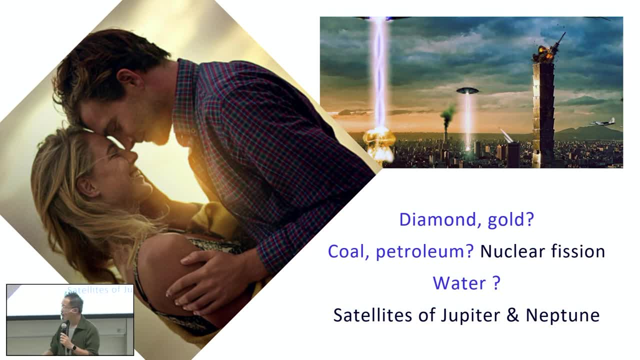 if they can travel at light speed, they must possess nuclear fission, So petroleum would be of no value to them. Ah, John thinks maybe it's water. Besides, 70% of the Earth's surface is covered by water. 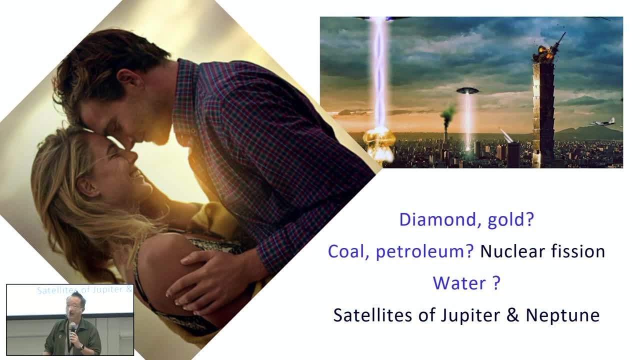 Maybe that is the answer, But later on he found out that that is not true, because in satellites in Neptune and Jupiter there are also water, maybe more water than Earth. So what would possibly these aliens want from Earth? The answer is very simple. 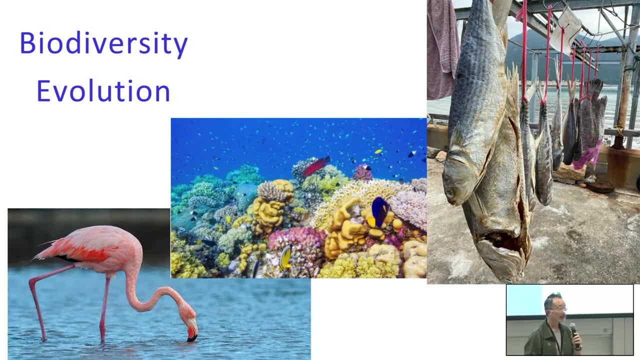 Biodiversity. Why is that? Because every time, okay, to start with, we are like a single-cell, amoeba-like organism And when we evolve, like a complex organism, like a horse, like a bird, like a fish. 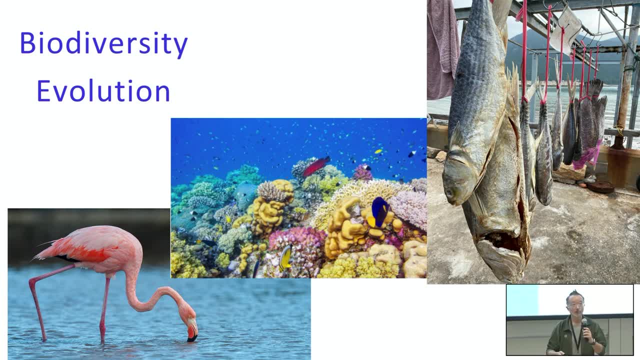 every time we evolve it's a solution to the problem we face at that time. So that means on every single organism. when you look at the DNA, it contains solutions to hundreds or thousands answers to problems. And if we have so many different organisms, 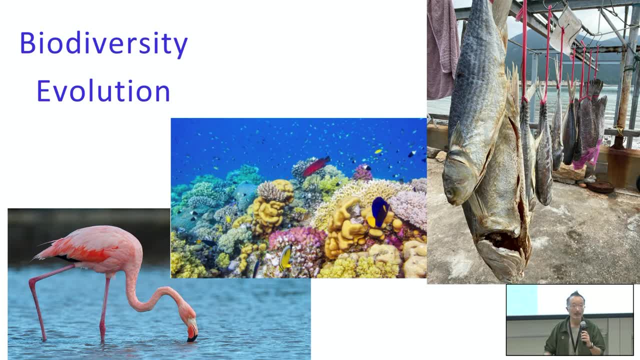 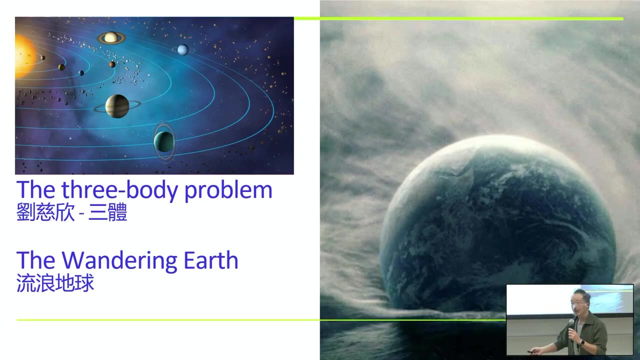 in the world. we are talking about millions or billions of solutions, So that is of value in the universe: Diversity, Biodiversity. Let's go to another story. I think many of us might have read this book: The Three-Body Problem. 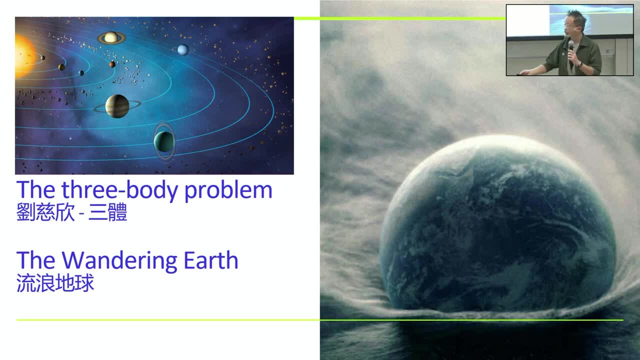 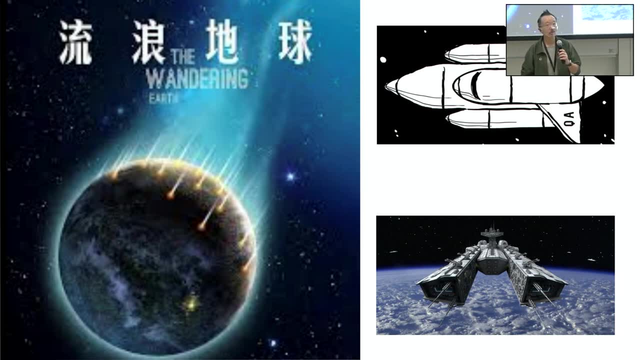 by Liu Zi'an, And it was made into a movie: Wandering Earth. The story goes like this: Human beings find out that the solar system- not just the Earth, the solar system- would be destroyed sometime in the future. So they come up with three options. 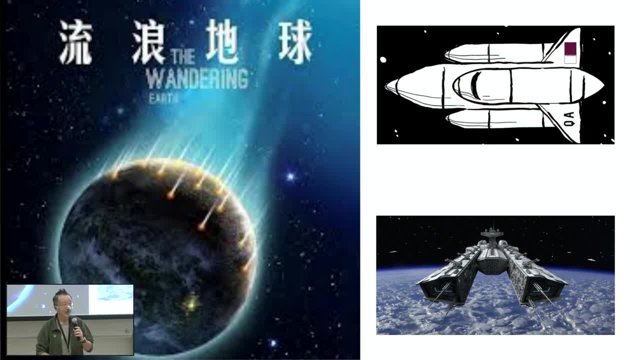 to save human beings. The first option is very simple: They will make millions of spaceships And on each one they put a few thousand human beings onto the spaceship And they fire them off in all different directions. Of course, the human beings. 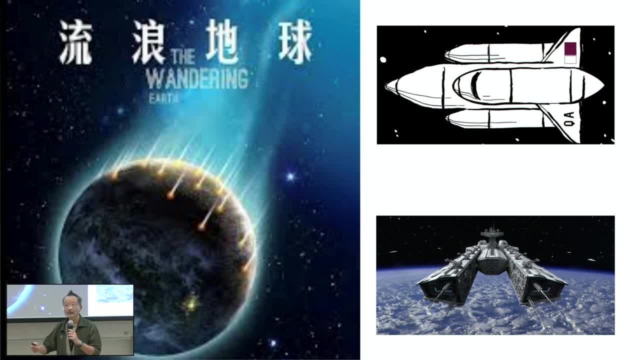 will be put to sleep at the beginning, And when this spaceship lands on a planet, a strange planet, the computer would test: If the planet is suitable for humans, they will wake the people up. If not, they will go about to another planet. 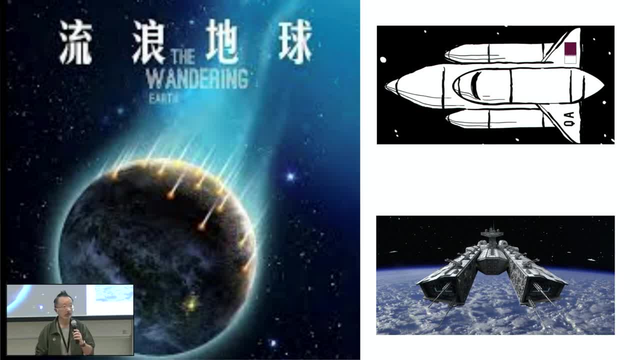 The second option is they will make a dozen of big spaceships And each one of them they put millions and millions of humans, like cities, And they go to different directions. And the third is the most difficult solution And that is they will move the whole Earth. 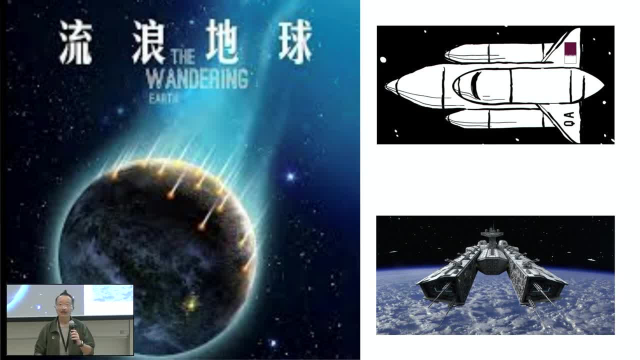 out of orbit. Ladies and gentlemen, which option would you go for? I talked to my friends. They said: isn't it obvious? Of course, option one, because it's simple, easy, sensible and you don't put all your eggs. 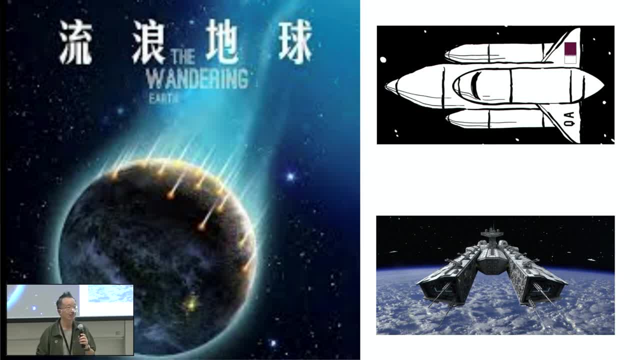 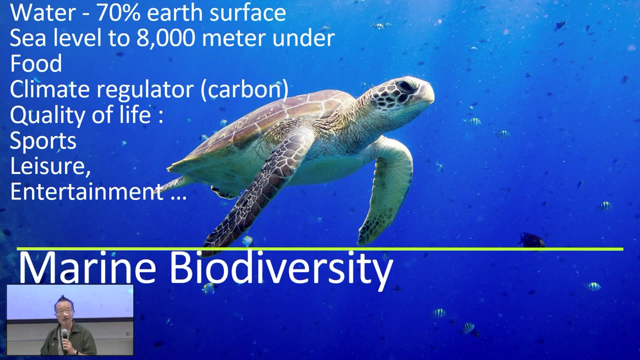 in one basket, right, So you get highest chance of survival for human beings. But the scientists go for option three. And the reason Again: biodiversity. So that is how important biodiversity is. So how about marine biodiversity? Look at these figures. 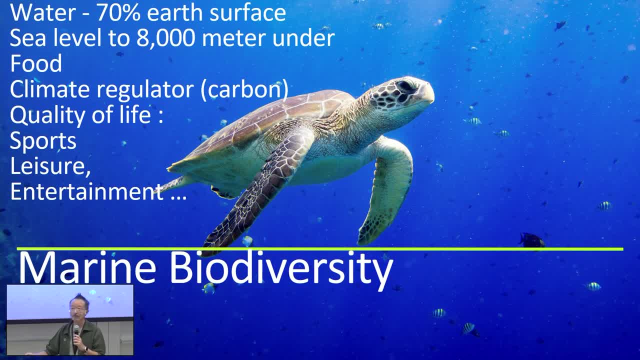 Many of these figures. you know. Water covers 70% of the Earth's surface And, unlike when human beings live on the Earth's surface, we are like living on a flatland, But in the ocean we're talking about from sea level. 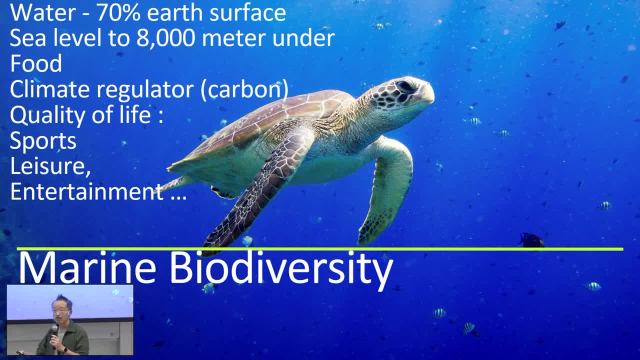 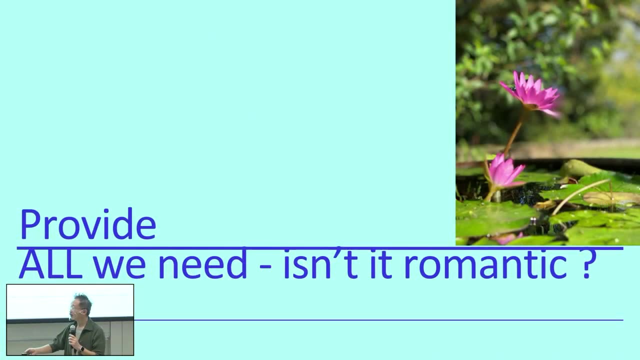 to 8,000 meters under below And they provide food for us and these climate regulators And this quality of life. I mean sport, leisure, entertainment and all this marine biodiversity, And the ocean and marine biodiversity provide all of this to us. 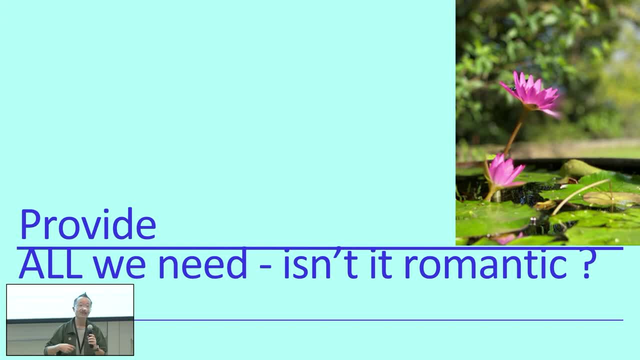 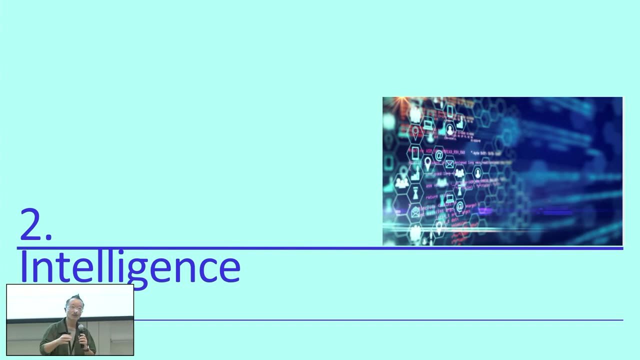 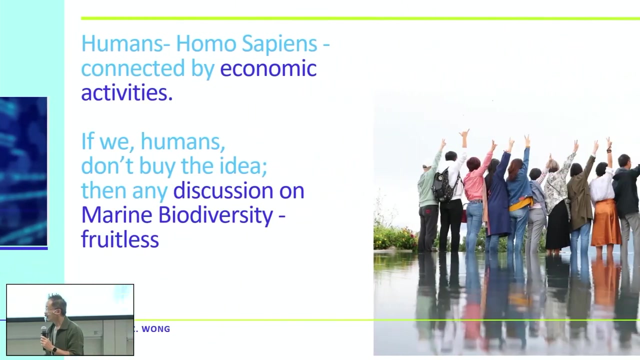 All that we need without asking anything back from us. So all give to us and nothing they ask back. Isn't it romantic? Okay, So that is the romantic part. In front of all these intelligent people, I have to come up with some intelligent topic as well. 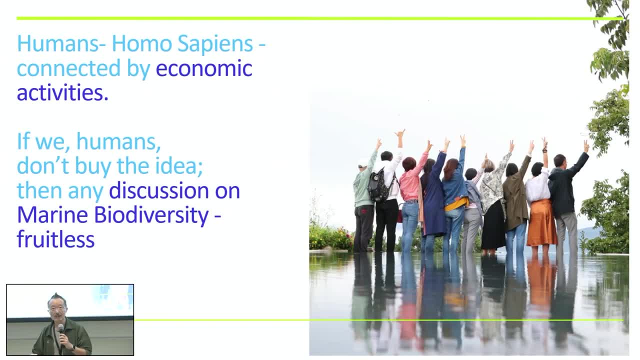 Human beings. How do we connect with each other, especially with strangers? Economic activities is the most efficient way of connecting human beings. Anything, if we want anything to work, we human beings must buy the idea. So if we human beings don't buy the idea, 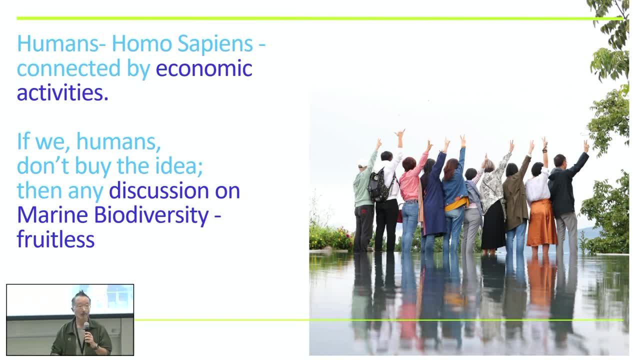 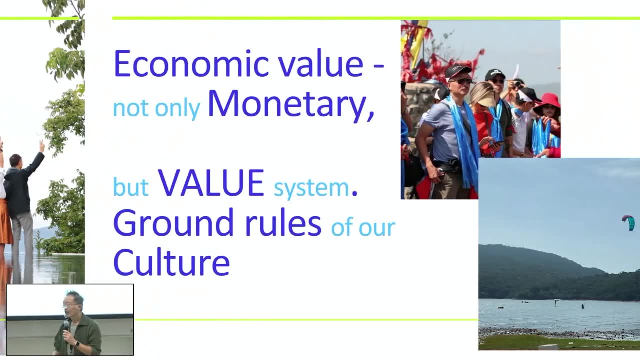 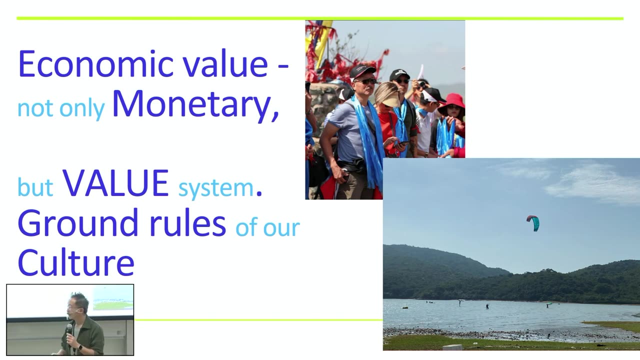 of marine biodiversity, then any discussion on marine biodiversity is meaningless, fruitless. So when we are talking about value, what are we talking about? I mean, all of we know that it's not just money we are talking about. We are talking about 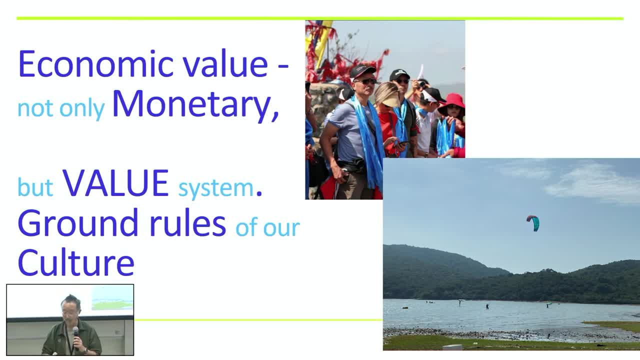 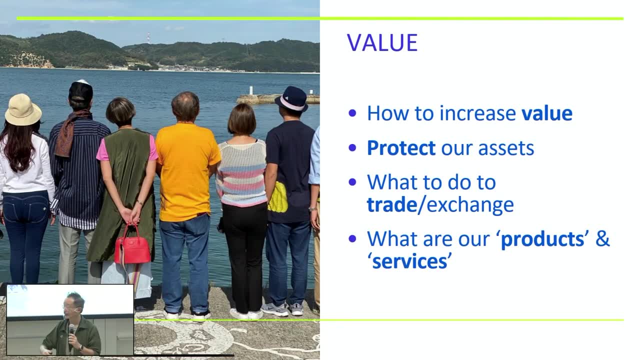 whole value system and the ground rules of our culture, Such as how do we increase our value, For example, how to make more money and all this, How to protect our asset, What to do to trade or exchange what we have with things that other people have. 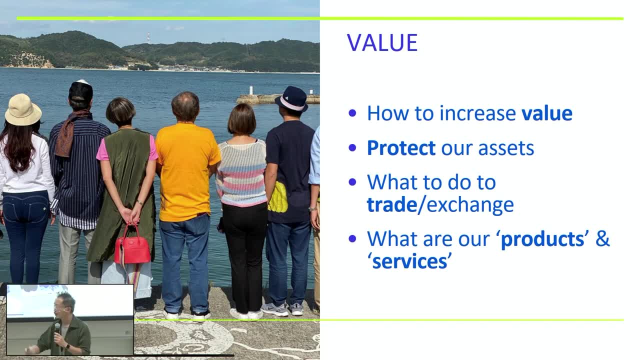 but we don't have or something that we want from the other people. How do we exchange or trade with them? And then it comes back to what are our product or service that the other people want. So this is the whole part of the value system. 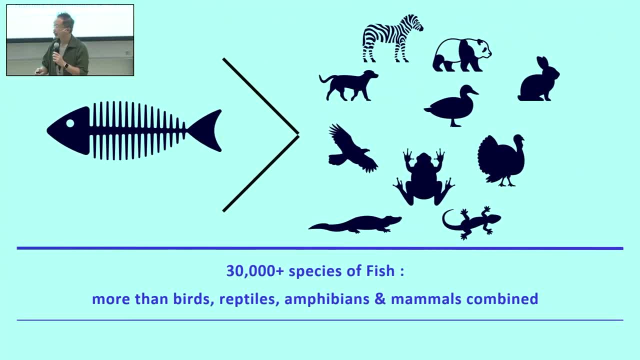 I mean the speakers before me. they have sort of touched upon this topic. Just fish, over 30,000, something like 34,000 species, And this is more than birds, reptiles, amphibians and mammals combined. That is the type of biodiversity. 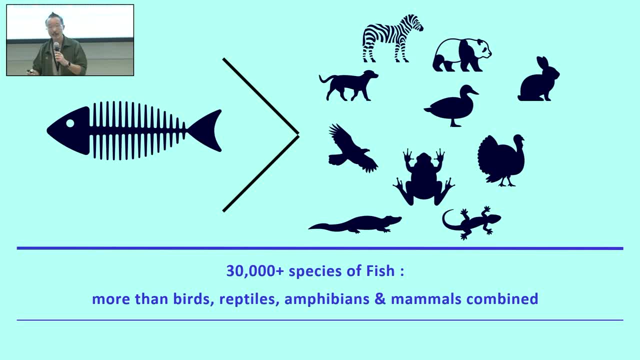 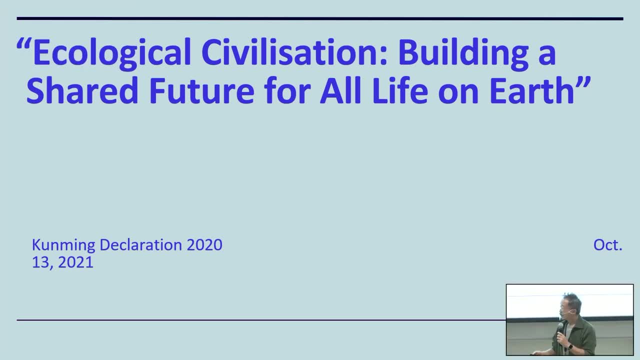 we have in marine And we are talking about just fish. I would like to use COP 15, Kwong Ming Conference. In the Kwong Ming Declaration it says: ecological civilisation, building a shared future for all life on Earth. 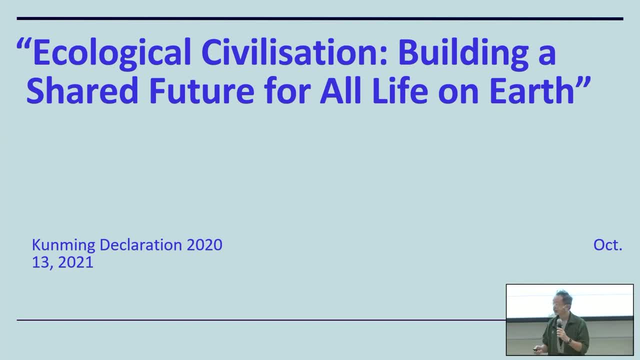 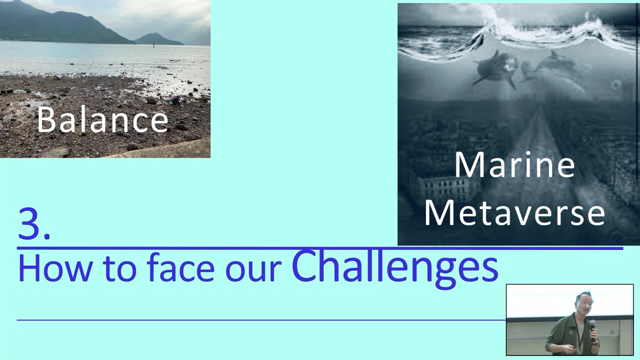 To me, the key word is shared future and life on Earth. These are the two key words. that hits me. So how do we face our challenges After we hear this romantic story, after all this intelligence? I propose balance and metaverse. 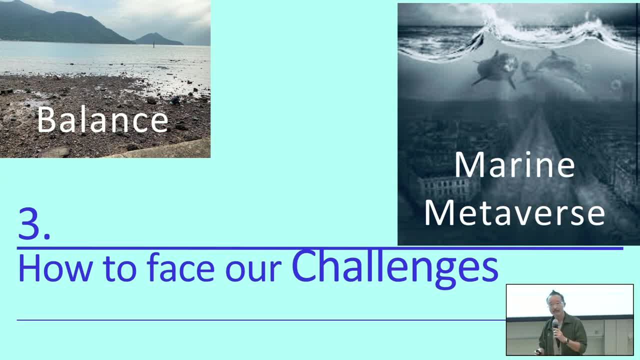 Balance may be easy to understand, But we will go into this later on a bit. How about metaverse? What does metaverse have? anything to do with marine biodiversity? Ladies and gentlemen, I propose to you that it has a lot to do with marine biodiversity. 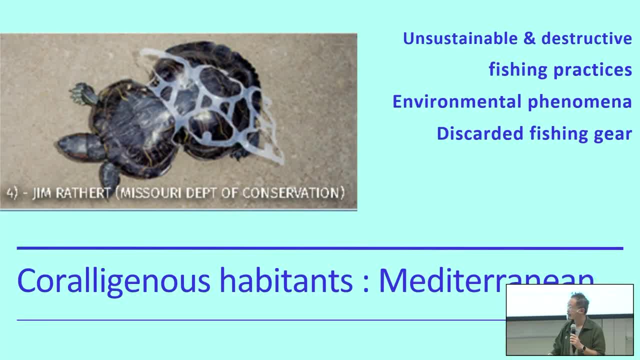 Let's see what happens. Balance and metaverse: What do we mean by balance? We can go into the Mediterranean to give you examples: Unsustainable and destructive fishing practice, environmental phenomenon, discarded fishing gears, All these- we can talk about this. 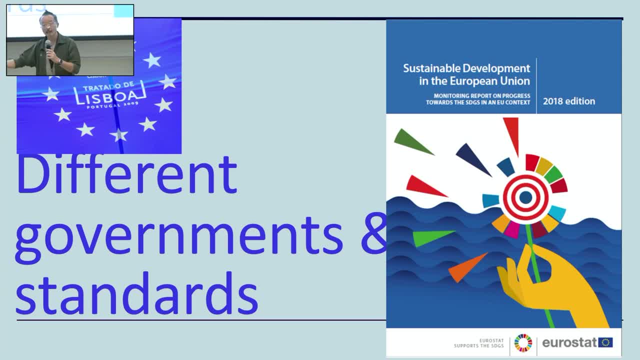 But how about solutions? But in addition to the last slide, we have even more difficulties: Different governments and different standards. Just with EU, we have the Treaty of Lisbon and we have the sustainable developments in the European Union. There are different standards. 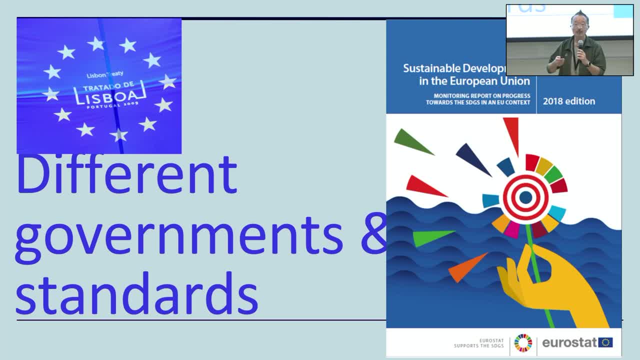 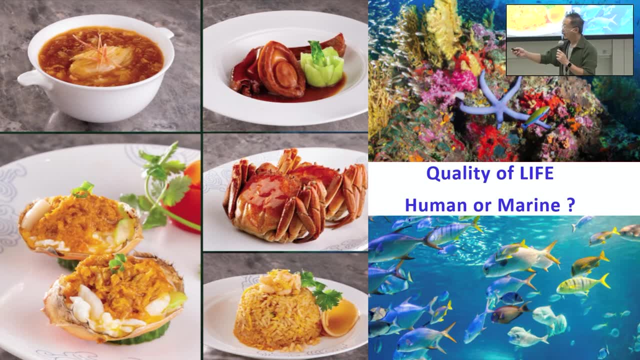 even within the EU. So they make a challenging situation even more challenging. So what are the solutions? First of all, we have to ask ourselves for the fish. do we want to put it on the desk as our food, Or we want to leave it in the ocean? 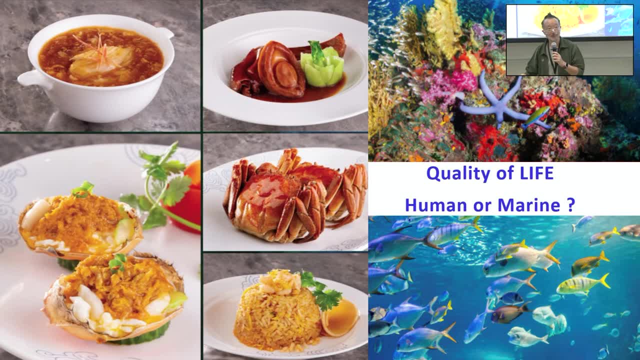 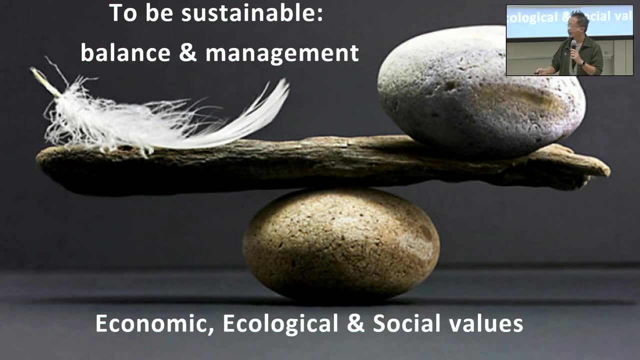 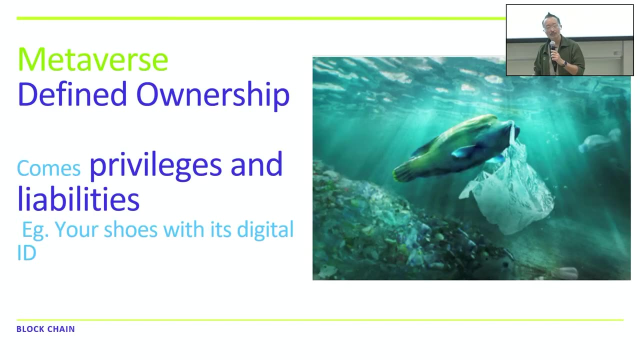 So when we are talking about quality of life, are we talking about human life or marine life? So the balance is very important. For balance I mean economic, ecological and social values. So it's balance and management. Metaverse. How could possibly metaverse? 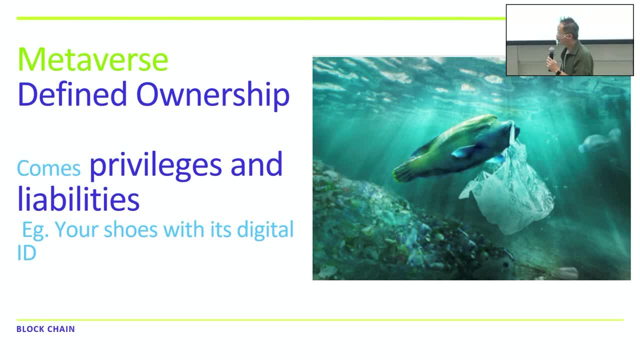 has anything to do with marine biodiversity. Metaverse is the best way to define ownership, And with ownership it comes privileges and liabilities, For example, if my shoes has its own digital ID and if one day you find a dead dolphin on the beach. 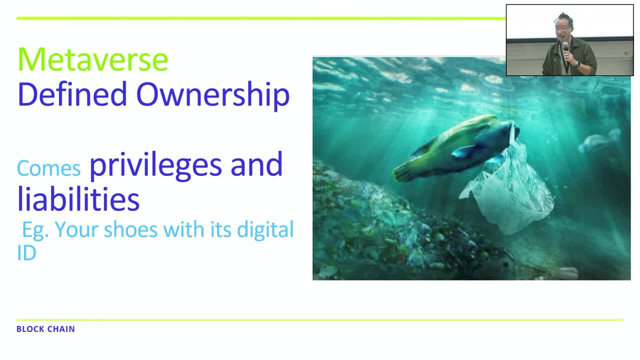 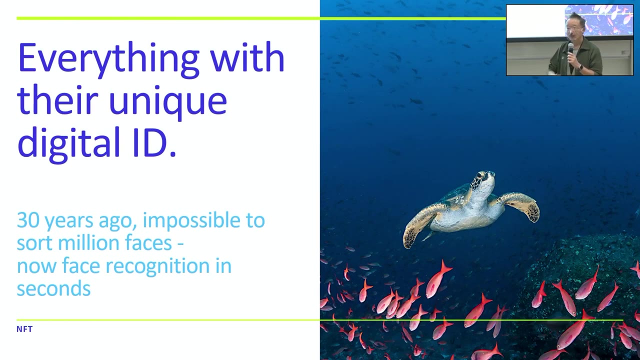 and when you do the autopsy you see that there's my shoes inside the dolphin's stomach and you can trace it back to me. I think I would think twice to see where my shoes would end up to. So in the metaverse, 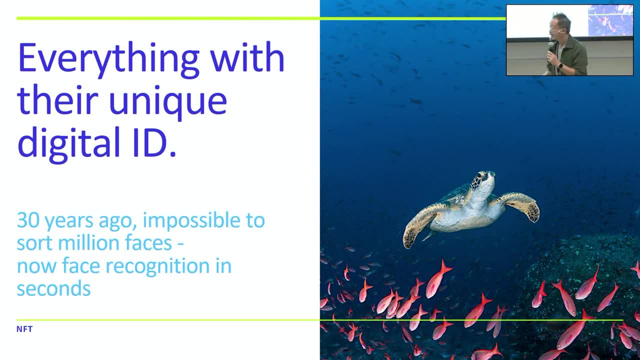 everything will have their own unique digital ID. Maybe you think: hey Thomas, this is almost impossible, if not difficult or expensive. Ladies and gentlemen, I want to ask you a question 30 years ago. if you have one million photos of human beings, 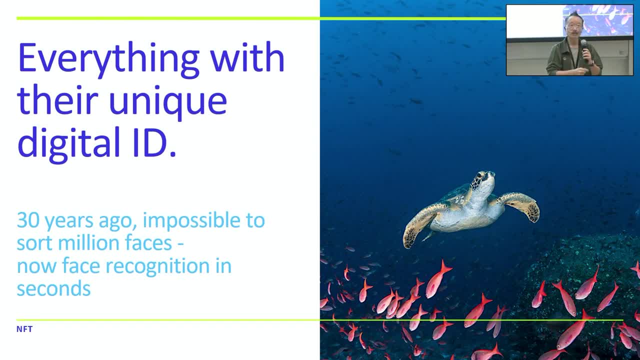 on your left hand. on the right hand you have one photo of someone you want to look for and you ask a computer engineer and say: can you compare this and tell me if there's any match? The computer engineer 30 years ago. 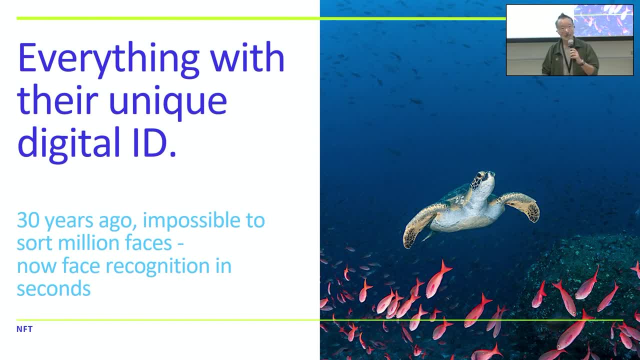 he would tell you: well, it's possible, but it takes almost a month And it's very expensive. But now, with Facebook- by the way, they changed the name to Meta- they can do a face recognition nowadays in just one second. 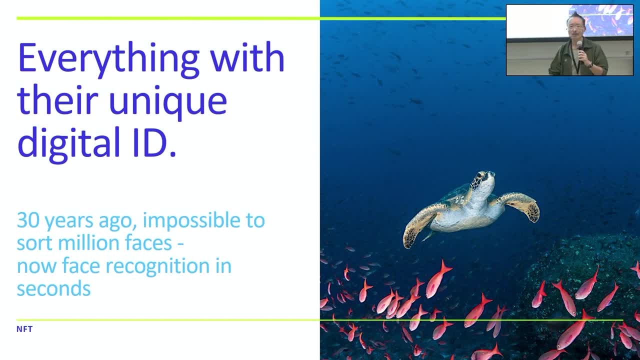 And they can do more than one million. the database is what one billion faces just in one second. What was impossible 30 years ago is just a click of a finger today. What is impossible today, 20,, 30 years ago. 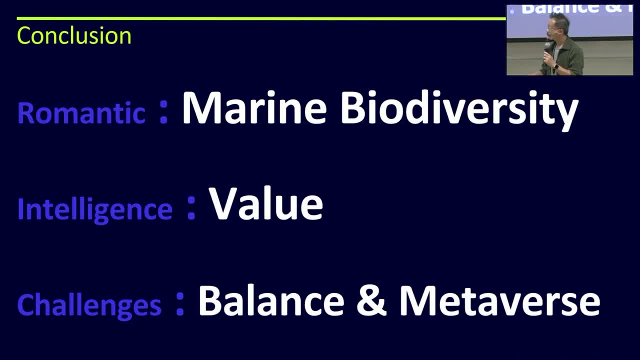 is a piece of cake. So digital ideas. So, ladies and gentlemen, I propose that we know how important marine biodiversity is. You know even the aliens. they want it from us And the value to us and the way to solve this is. 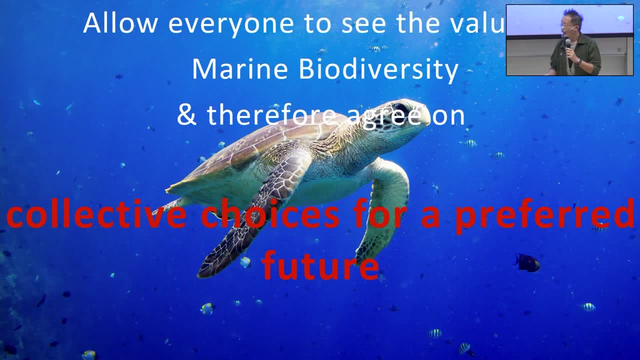 balance and metaverse. So I would say that allow everyone to see the value of marine biodiversity and therefore agree on collective choices for a preferred future, Because if we human beings do not agree and do not see it as a value, there's no way that we can. 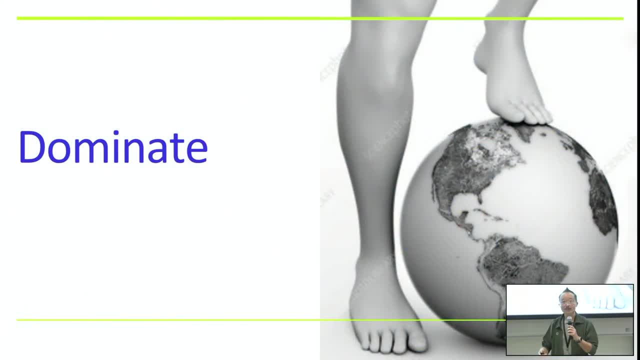 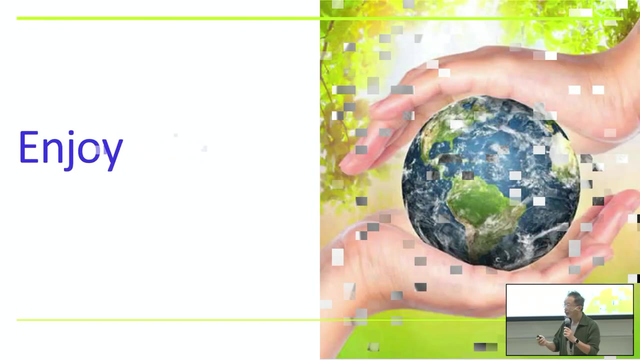 do anything. So, lastly, our relationship with the Earth. Now we dominate Earth, Like we are, like the owner of the Earth. Do we do we want to continue doing this, Or we want to enjoy Earth, To love and protect Earth? 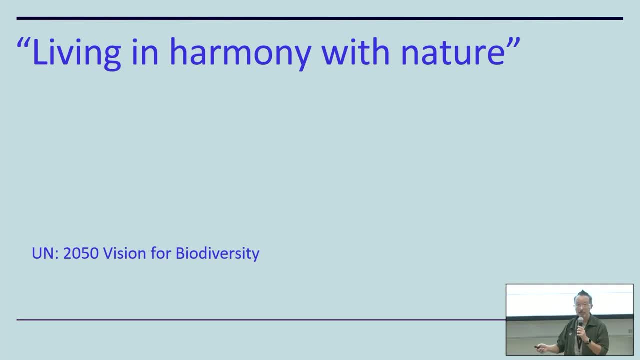 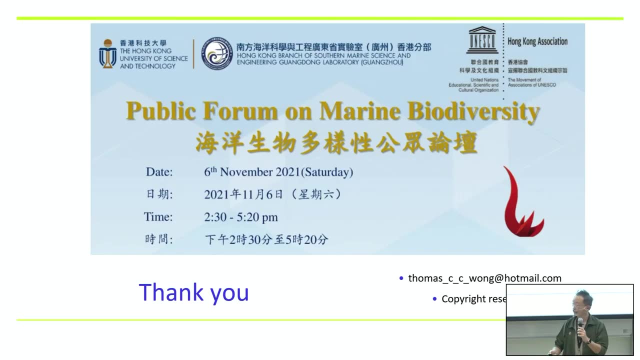 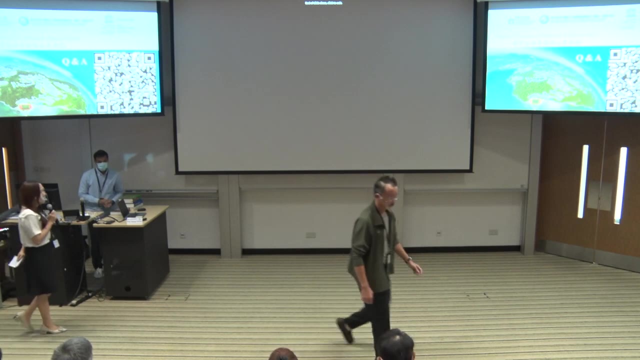 So, to end up, I will use United Nations 2050 vision for biodiversity: Living in harmony with nature. Thank you, Thank you. Thank you, Professor Wong, to share his different angle to see the relationship between human beings and marine biodiversity. 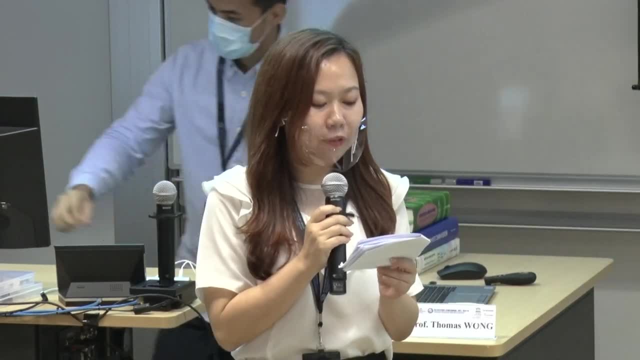 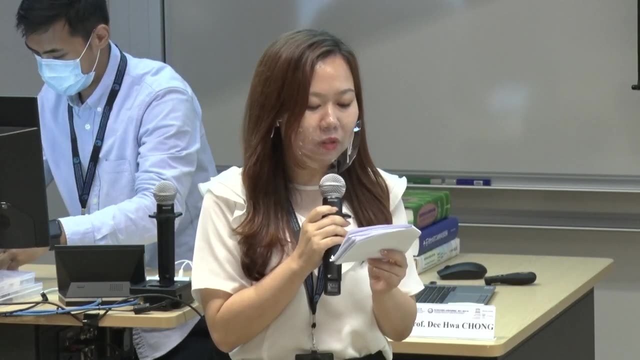 So, moving right along, we'll have another guest speaker, Professor Dewa Chong, the Society President of Ecological Society of Hong Kong, Academic Consultant of Laboratory of Ethology Shanghai Ocean University and also the Visiting Professor School of Life Sciences. 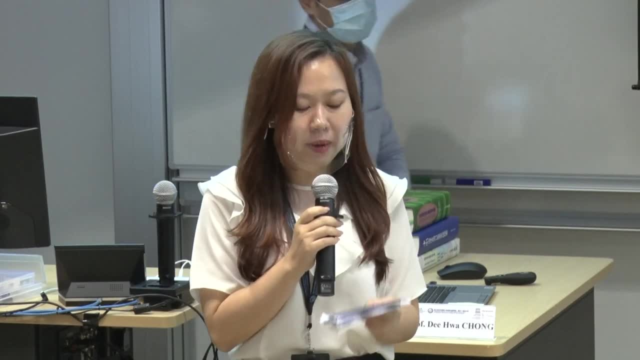 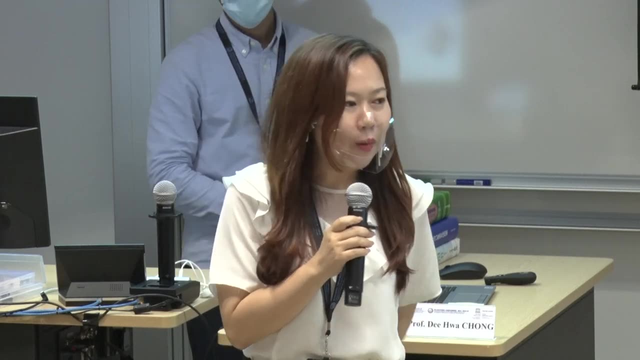 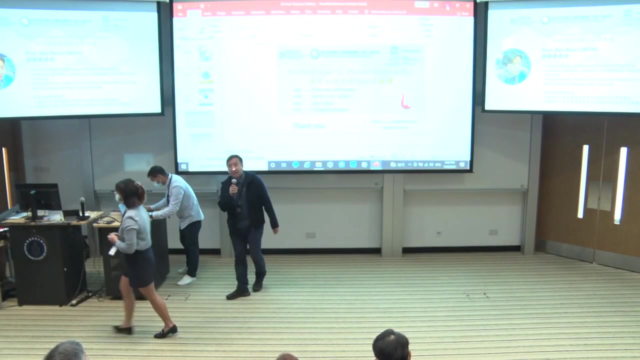 Department of Ecology and Evolutionary Biology of Fudan University, And he will share with us the diversity on the marine fishes of Hong Kong. Welcome, Professor Chong. Oh, thank you, And nice to meet you all. Actually, what I'm going to talking about, 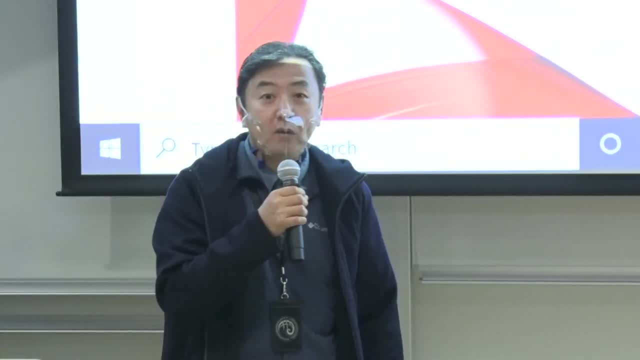 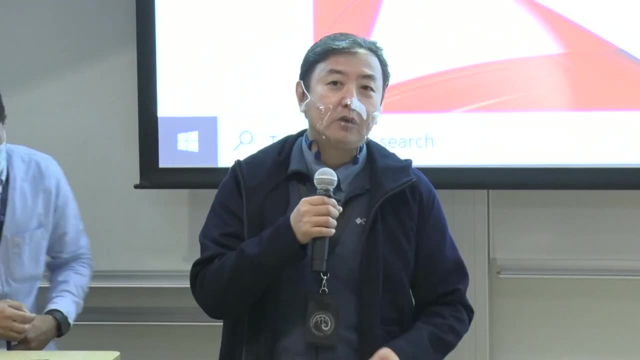 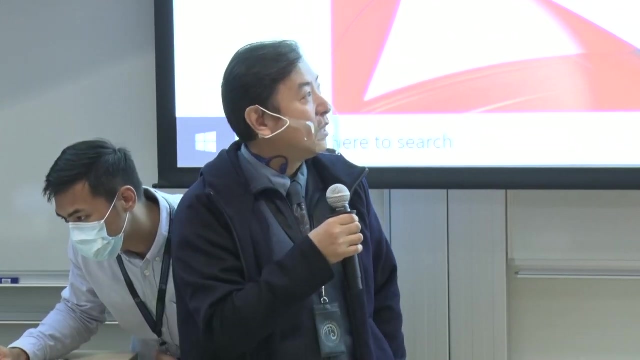 is biodiversity of marine fishes of Hong Kong And, as you know, at that time I established- they founded- the Ecological Society of Hong Kong more than 13 years ago And I found that at that time I found that it's quite strange that 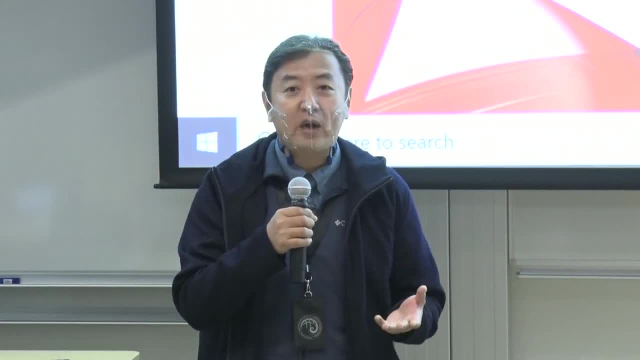 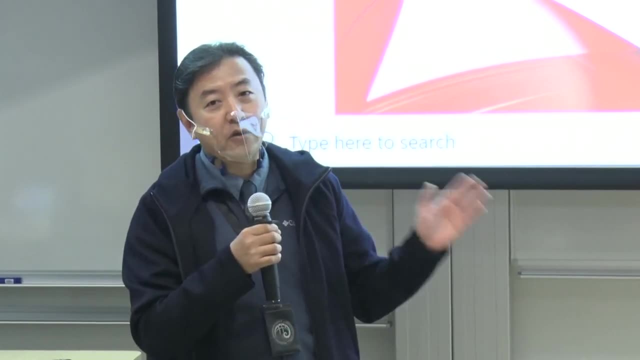 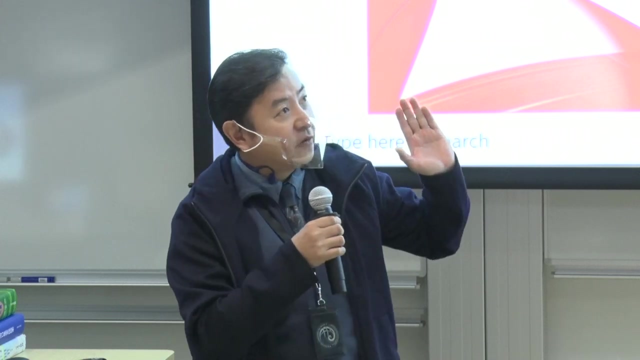 you know, Hong Kong has a fish biodiversity because of surrounding by the ocean and also the northern part of Shenzhen River, And we have both freshwater fishes and also the all the marine fishes, And also in the western part of Hong Kong. 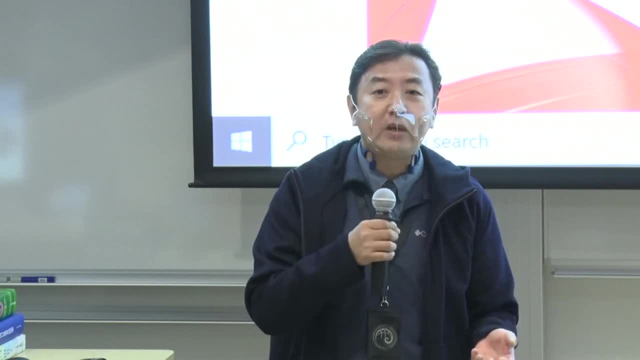 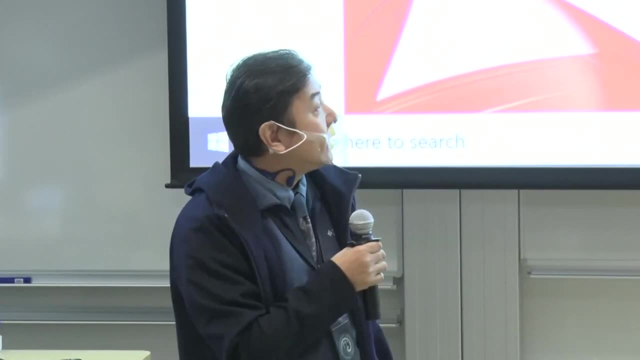 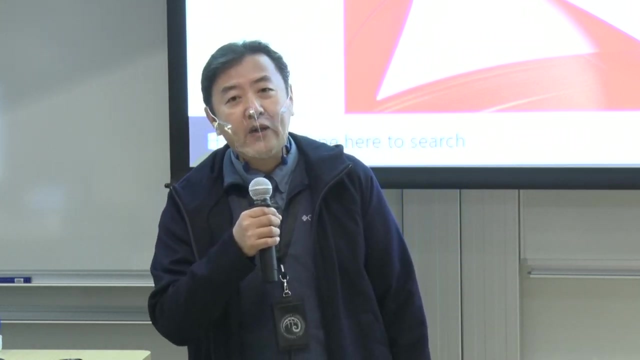 we are facing. we have: we have a Pearl River- It's an international grade of big river opening in our western part And then affecting Hong Kong a lot- and then we have a lot of lot of fishes and biodiversity and also the environmental heterogeneity. 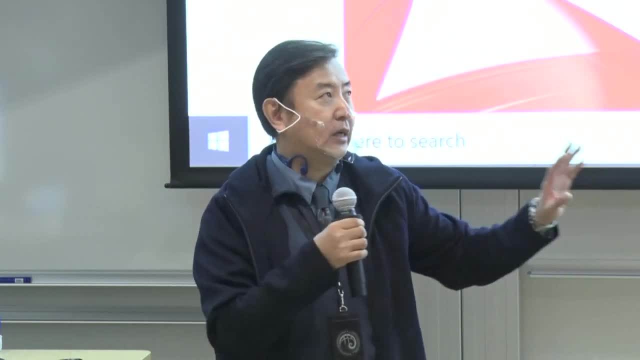 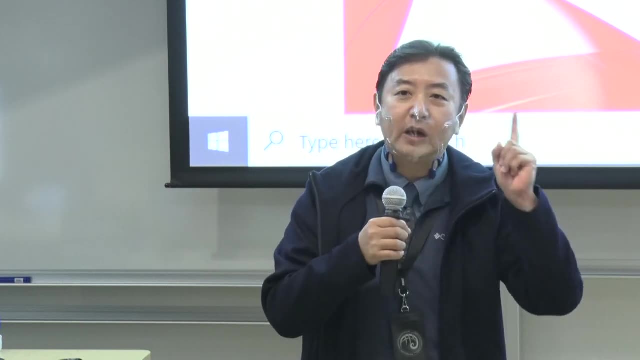 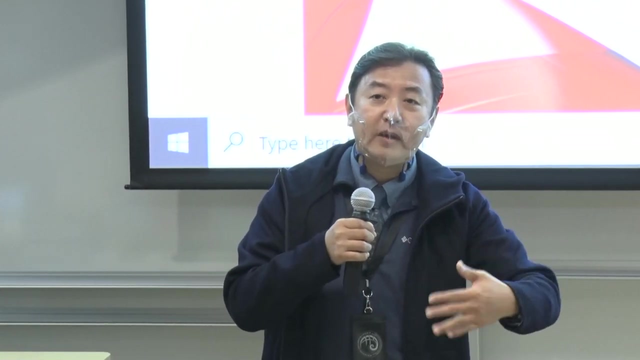 It's different from western to to eastern. All the environment are are gradually changing. It's not the, it's not one kind. So we are not in the middle of the ocean And also we also have have located in the. 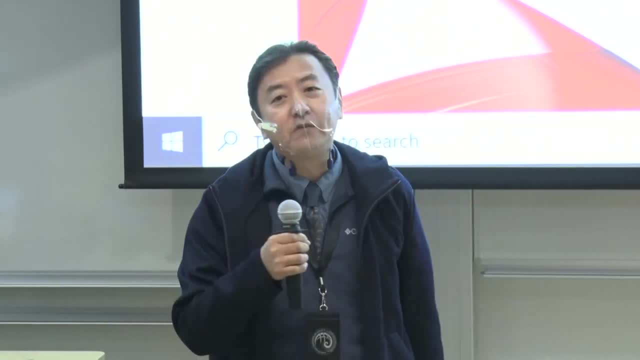 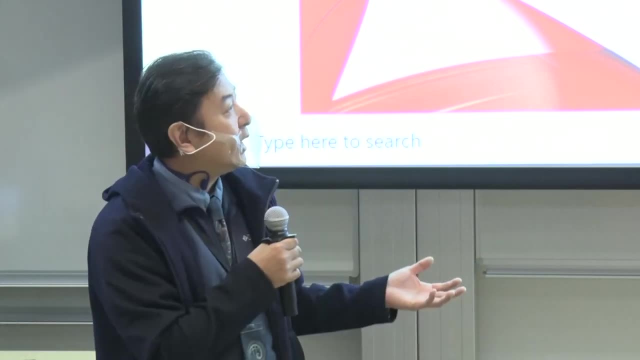 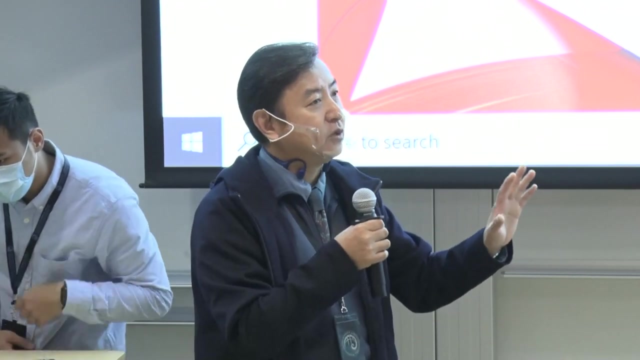 in the southern part of margin of the south, southern China. So we have ocean, we have, we have rivers, rivers, and also we have from asteroid to to transitional to the, to the oceanic environment, from western to eastern. 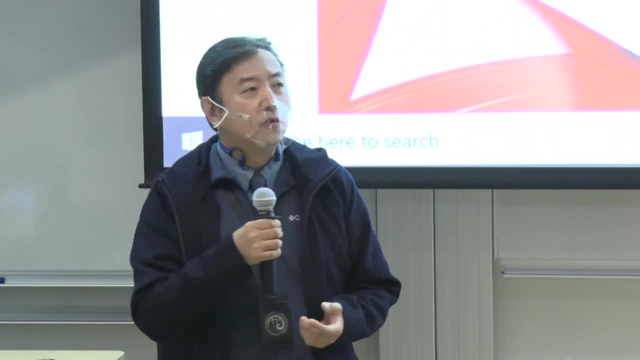 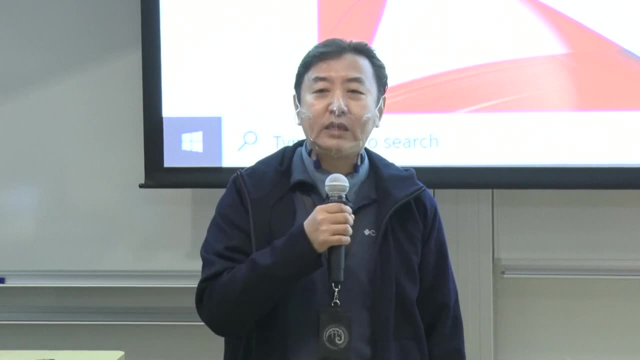 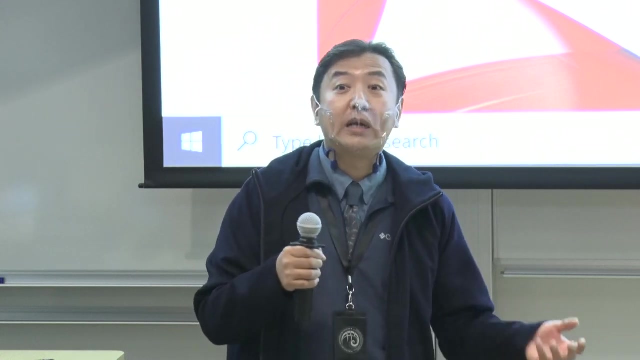 It's very complicated. So we have. we have about a thousand species we recorded. And also this arrangement is not easy because I'm a taxonomist and I'm very classic type of taxonomist It's I'm 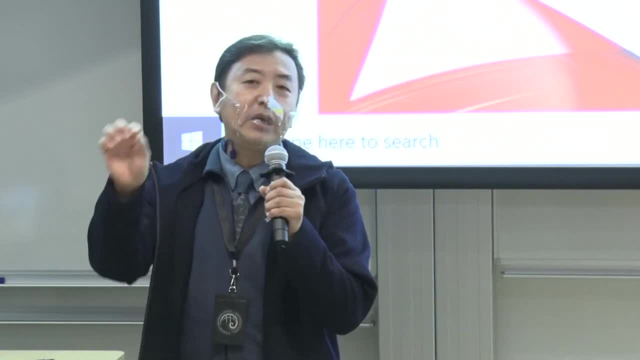 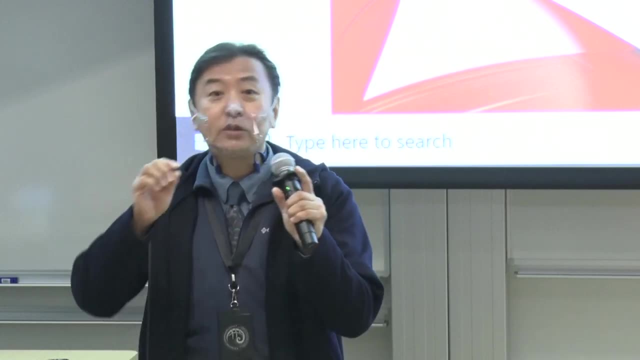 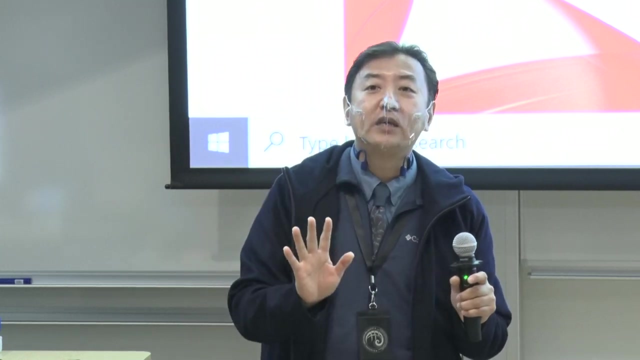 doing the, the taxonomy, with the, with the characteristic morphological characteristics, the outlooking and also spines and scales, and just to identifying fishes, So not using the genetics. So we found that many, many fishes has to be combined with the names. 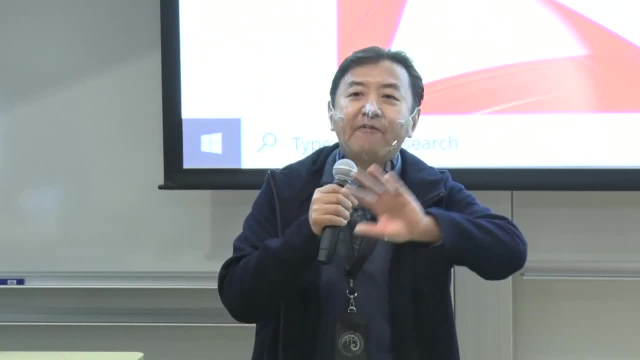 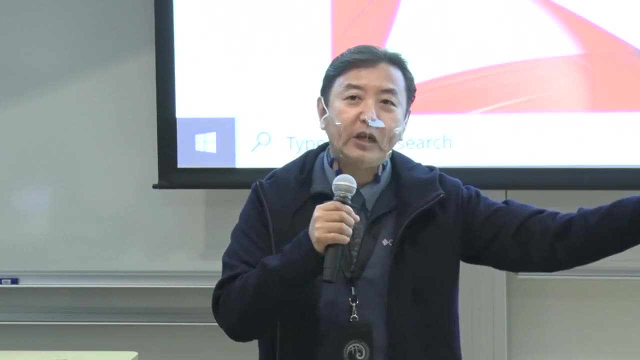 because you know, we, we have synonyms: The same fish, that same kind of fish that found in different kind of locations around the world, and then we have to combine the name and then we, we replace it with the oldest. 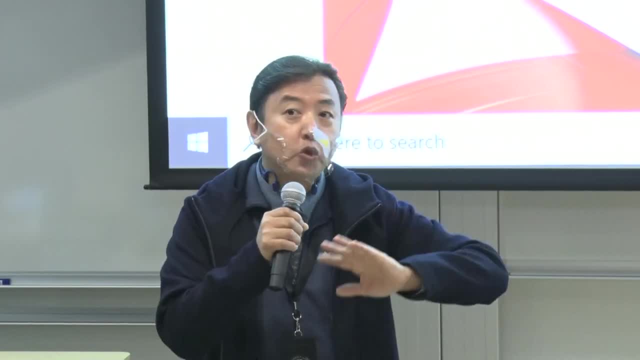 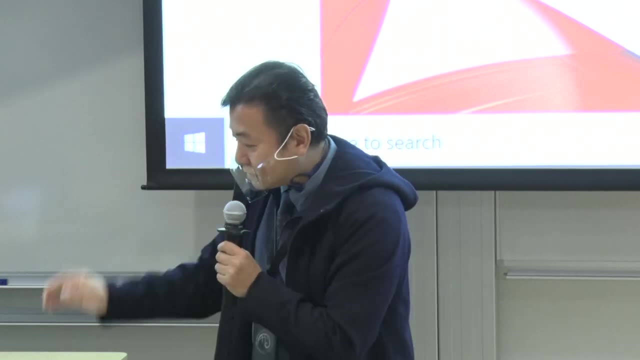 We, we called it senior synonym, And then junior synonyms are the after and then the, the newer, And then we, we have to replace all. So this is the brief introduction that I, I I've done. 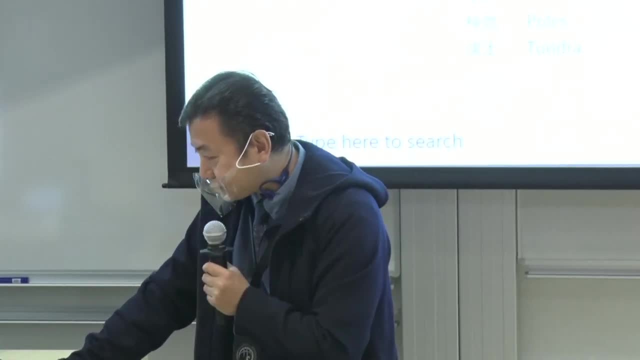 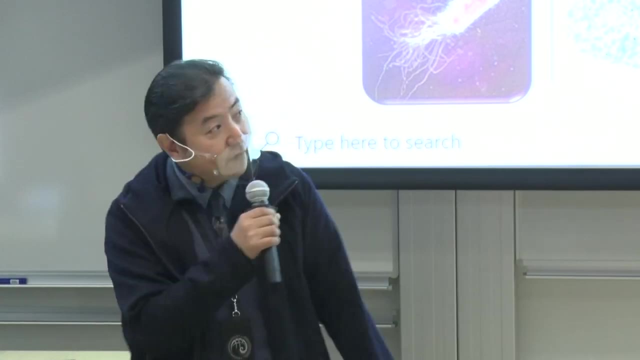 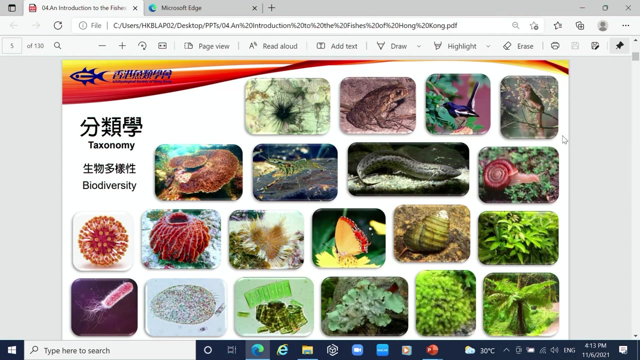 in the in the previous several decades. Okay, Okay, We we going going forward And we have biodiversity and from the, from viruses, and then to to very complicated the vertebrates in the. 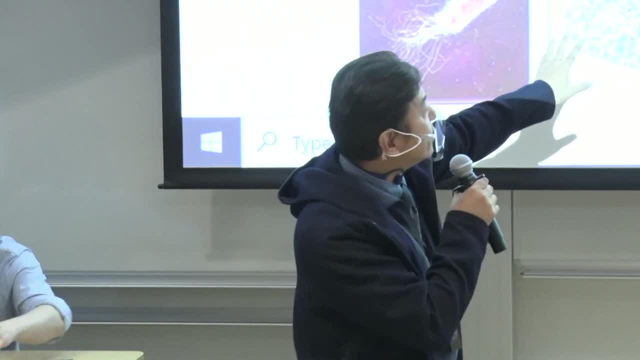 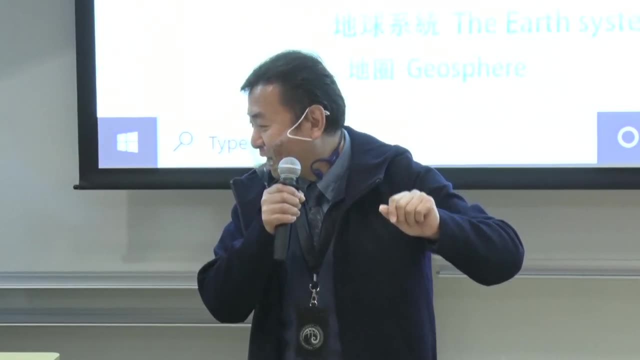 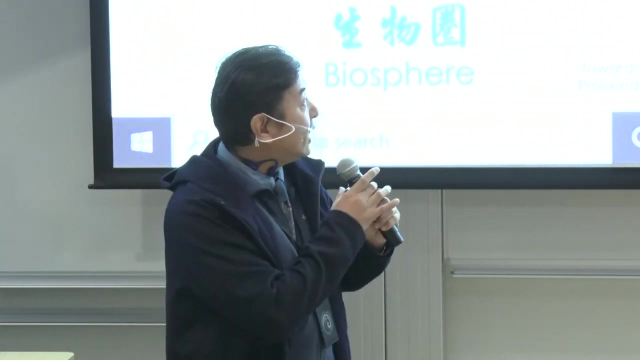 this kind this, this kind of distribution, And you see some, some oh, That's okay, okay, okay. So, yeah, Yeah, And we, we have a lot of changes in this decade Cause. 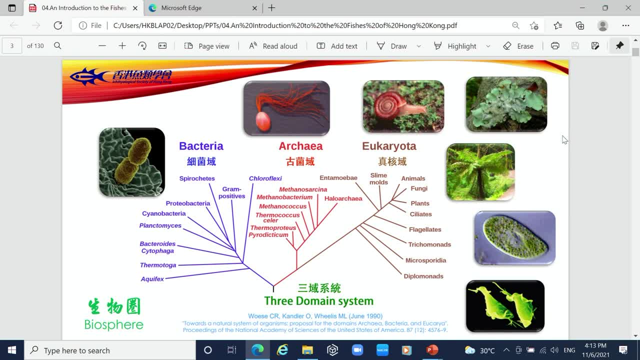 we have the technology on genetics, Cause it differs from from from mine, the, the classic classification. You know, we, we, we are using the morphological characteristic, But the newest is engaged in. 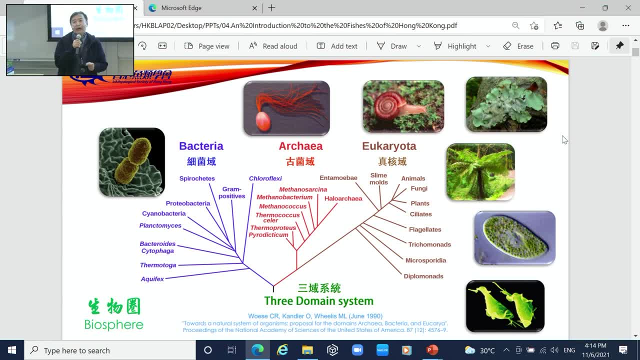 the, the, the. it's about DNA. So we have totally we obtained a very different tree of life. You know that. you know the in evolution from very simple form. 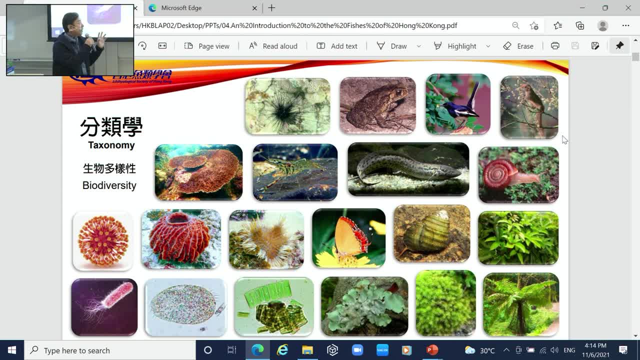 to complicated form. there's a evolution, And then we have a tree of life like a tree, And then they, they are evolving into different kinds of in habitats and then selected, And then we. 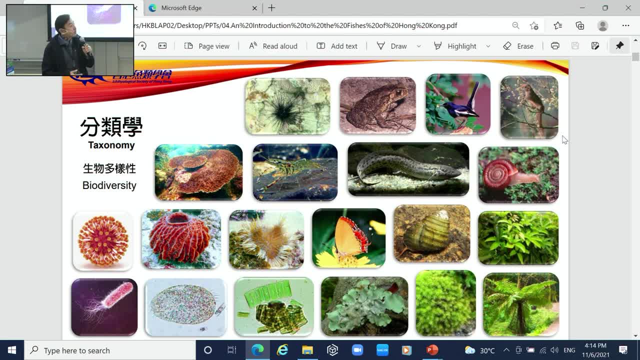 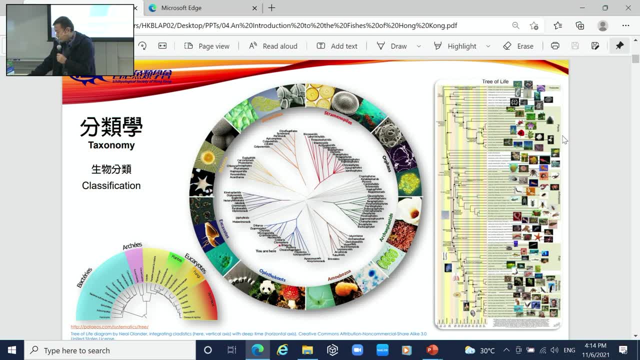 they, they are changing shapes and also the structure and also function of the body. And then we have- we have a lot of, lots of life forms And okay, and the taxonomy is becomes. 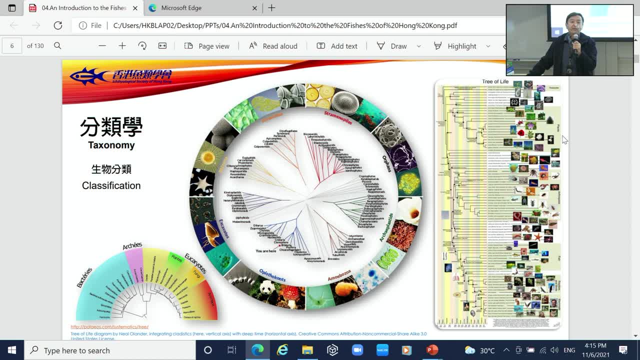 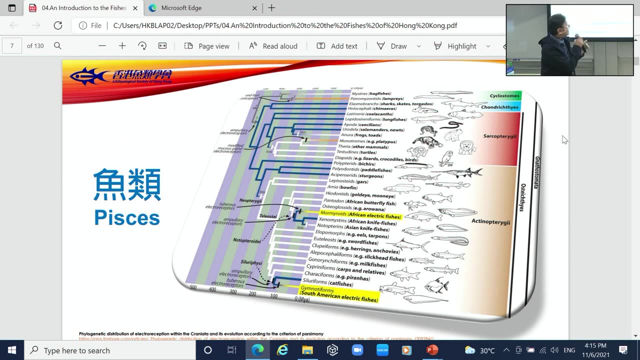 much more diverse, And then also we maybe for students that you have to do it in in a very high tech, And then the- the fish is also the same, And then 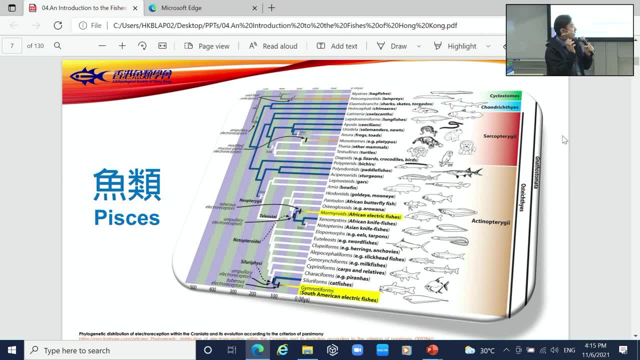 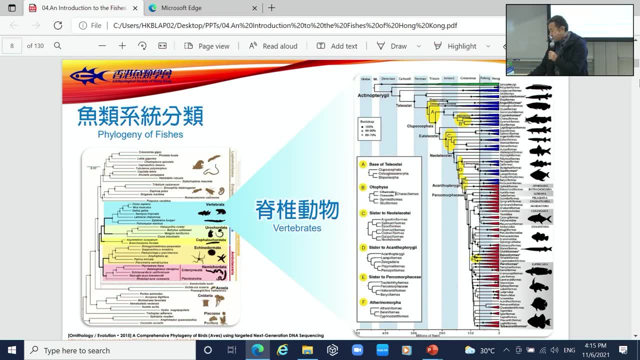 we, we have to, we have to adapt into the this kind of molecular classification And then changing. This is fish There are, this is the all kind of living organisms, And then just this part. 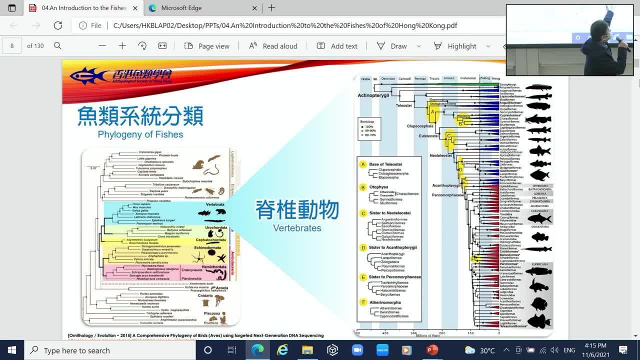 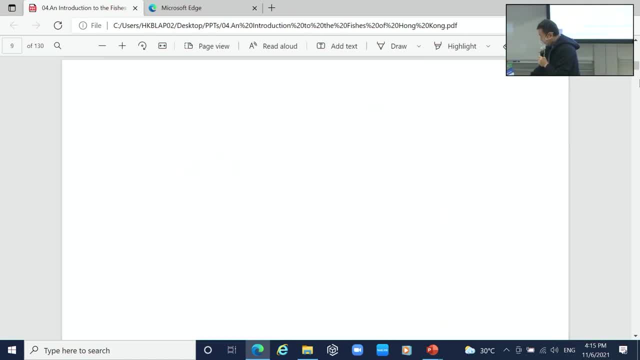 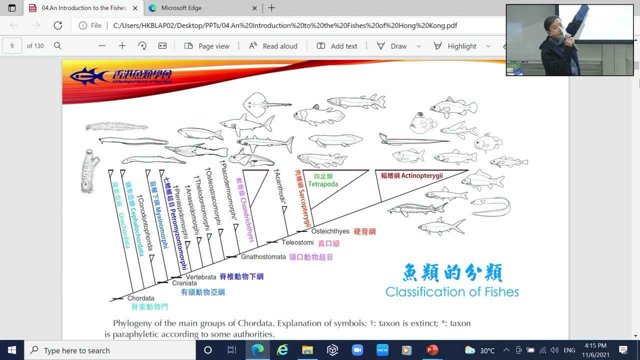 is a vertebrate And then this part vertebrates- We, we are still living in the water- is fishes. Okay, So we're talking about fish still, And from very different form, is primitive form. 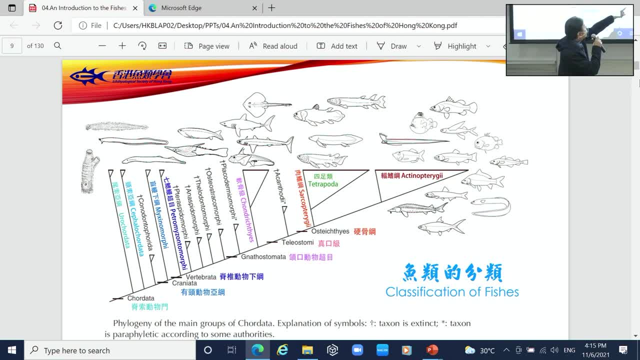 of fish, And then to the most advanced, And also here you see, this is tetrapod. Tetrapod it's go up to the, to the, to the land, And then there are all. 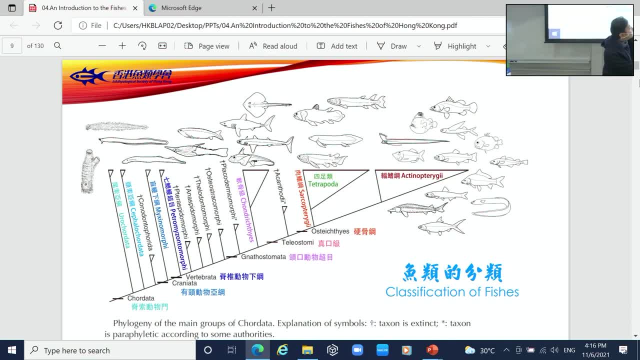 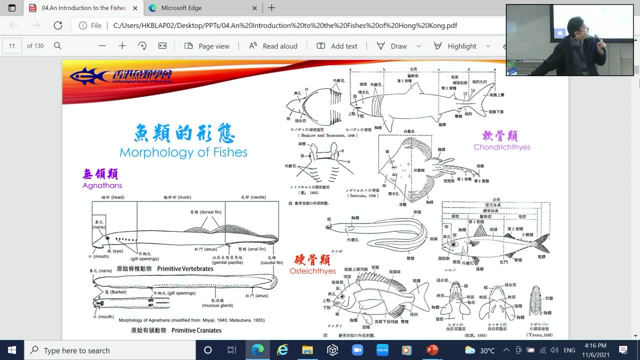 limbs. So that says the we're talking about fish, And that that's also talking about the, the fishes found in Hong Kong. The groups is here And then we use the, these kind of. 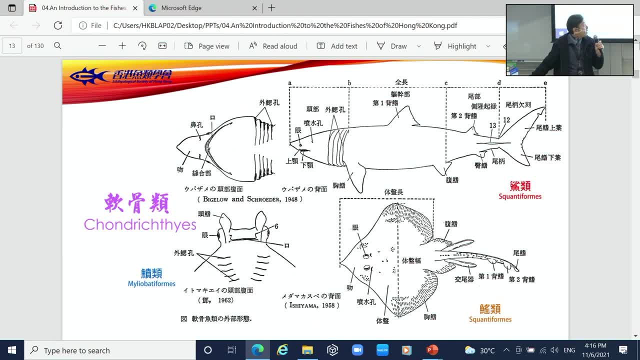 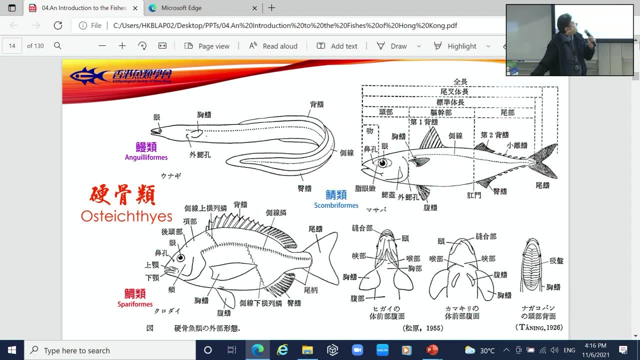 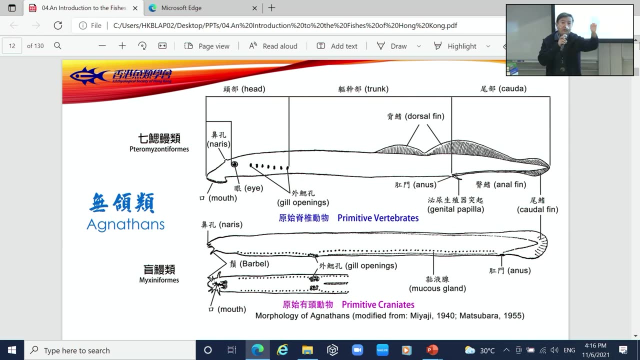 characteristics. and then we identified fish in Hong Kong: Okay, Sharks, And also the bony fishes. So cartilaginous fishes, bony fishes, And that's the. This is the most primitive one. It's without jaw, It's jawless fish, It's not existing in Hong Kong because it's quite northern. 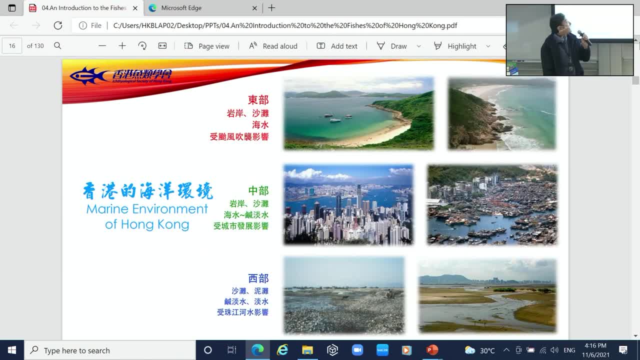 Okay, so go on and talk about the. Let's talk about the marine environment of Hong Kong. This is very simple form that I can introduce. in the eastern part, there's a rocky shore, a sandy shore and affected by the typhoon, and, And in the middle we found that we are occupied by human and then the polluted and also metallized. 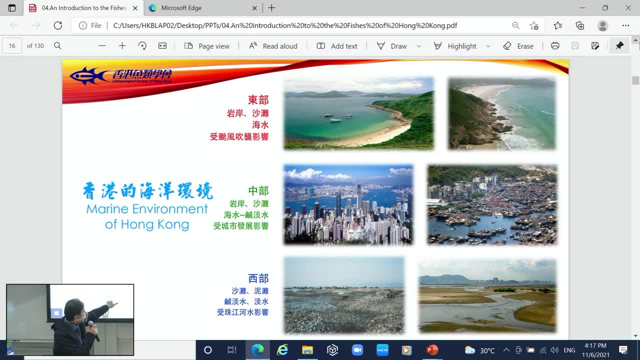 and and it's at the, at the western part there's there are. so you know, because we are affected by the Pearl River. so it is muddy and In and it's yellowish water and then full of muds and also very highly nude with high in nutrients. 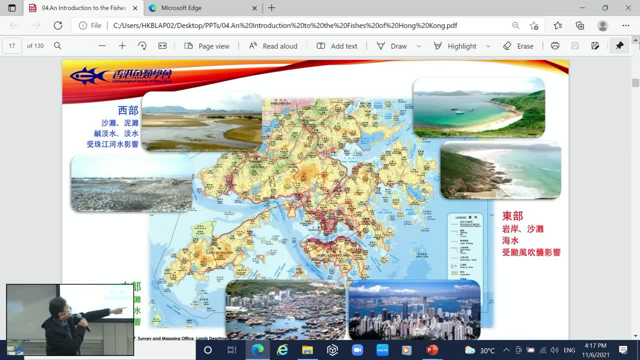 So look at this, This is the distribution of Hong Kong. just look like if they're very simple form. and then those fishes in the water from Western to to north to Eastern, that in different environment. we have a serious series of gradual changes in different kind of fishes. Okay, let's look into it and 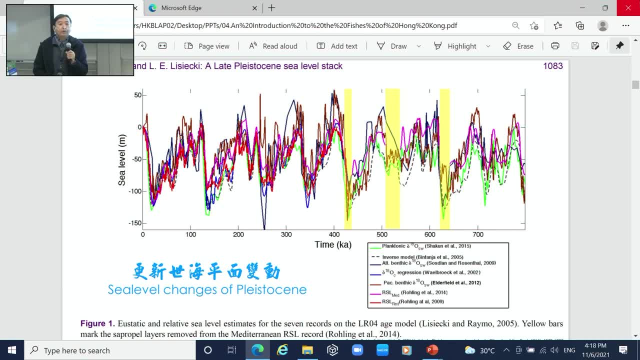 And also I also have to have to talk about the, Because this is the background of Hong Kong that I have to face. This is the sea level, changes of place, a plastic scene. It's talking about the 40,000 years to to 10,000 years ago that there's a very, very severe. 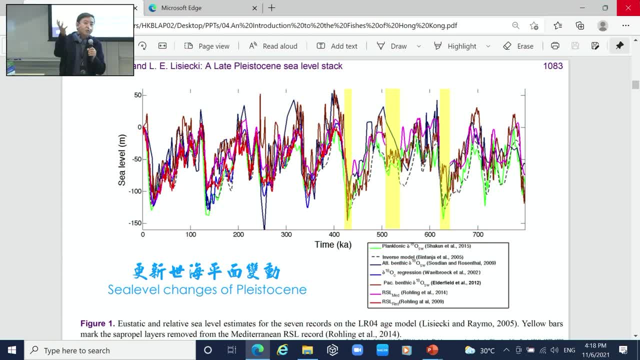 Sea. sea level changes because when the earth is becomes, becomes an ice form, and that it the The ice will remain on the land but not into the sea. So the sea level changes will become. sea level will go lower and then up to 150 meters below. Now, so it's so, it's not. 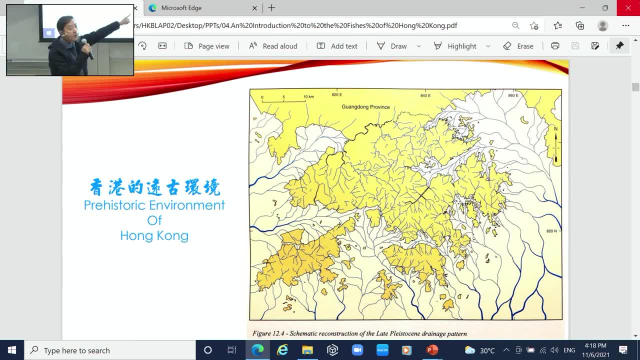 Not so, not so difficult to understand, that Hong Kong becomes a totally land. so What I'm talking about, what I'm telling, trying to talk is to tell you- is the Hong Kong marine fish and Hong- They are secondarily invaded Hong Kong's water. So this is very important, So so that the environments are always changing. 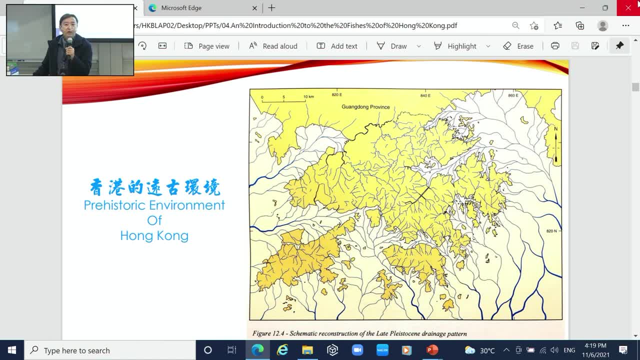 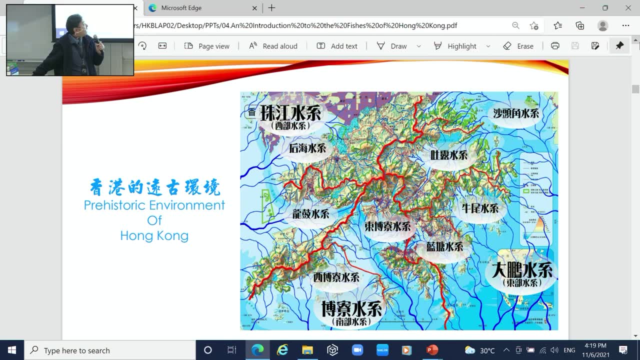 It's not, it's not, it's not always in in very steady and stable. So, okay, This is. this is my freshwater fish analysis. so they, the orange part is the, is the the water, dividing that water device of Amount, the amount of regions, and then we'll even the freshwater fish, it divided into this kind of system. 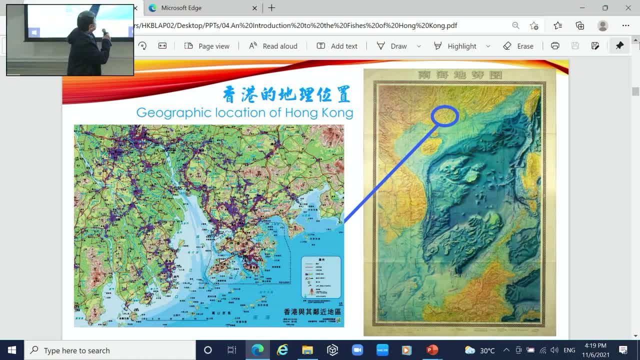 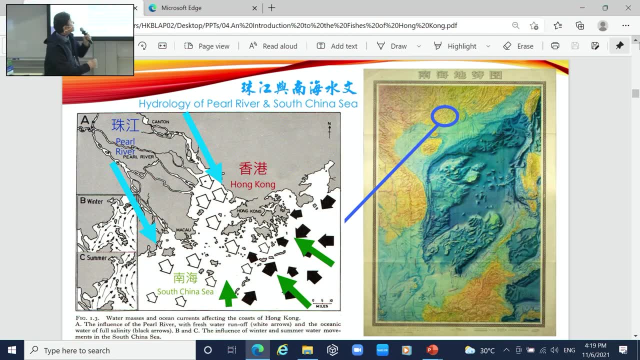 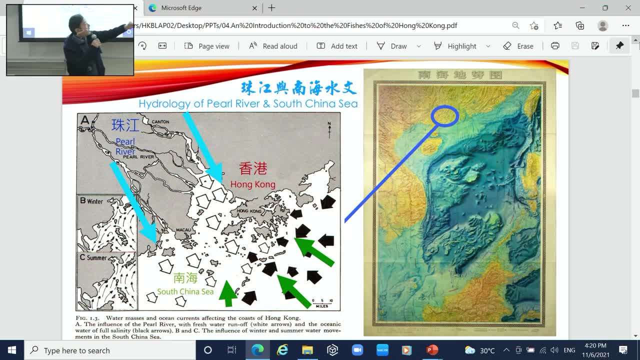 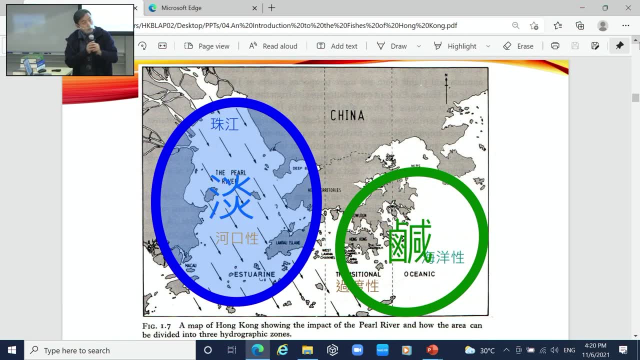 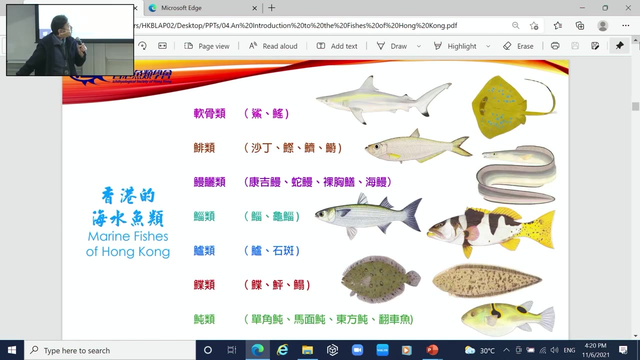 freshwater and and the marine water is just like this and So Okay, So this is freshwater and This is salty. It's very clear. So the GoPro, This is the glaube. So different kind of fishes, So different kind of fishes will invade different type of 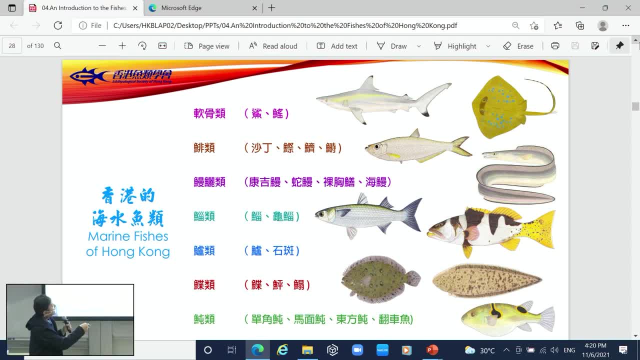 environments in Hong Kong and just like these are. Is there any pointer? Sorry? So The mullets grouppers and also the bottom surface fishes, just like flatfishes, and also the pufferfish, These are all very popular in Hong Kong. 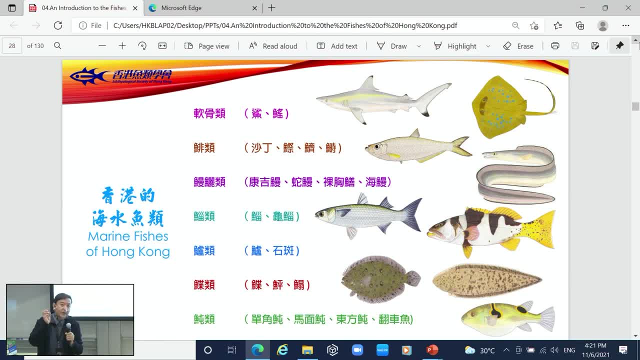 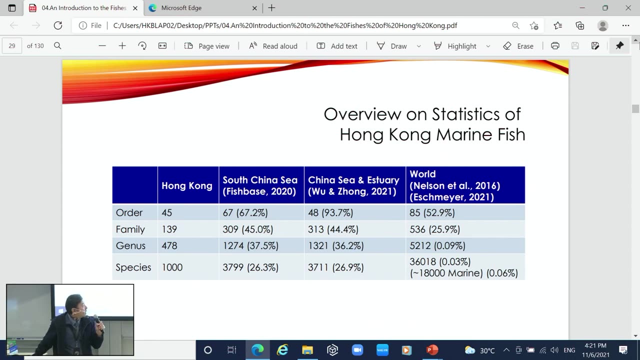 And they live on different kind of, based on different kind of foods, And then their foods are divided in two different kinds: One is plantonic, one is the banthus. So because of this we calculated, in Hong Kong there are 45 orders and 135 families. 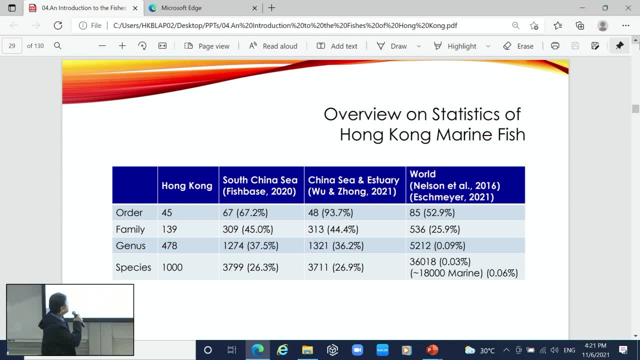 and then genus: 478 genus and species in about 1,000.. And so in South China Sea we previously recorded this: 67, 309, and 1,000.. 1,274, and so we see, totally for the world will be 50%. 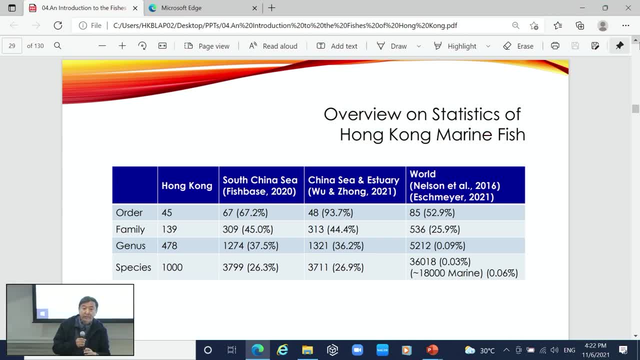 of the orders existing in Hong Kong is great. The biodiversity is unbelievable. So about family? it reduces, but still have a one-fourth family existing in Hong Kong, genus, so 0.09.. And so we have about 1,000.. 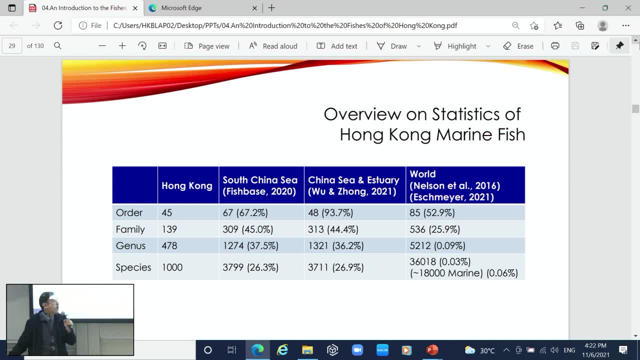 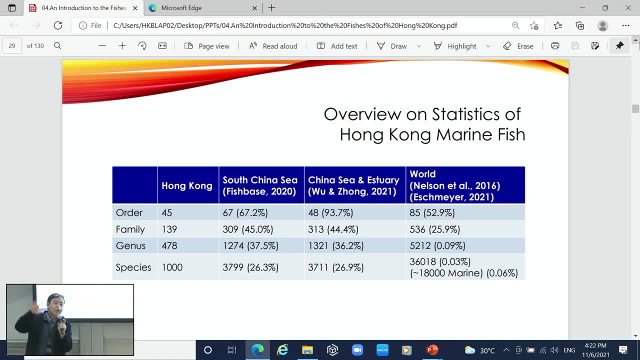 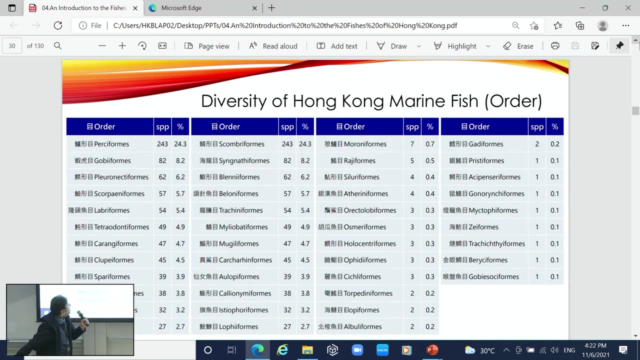 we are classifying to order and family. This is a classification. This is talking about the closer relationship. So the representative of order is about 50%- is very, very important. So many representative fishes around the world- world. is it existing in Hong Kong? okay, this is diversity of 30. it's about the 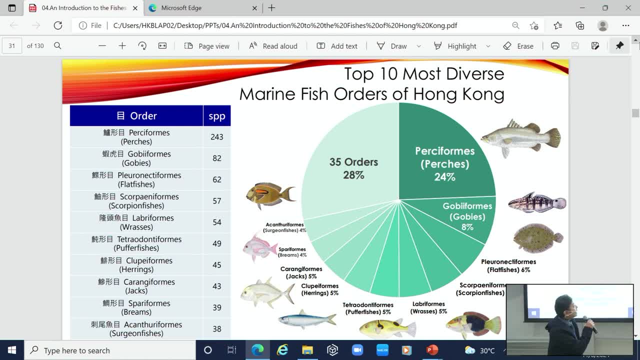 order, and also it's not not so difficult to understand the purge: a purposeful, that that's just like sea bream, and another, this is a, the purge, it's just like butterfly fish, and so so for that, all included. and the second is goby forms. it's my, one of my target office of the of the group of fish, that doing. 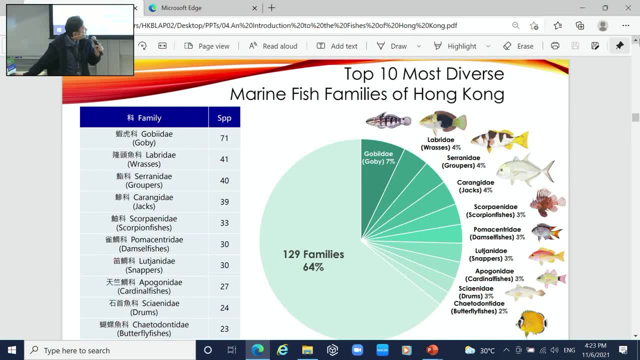 doing studies and okay, so we are because of the, because of we are located in the estuary, so goby goby's it's dominated in in Hong Kong. it's a. it's highly diverse in muddy and also rocky, and also the also the coral reefs. 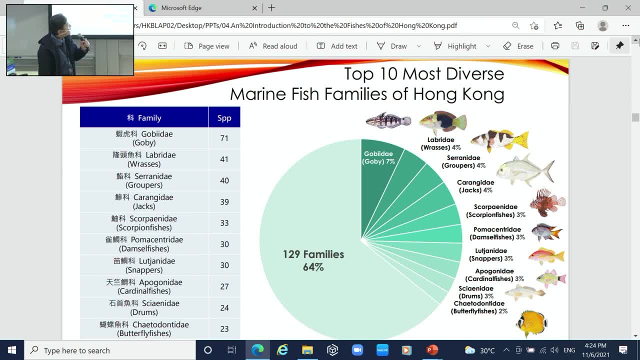 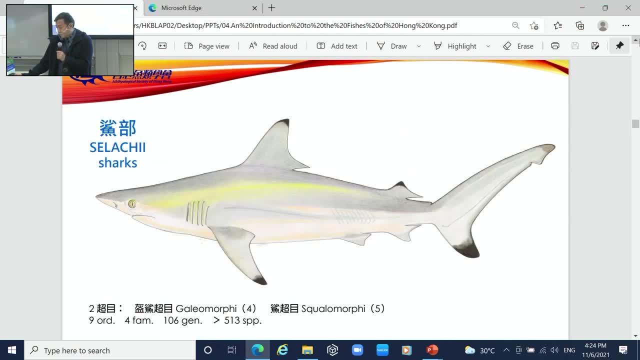 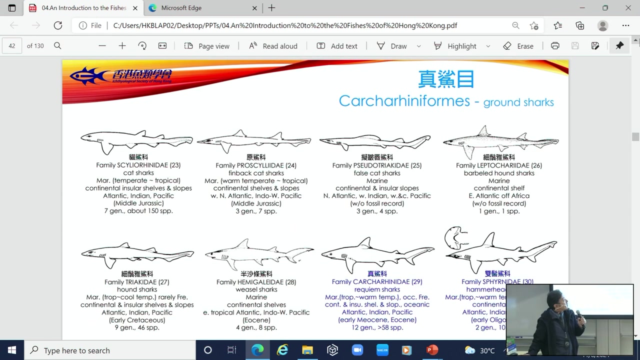 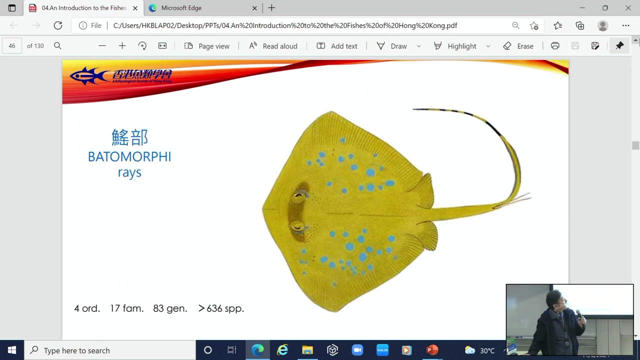 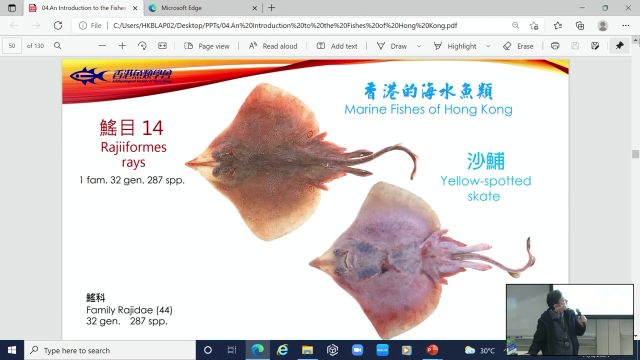 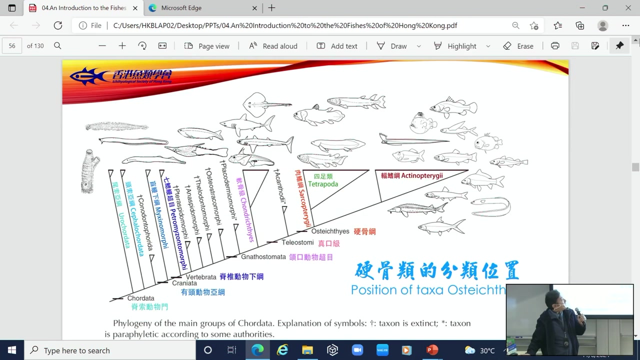 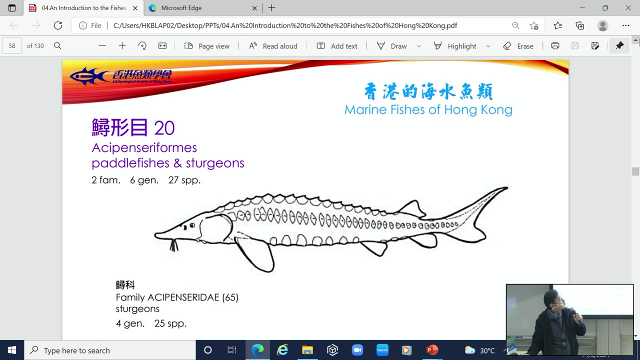 and then it has a occupies a seven, seven, about the seven percent of the family. okay, so, just okay, just look at- I think better to look at the the pictures: sharks in Hong Kong gi to sea and rays as electric race and they saw this bottom service and the Boni fishes as sturgeon. these, this, these penetrates. 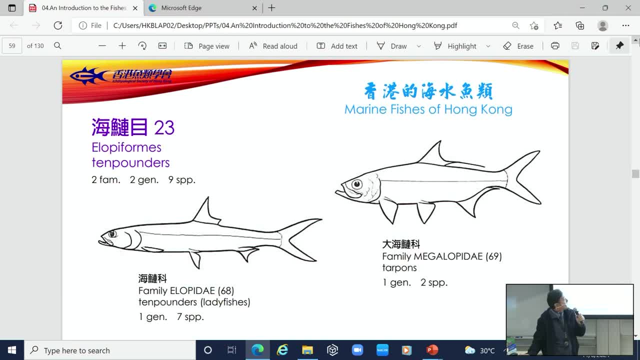 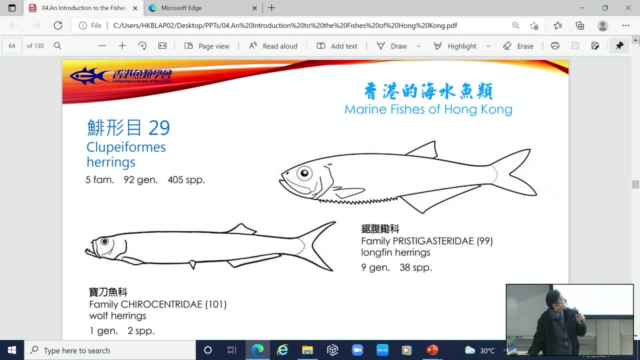 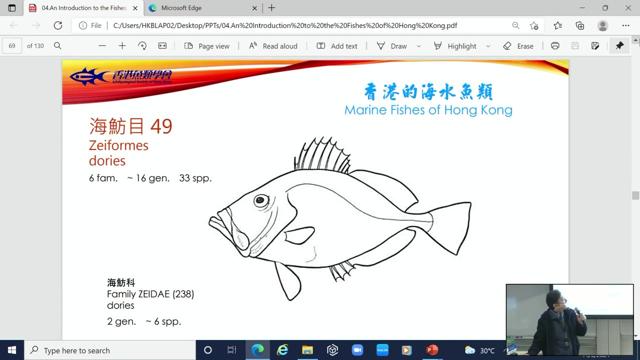 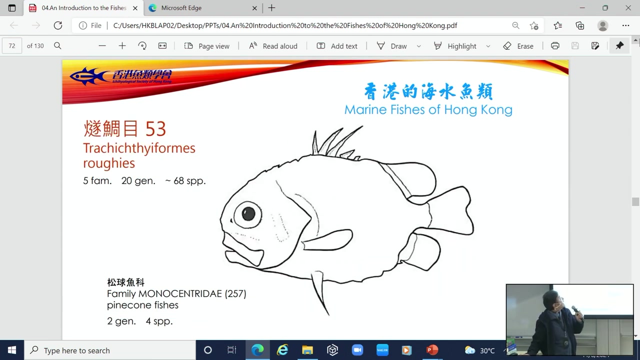 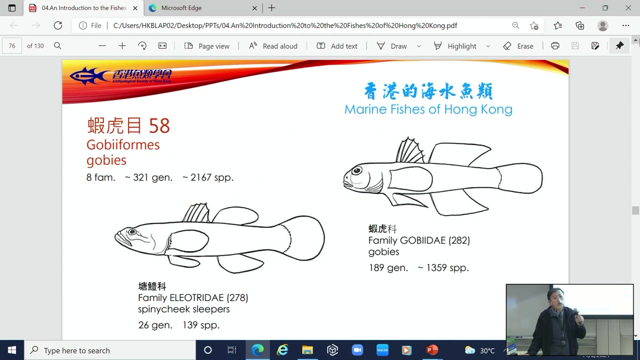 sea, Pearl River, and also herrings, eels different kinds, and also the herrings and catfish and cots and squirrel fishes. I think it's too many species, so I would like you to have a look today. it's huge. 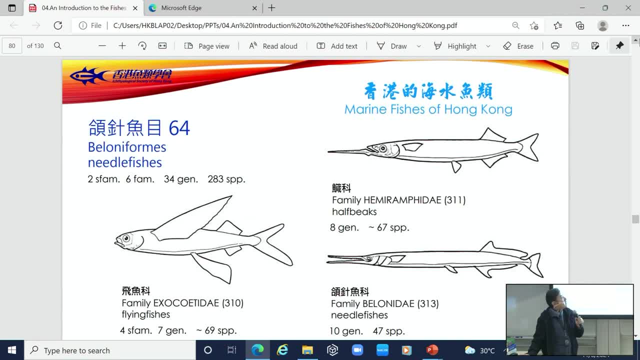 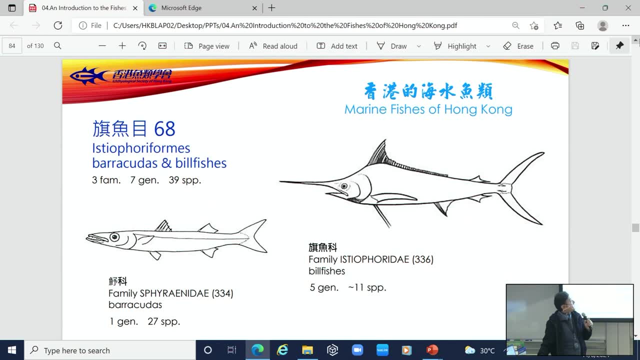 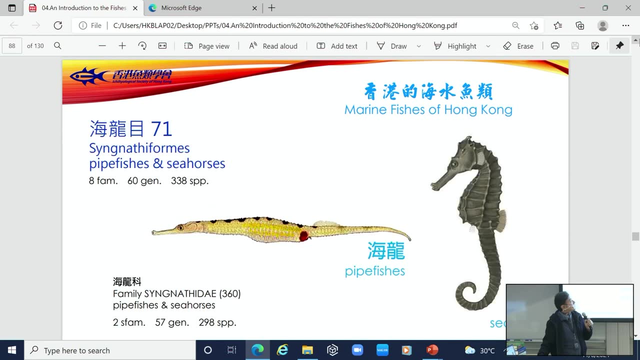 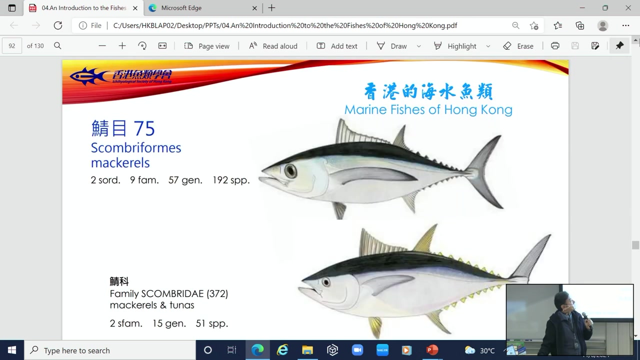 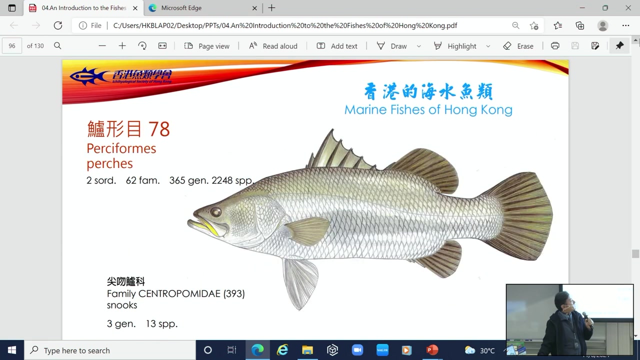 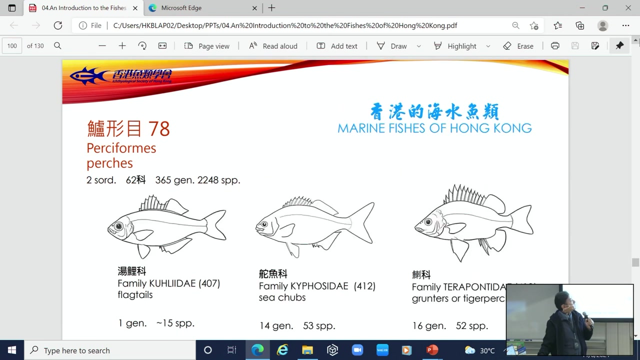 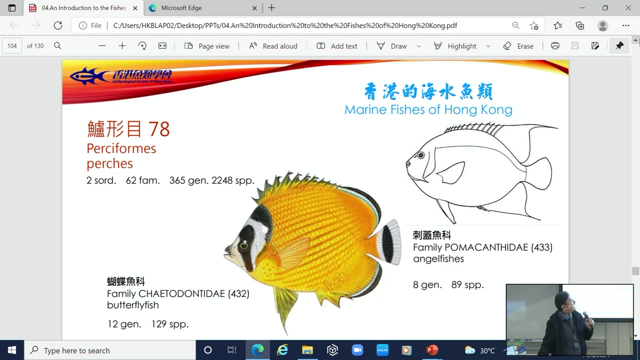 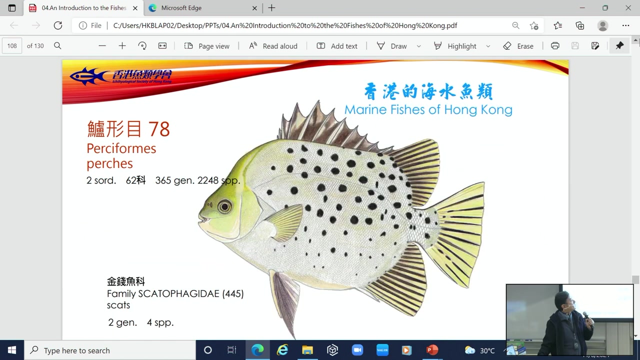 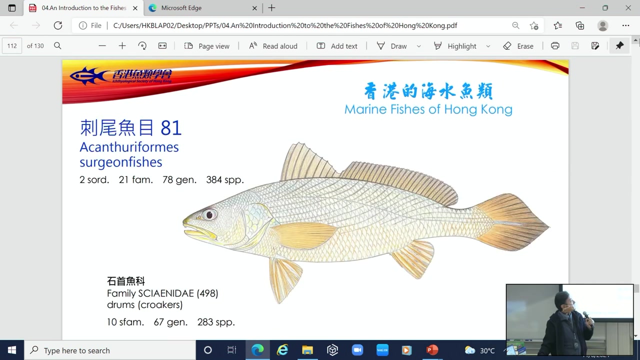 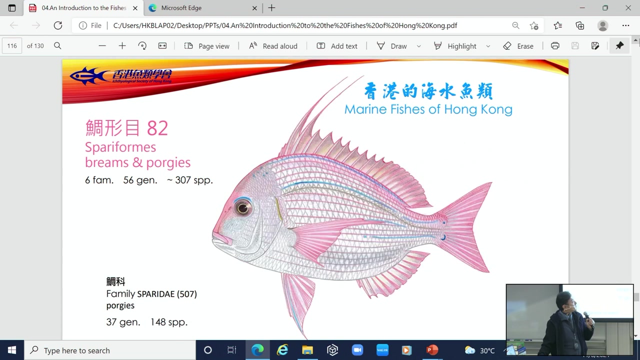 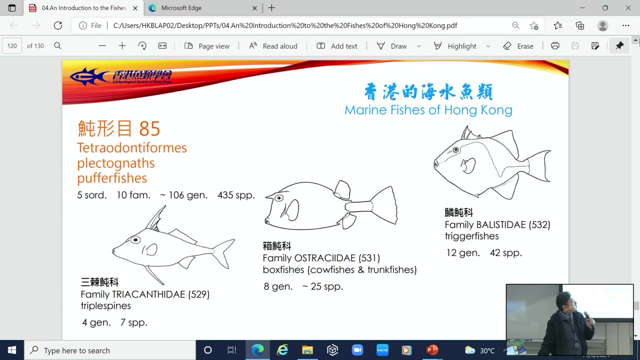 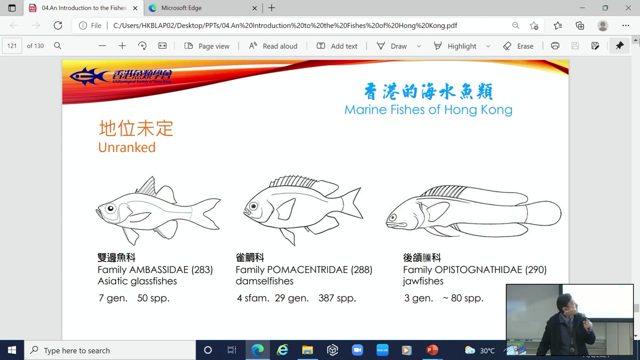 So these are what we found in Hong Kong. Some are very familiar, but maybe some are very rare, but still counted Okay. So it's very easy to understand that there are so many. there are many type and shape of fishes. Then the 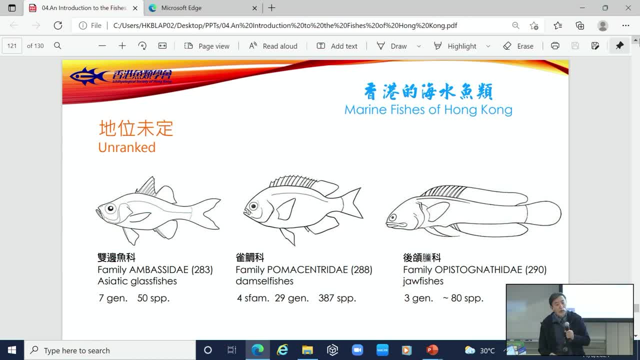 It's, It's, If you look at it, you know they are all very rare: Seven species of fish. they are all very rare and that's the point. So now we have a very large, you know, one species that we are very curious about and 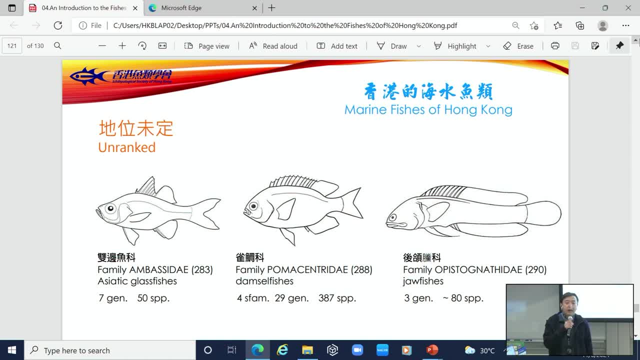 for us one species we only can not find. So this is how we would place it in Hong Kong: Okay, Okay. So what I am going to do is we are going to put it in Hong Kong, so it will be it. 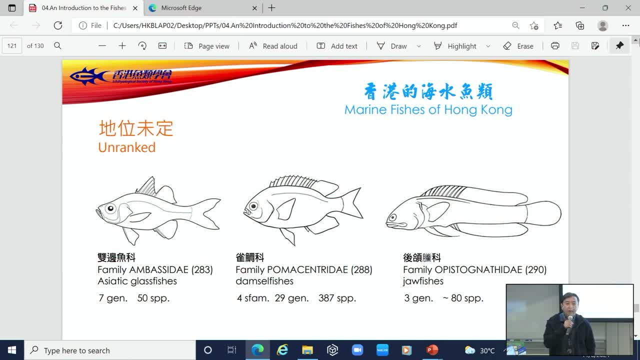 will be found in Hong Kong, So we have to protect it. and then someone that asked about the: oh, we have several marine parks in Hong Kong. Where should we place they are coming? And I answered: Hong Kong is such a small place and I would like to have a whole place. 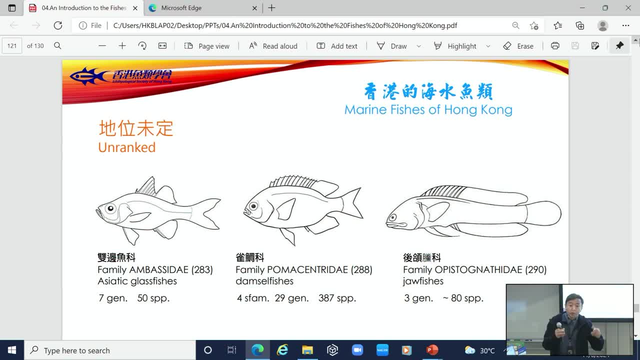 for the, For the, For Hong Kong to become a, A small marine park, because this is itself is very the environment and all the fishes are very diverse, and then we have to protect, and then it's not only talking about the bank drawing or something. 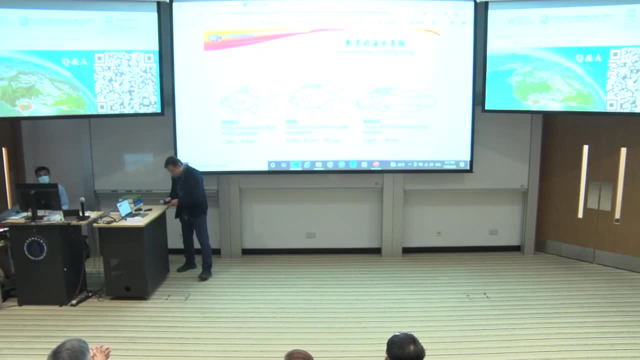 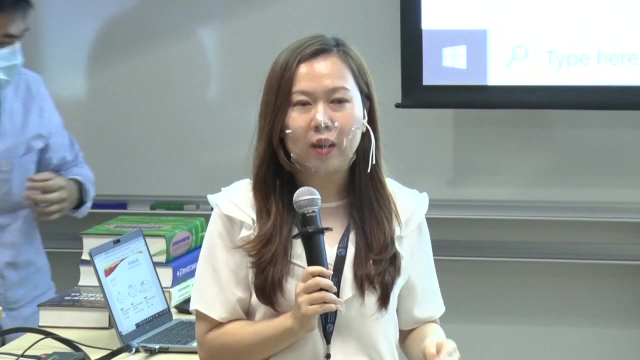 yeah, thank you. Thank you. thank you, Professor Chong. Actually, other than our on-site participants, today, there are a lot of- about a hundred- of online audience. they join our forums today. so any of you, if you would like to ask Professor Chong or other speakers for. 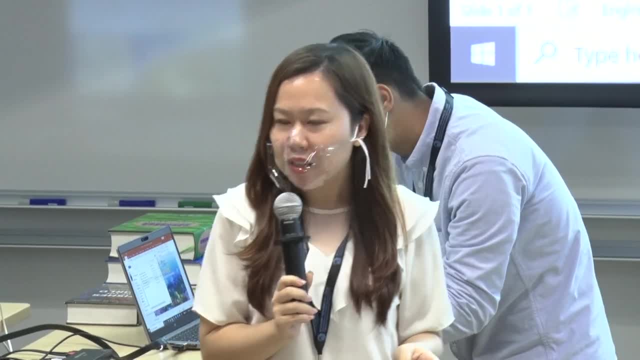 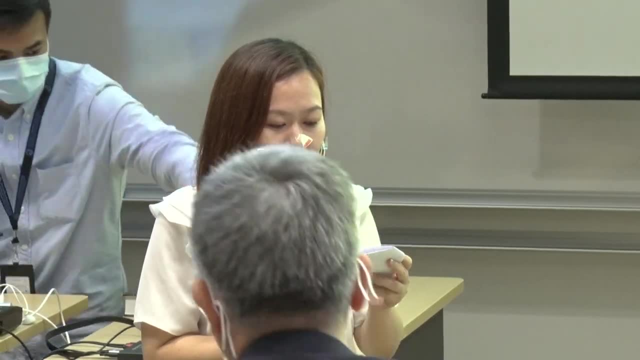 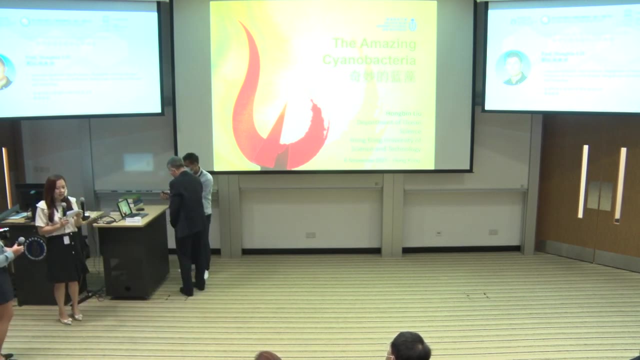 some questions. please scan the QR code again and enter your question, and we will deal with it during the panel discussion part. so, moving right along, may I now invite another guest speaker, Professor Liu Hongbin, Associate Head and Chair Professor of Department of Ocean Science. Professor. Professor of Division of Life Science. Hong Kong University of Science and Technology. 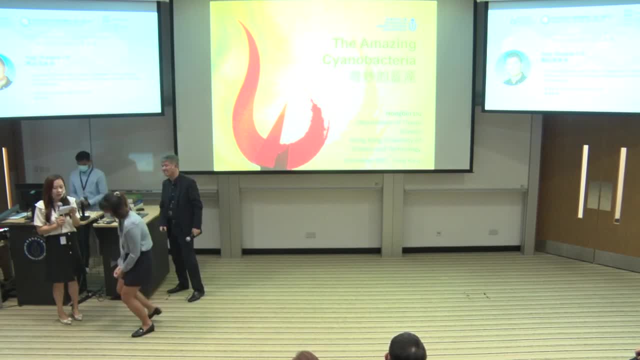 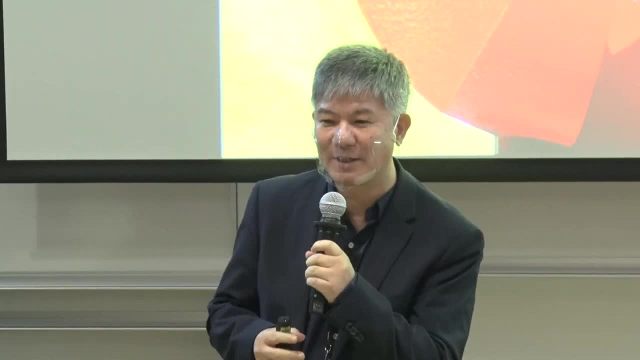 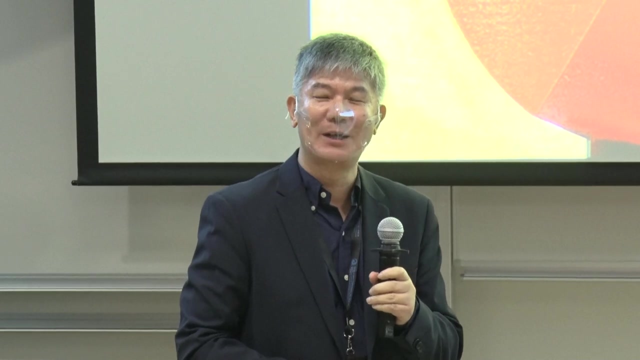 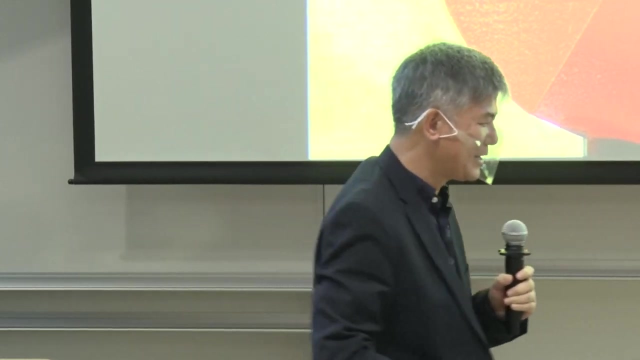 to share with us the amazingly high diversity of marine cyanobacteria. Welcome, Professor Liu. Good afternoon, Thank you for giving me this opportunity to introduce something really probably most of you don't know. as the previous speaker already said, it's pretty boring, maybe talking about 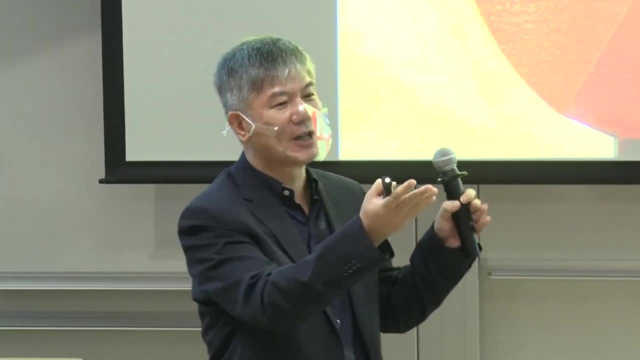 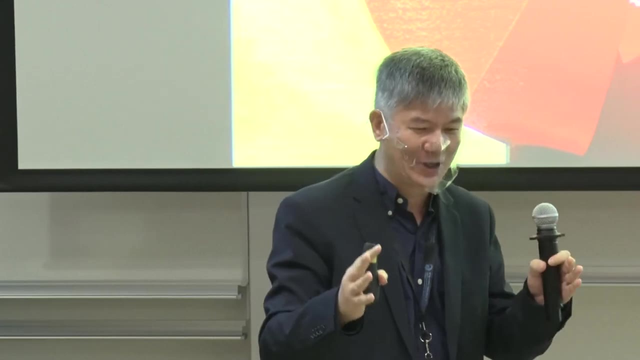 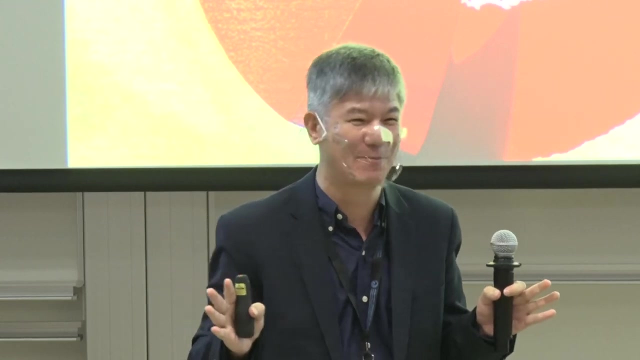 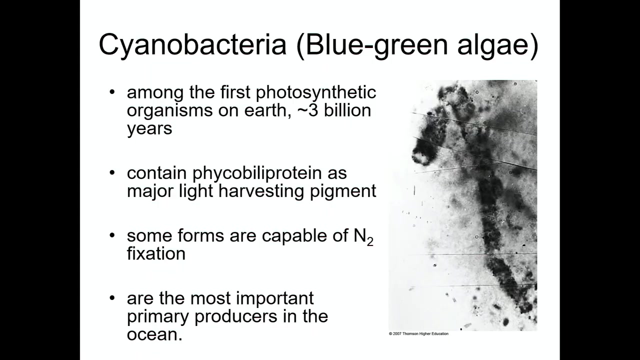 the, But still, when you talk about biodiversity now, we are often talking about whale turtle. What I'm going to talk is something invisible, it's microscopic, but they are very high, diverse, very high diversity. So, blue-green algae, cyanobacteria- although it's not algae usually called blue-green- 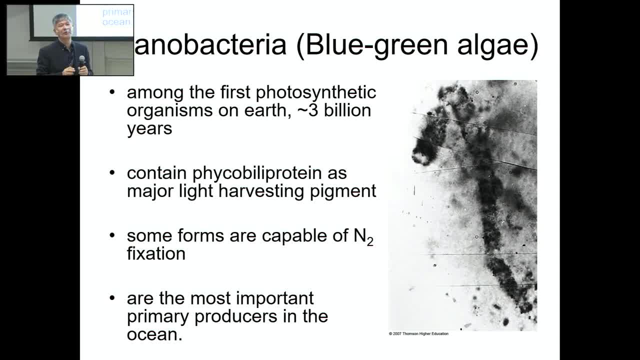 algae. it's the first photosynthetic organism on the earth. So this microfossil indicate that almost three billion years ago they are the first photosynthetic organisms. Because I prepared quite some slides, I may just skip each. I'm not going to talk very detail. 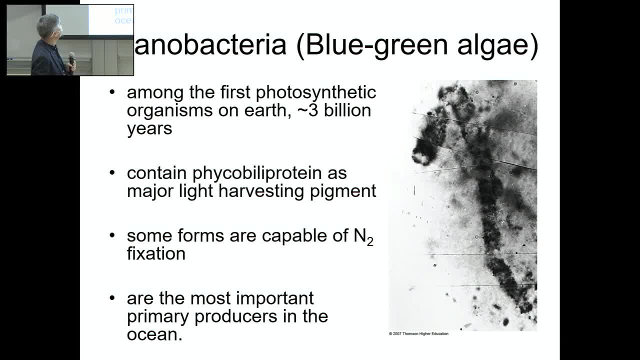 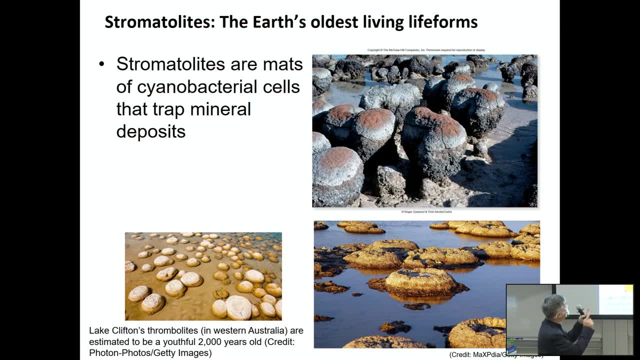 I just realized- I don't have enough time. And not only we have evidence from this microfossil, we do have some living fossil. So this is called stromatolites. This is a kind of a stone which is a cyanobacteria. 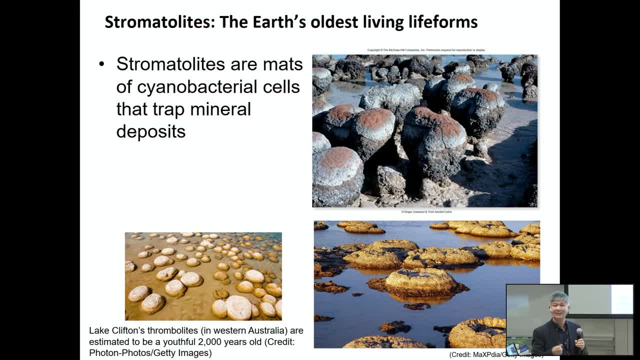 They are very, very old. The cyanobacteria- Okay, They the minerals precipitating, forming this kind of structure, And you can see this in Australia, some shallow lagoon, okay, And they are also very, very old. 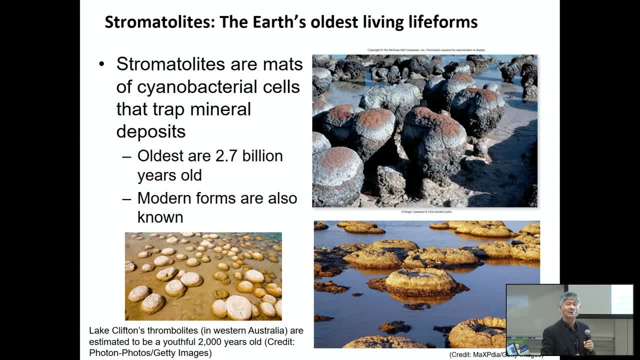 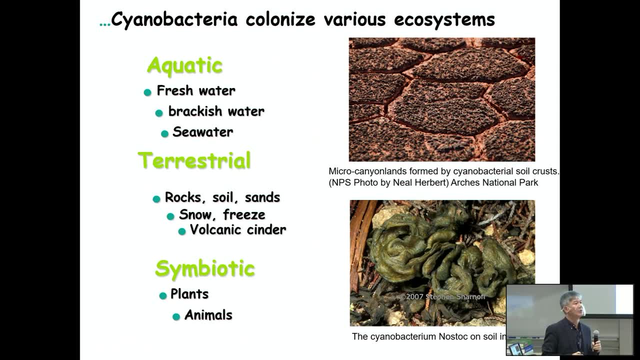 And some of them are relatively new, only a few thousand old, So it's still forming. And cyanobacteria can be found everywhere, okay, Everywhere, virtually everywhere. So they are in the freshwater, Marine water, They are in the soil, rocks, even desert, okay. 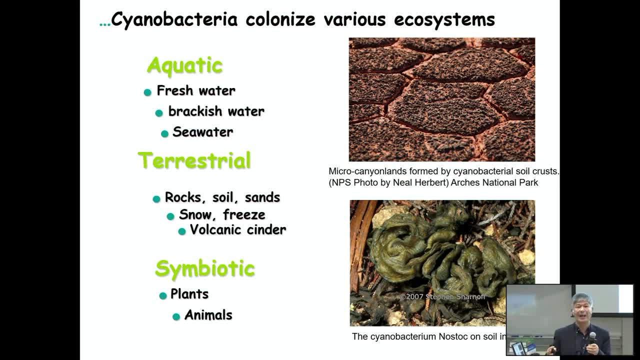 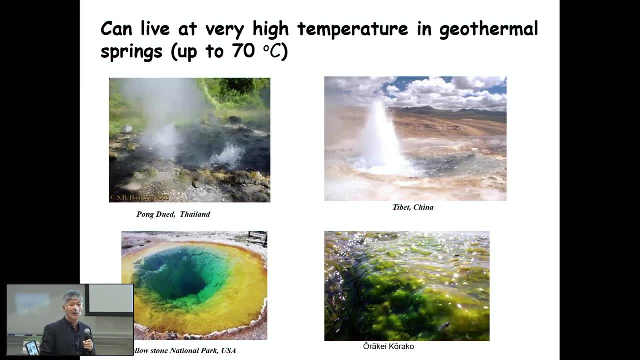 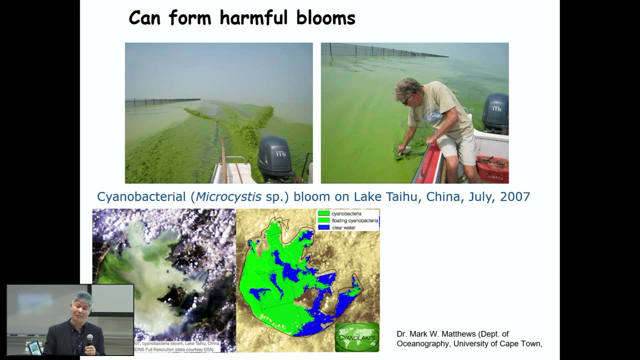 And they form symbiotic relationship with plants and animals. okay, So virtually everywhere. They can live in some extreme environment, For example in hot spring. okay, And they can form harmful bloom- This one in Taihu- okay, And it blooms everywhere. 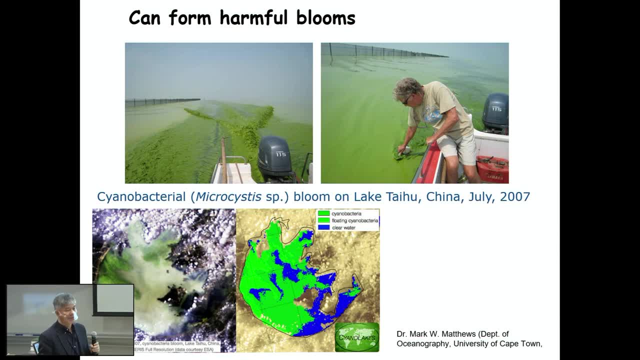 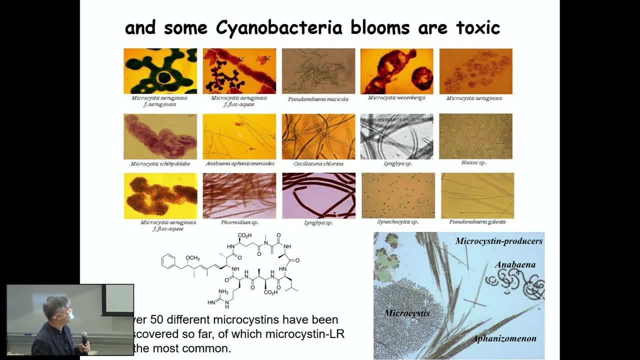 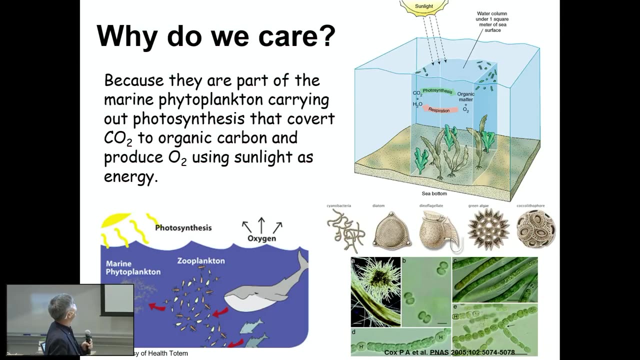 Okay, It blooms everywhere, every year, somewhere. okay, And lots of them are toxic, okay, So one of the most common one is microcystin, which is quite toxic. So why do we care? okay, We are all talking about climate change, global warming, okay. 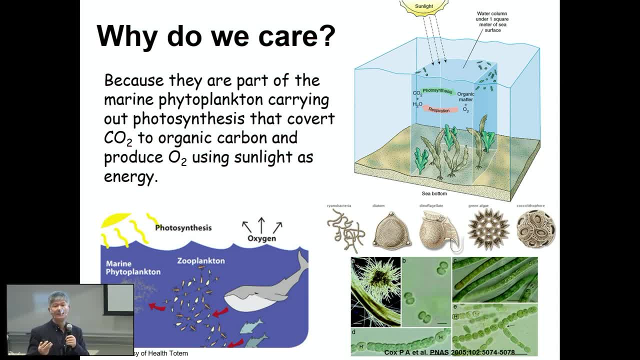 So, since they are photosynthetic organisms, Okay, They convert CO2 to organic carbon and produce oxygen. So why it's significant? okay, Because they are the base of the food chain And they supply all the energy- you know, all the high-level organisms- as the food for. 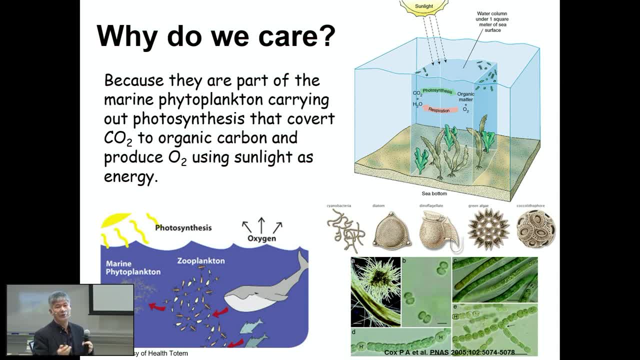 them. So we know that fishery, marine, all of them, Okay, Okay, And the ocean, provide lots of protein, especially for less developed countries. So they are very important. They are the base of the And, especially at this moment, we are talking about carbon cycle. 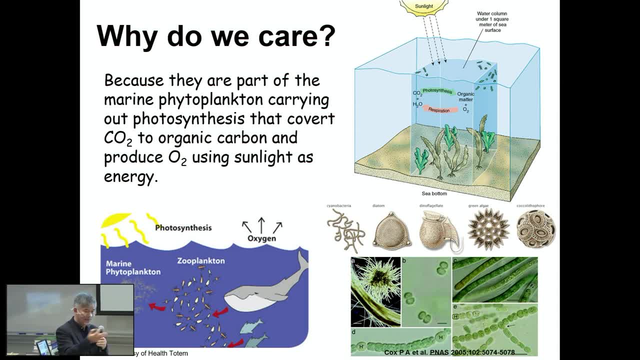 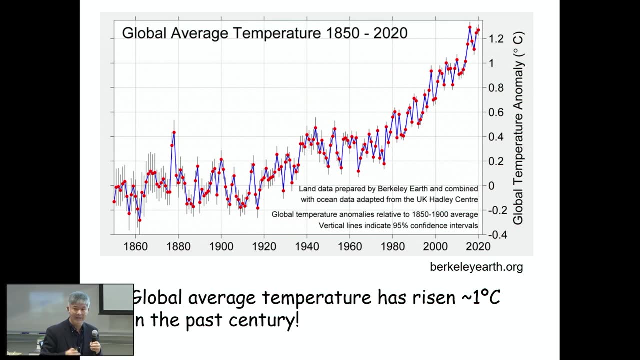 We are care of global change. you know, as many of us already heard, there's a summit taking place right now. Okay, So global warming is really an issue. You have been, You have been hearing almost every day. okay, So our planet has. 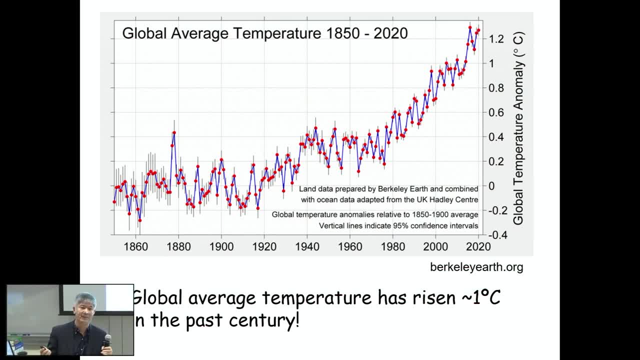 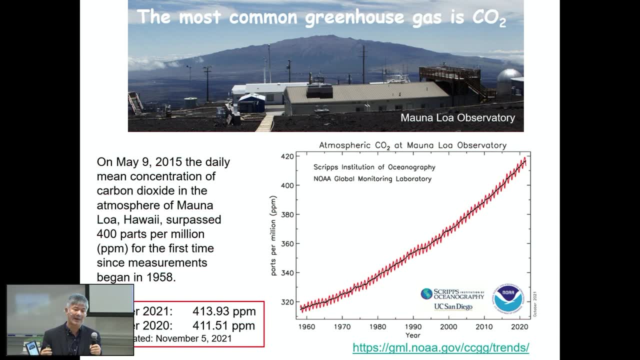 The temperature has risen about one degree in the last century. okay, And we believe that this warming is caused by human meat. We are releasing, We are burning fossil fuel and we are destroying our forests, et cetera. So anthropogenic CO2 is one of the 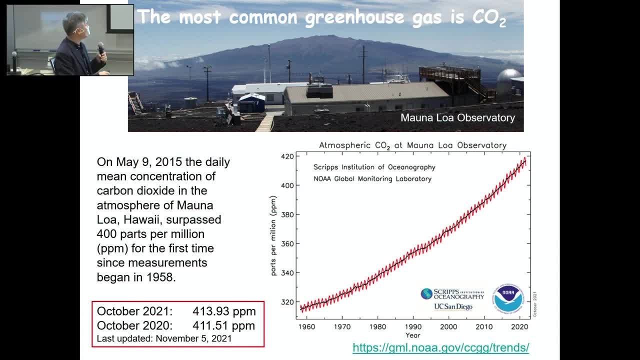 It's the number one greenhouse gas. Okay, So this is a record start from 1958 at top of the Mauna Loa mountain in Hawaii. So you see it started with around 300, now it's 400. If you go to this website you can get the number. 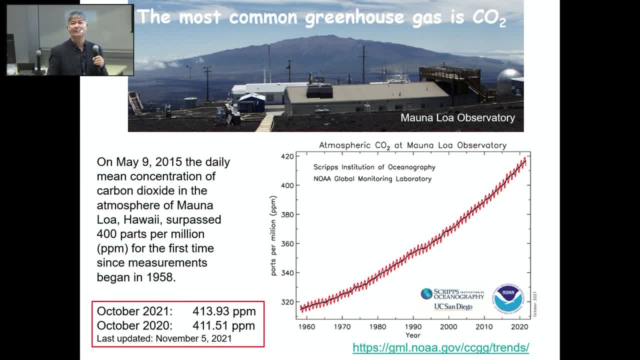 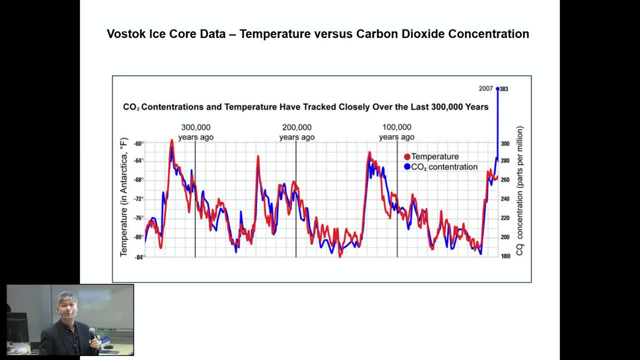 Okay, So it's keep rising still. And there are studies. Okay, So a study like this one is from the ice core, you know, showing very, very good correlation between temperature and the CO2.. Okay, So, in the last several glacial interglacial cycle, the CO2 concentration never exceeded. 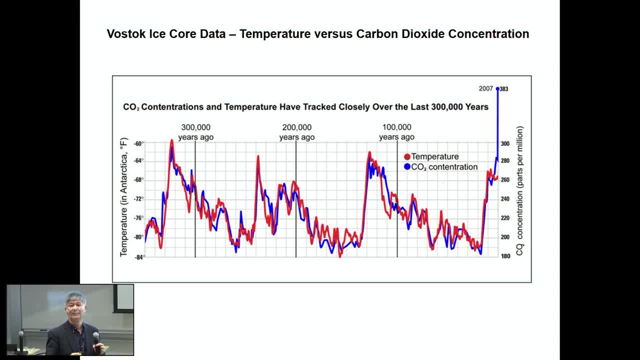 300.. Right now we are at 450.. Okay, So scientists are worried, You know, You know They're worried, you know whether we're gonna ever have this kind of glacial or interglacial cycle again. Okay, 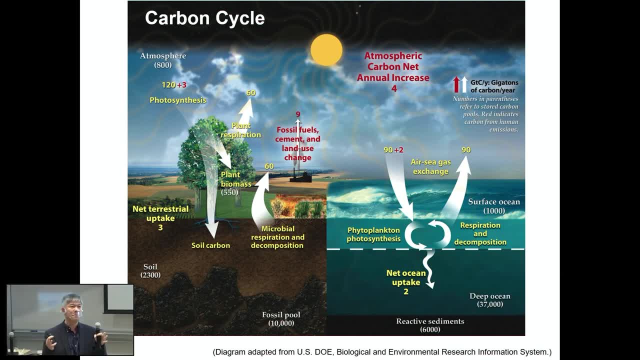 So ocean? you know lots of people, surprisingly. you know Hong Kong is surrounded by ocean, but our knowledge on ocean are quite limited. Okay, So ocean is very important in absorbing low CO2.. Okay, So here I don't have the detail to talk about. 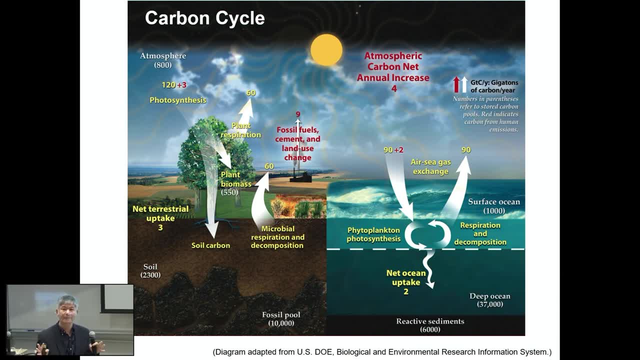 And don't worry about this detailed number, because different model gives different number. But one thing: ocean is as important as the terrestrial ecosystem. They are about half-half in total primary production, And ocean also absorb about one-third of the anthropogenic CO2 we emit every year. 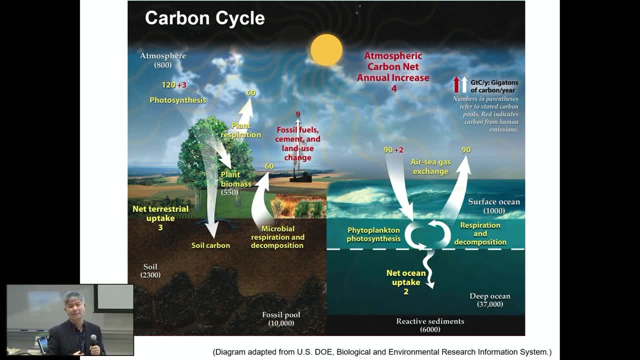 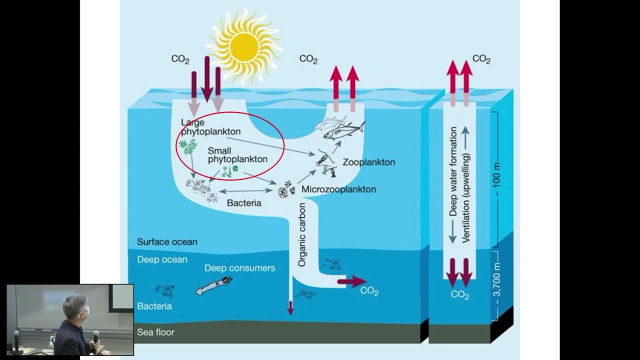 Okay, So if we absorb CO2 from the ocean, the Earth will be much harder. Okay, So what happened? What? How? the ocean? You know this is what happened. Photosynthesis: Okay, Although this is a very complex, this is called a biological pump, but it start with photosynthesis. 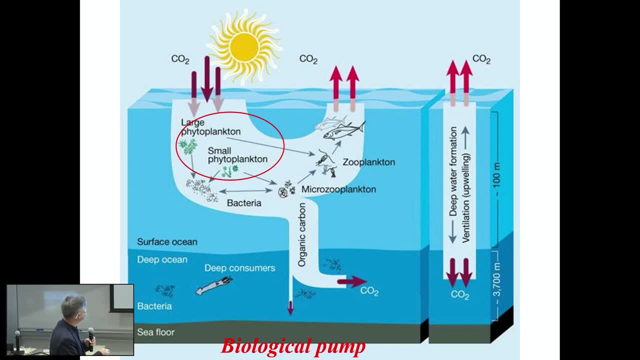 It absorbs CO2.. Okay, And most of this CO2, organic carbon, eventually return through renewable energy, Right Right Through respiration degradation, et cetera. Okay, But a small portion exported to the deep ocean and eventually buried in the sea floor. 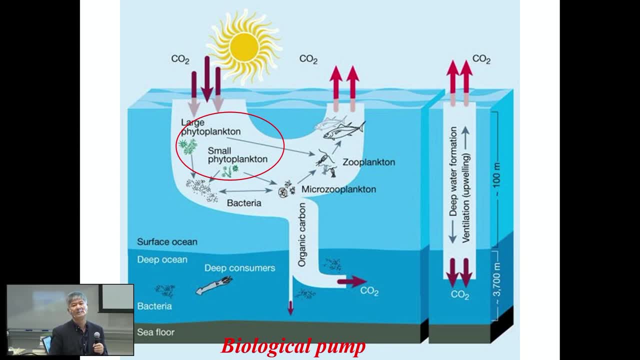 Okay, So they will be there, probably locked for a thousand or million years. So that's very, very important. carbon sequestration, Okay, As we are now talking about carbon neutral Okay, Zero emission, et cetera, you know. 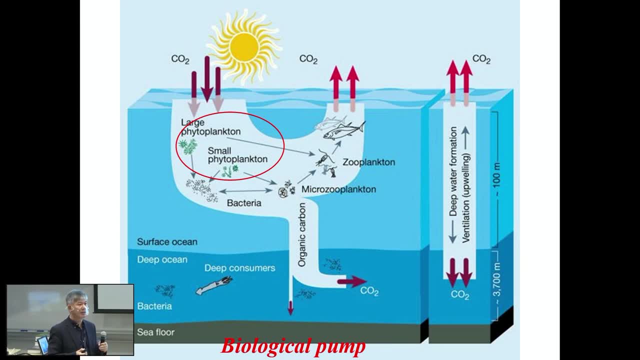 But no one talking about ocean. Our university have some initiative. I went there a briefing: one, two, three, four, five. you know this area with no ocean And I told them: ocean equal all of your. one, two, three, four, five, more than that. 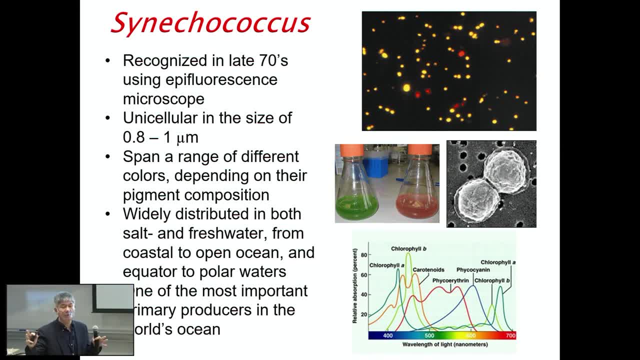 So they will add that. Okay. So I'm back to the cyanobacteria I studied. These are very, very tiny thing, Smaller than one micrometer. Okay. So you cannot even see them under microscope regularly. So there's a few groups. 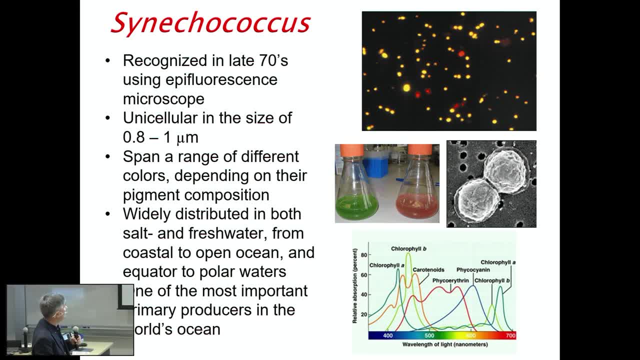 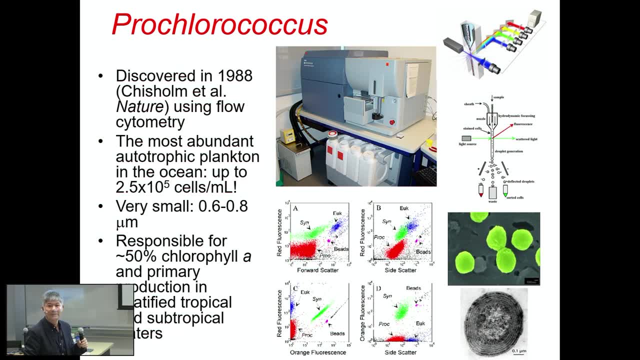 One is called the Sinica carcass, which I you know- I won't talk very detail because I can talk hours about that- Okay. Another one is Proco carcass. They're even smaller, Okay, And they cannot even seen, be seen by epiphylaxis microscope. 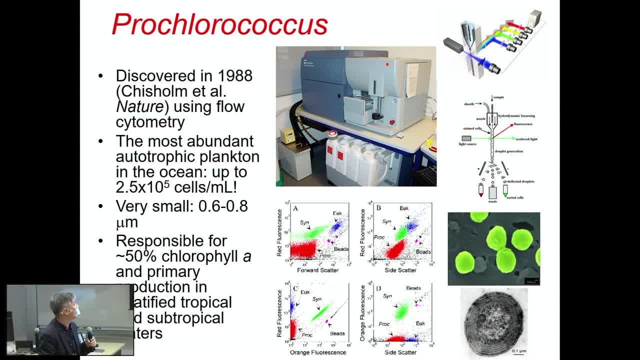 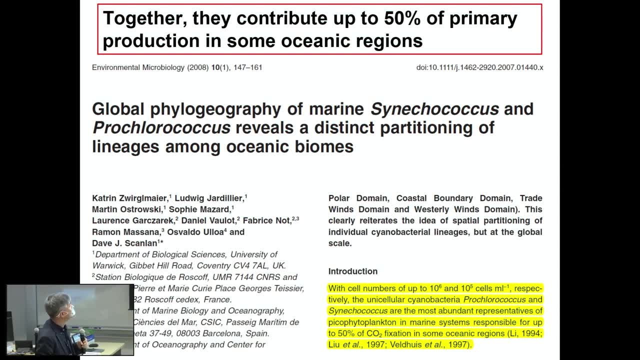 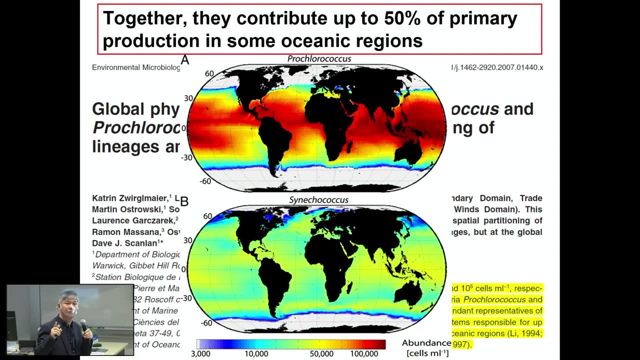 They can only be seen in this flow cytometry. Okay, I have five minutes. Okay, So why they important? Because they are up to 50% of primary production in some oceanic waters. Okay, And you know, the Proco carcass mostly only distributed in the warm subtropical region. 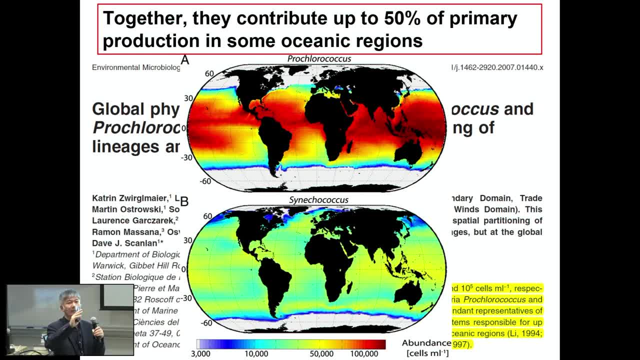 Okay, Oceanic waters. You know, if you go to pool shelter in front of our campus, take some water. no Proco carcass, Because only in very, very nutrient pool open ocean water. But Sinica carcass is everywhere, from equator all the way to polar, from freshwater to open. 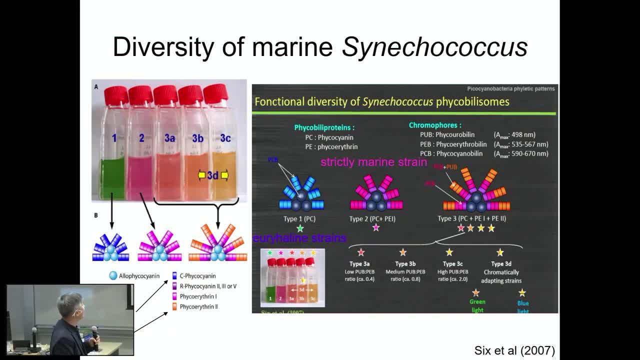 ocean. Okay, So the focus is on Sinica carcass. Okay, So they have all different kind of phenotypes, different pigment types. These are all Sinica carcass with different pigment composition, which I don't have time to go deep. 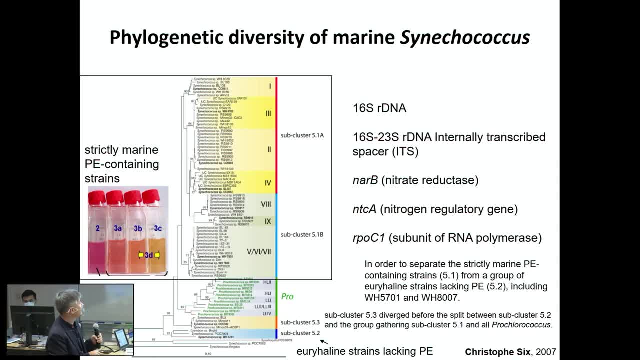 Okay. And also phylogenetically, they're even more complicated. you know, high diversity, Because this forum is about biodiversity. Okay, So there's many, many different clades, Okay. So again, you know, we are focused on this Urihalium species. 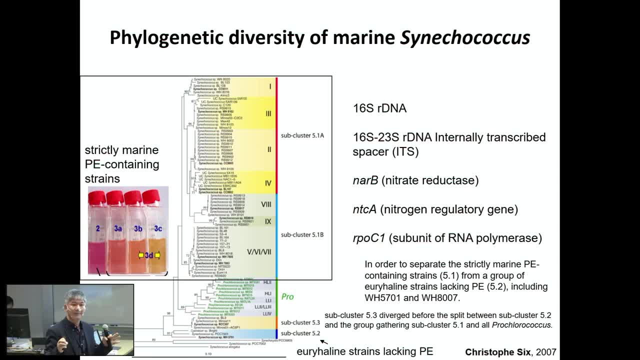 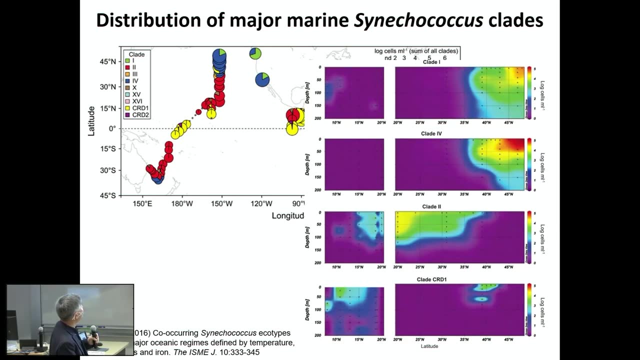 Here we have Pearl River, So this species can grow in very broad range of salinity. Okay, And they are understudied. Most of the study is in open ocean and this area Okay, So I mentioned there's lots of different clades. 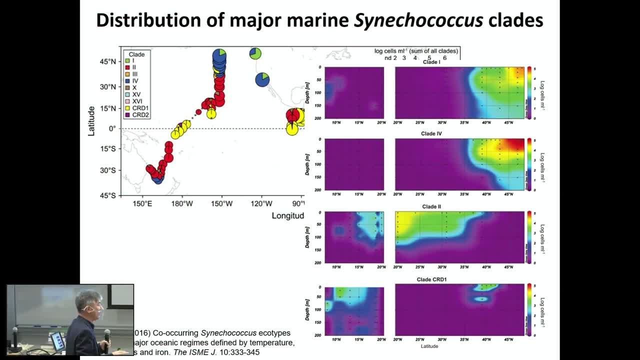 Different types. They all have different features- physiology, ecology- And they have a different geographic distribution. Okay, For example, clade one, clade four are kind of a cold water, Okay, Along this cruise, You know. Clade two is typical warm water, subtropical. 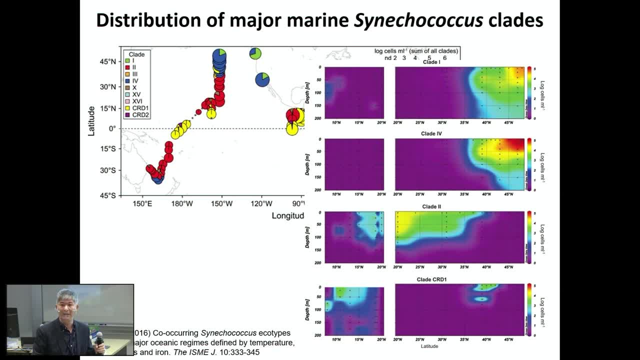 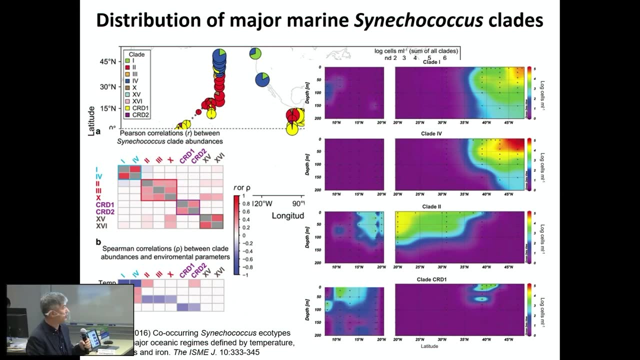 And clade. CRD is related to the upwelling- Coastal, I mean equatorial, upwelling, Okay. CRD means Costa Rica Dome, which is where they first discovered Okay. So, and they are related, controlled by different environment factors. 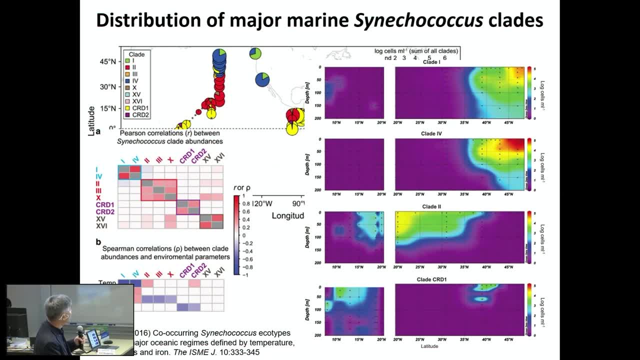 For example, this clade, one and two, four. they are, you know, negatively correlated to temperature. You know They love cold, and nutrients, et cetera. Okay, Due to time limit. Okay, So we have Hong Kong. 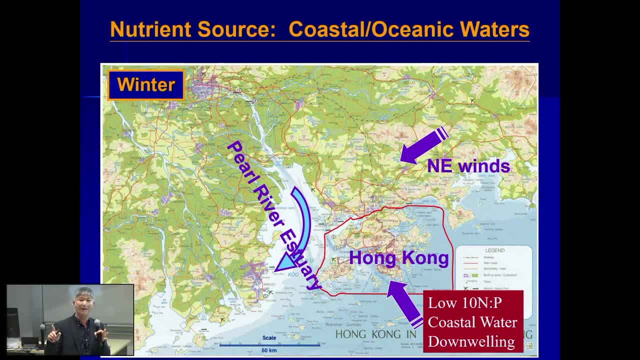 Hong Kong is actually a very cold place. Okay, Hong Kong is actually a hot spot of the diversity of cynical cultures. Okay, Because we have a river, we have a monsoon. Okay, Wintertime, Northeast monsoon, Okay. 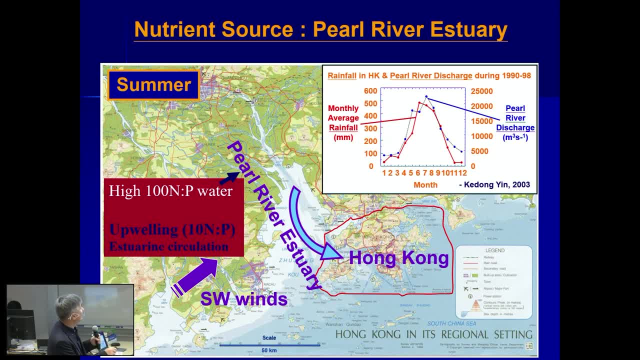 One minute. Okay, You know, summertime we have a southwest monsoon and river discharge, So there's a mixing of all kinds of water. That's why we have all types of water. That's why we have all types of cynical cultures. 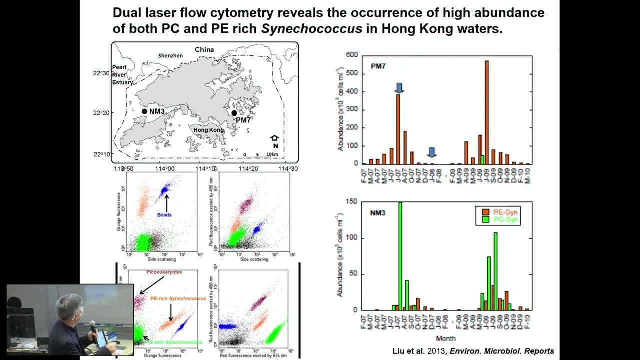 Okay, For example, here in the riverside, in the port shelter, you see there's a. every month we do this study. there's a peak in summer, but different types. You know, In the riverside there's lots of green forest. 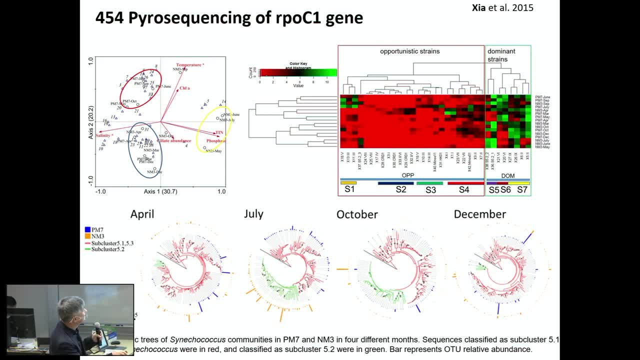 And you see the different clade: Okay, Some of them they are all year round, Some of them only a few, a special period of time, Okay. And if you compare the riverside with the UST side, okay, some season they are overlap. 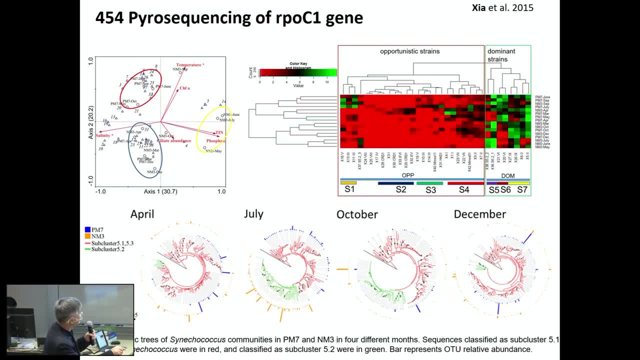 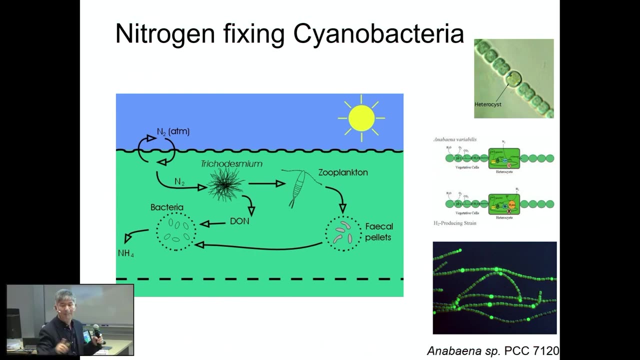 In the summer it's completely separate. Okay, In this side it's mostly 5.1. And over that side it's 5.2.. Okay, So I give me one more minutes. I'll talk a little bit about some of them: fixed nitrogen. 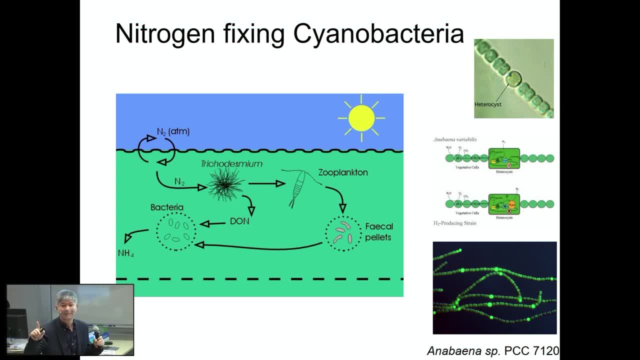 Okay, Why they are important. You know here we have eutrophication: too much nitrogen, But in the middle of ocean no nitrogen, Very, very low nitrogen, And that limited the primary production. Okay, So this cyanobacteria can fix nitrogen. 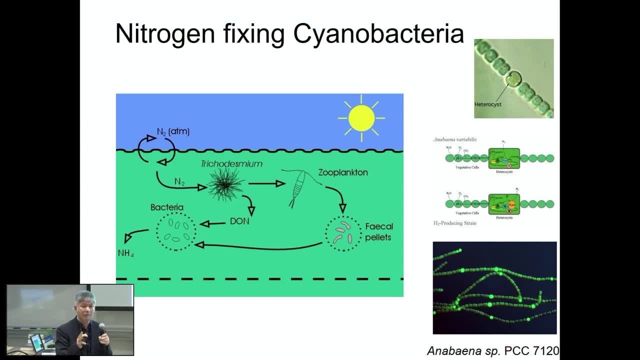 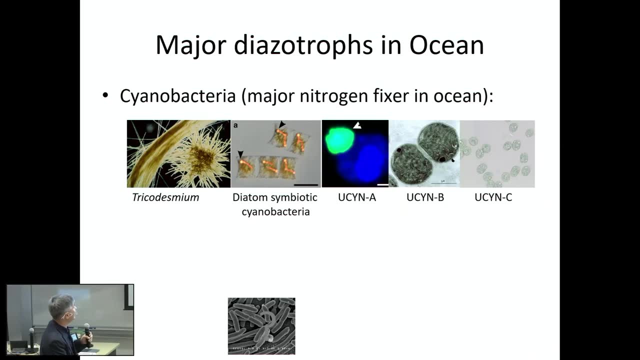 So this nitrogen not only provide nutrient for themselves, they can also supply other phytoplankton to grow Okay. So this I don't have time. There's a different type of nitrogen fixer: cyanobacteria. Okay, And I just want to show you one study we did from across the Pacific Ocean with the Japanese. 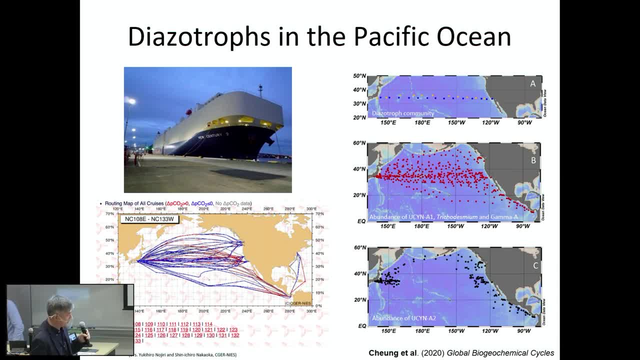 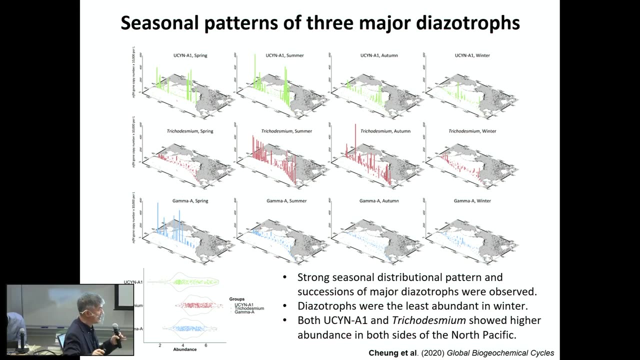 collaborator, This huge ship. they ship Toyota, belong to Toyota. They ship car to North America. So we did kind of study And we discover lots of different nitrogen fixing, cyanobacteria. Okay, So I think that's all. We are studying the effect of global warming. 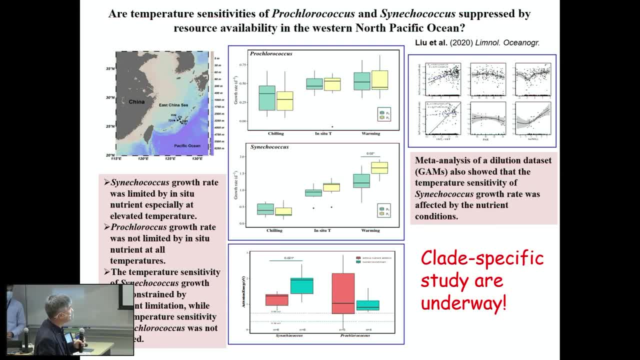 And we are going to study the so-called clay-specific, Which means I told you, there are many, many, many types And we want to know their different response to the global warming. Okay, So, thank you very much, Thank you. 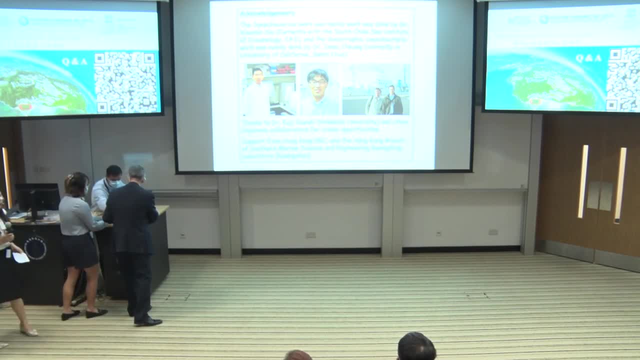 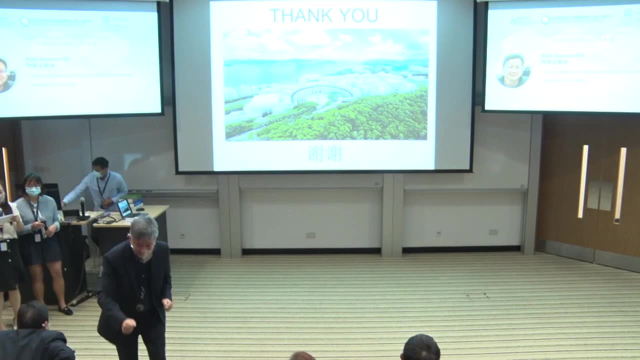 Thank you, Professor. Thank you, Professor Liu. Okay, Time is running short, So moving right along, let's welcome another guest speaker, Professor Qiu Jianwen, the professor of Department of Biology of Hong Kong Baptist University. The presentation topic is Searching for the Footprints of Marine Worms of Hong Kong. 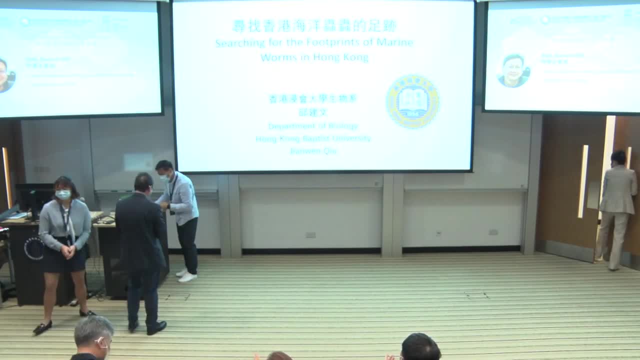 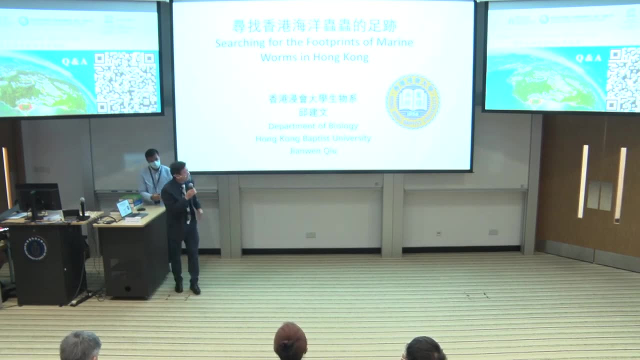 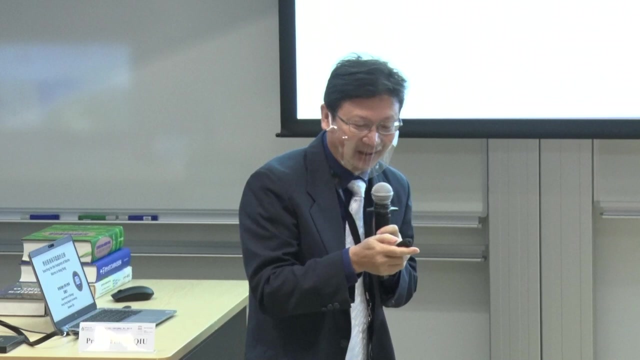 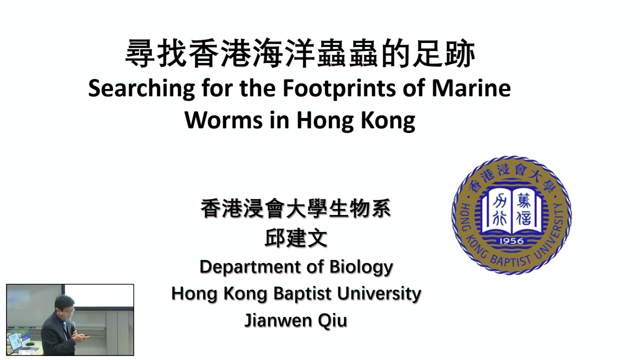 Welcome, Professor Qiu. Thank you for the invitation to speak here. Thank you. So again, like Hongping's talk, my talk is about something that people usually won't consider to be important for that group of organisms, So people won't even consider them when they evaluate the ecological values of the animals. 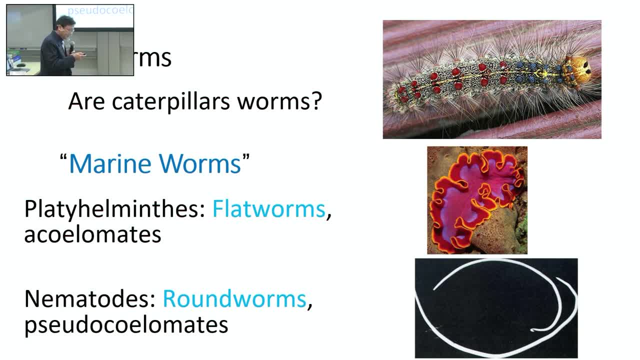 So my talk is about worms. So when people think about worms, normally they will think about terrestrial insects. But actually in the marine environment there are a lot of worms. So we have heard about flatworms, We have heard about roundworms. 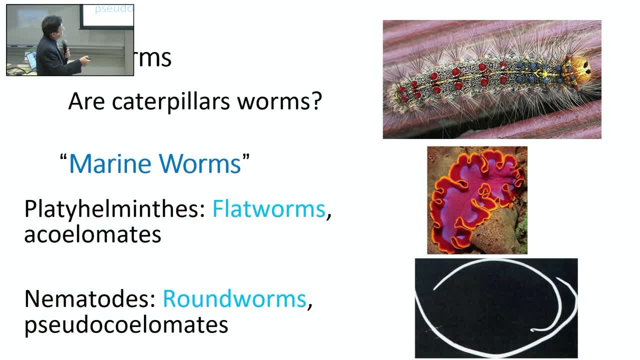 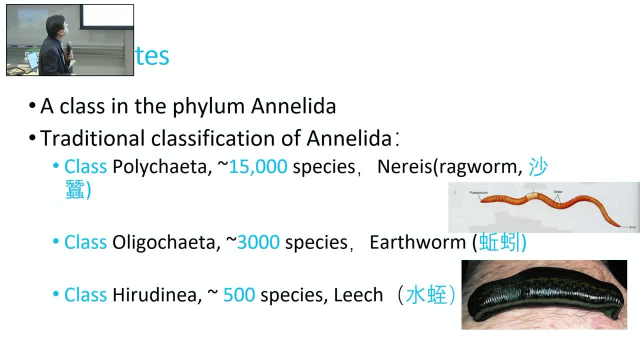 So we know flatworms: they have very simple body, They don't have a coelom. And roundworms: they have a pseudocelum. But my talk will be focused on this group of animals. They are called pollicates. 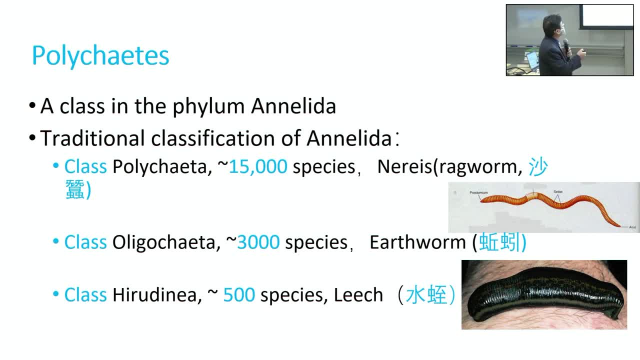 So they belong to a class, traditionally a class of analida. So in analida, we know, there are pollicates, There are oligocates, represented by a worm, And Herodinia, represented by leech. So what I'm focusing on is this group of animals. 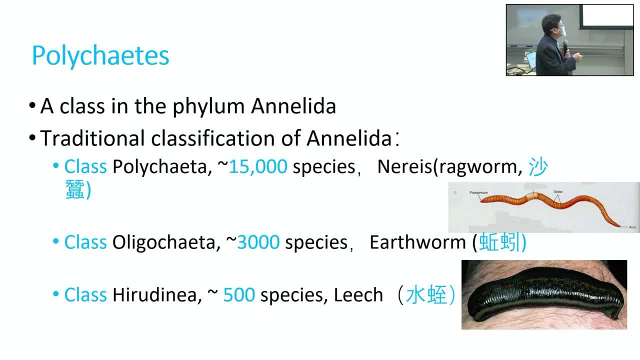 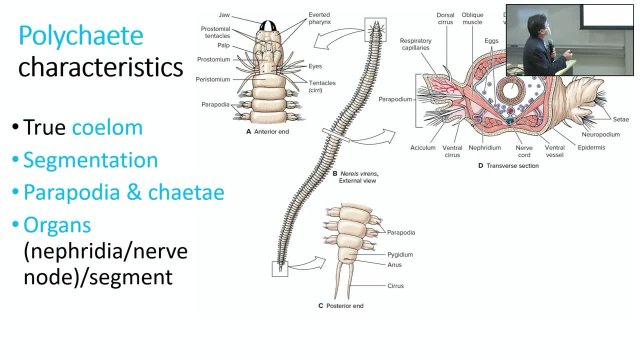 It's this group of animals called pollicates. So these organisms, they are called pollicates because they have a lot of hair, A lot of kitty on their body And, attached to their parapodia, This is actually their locomotive organ. 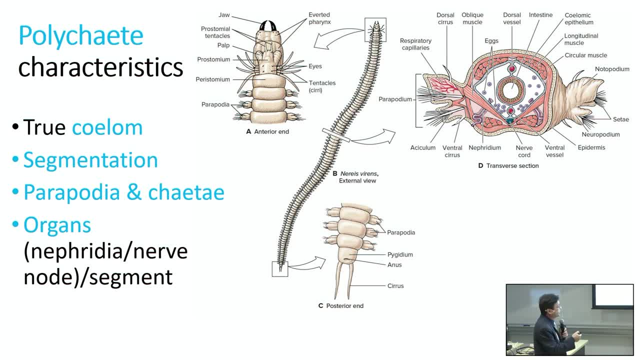 They used to move about, They used to swim. They have a true coelom over here And their body has a lot of segments, segmentation And their organs- some of their organs, like an aphidia, and nerve nodes, are repeated in each segment. 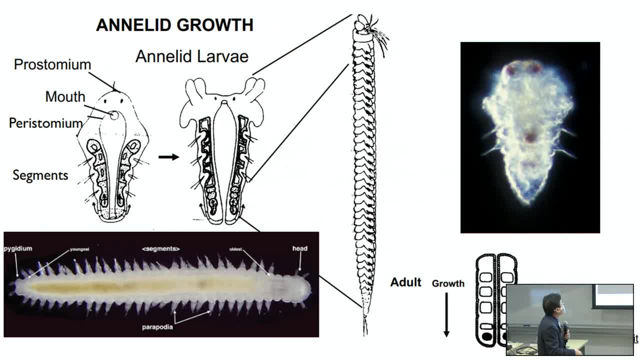 So that's the pollicates, But pollicates, they have a lot of segments, but the segments will not form In the beginning of their life. So in the beginning of their life they have only very few segments. So these segments, they grow. 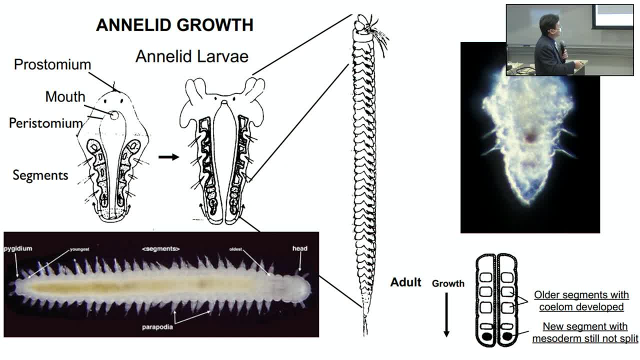 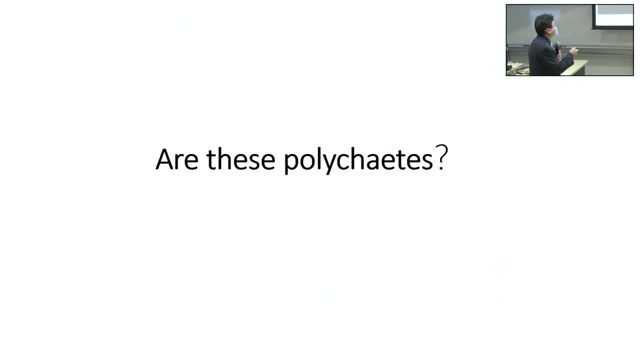 So those near the head are old ones, And those at the tail they are young ones. So as they grow they elongate. So this is how their body is arranged. So pollicates have undergone some changes over the years, Like fishes. 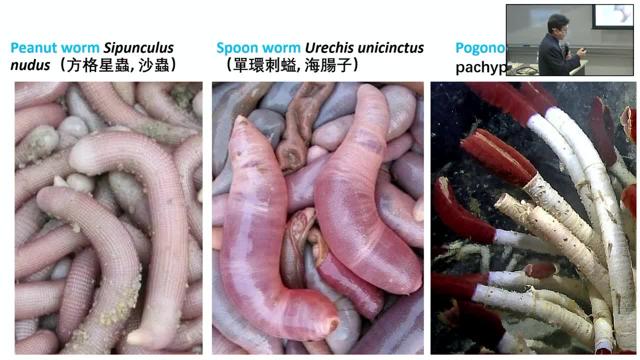 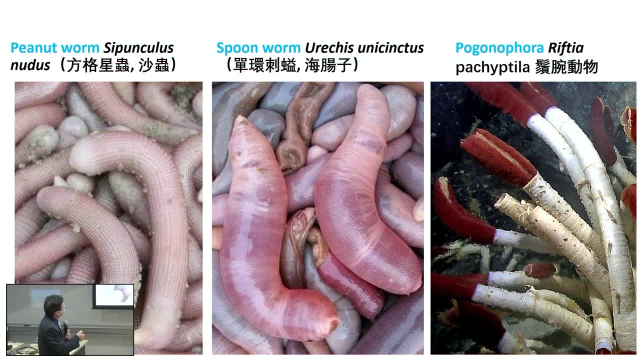 So their taxonomy has changed. Previously, some of these animals- peanut worms, spoon worms- they don't have segmentation- And Poconophora, which is a deep-sea animal. they don't even have a gut. This was considered a separate phylum. 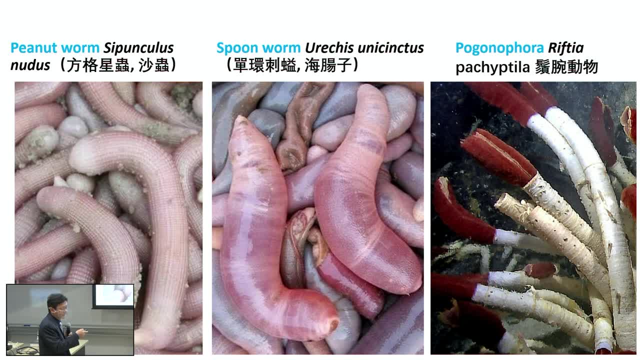 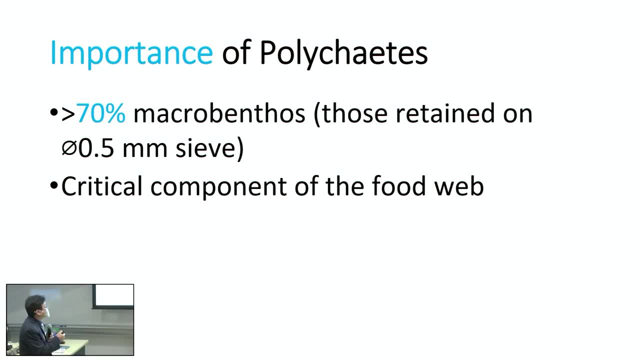 But now they are considered as animals. They are very closely related to pollicates. So pollicates, although they are not very impressive, they're not very beautiful, but they are ecologically important. They account for 70% of medical benefits. 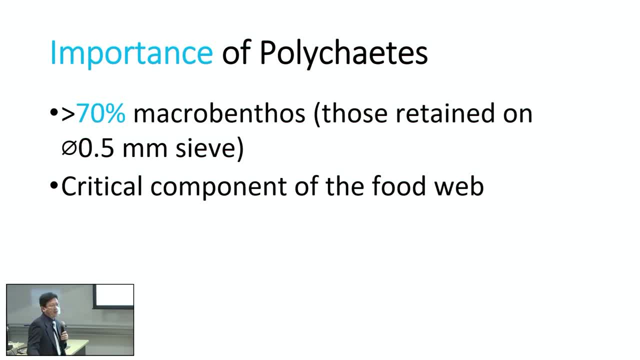 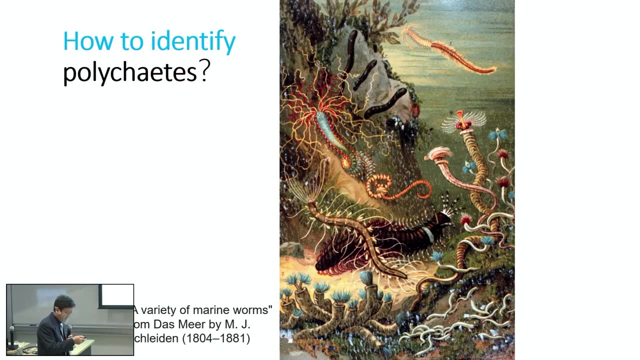 which means if you take a grout of mud from the seabottom and you sieve them, you'll see 70% of the animals are pollicates, So they are critical components of the food, where they serve as an important node in the food chain. 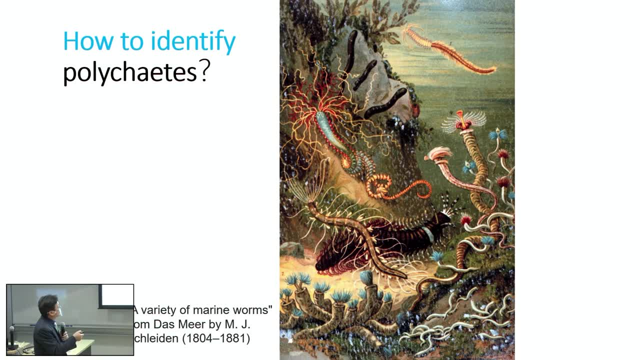 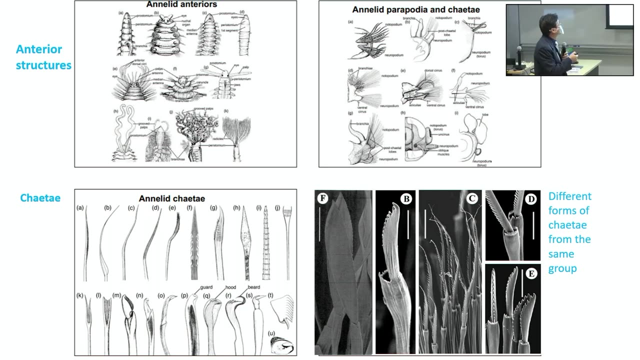 Pollicates. they are very diverse. So, as you can see from here, some are swimming, some are attached to rocks, some move above, really. So how do you identify pollicates? So we identify pollicates by morphology, Traditionally, of course, recently. 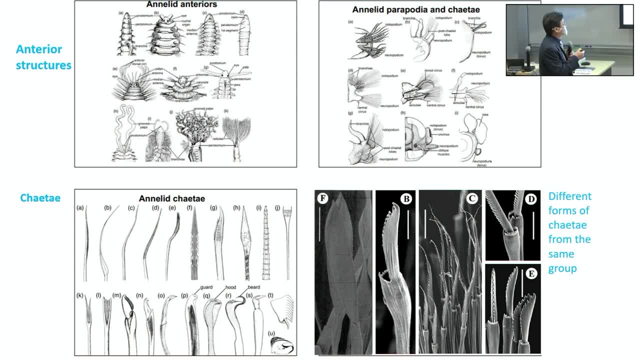 we also use molecular techniques to identify pollicates. So we first look at the anterior structures, So they are very distinct, And also the parapodia and the city. So in an earlier study I did with Professor Chen from just one group of pollicates 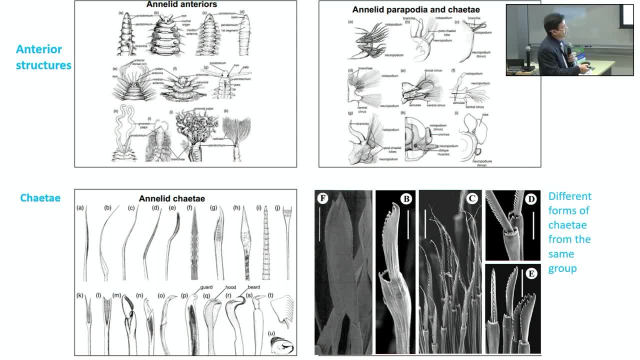 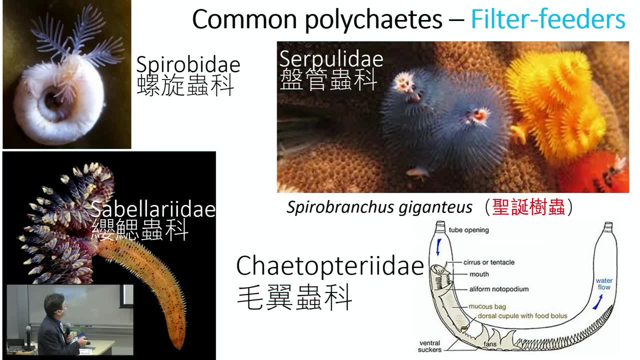 we see very different. The first group of pollicates are filter feeders. So based on this we can identify these pollicates. So I'll just briefly introduce you to several groups of pollicates. The first group of pollicates are filter feeders. 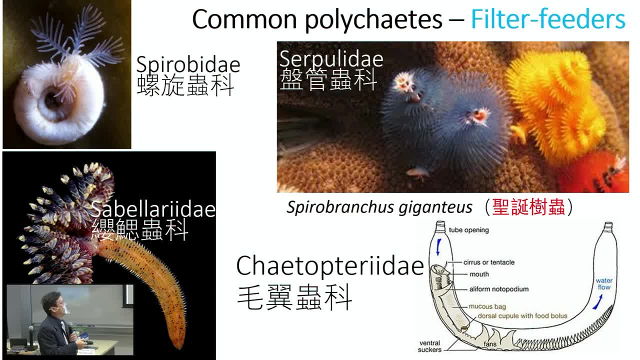 like the very commonly encountered pollicates when you go diving in more tropical water- The Christmas tree ones. they are filter feeders, But there are also spirobates. There are also the feather-dusty ones, sabelis, and also these chytoterras living in a tube. 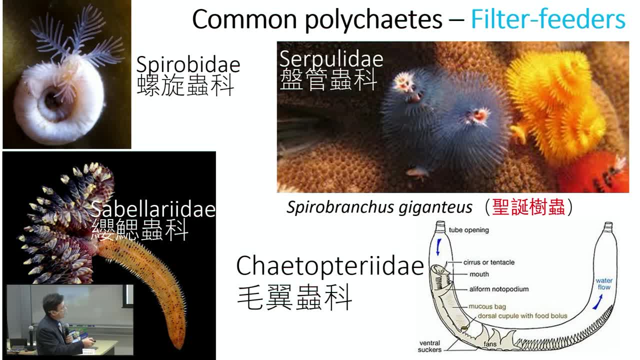 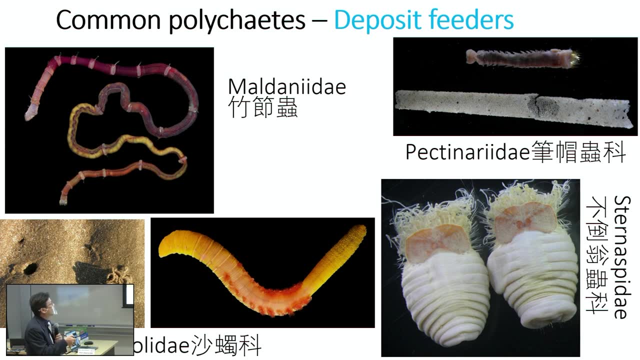 pumping water from this side to the fluid and acetic water from this side. So these are filter feeders And there are also deposit feeders, like this one bamboo one, and also this ice cream cone one, and also this rock one. 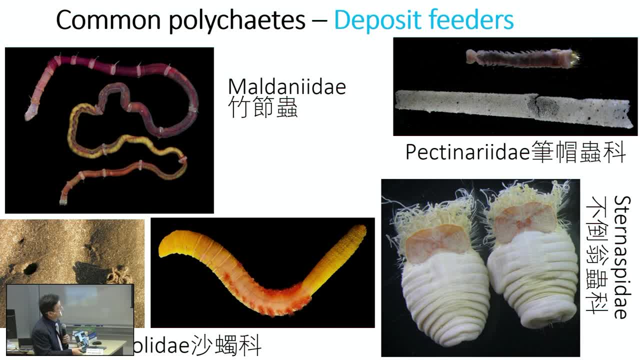 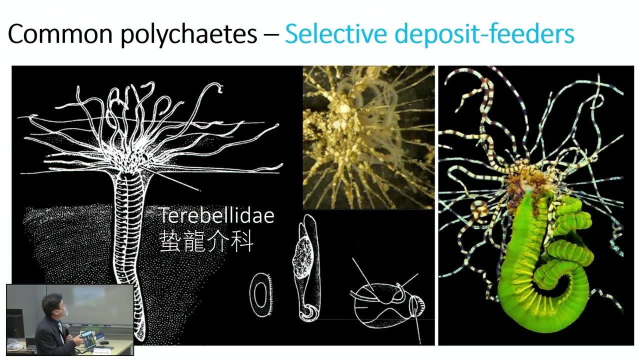 and as well as this, this last big like. they look like Russian dolls, So very pretty, with very short body, So they can be- some of them can be quite pretty. And there are some selective deposit feeders, like those spaghetti one. 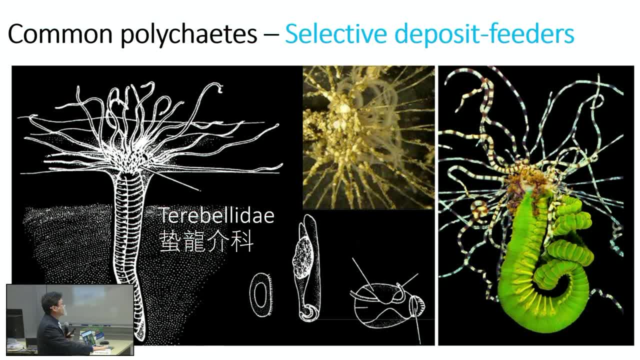 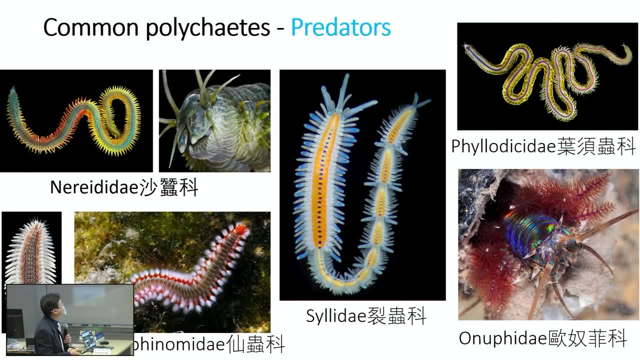 They extend their tentacles to the surface of the of the mouth and they collect the organic matter and they roll this organic matter into the mouth. So these are selective deposit feeders But probably the most impressive ones are predators like the nereids. 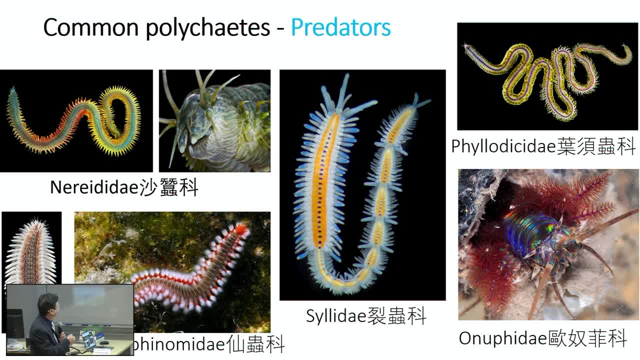 So they are common predators And the fire worms. they have toxic venoms in their bristles And cilis, which are famous for their remarkable ability to reproduce essentially, And phallodocytes, which can be identified very easily because their dorsal series. 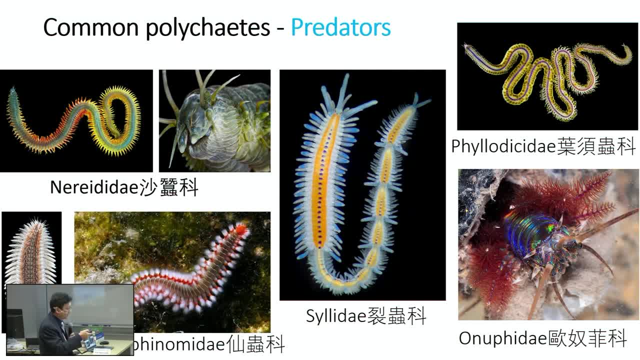 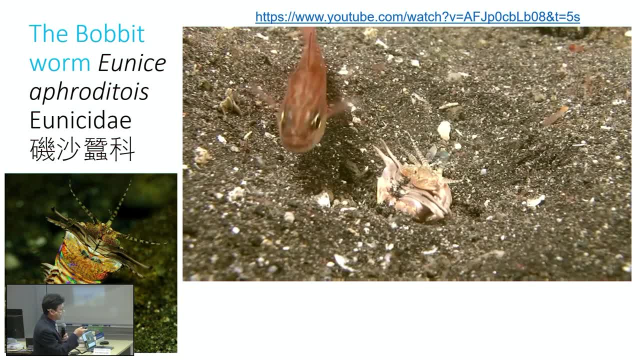 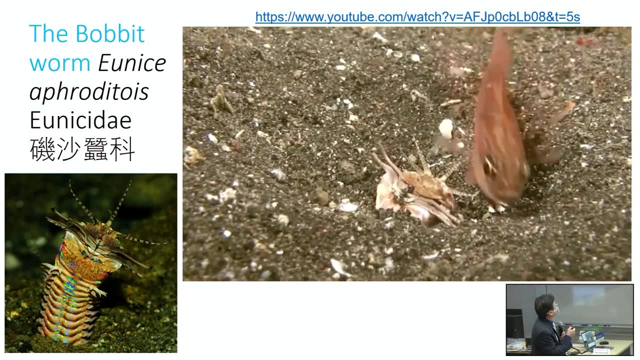 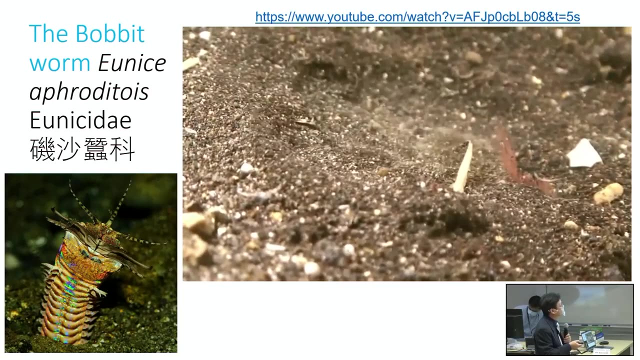 is expanding like a leaf, And then the ambush predators, or nereids. So I'd like to share with you this video I took from the internet about this bobby worm, which is a famous predator of the morning water. It's located. 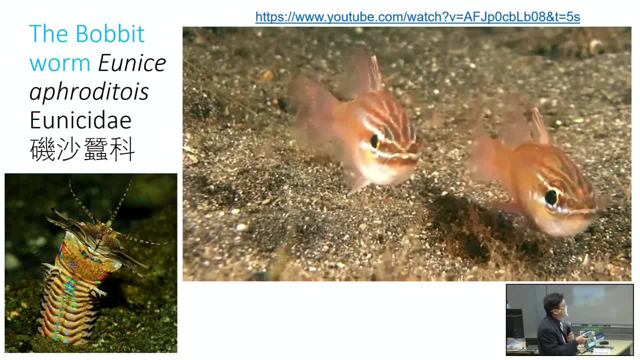 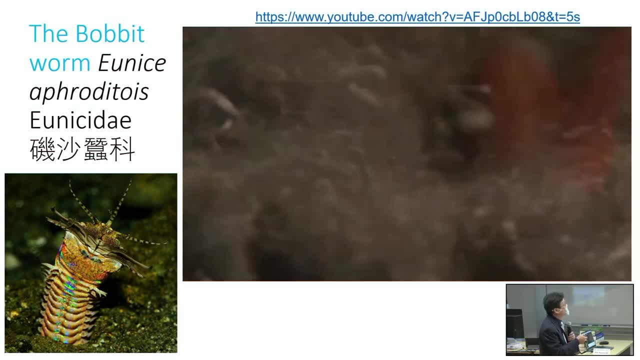 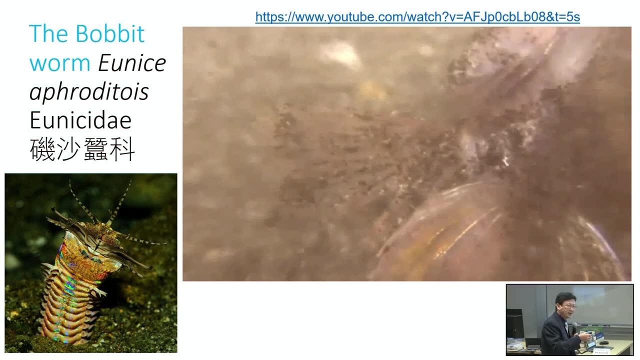 its habitat is more tropical in Indonesia, but in Hong Kong we have a relative of this bobby worm as well. So polychaes, although they are not very pretty most of them, but they have very different functions in the ecosystem. 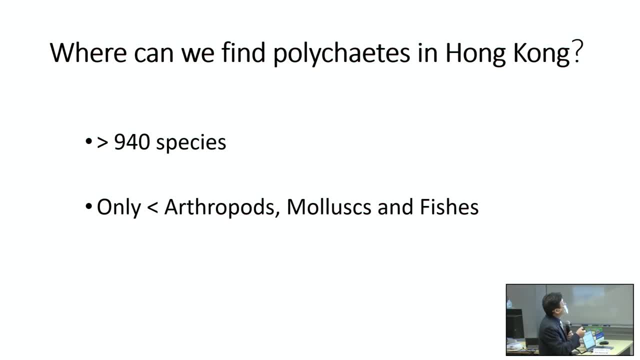 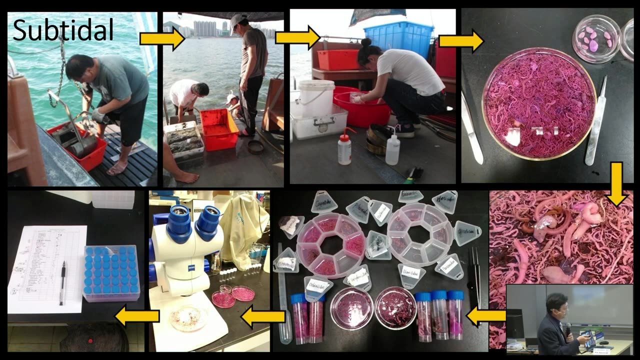 In Hong Kong we have about 940 species, So just less than arthropods, molluscars and fishes, but they are still a very dominant group of animals in Hong Kong. But two of the problems: we don't know much about them. 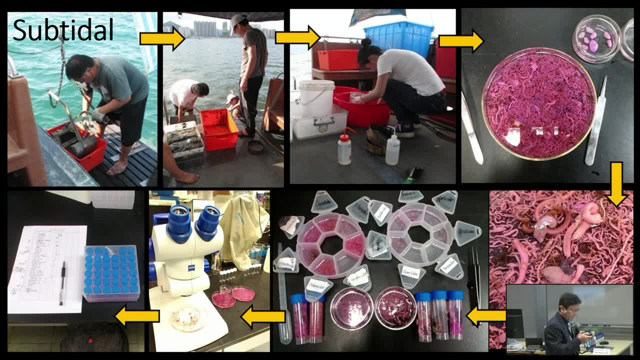 So where you can find them? The first place you can find them is to go down to the water. This is how, previously, we collect these animals. We use the muck grout, We grab the muck and we sieve the muck and we sort the muck. 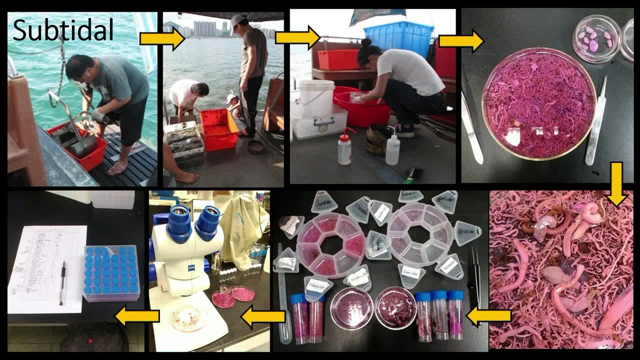 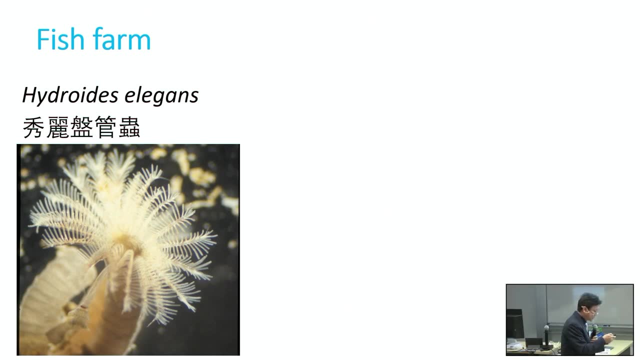 Sometimes you can get a lot of animals in a lot of animals. Among them, a lot are polychaes from just one one web of muck, And then we saw them, we identified them. So, in addition to this, we can find them. 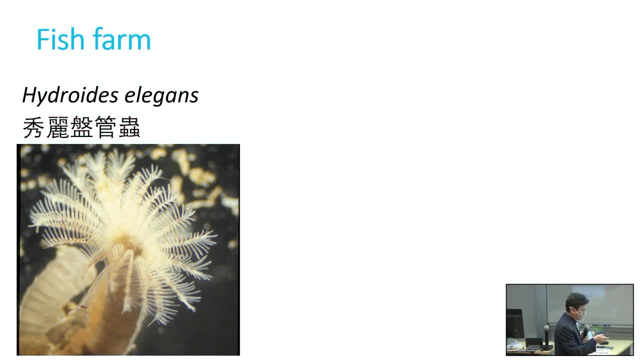 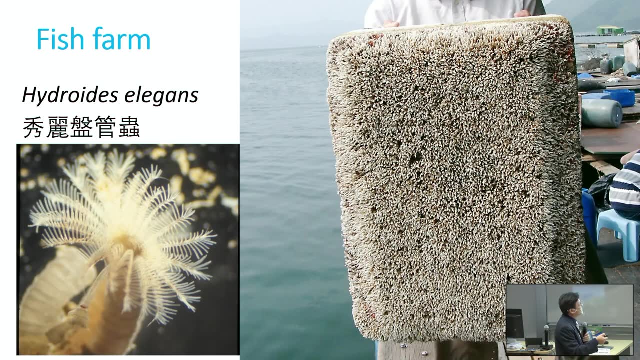 in a lot of other habitats like fish farms. This one, a hydroides, is a small one. You wouldn't think you can find so many polychaes just in one style form put into the water. That's the picture I took. 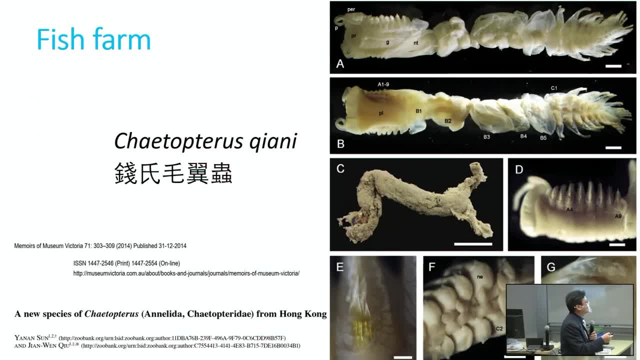 when I did my PhD with Professor Chen, And also in a fish farm. we also collect chytoterras And I named this after Professor Chen. Not very pretty, But it's leaves inside a tube and it pumps water through the tube. 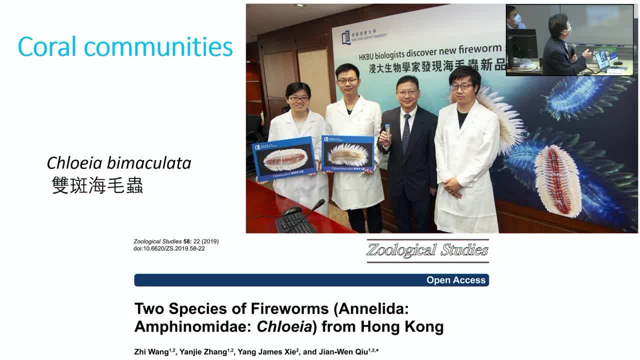 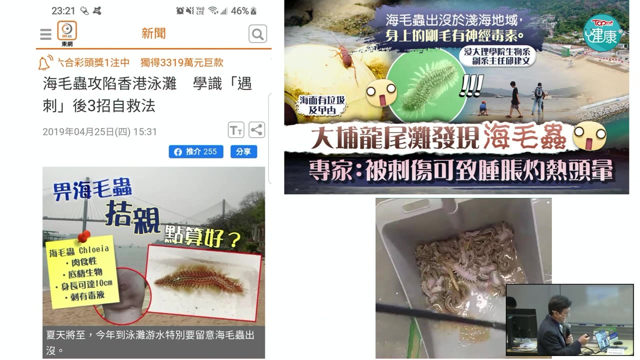 So you can find animals in a lot of places And they are also very common components of the coral community. So two years ago we found two species of these fireworms in Hong Kong. One of them actually lives in coral communities. We were interested in this. 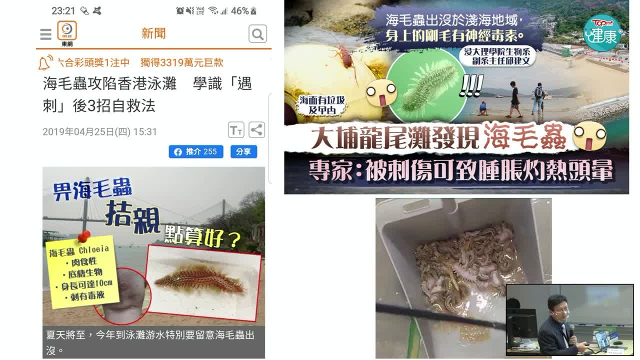 because they had to cause some panic to the public because they are toxic. as I have mentioned, If you are not very careful, you are in touch with the chyti. the infected area can be very bad, can induce a very burning sensation. 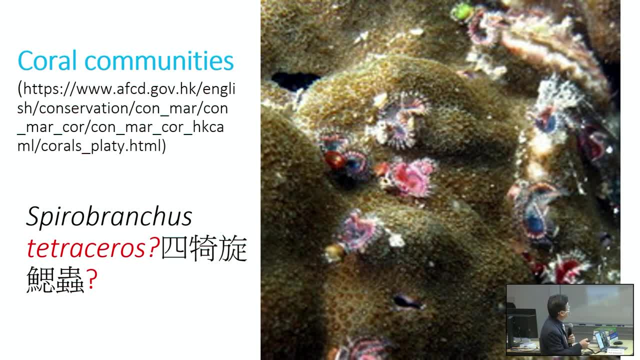 So, in addition to this, there are also a lot of other prettier polychaes, I would say So. for instance, this is Spiroblancus, which is a close relative of Christmas tree worm, But it doesn't form a tree-like structure. 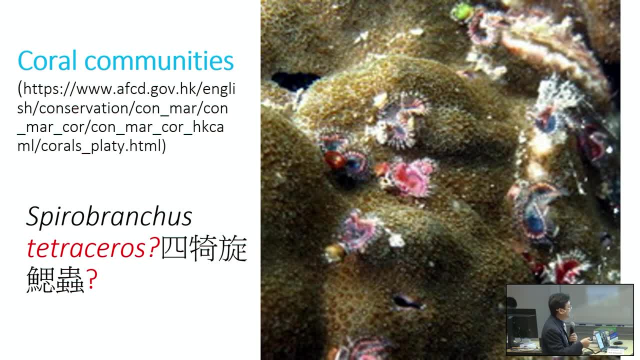 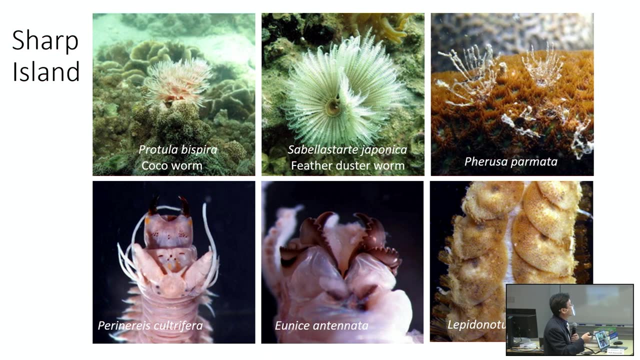 although they are very colorful as well. So it drills into a coral And it's very common in Hong Kong. Previously we gave this name to AFCD, But recently I realized it's a new. species Still are undescribed And also 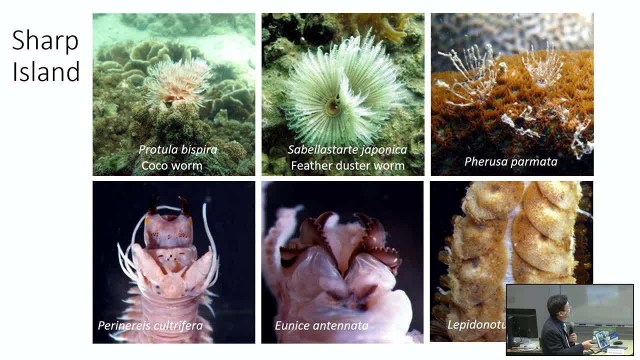 this portuna, and also the ballastis. these two species are also wrongly identified, So these are also new species. So I will describe these species later on. And there are also other predators in the area. These are filter feeders. 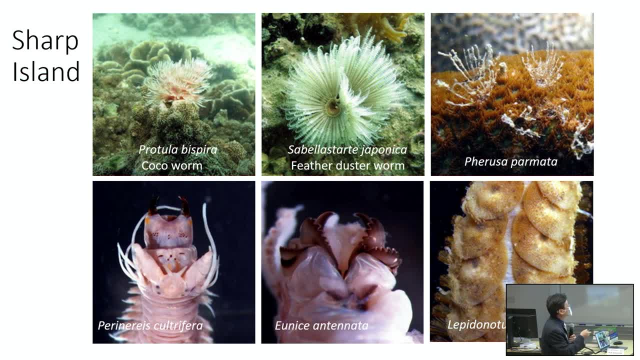 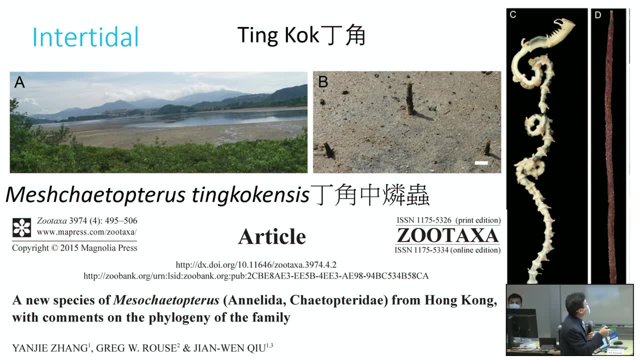 So we can find a lot of polychaes in coral communities. Another place where you can find polychaes are intertidal areas, So this new species was described a number of years ago when we visited Dinggong, So we couldn't see the animal. 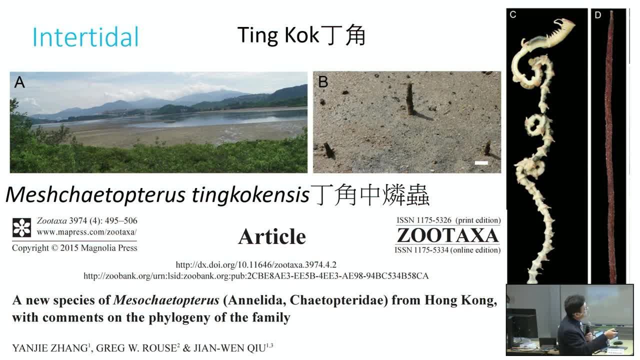 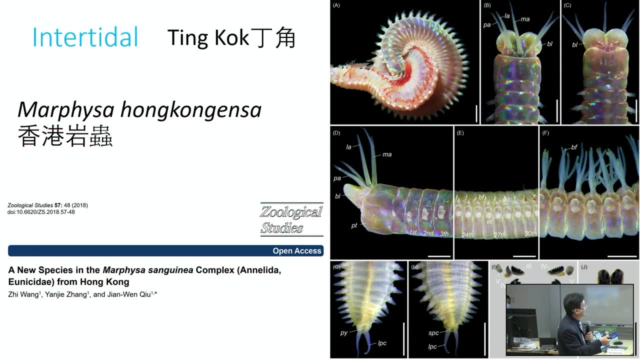 We only saw the tube, But when we dig deeper we saw this animals living inside And it's a new species. And we also saw another species. This is a relative of the bobby worm, which is a fierce predator, But in Hong Kong. 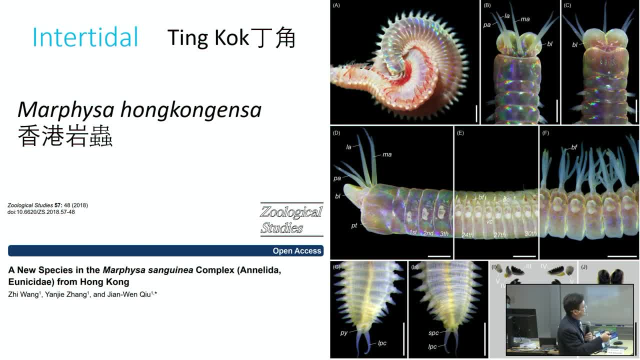 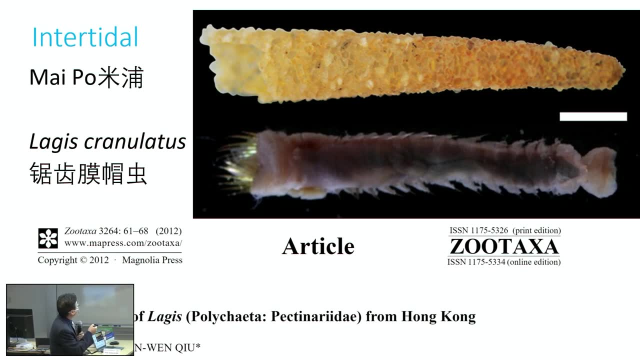 we have this species, Marfisa Hong Kong Ansa, So it has very powerful jaws as well, But people just didn't pay attention when they visited. They are very common And in the tidal area we also found this ice cream worm. 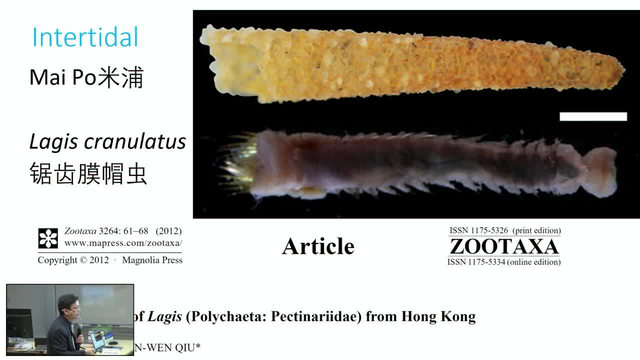 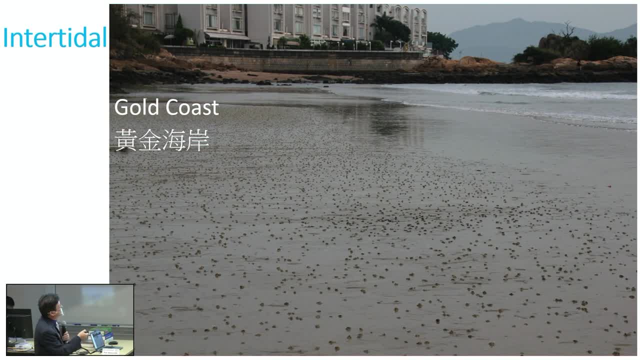 from Maipo, So you wouldn't Sorry, I don't have a lot of time, But I'll briefly go through this very quickly. So when we visited Gold Coast, we saw a lot of these small sand piles, But when we look closer, 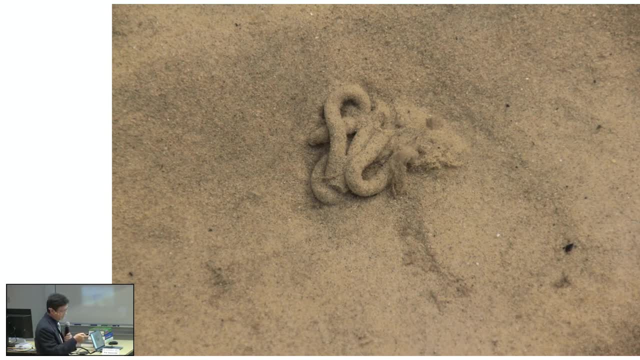 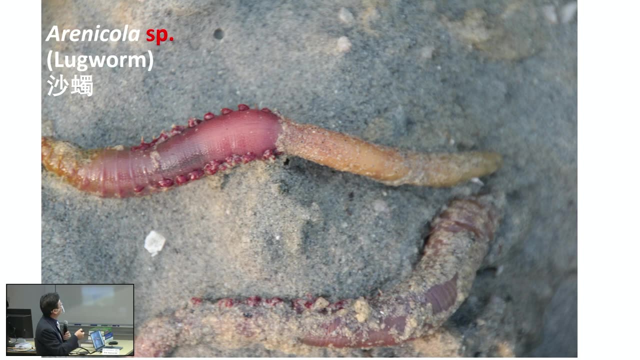 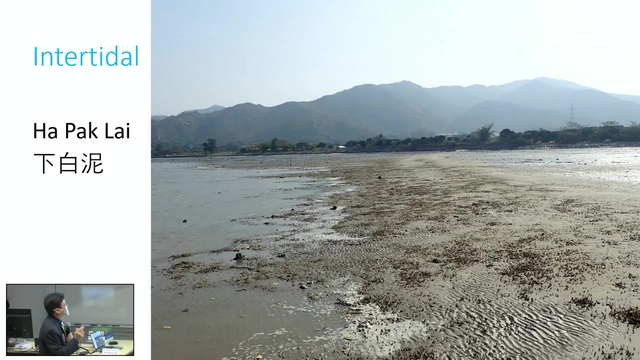 we realize these are the pools of polychaes. And when we dug inside we saw very big lugworms. They're so big, they are chopstick size each of them, So very, very impressive. And when we went to Harbaugh, 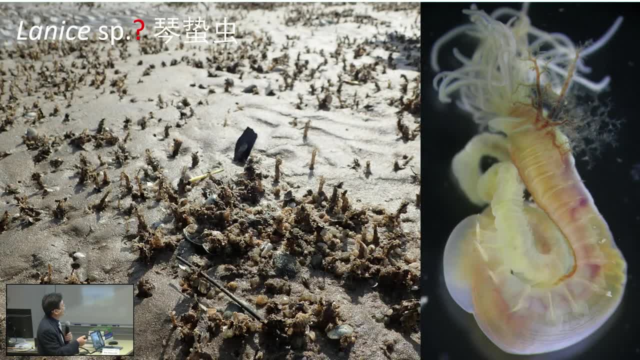 we also saw a lot of polychae tubes. Each of them is a polychae, So polychaes, they are very common, They are around us, But we just don't know about them. This is also a new species waiting for this Christian. 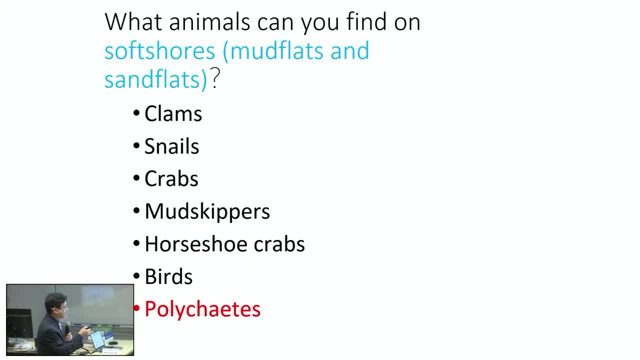 But we haven't had time to do so yet. So the message I want to bring is: when we visit a lot of places, we saw a lot of other animals, But we pay very little attention to polychaes And we feel that the soft shores 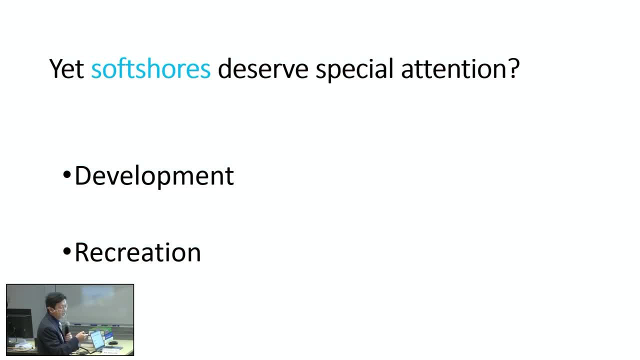 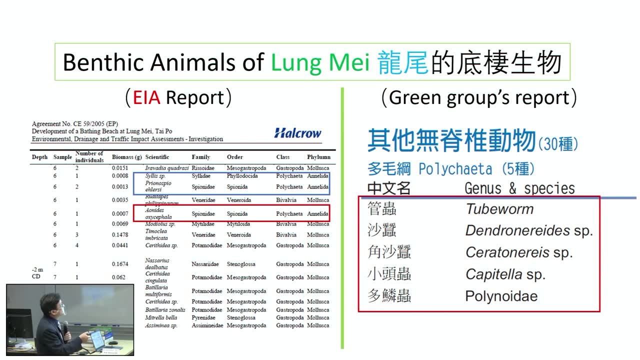 they deserve special attention because they are under the threat of development. They are under the threat of recreational activities. So, for instance, when I look at some EIA reports, I saw very few names of polychaes And a lot of names given. 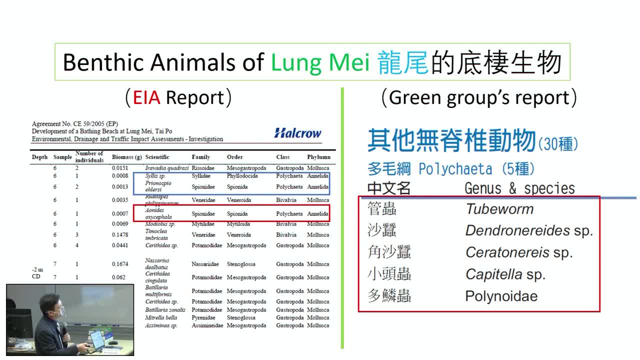 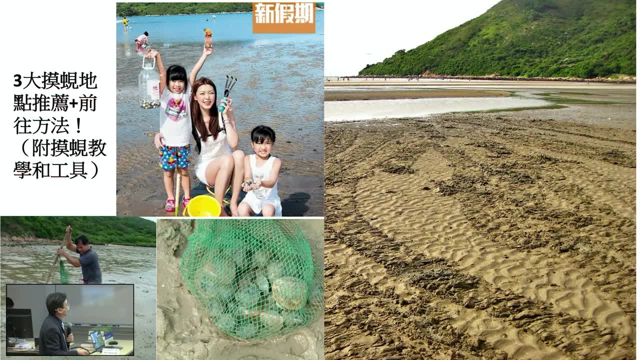 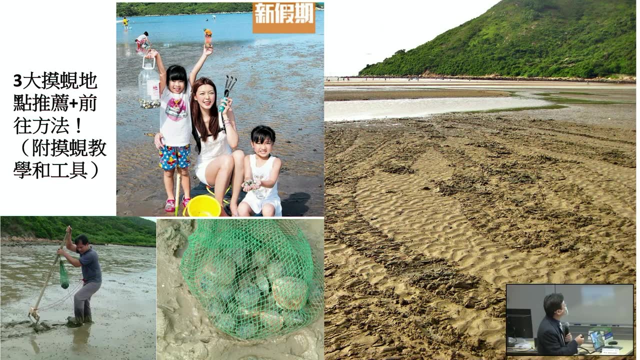 by other people. they are not even down to the species or down to the families, So they very poorly understood the diversity. So very impressive when I look at the photos of some newspapers: people actually encouraging them to go digging- clam digging. But it could be very destructive. 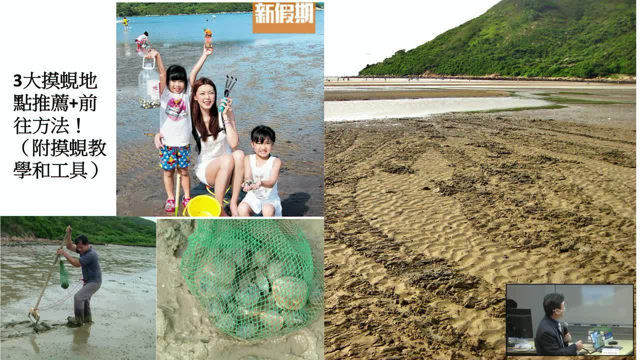 if you use this kind, especially if you have a lot of people, and some of them, using this kind of destructive sampling method. So after a long time, you will see how the habitat is destroyed. Okay, So I'll just stop here. I don't have time to go through. 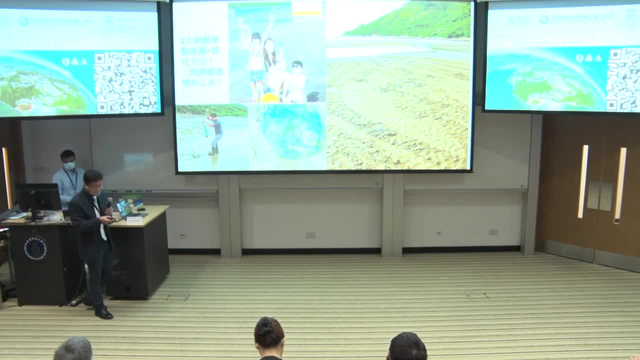 Okay, Thank you very much for your attention. Thank you, Thank you, Professor Chiu. We also have another guest speaker, but who can join us in person today, but have pre-recorded a video about natural product derived antifouling coating. 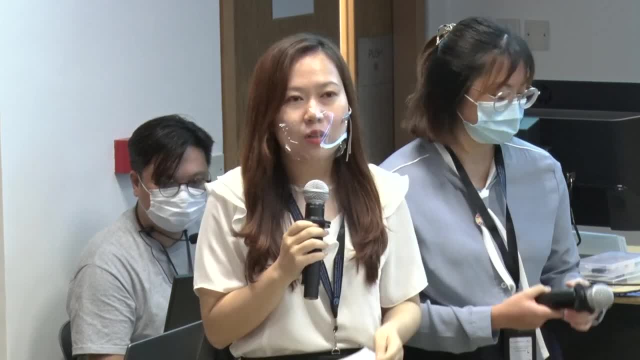 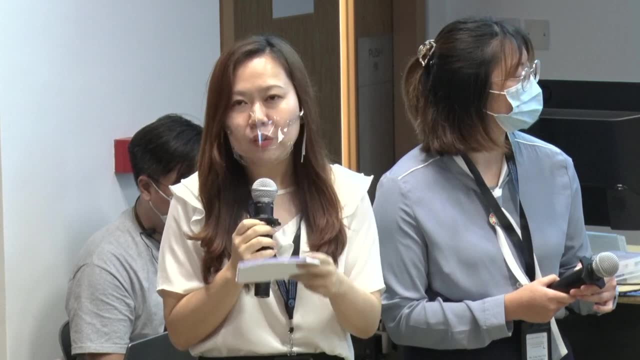 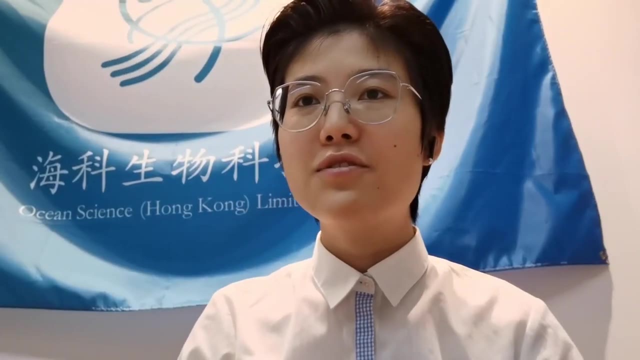 and marine environmental protection. So let's watch the video provided by Ms Ye Ma, young entrepreneur, OCES of Hong Kong University of Science and Technology and also the CEO of Ocean Science Hong Kong Limited. Good afternoon everyone. I'm very glad to be invited. 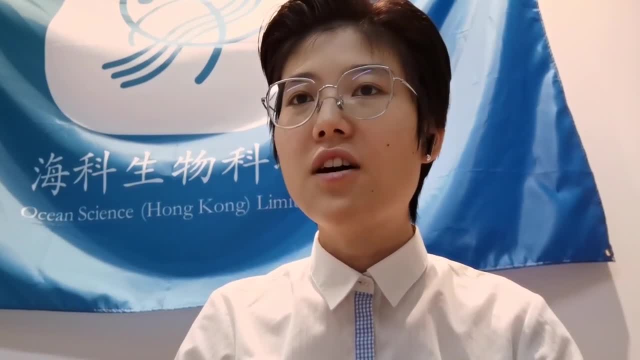 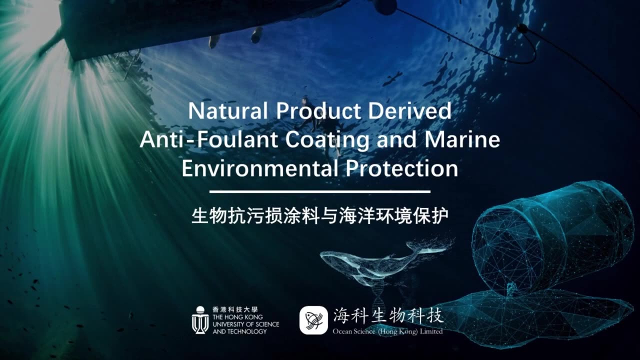 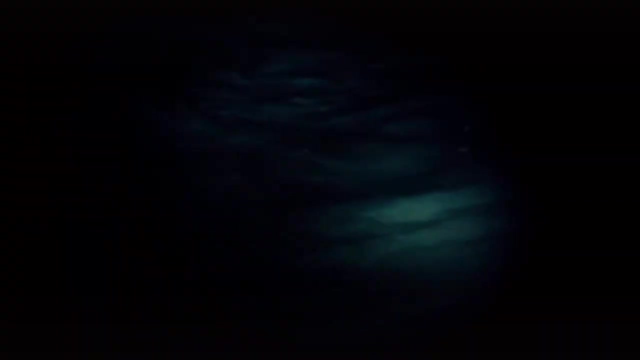 to this forum. I'm Ma Ye, CEO of Ocean Science Hong Kong Limited. The share I bring to you this time is natural product that wore, antifouling coating and marine environmental protection to protect the environment. The ocean is a mysterious underwater kingdom. 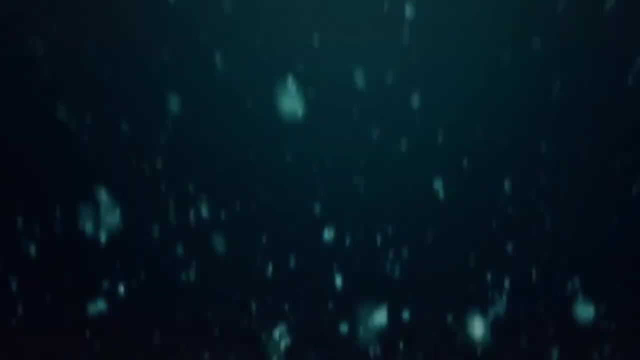 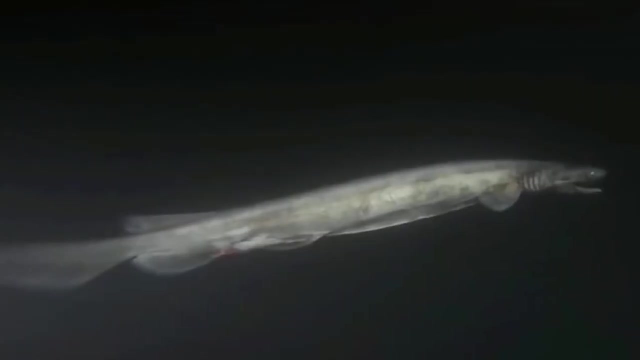 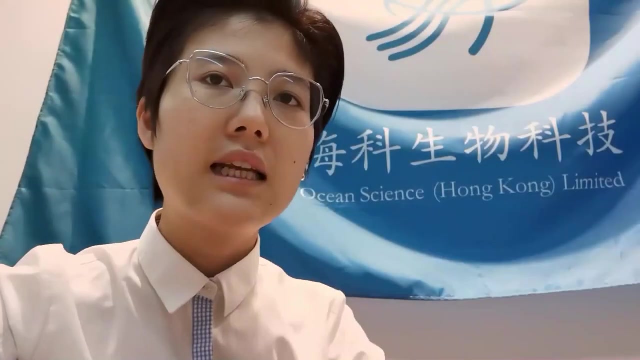 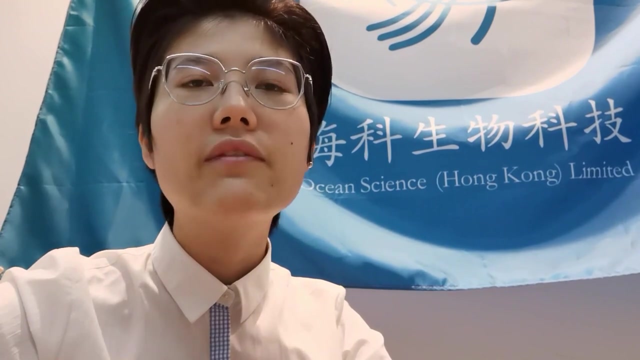 in which countless creatures live. Some of them are grotesque. Some have special lives. You may think their way of life is very different from that of life on the land, but they have many similarities. We know that land butterflies need to undergo abnormal development. 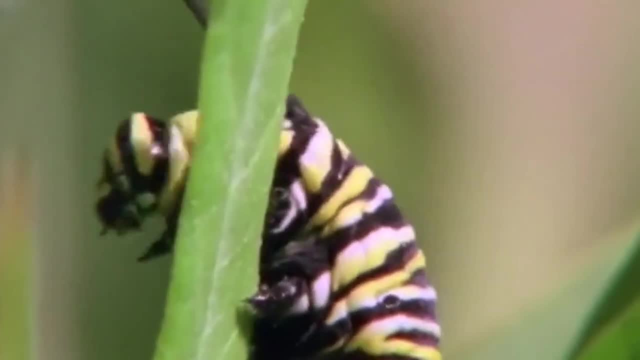 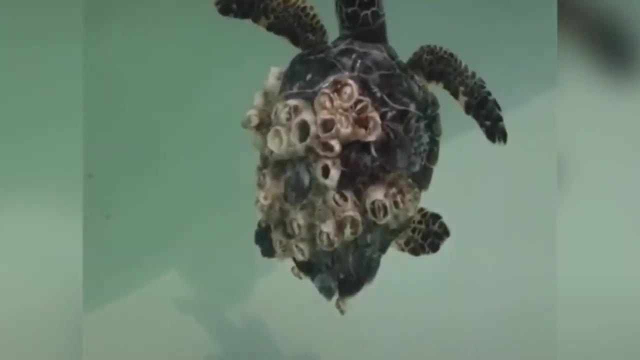 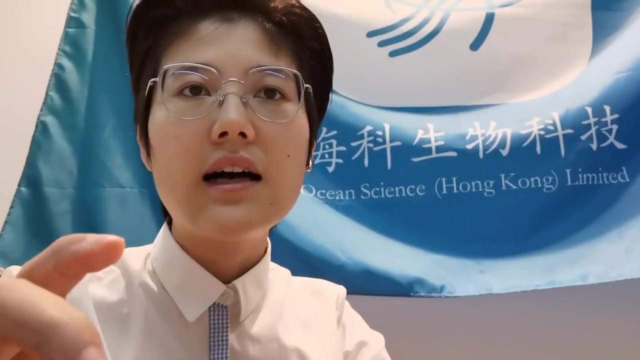 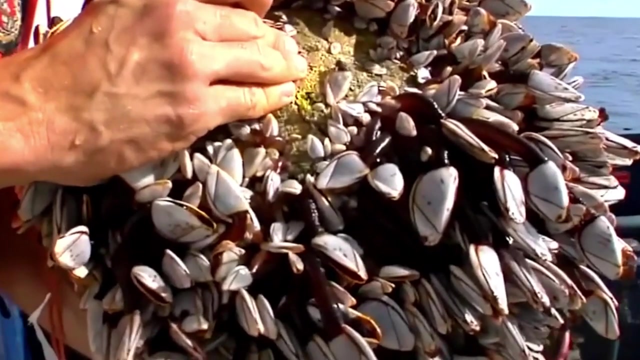 from caterpillars to chrysalides, to butterflies, And there are similar creatures in the ocean just like this, and this I don't mean the whales and turtles, but the hard little volcanoes attached to them. They are barnacles. 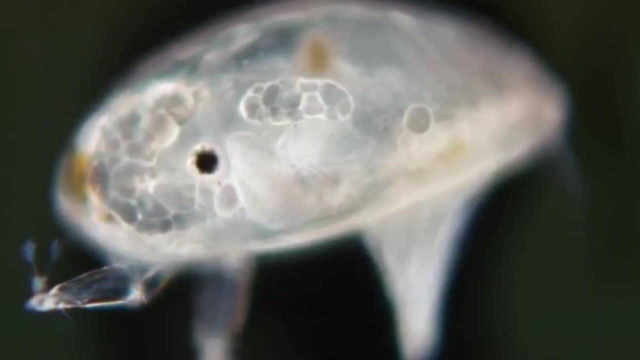 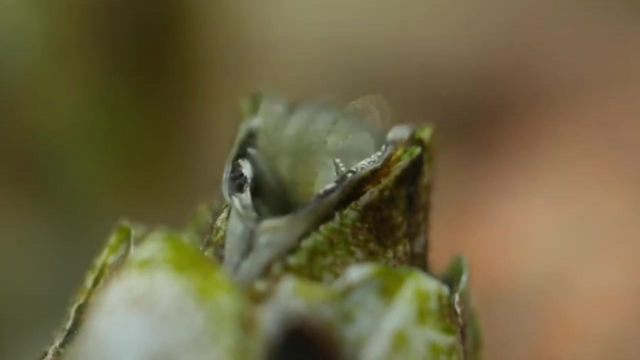 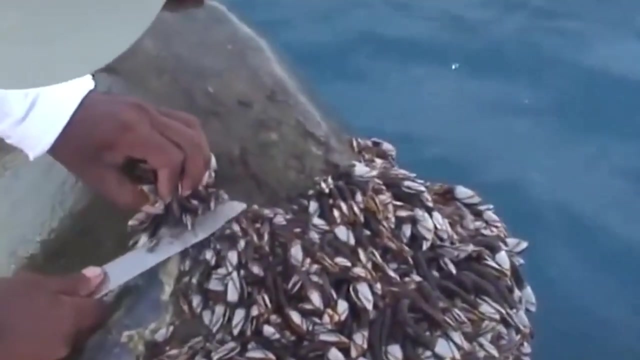 The larval barnacles are just worms. They are floating in the sea And then they were attached on some hard surface for abnormal development. However, this has brought a lot of troubles to the sea turtles. According to the research, barnacles are not the only one. 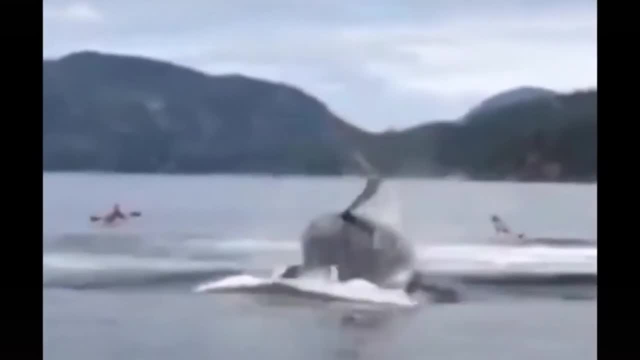 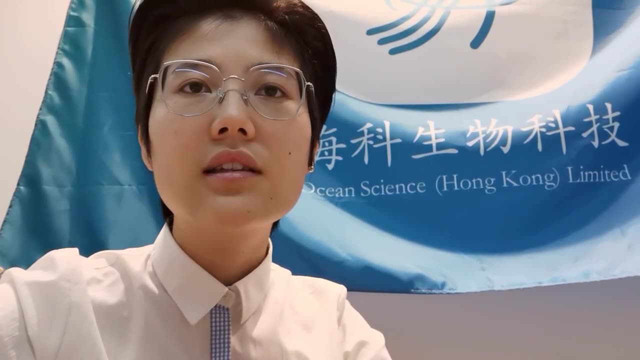 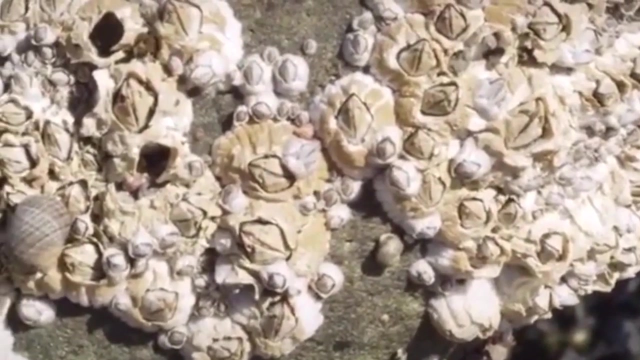 that's attached on the surface of other organisms. In fact, more than 4,500 different marine organisms have been found growing on the hard surface in the sea. We call them falling organisms. In addition to sea turtles and whales, the human marine facilities. 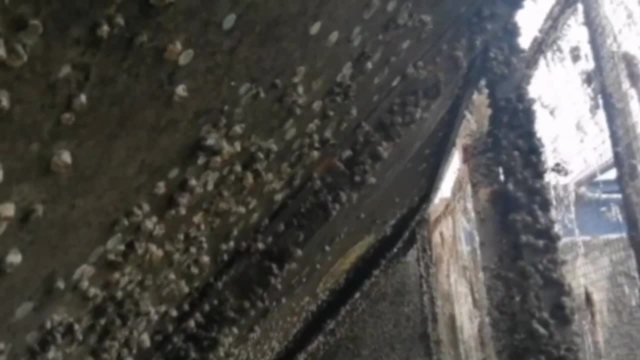 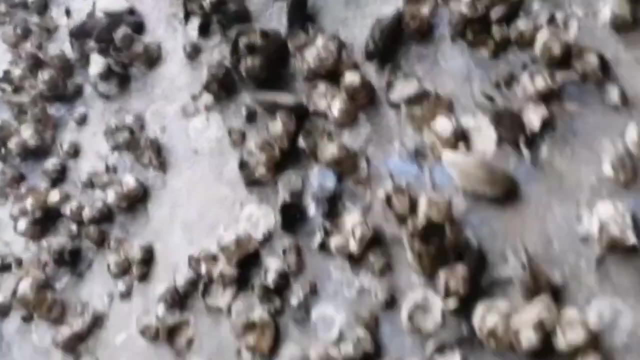 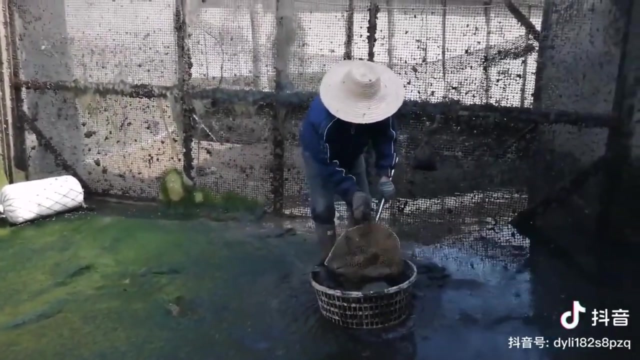 are also suitable for them to grow, such as the bottom of our ship, the inside and outside of the submarine pipeline, offshore construction projects, the camera and the fishing nets in the sea farms. So will the falling issue bring us any trouble? 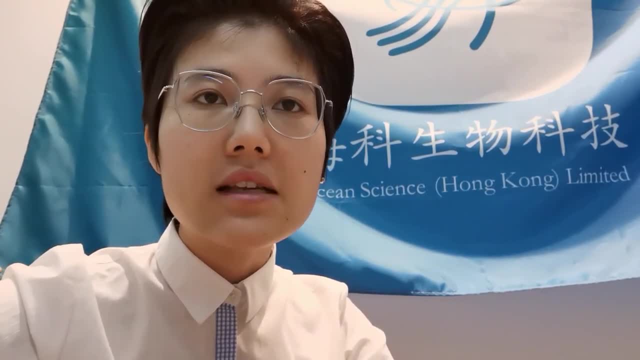 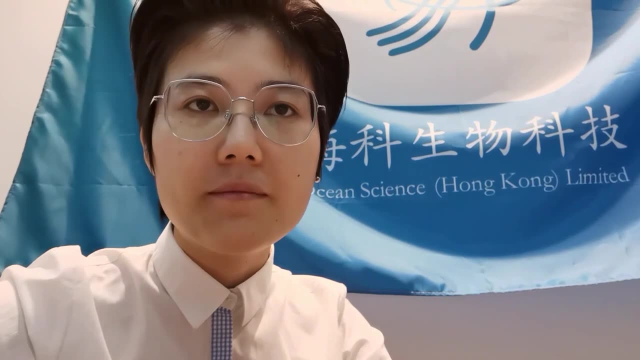 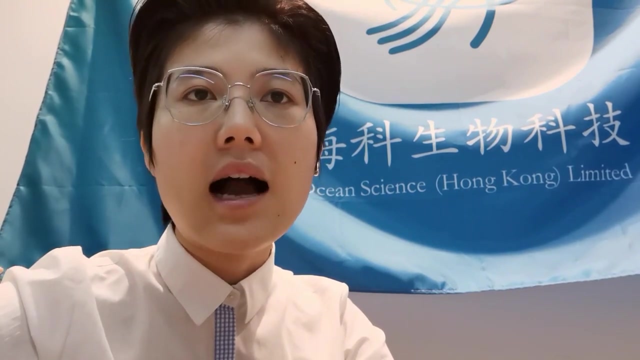 In fact, the direct economic losses caused by falling issues are as high as more than 27 billion US dollars per year. You may think this has nothing to do with you, but it is not. As long as there is falling, the ship will sink. 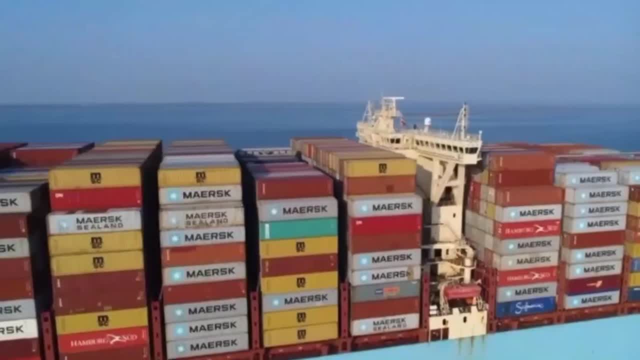 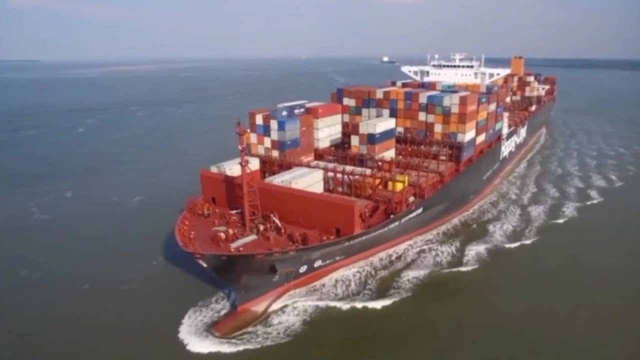 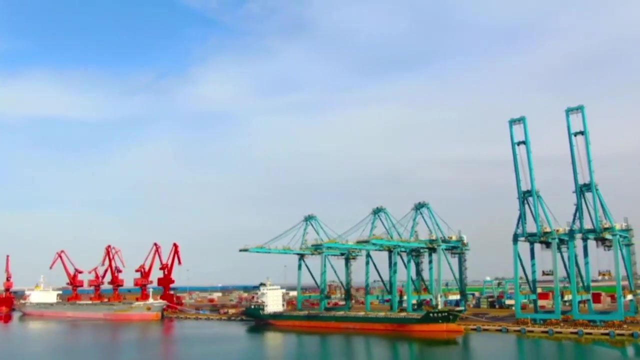 and the sealing resistance will increase. Thus, the ship will need to consume 40% more fuel. The ship owner will pass these expenses to the consumers in form of the goals and service. Therefore, the high prices of imported products are partly due to the falling issue. 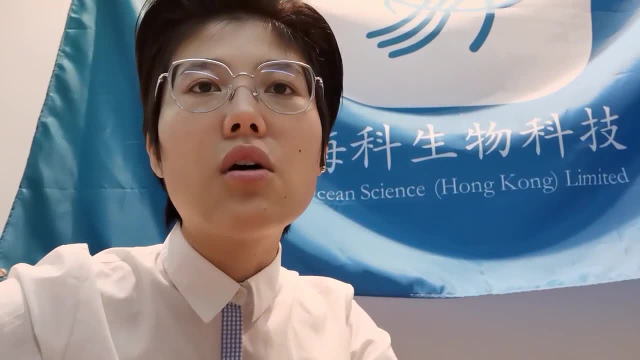 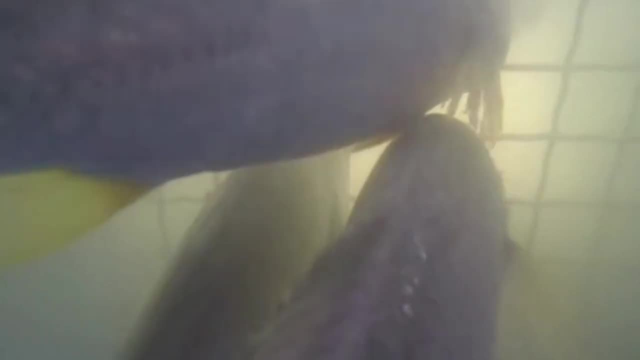 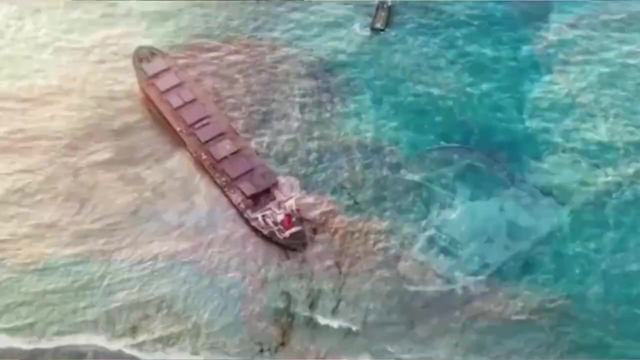 It is just an economic loss. So what about the health and safety? Falling spots can clog the nets of the sea farming and make fish sick from lack of oxygen. They also plug the pipeline and cause oil and nuclear leaks. No one wants. 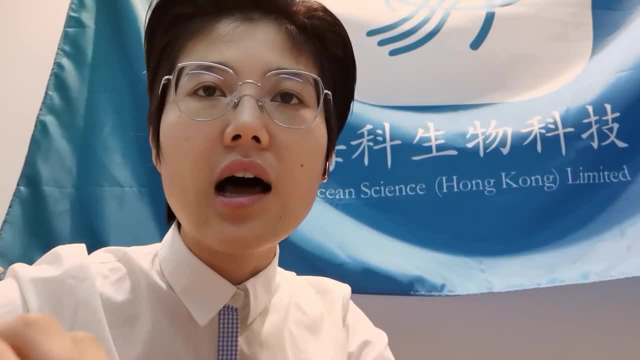 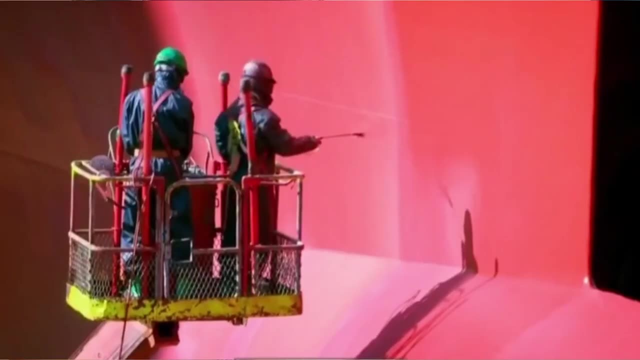 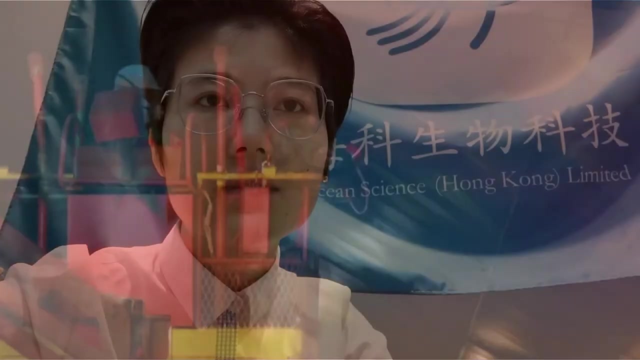 to go through this. So people have long invented anti-falling coating. Anti-falling coating can effectively reduce the falling issue. It is widely applied to the surface of a variety of marine facilities. So what is the principle of anti-falling coating? 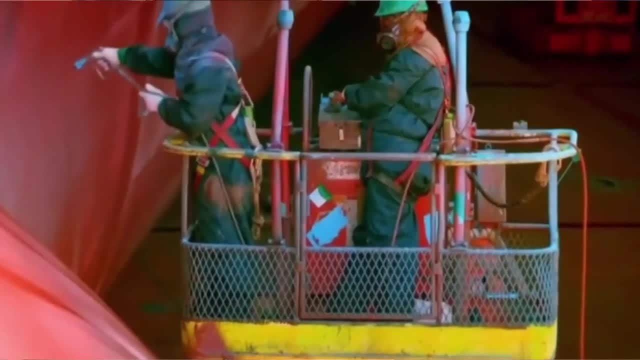 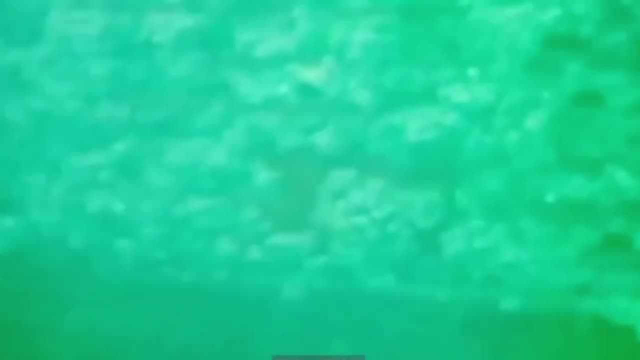 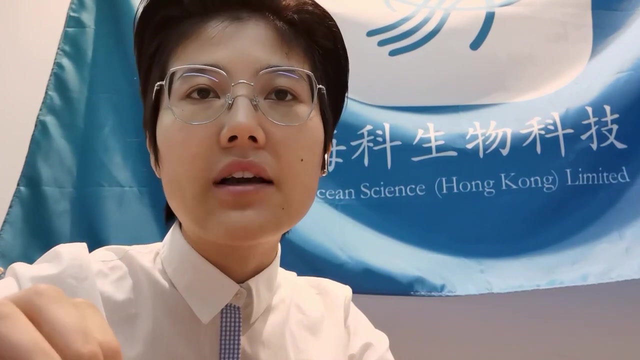 Poison and heavy metal. Yes, you heard right. In order to reduce the falling issue, humans have dropped large amounts of poison and heavy metal into the ocean. Over time, our ocean has been overwhelmed. Look at this conch Poison makes them. 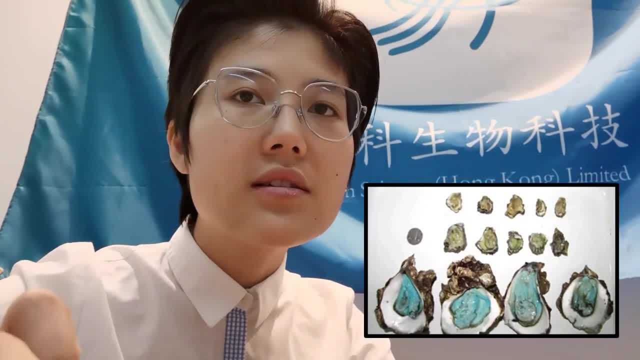 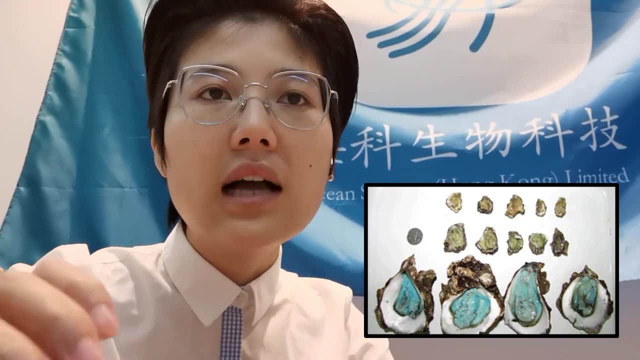 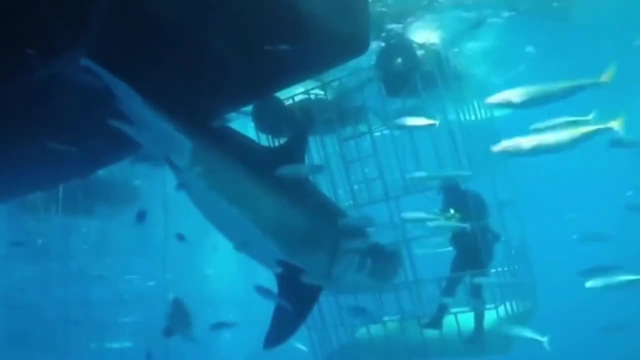 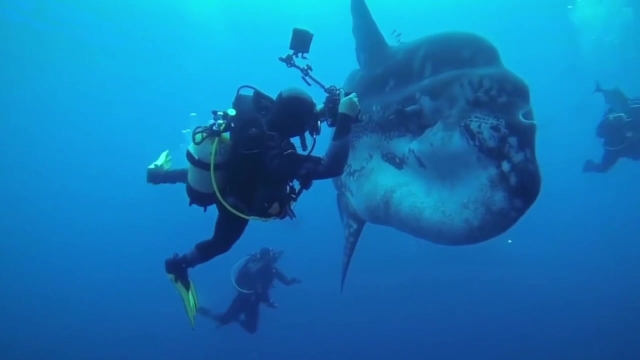 deformed or cancerous. And the blue oyster. they are beautiful but dangerous. We can't eat them. Their heavy metal content exists nearly 70 times. The influence of human beings on the ocean will return to human beings along with the marine ecological chain. 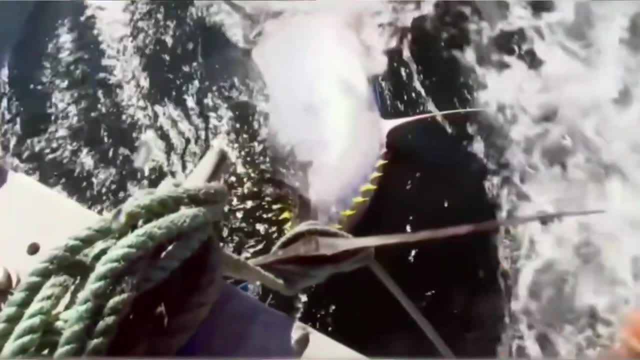 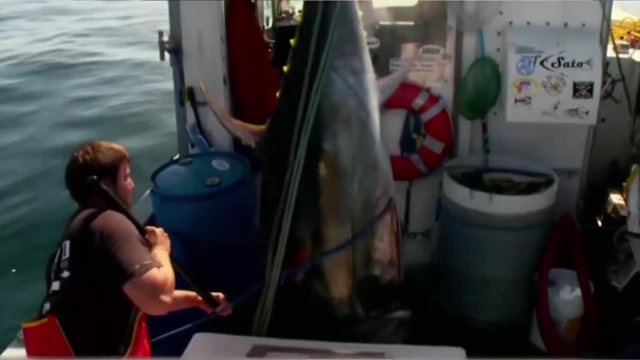 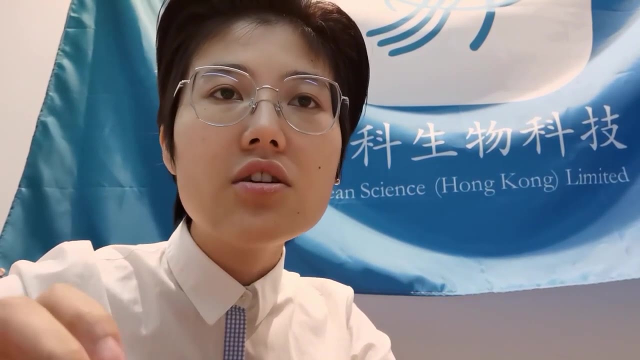 and food chain. We will eat nearly 15 million tons of fish every year And we need a safe ocean. However, according to the prediction of the IMO, the marine ecology will be completely destroyed in the next 40 years. People have long resisted. 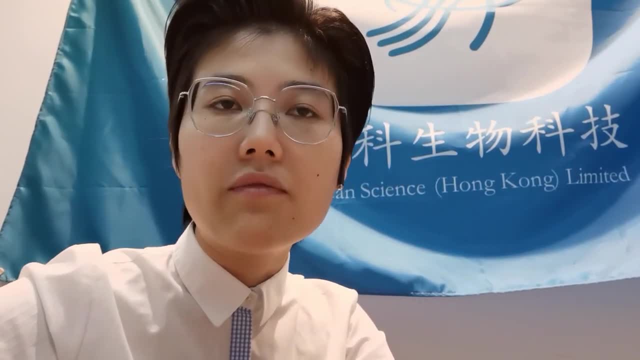 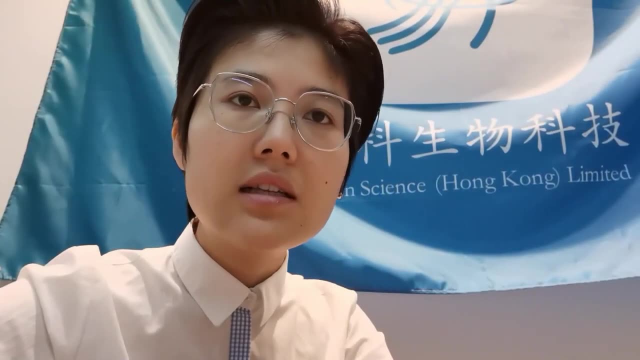 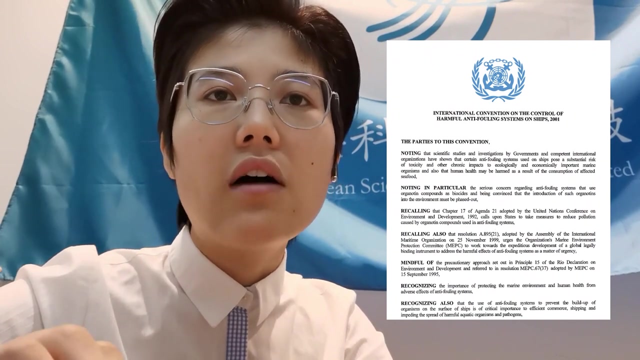 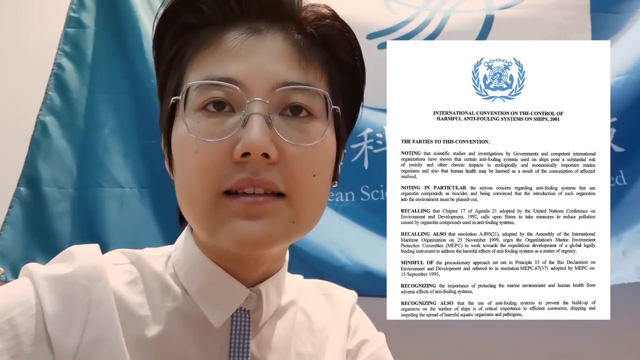 toxic and harmful technologies. A lot of marine personnel once held flags to protest. In October 2001,, IMO convened a conference to adopt the Convention on the Control of Harmful Antifouling Systems. Some toxic coatings containing TBT are banned. 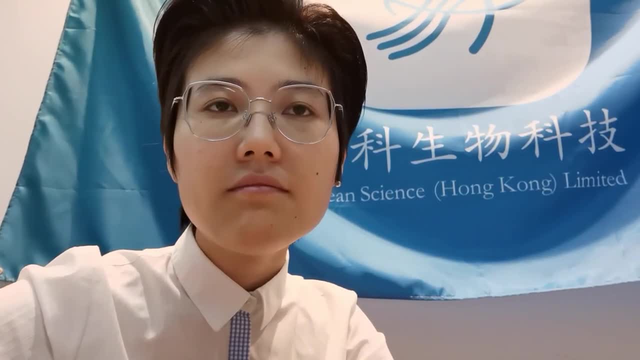 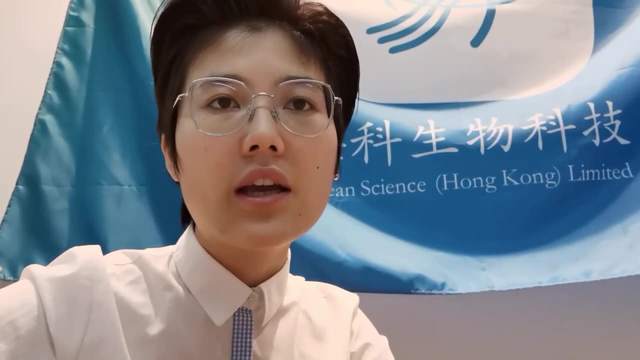 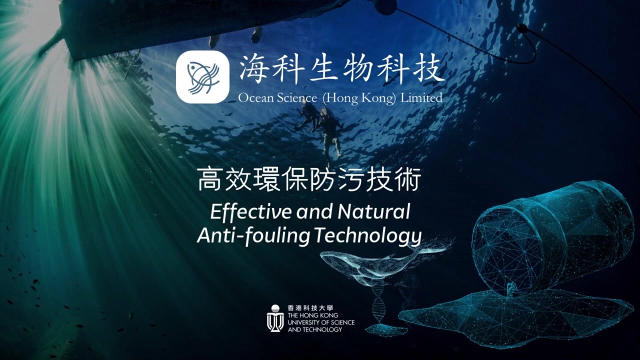 but others are still in use. The world is urgently looking for new environmental protection anti-fouling coating technology. So here we come. We are OSL Ocean Science Hong Kong Limited. We are from the team of the Professor Chen Peiyuan. 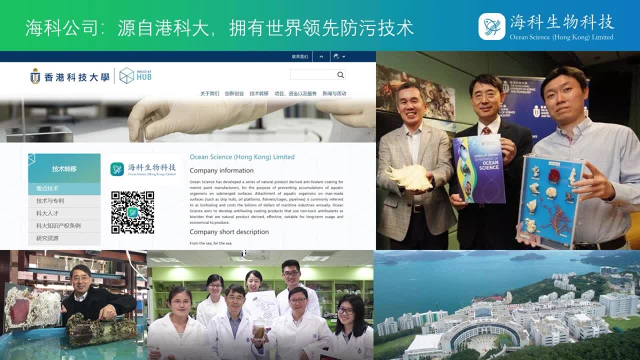 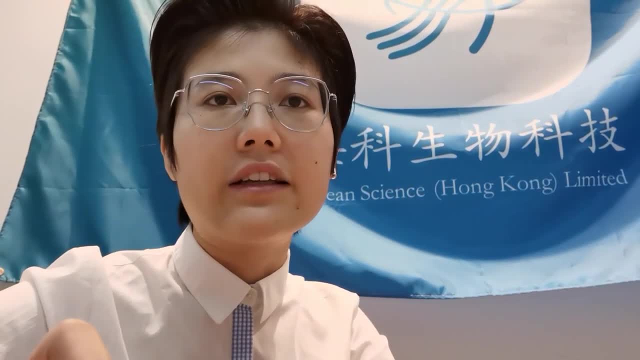 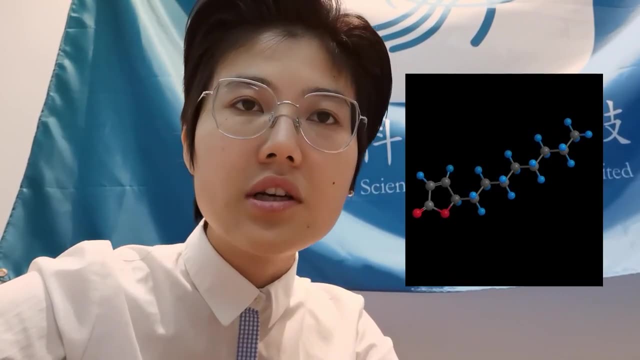 of Hong Kong University of Science and Technology. After 30 years explanation and research, we have finally found a green and natural way to expose the fouling organisms in the ocean. that is, to use biological signals to guide fouling organisms away from signal source. 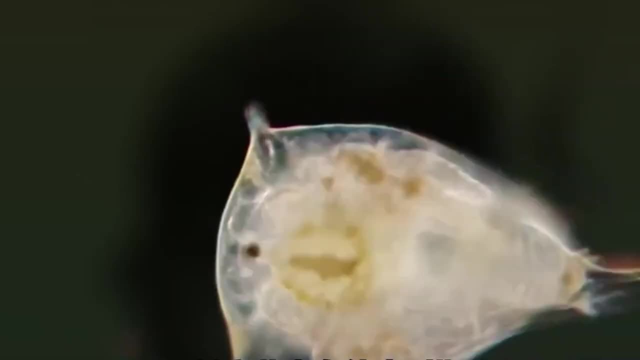 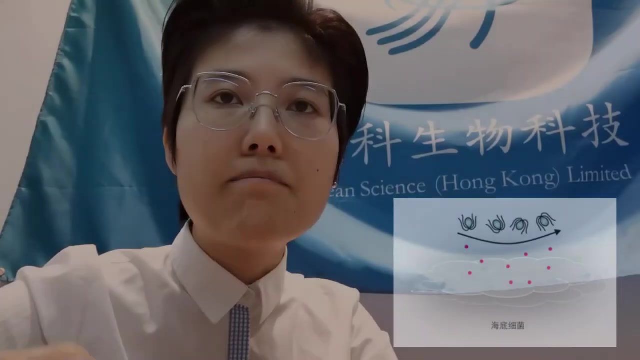 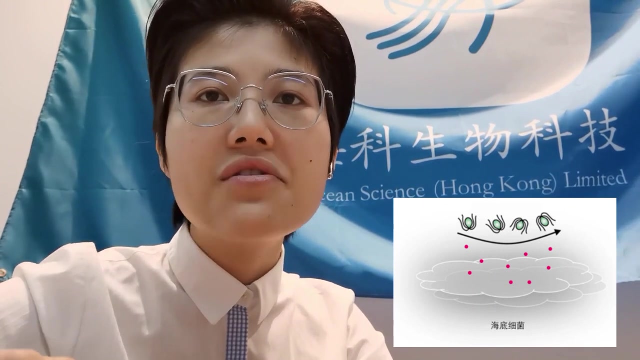 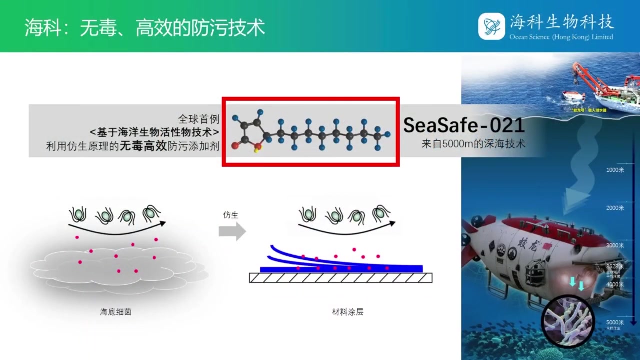 You may not have noticed that the resources in the ocean are very limited. In this competitive environment, some bacteria in the ocean will release some special biological signals to keep away other creatures in order not to be eaten by nature. We call these special biological signals. 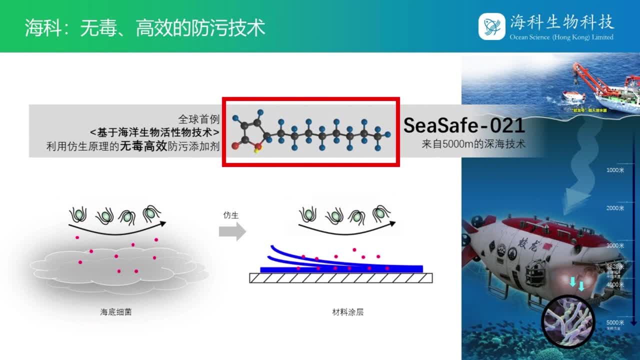 CCF021.. We use this biological competition mechanism to integrate CCF021 with coating technology so that our marine facilities can continuously release CCF021, like marine bacteria, so as to achieve harmless anti-fouling effects. About toxicity, we have conducted a large 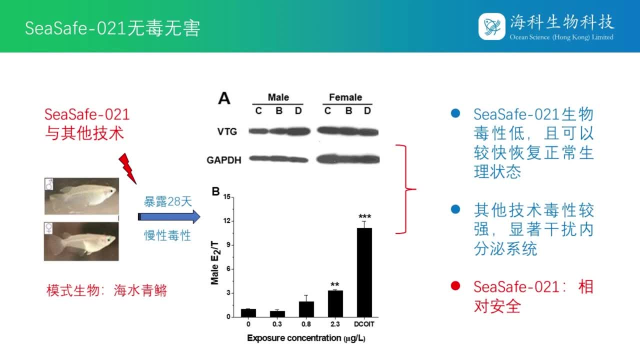 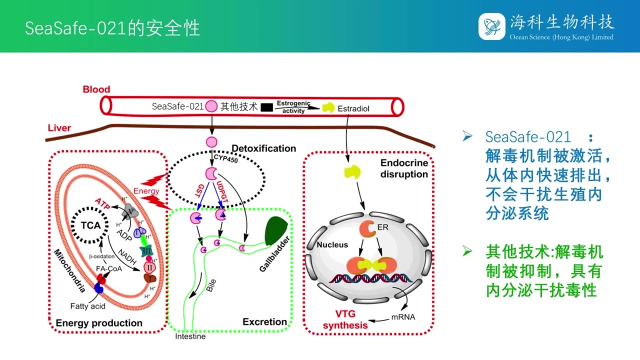 number of toxicity tests, and CCF021 is safe not only to the fouling organisms, but also to the fish: shrimp, crow, dolphin and so on. Even if CCF021 is ingested by marine organisms, it will be dangerous for marine organisms. 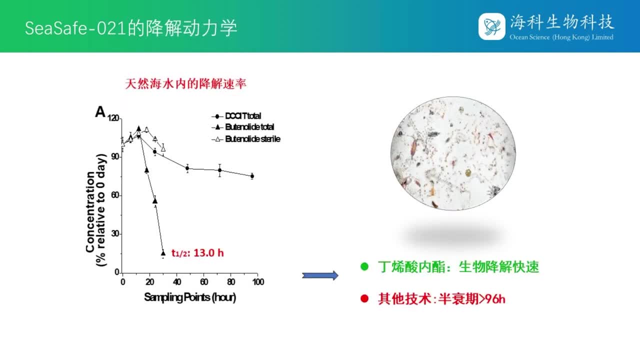 About environmental protection. we ingested the degradation connectivity test. We found that in natural sea water, CCF021 was rapidly biodegraded, with a half life of half day. CCF021 has a reduced persistence and accumulation in marine environments and play a good 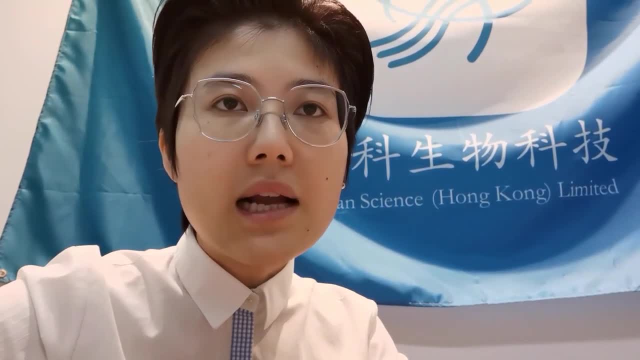 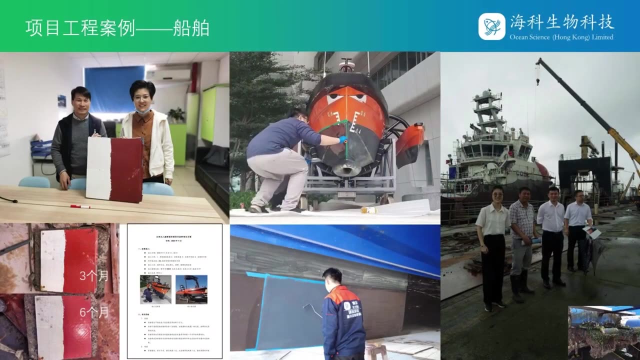 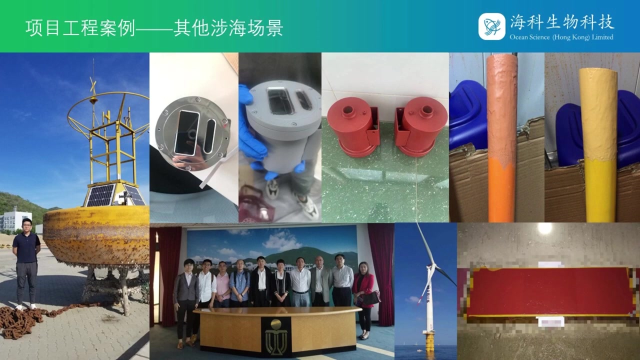 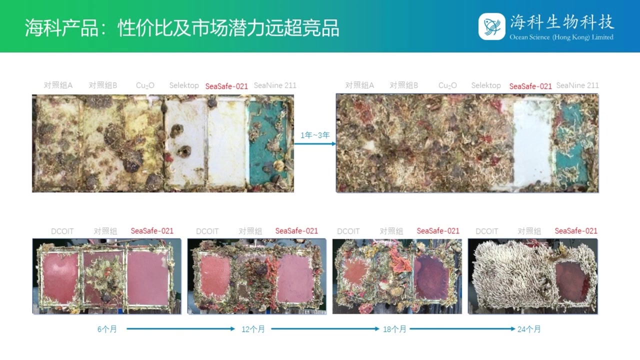 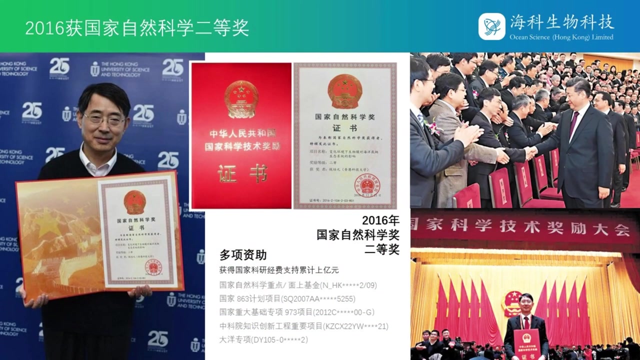 role in protecting the marine environment. At present, we have conducted a joint test with some partners using small boats, large ships, fish nets, underwater vessels and sea water. Comparing these pictures, CCF021 shows us excellent results. We are 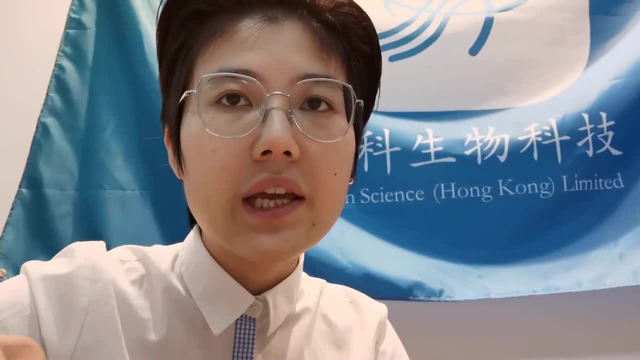 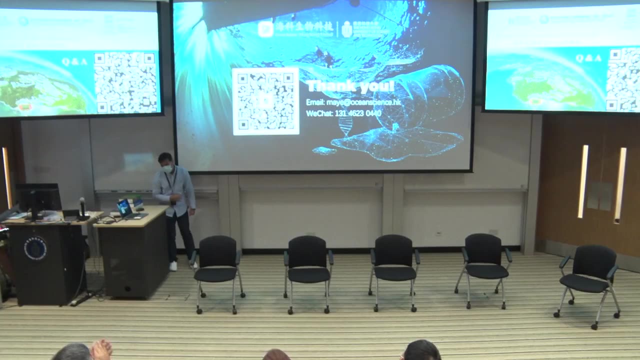 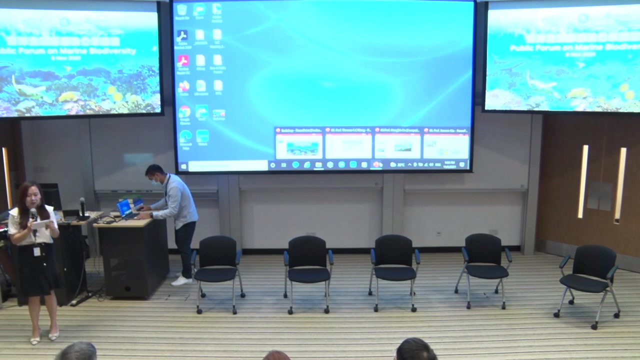 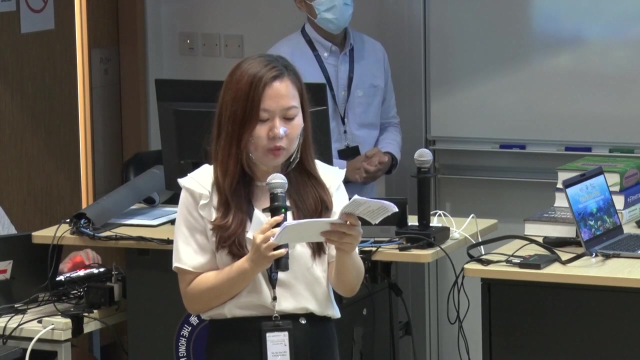 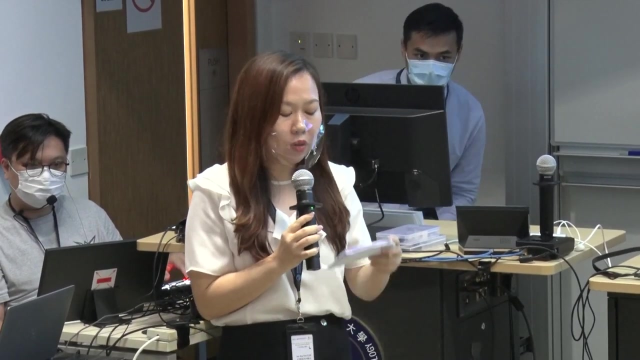 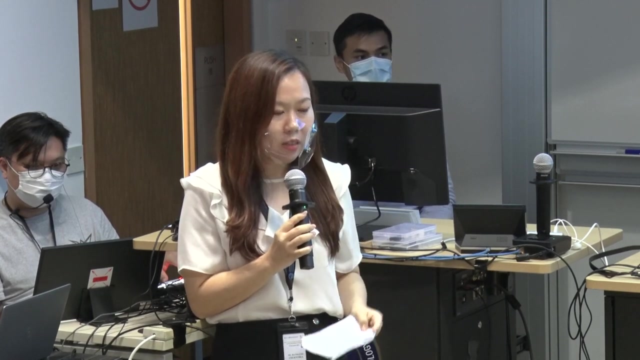 working hard to popularize this technology in different marine fields and hope that we can enjoy a chance to participate in discussions like this. Thank you very much. Thank you. This is a very special event. I would like to hear some questions from you. 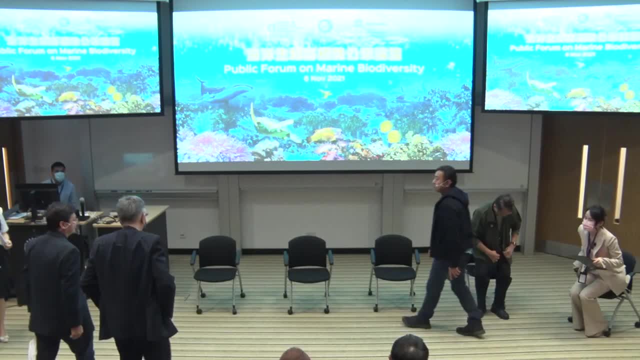 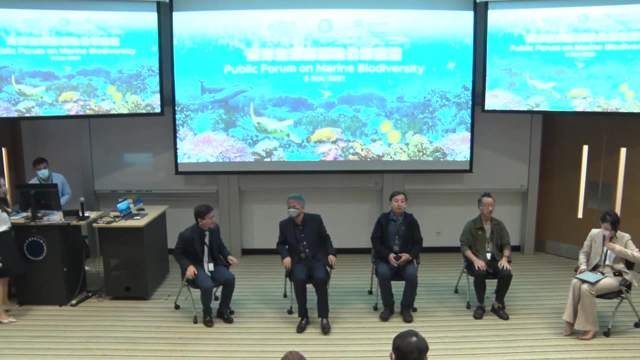 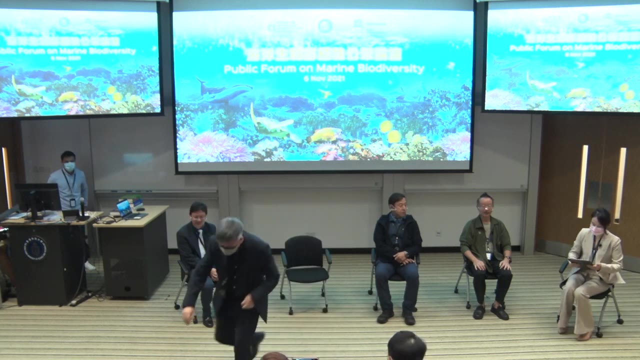 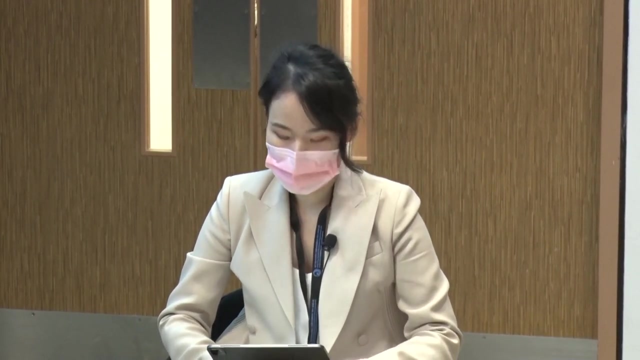 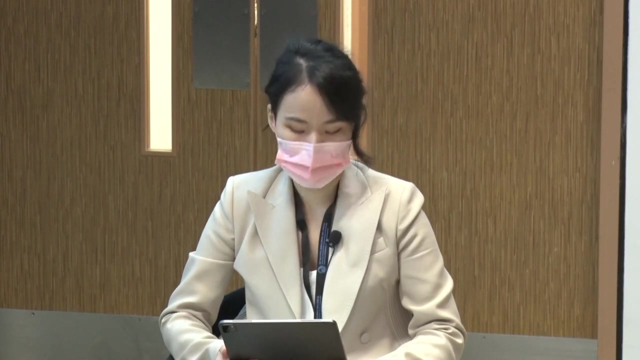 and check. Thank you very much, Yan. So we really appreciate audience continued support, both online and outside. So, before we start the first question, let us encode the theme of today's forum, which is the COP15- biodiversity- and also the COP26- climate change. 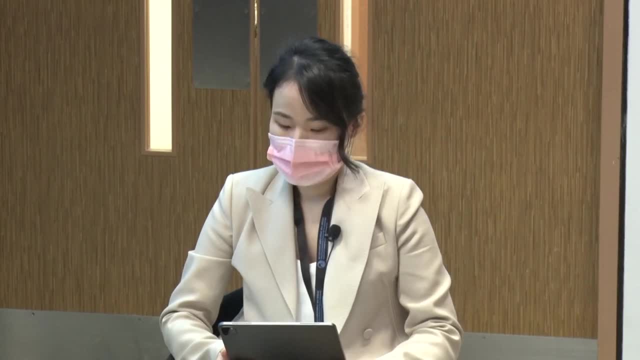 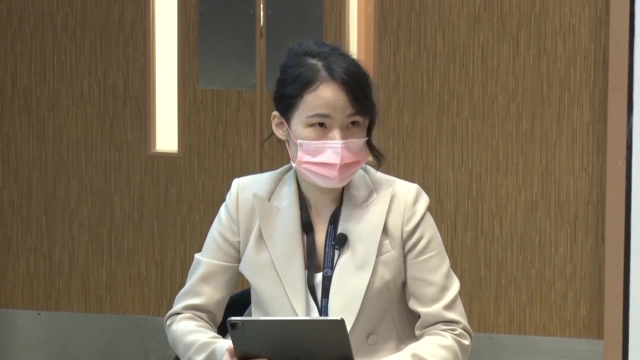 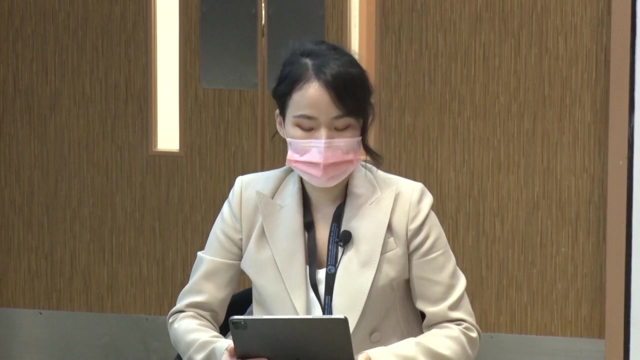 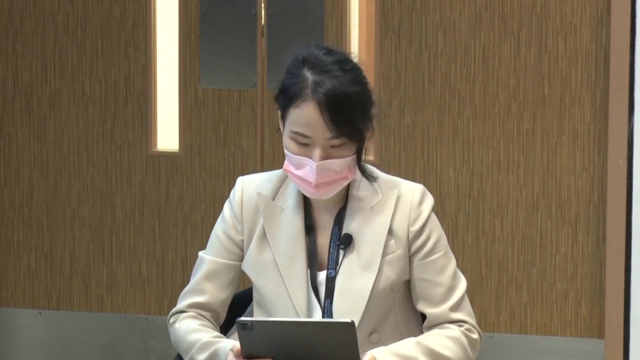 So the whole proposal of the COP15 is 30 by 30, a plan to conserve 30% lands and the sea areas by 2030.. So for the COP26 climate change In Glasgow, UK, now there are almost 80% world economy is covered by the net zero targets. 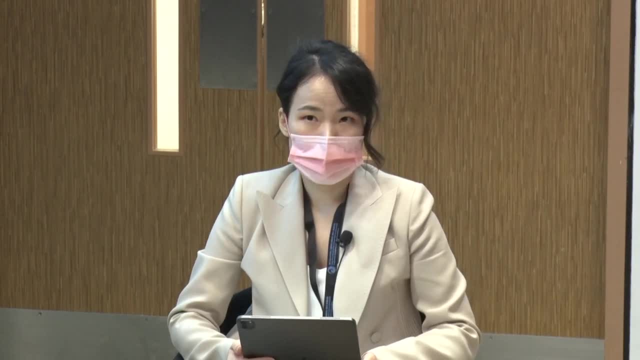 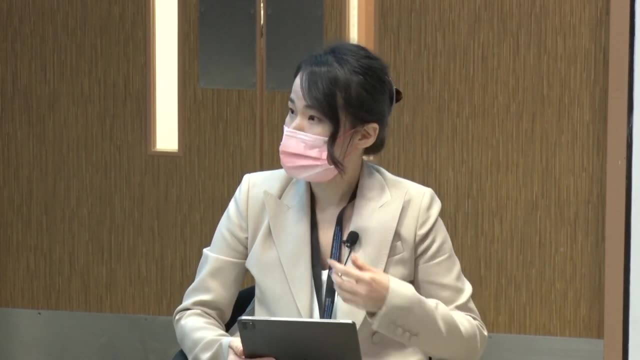 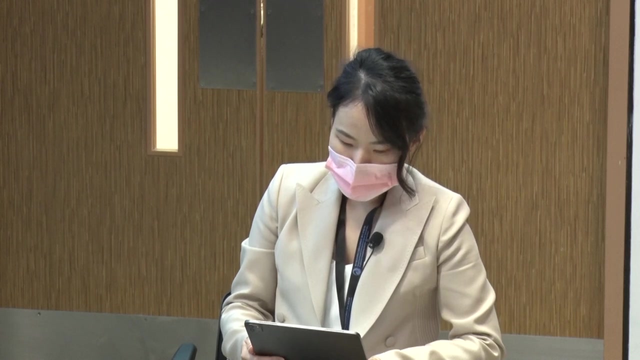 and the joint efforts to reduce the global warming to the 1.5 degree. So the first round warm up question is regarding the both global initiatives. So which excellent action will you suggest In terms of infrastructure? we think it's going to be very, very good. 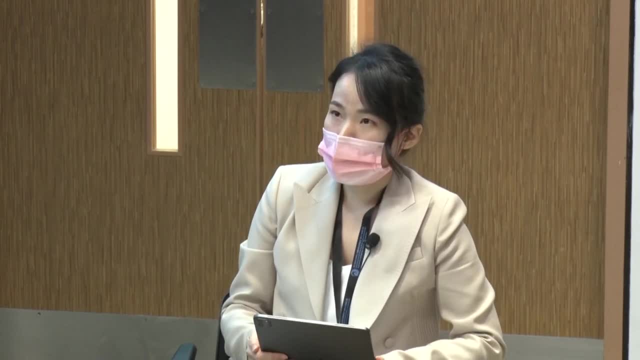 We think it's going to be really good. We think it's going to be very, very good, But we know it's not gonna be new. So we are really interested in the future. We're not even sure. We are very interested in having some kind of a pretty new policy, maybe a party where we're actually going to have some kind of a new approach to the data. So it's going to be a very, very good way, because we really believe that we have to really constructive policy and really want to get to know more about the data and also. 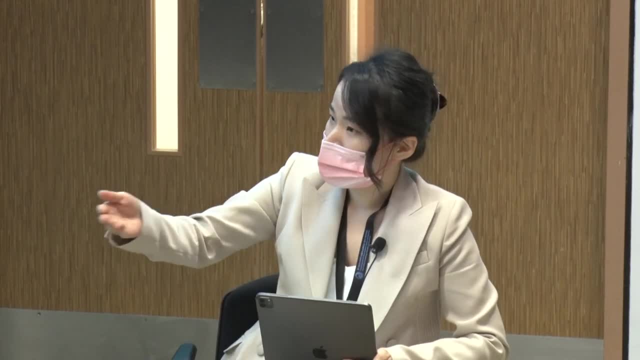 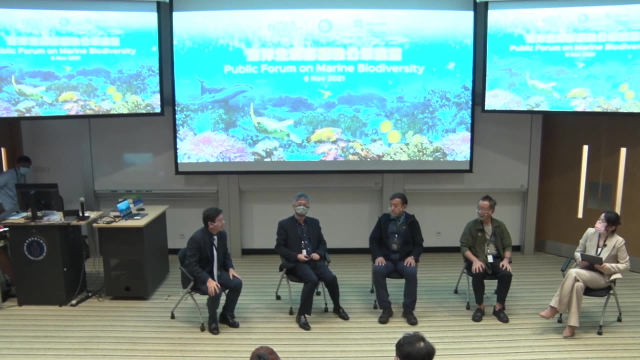 for the environmental impact and also to have some sort of a good public policy and the kind of measures that we can introduce that we need to make and also also to make improvements to the document. So we are very, very interested in that, Professor Cho, starting from you. biodiversity data. 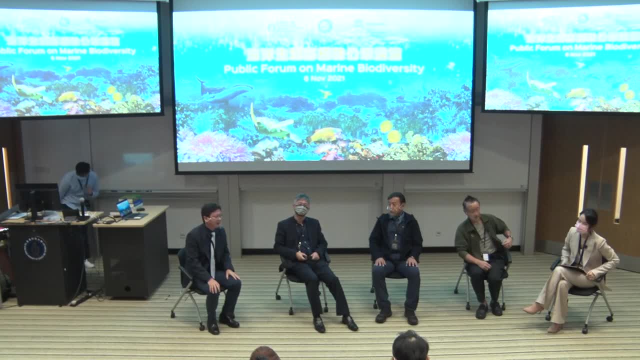 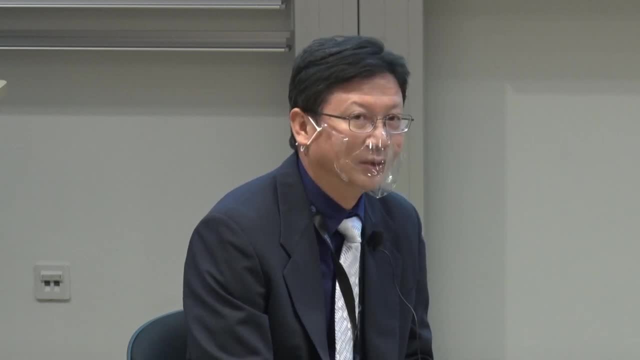 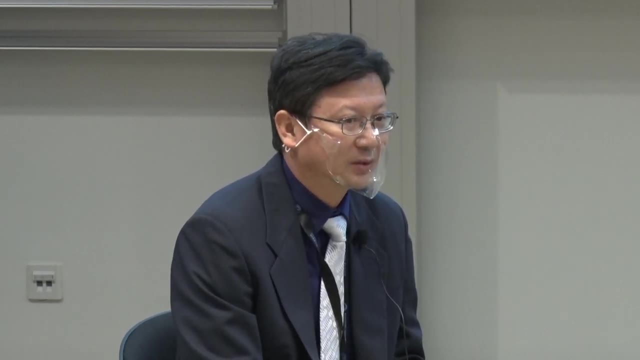 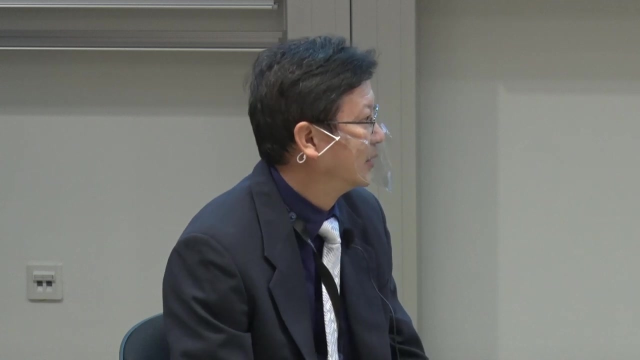 Regarding the sharing of biodiversity data, I think there are some mechanisms allowing you to share the biodiversity data. For instance, I know for some group of animals those data are widely available. For instance, in Hong Kong we have Hong Kong fishnet. although I don't do fish, 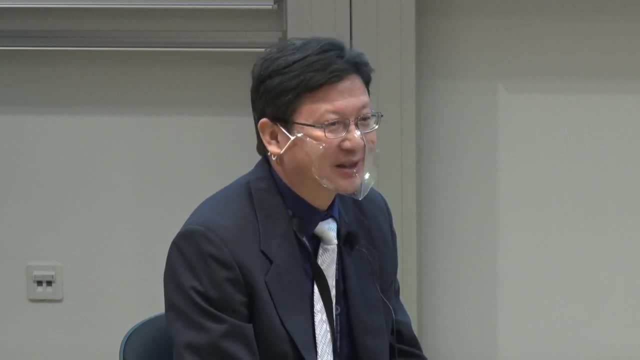 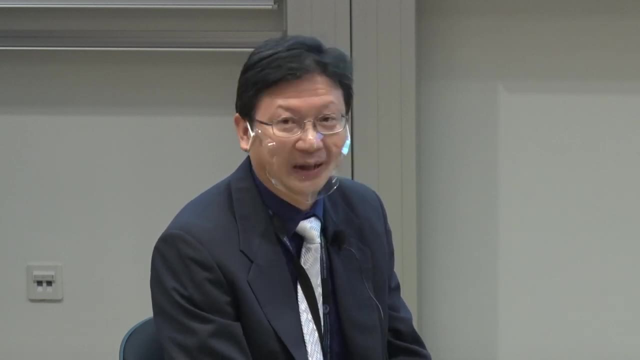 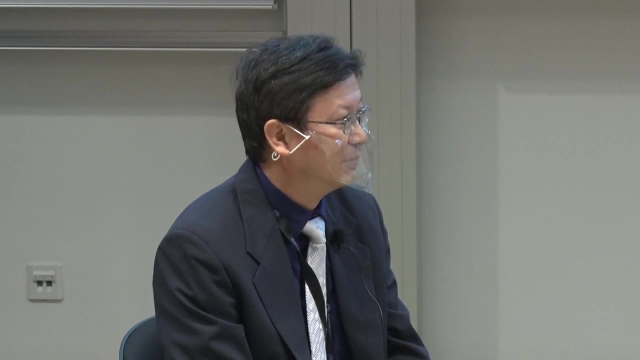 I know, For this kind of animals we have a very good data base, But for some animals we don't even know their existence. So I think more research should be done and more incentives should be provided for young people to go into this field. 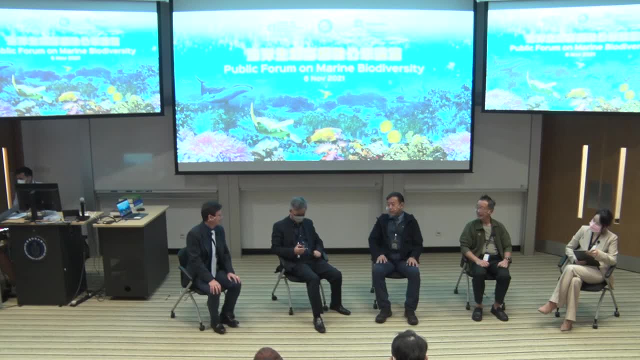 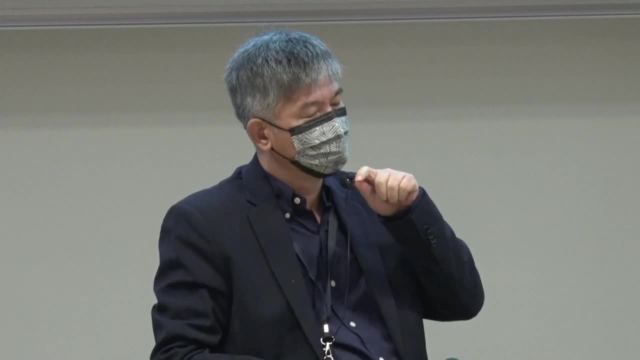 So, Professor Liu, do you want to? And some remarks. I do not have much to add. As Professor Chu mentioned, there are probably no centralized ones, but I know there are lots of different websites that host those data, For example for proteases. 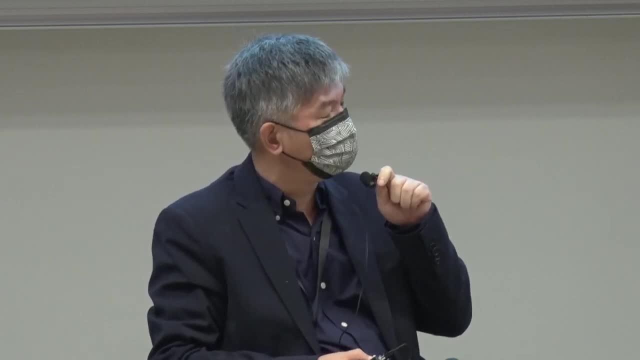 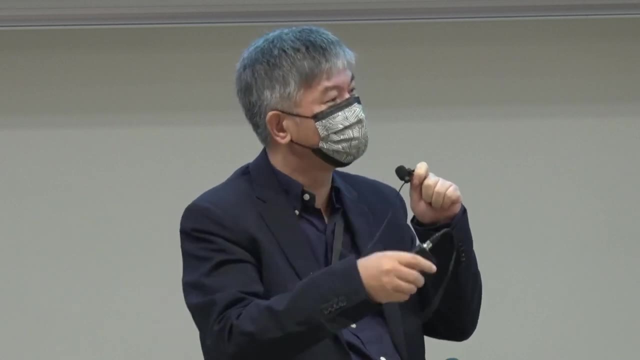 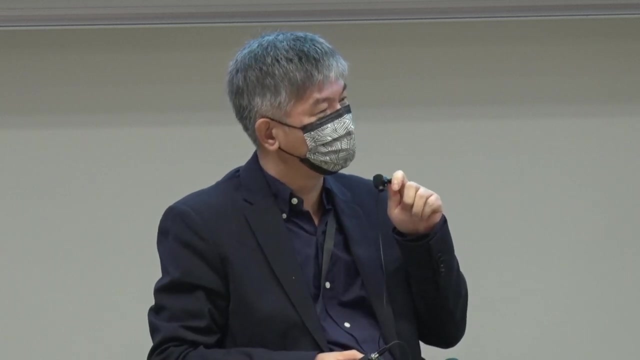 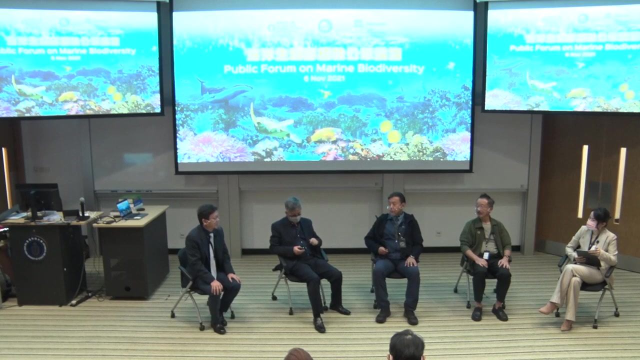 Sunweibo. they have this global kind of sensors, many, many, And for species, everyone can add to it, And for genetic obviously there's a deposition, So all kind of a variable there. Yeah, I want to add regarding the marine species: 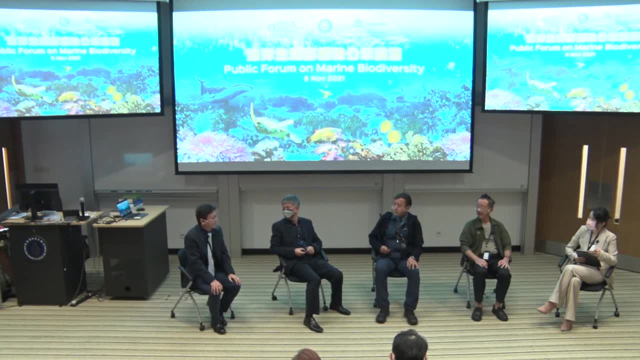 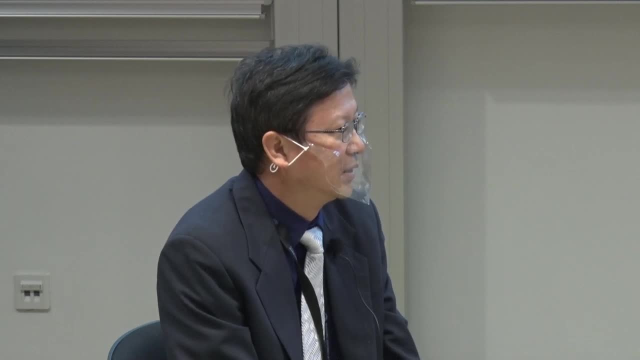 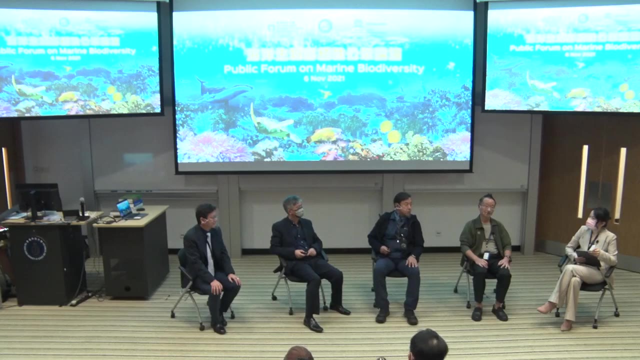 we do have Hong Kong marine species database, So that's why we know Hong Kong. in Hong Kong, there are roughly 6,000 marine species. How about you, Professor Chu? Yes, In my understanding, I think I very agree with the previous professors. 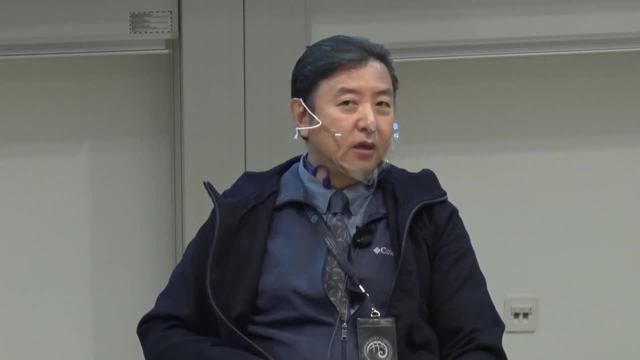 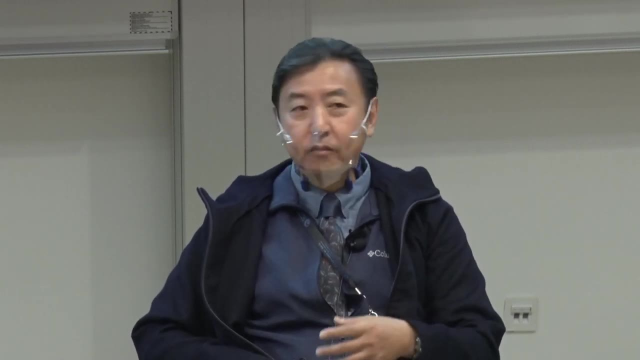 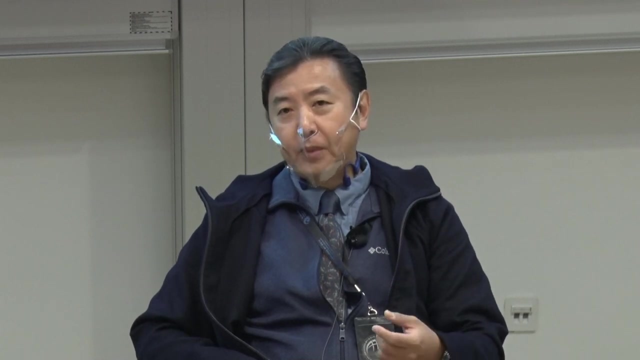 And also about the organism. it's not very simple. You know, we're talking about the taxonomy and also distribution of that, Yeah, And also, of course, their habits and life cycles and so on and so forth. So just like, for instance, we have a fish base developed, 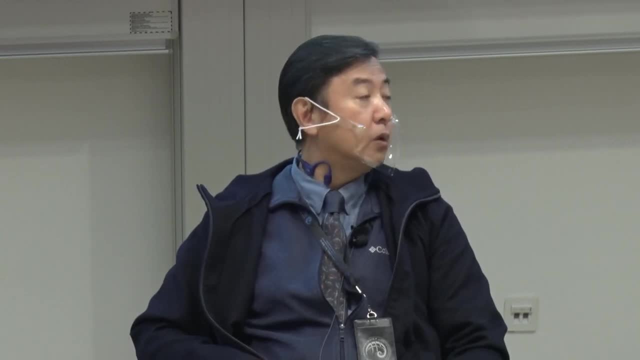 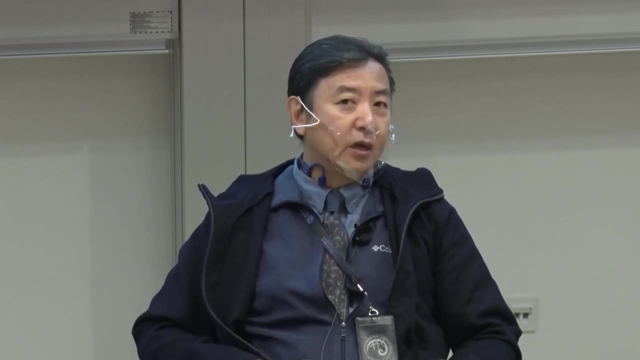 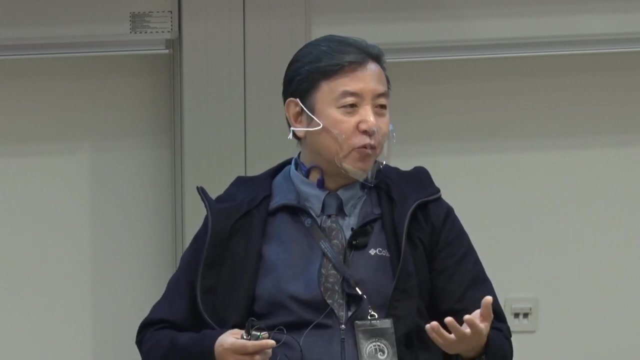 more than decades ago And I see we are all making efforts to improve that And they also. you know these are huge work. It's not only about the generalization, Right, Yeah, There are also some, you know just my work, like taxonomy, the classification, 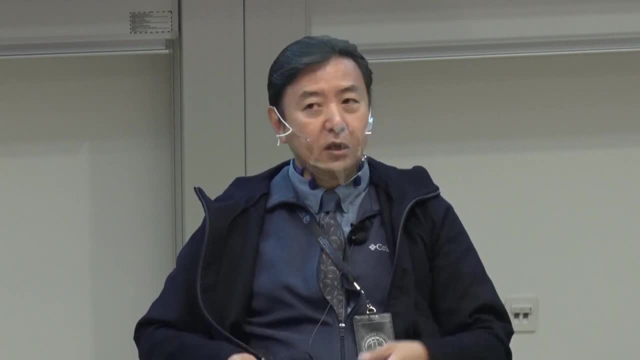 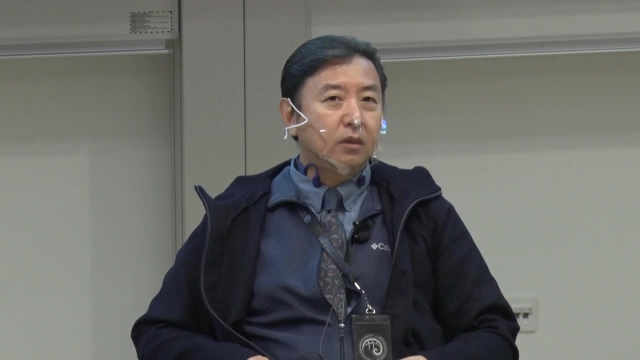 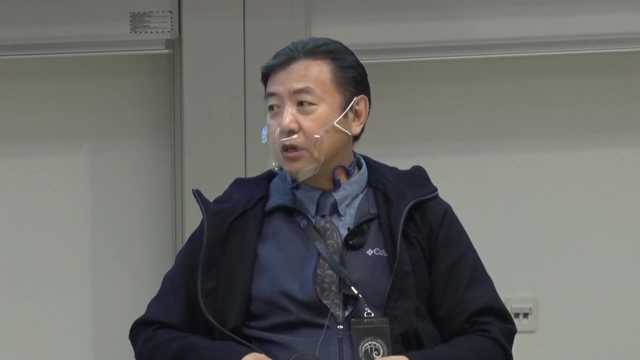 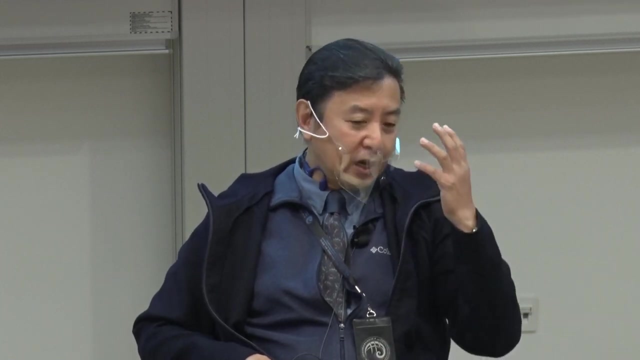 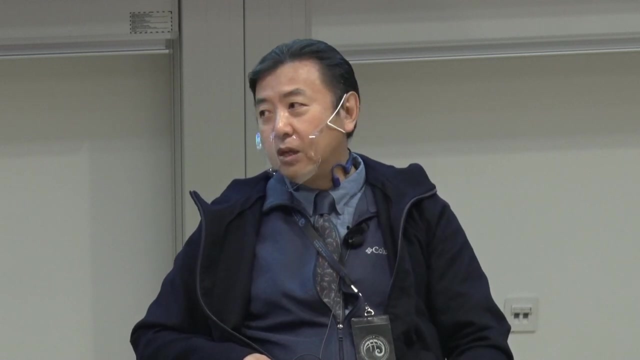 It's also about the ecology. So lots and lots of baseline data we need, And also we would like to have more interns and also those students involved in this area, And then also the knowledge. it covers huge subjects, So we have to combine the technology and so on, and so 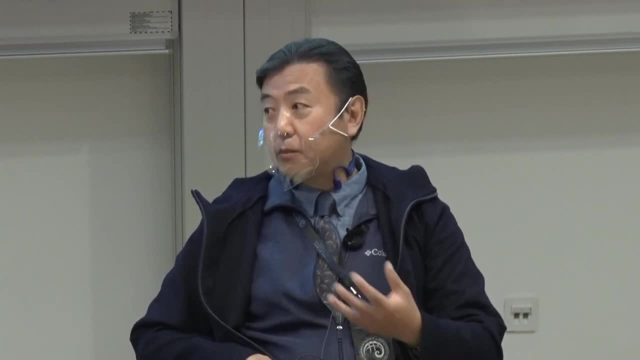 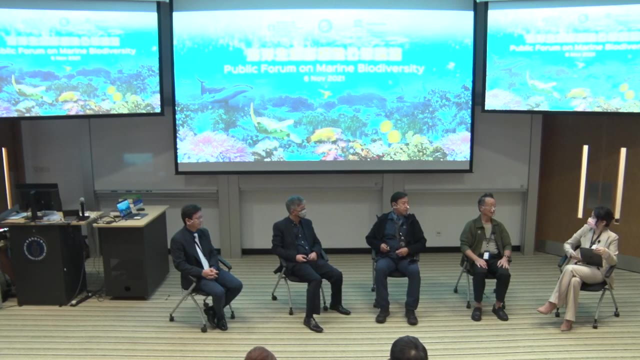 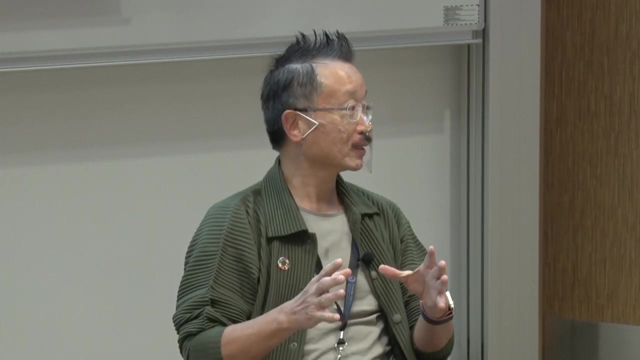 forth. So I think all the universities and also the collaborations of broad industries will be expected. Thank you, Do you want to add something Please? Yes, Emma, Thank you. To me the answer is as simple as ABC, But A stands for artificial intelligence. 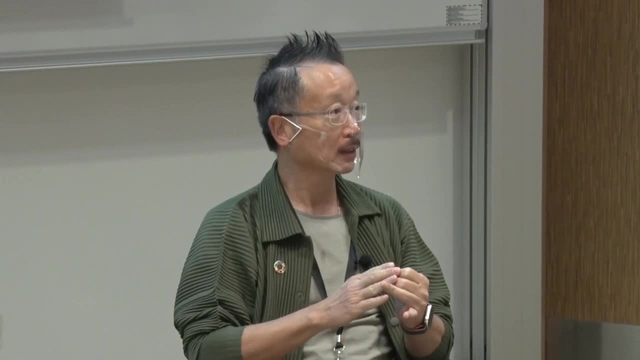 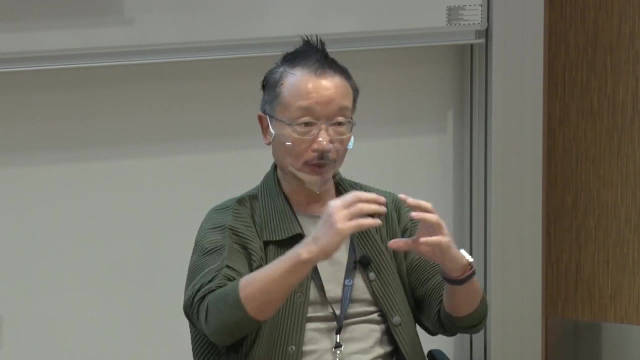 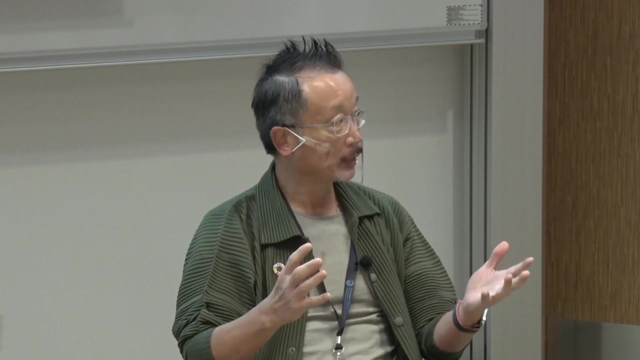 B stands for big data, C stands for cloud-based. So what do I mean? First of all, we need to get even more dimension to our data, not just one or two dimensions, but as many dimensions as possible. But how do we get all this data? AI, artificial intelligence. 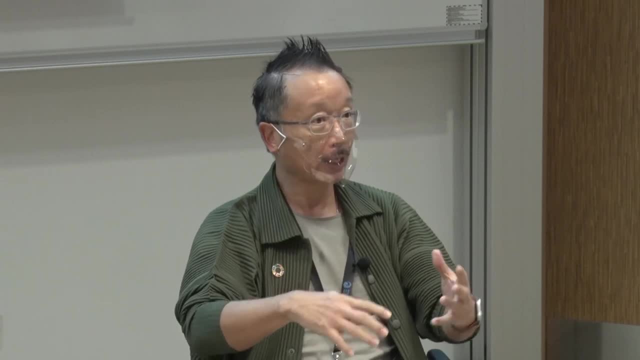 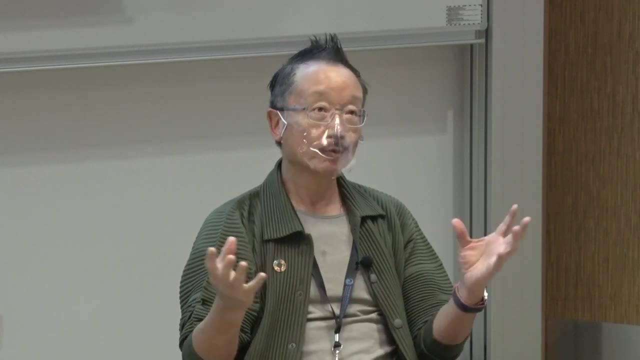 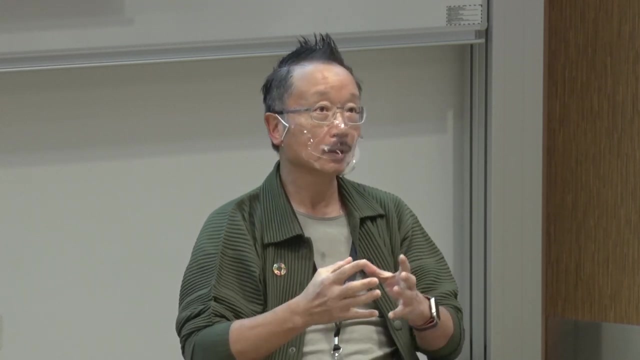 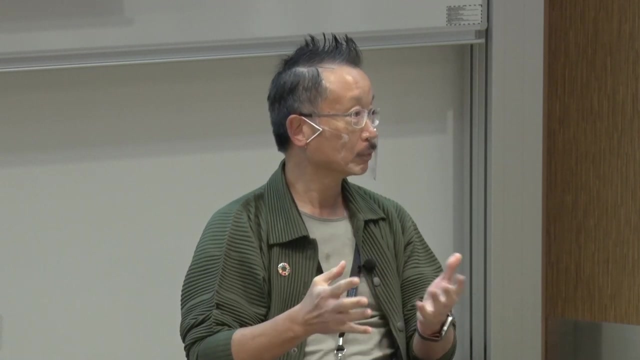 So maybe we'll be talking about robots in all levels of the marine life. After we collect all this data with scientists, with researchers, they will be able to give us more information about marine life And with that we'll be knowing more and therefore we 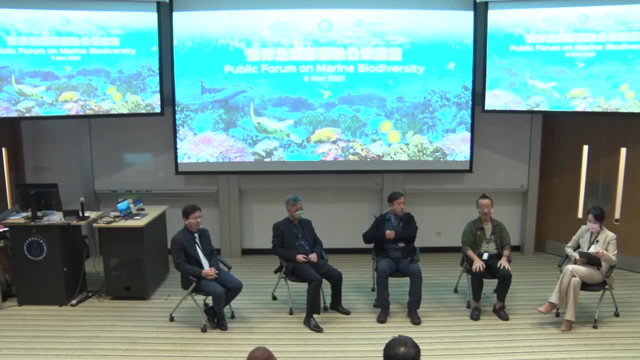 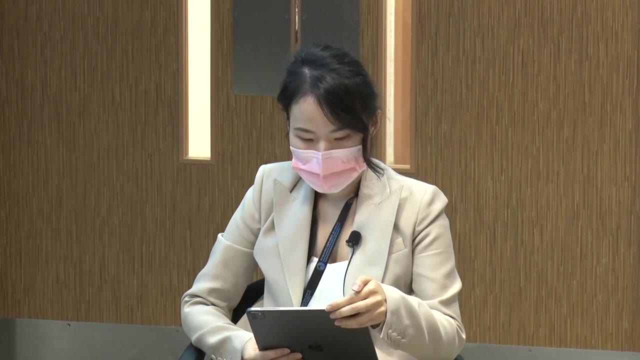 know what to do Next. Thank you, Yeah, I totally agree with your remarks here. So we received a couple of questions from our audience. So the first question is to Professor Thomas Wong. So we know that you have extensive working experience in the business world. 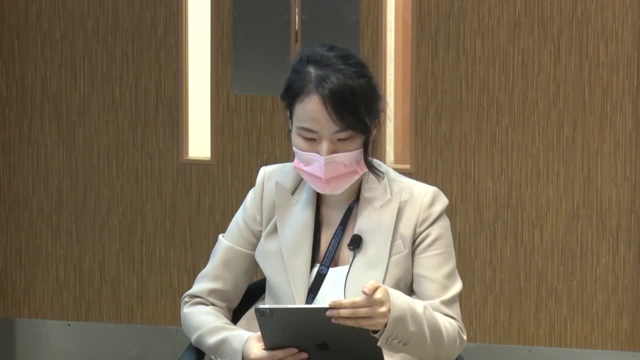 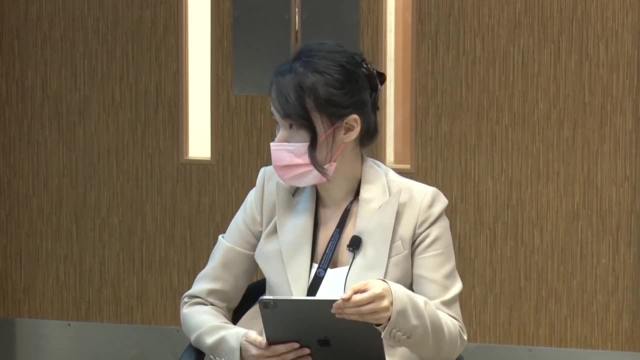 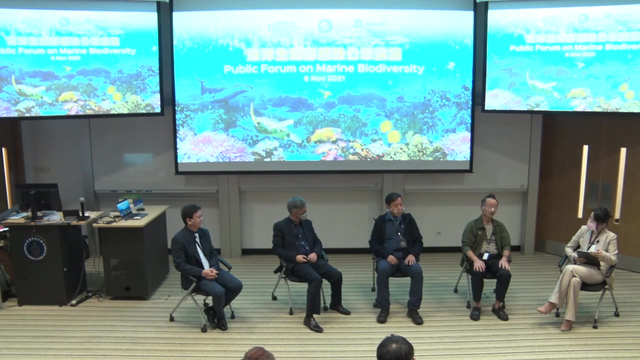 So how to balance the ecological value and economic value for those small median enterprises, especially for them? they don't have the pressure for releasing the environmental social governance report, So may I have your opinions on that? Yes, I can give you an example. 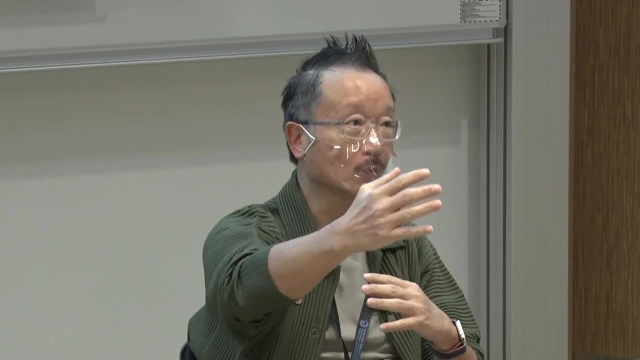 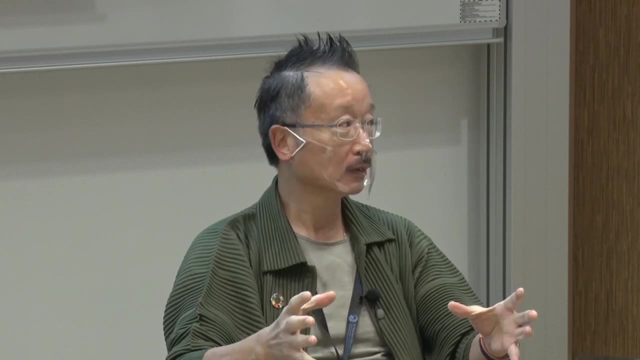 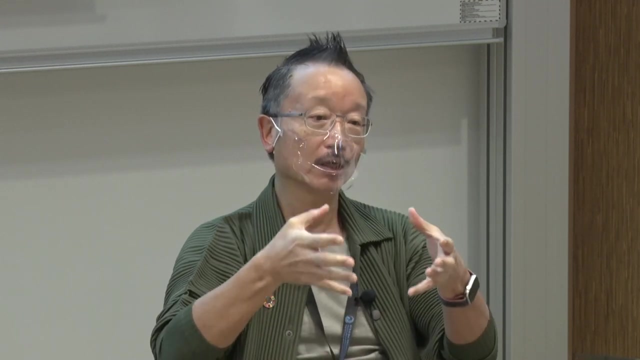 For example, if we want to travel to somewhere, to go to a destination, you can have the most beautiful car in front of you, But if you don't have an engine inside a car, I'm sorry, You're not going anywhere And business is like the engine of the car. 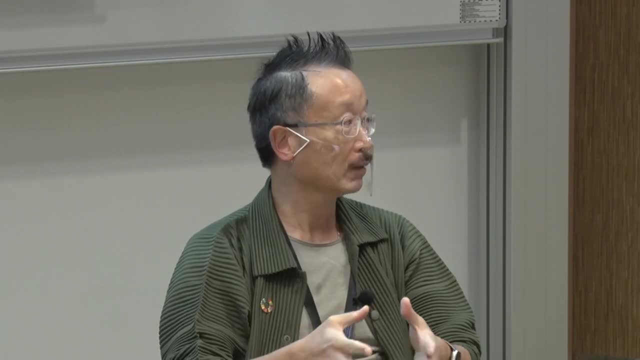 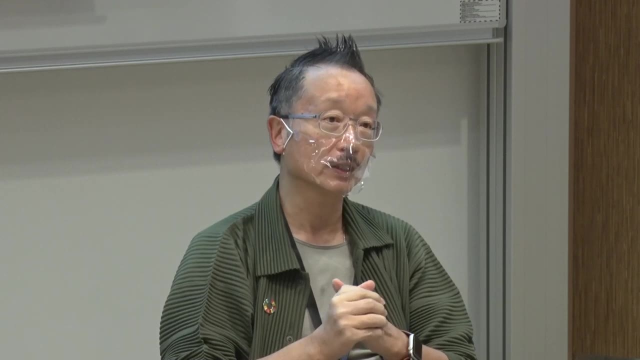 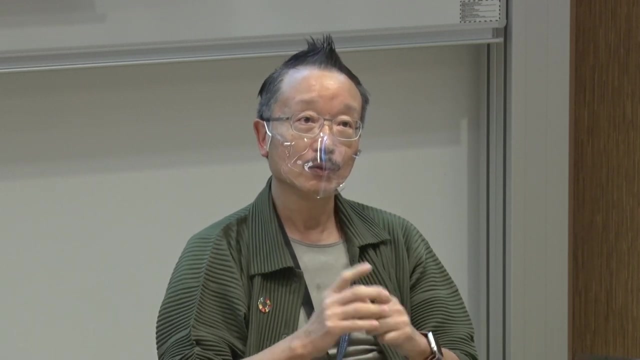 And SMEs. for example, in Hong Kong, 90% of the companies are SMEs, So SMEs are the engines. That is one thing, And the second thing I also want to mention is because I start with destination. destination is very important. 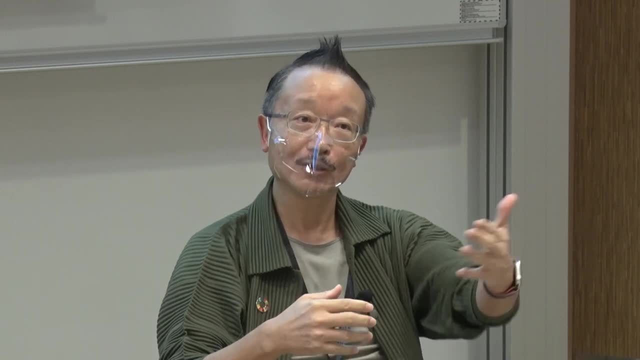 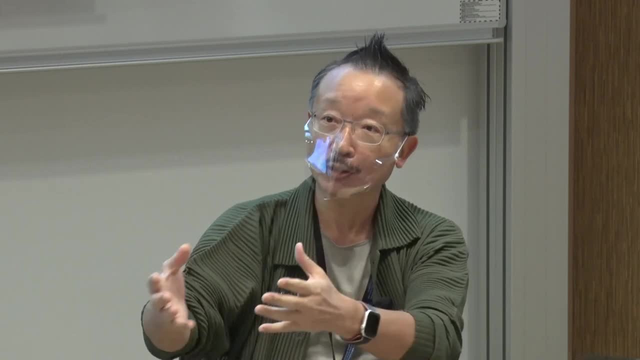 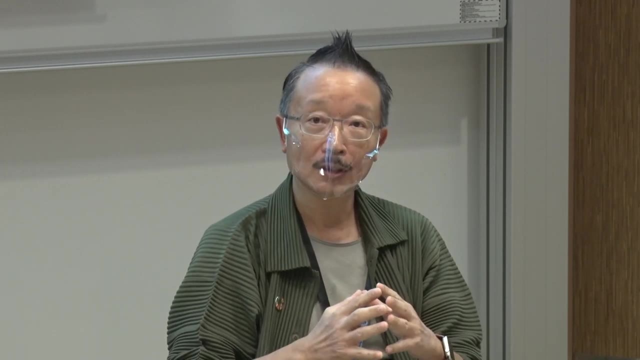 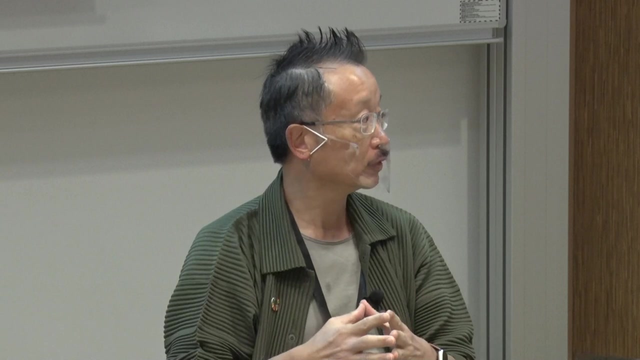 If we go to Hawai'i, we'll pack the things that are different if we would go to New York during wintertime. But the future is uncertain. If we don't know the future, how can we plan for the future? So the important thing is: how can we pay for the future? 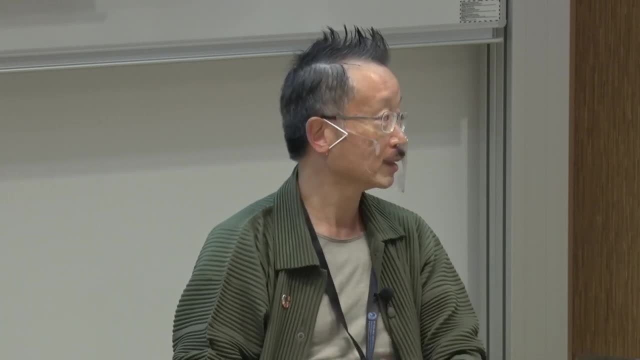 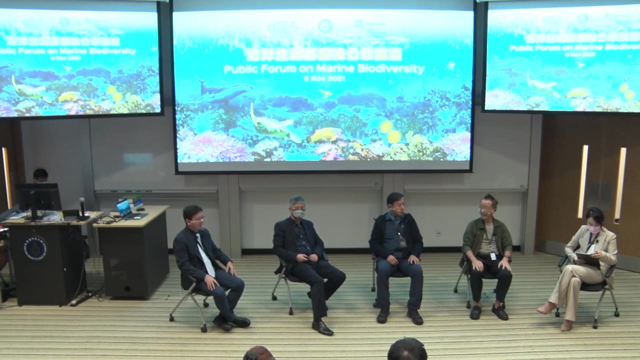 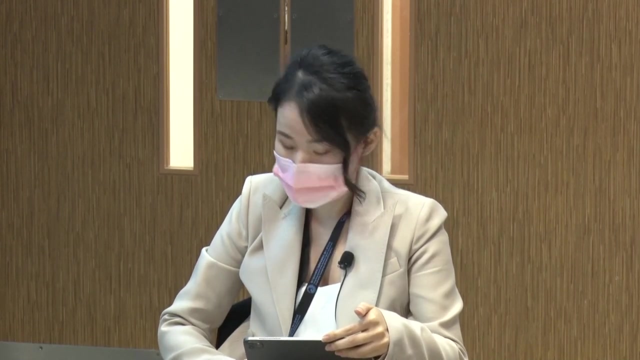 And that is where long-term impact comes in. handful might not exist. Thank you, Thank you for answering these questions. So the next question is to Professor Chong here, Yep. So, as an expert in fish taxonomy, from your perspective, how do we enhance? 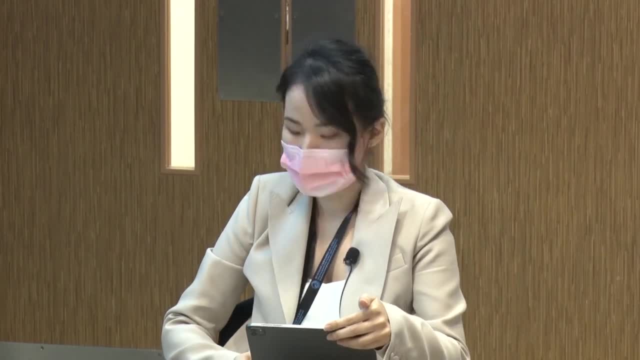 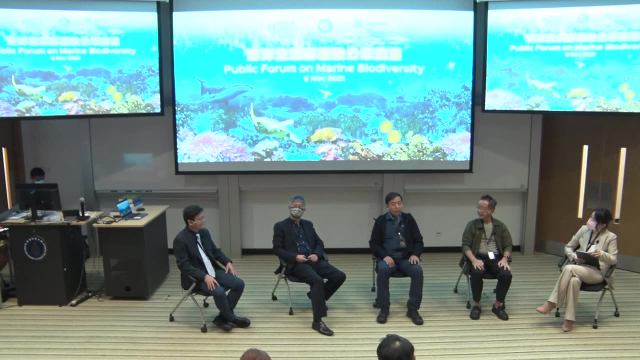 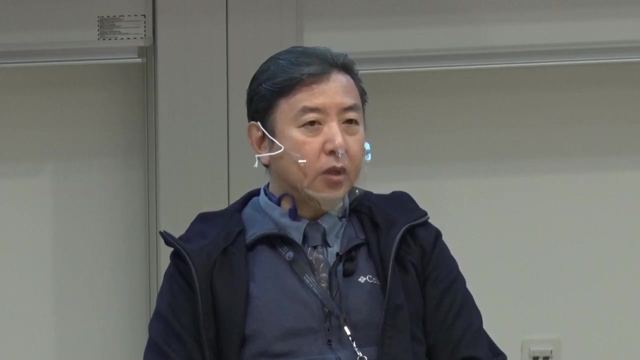 the knowledge to support the marine conservation in Hong Kong, And what are the critical information you wanna share us? Oh yes, That's a good question, Because what we have to know about nature is about its structure and function. So when something has a structure, and then we know. 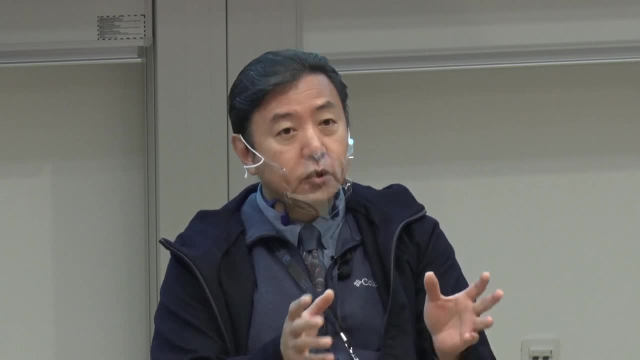 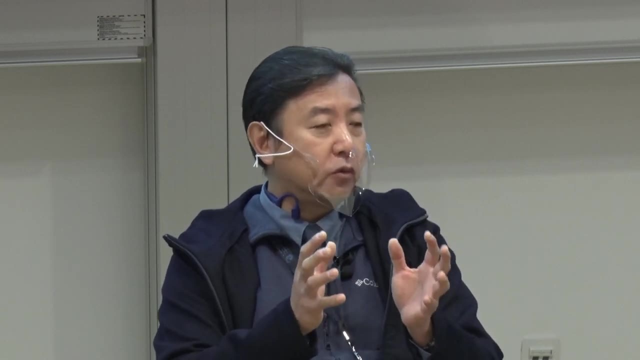 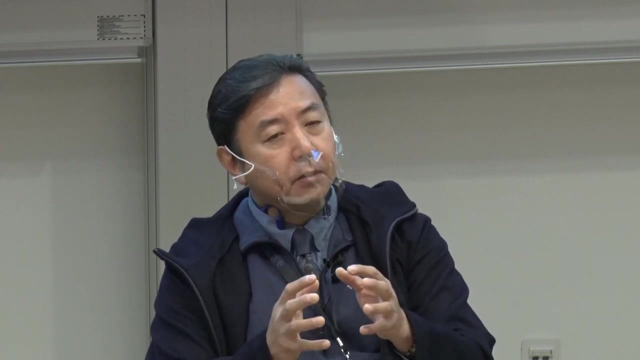 how it functions, and then we have to understand both. So just like fishes is not an exception, So we have to. Firstly, I would like to focus on the life cycle. It's very basic biological knowledge that we focus on more than a century. 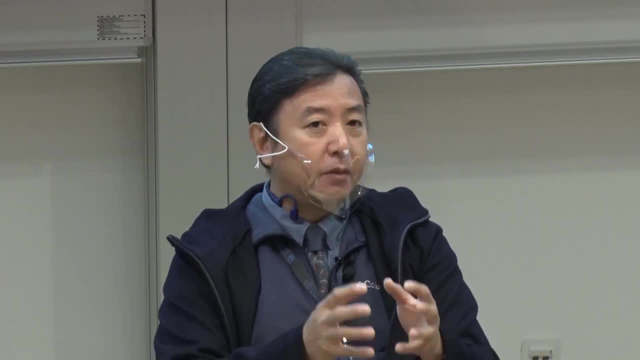 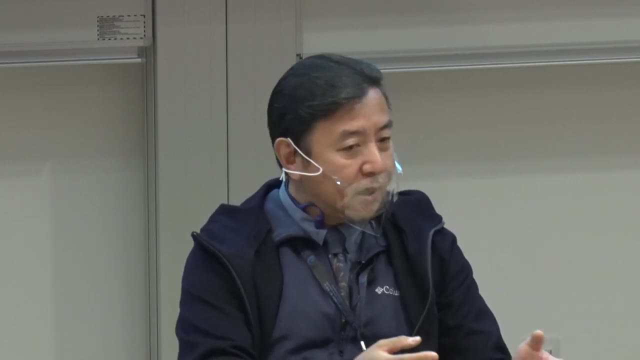 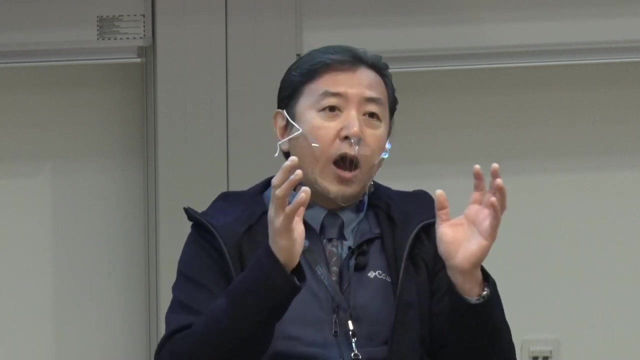 years ago. So it's very important for the This basic information, how they live, where they lay eggs and then they grow And then just like fishes- it's very complicated- and also the polychaetes and so on, and algae, I think. 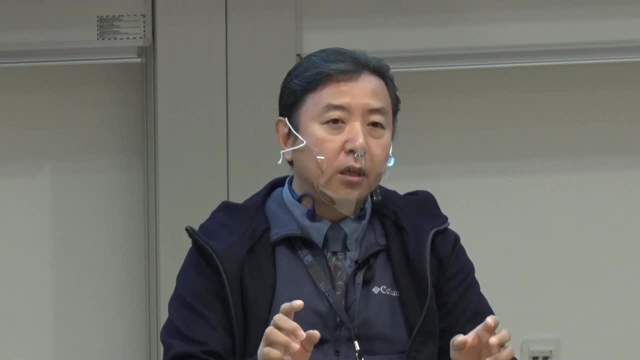 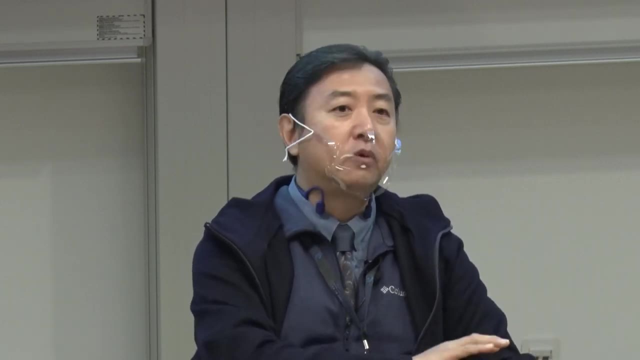 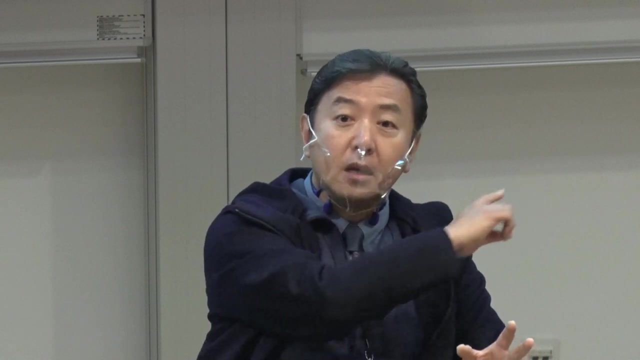 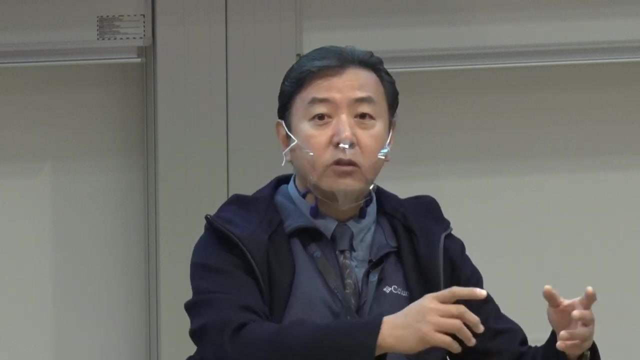 we all know that a creature is not only living in a very restricted area, what we call the habitat. Habitats are broad, It's just like. some are the diadromous fishes. They penetrate sea and also river, And also sometimes we found some freshwater fishes, sometimes in pond, and then they'll be in the flooded. 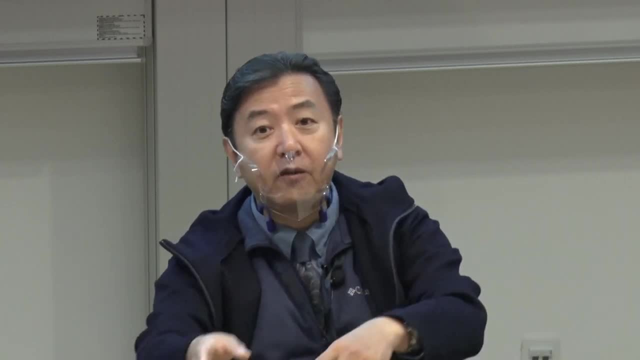 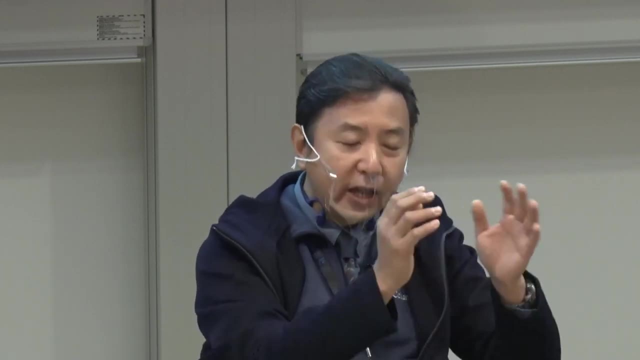 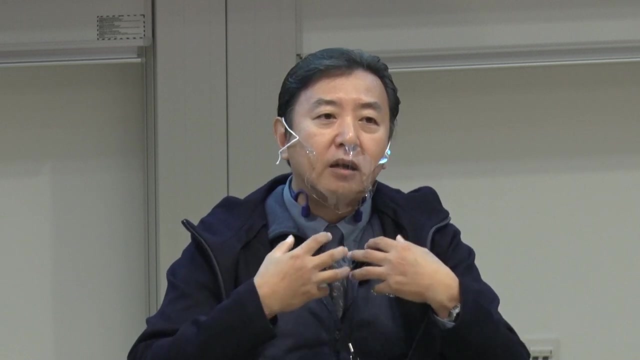 and then they go out to the river stream and then they have a, a find, a breeding place. So from hatching, laying eggs, hatching, and then growing up they have. Sometimes they change what they eat, So it's complicated, So we have to. 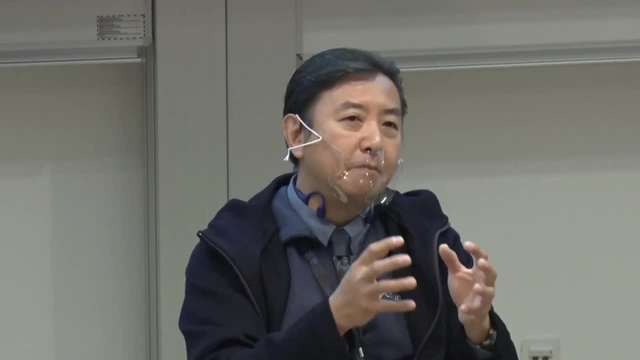 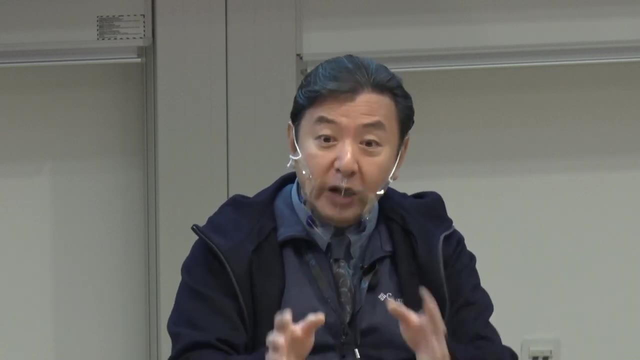 How to make good conservation of all the species. so they're all related. Some are eaten and preyed and predated, Some are eaten and preyed and predated. So we all have to concern the chain, the chain of food chain, and so 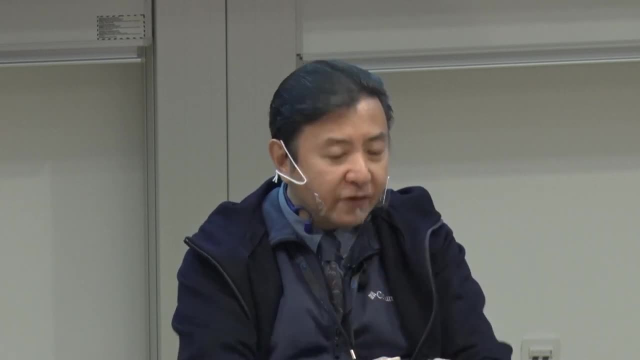 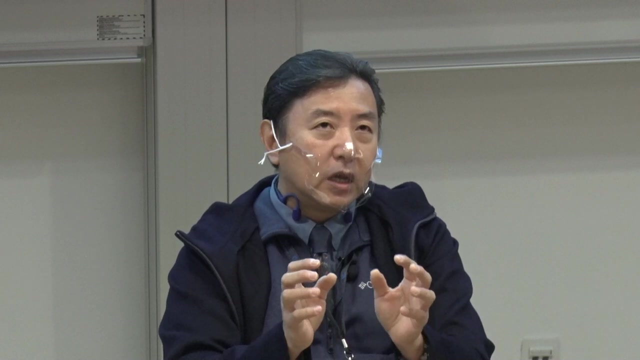 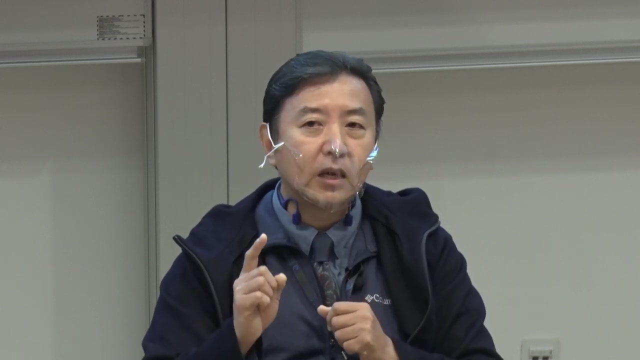 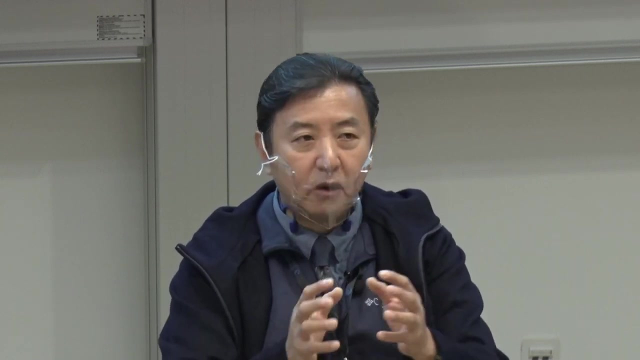 So you have to know the life cycle and food, food habit, and so the the habit itself. So So in Hong Kong, there's a very important characteristic we lack of: We lack of life cycle: a lifecycle database on each species. So I spent a lot of decades in building the aquarium, First time for myself and also after I established the Archaeological Society, And then I built a very simple aquarium To let those interns and also the workers and volunteers to observe how they grow, how they hatch and when. 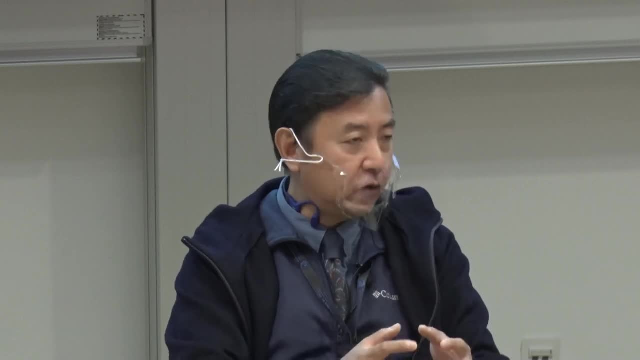 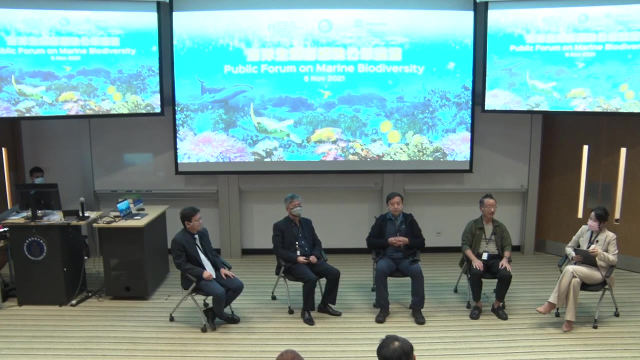 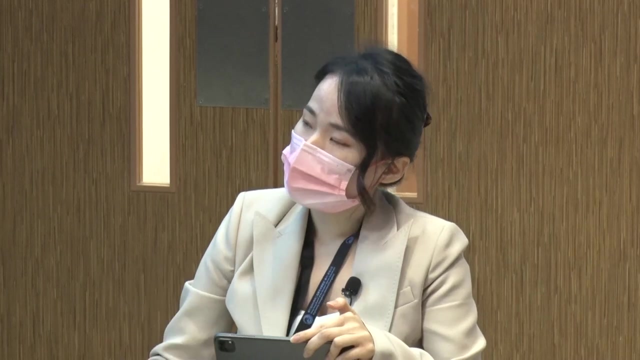 So these we have to know first, Otherwise we can't protect any species in Hong Kong. This is my feeling. Yes, Thank you for answering these questions. Actually, from your previous presentation, it is also very encouraging to see that Hong Kong 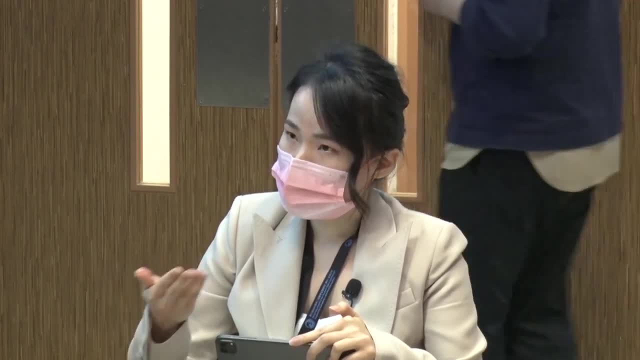 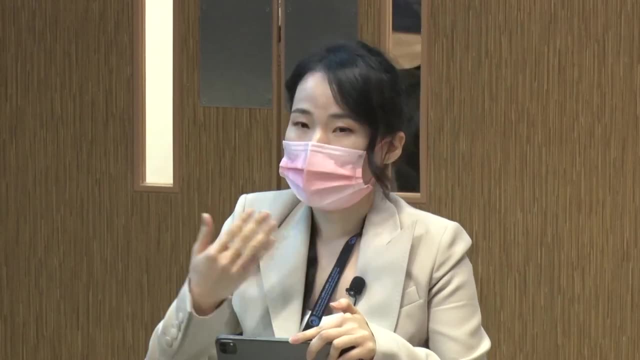 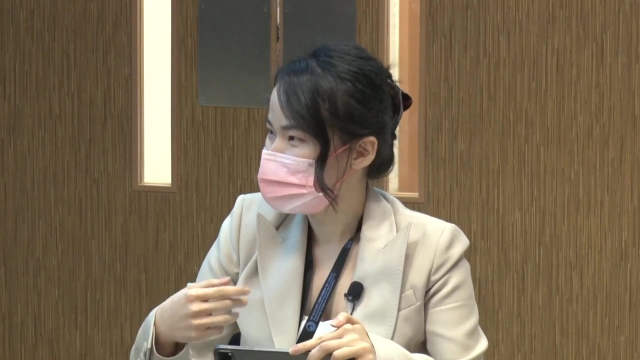 is doing quite well in the marine conservation, Because Hong Kong only has 0.03% marine areas of our country And we recorded over 20% marine species. It is quite encouraging though, Yeah, So the next question will to Professor Liu. 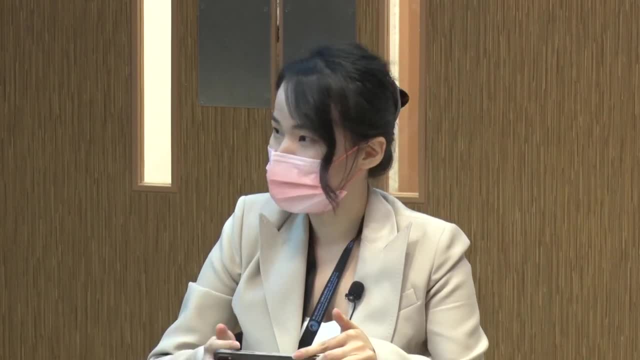 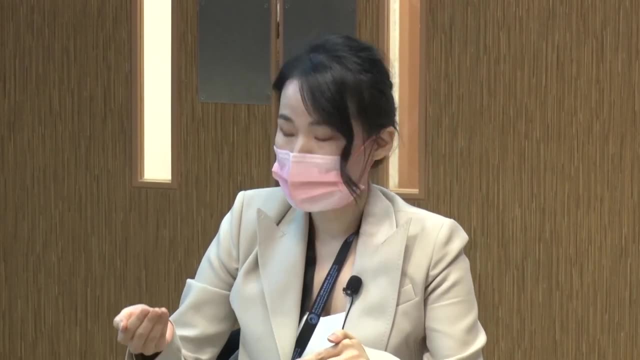 First of all, congratulations on your recent achievement, Professor Liu. Thank you, Thank you. It is really a pleasure. I really appreciate it And I would like to thank Professor Liu for her time. That was very informative. So I'm going to ask Professor Liu to give a few more questions. 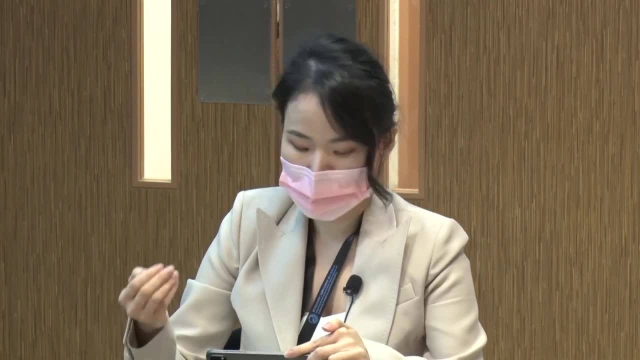 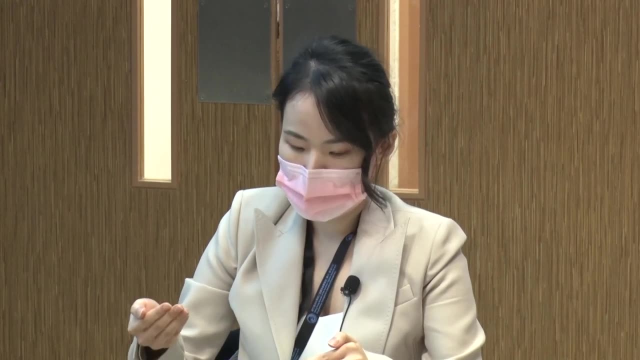 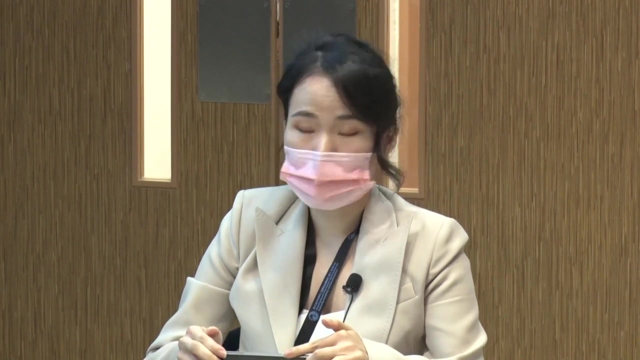 I think the last one is for you. So the question is: how do we, as the research team, establish a model to explain the influence of warming and the human activities on the change of the different phytoplankton which show the lights on protection and provision? 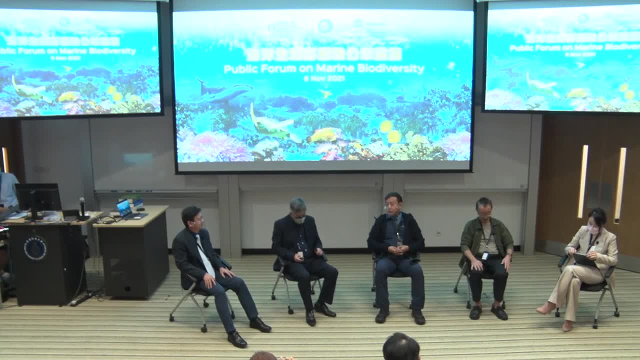 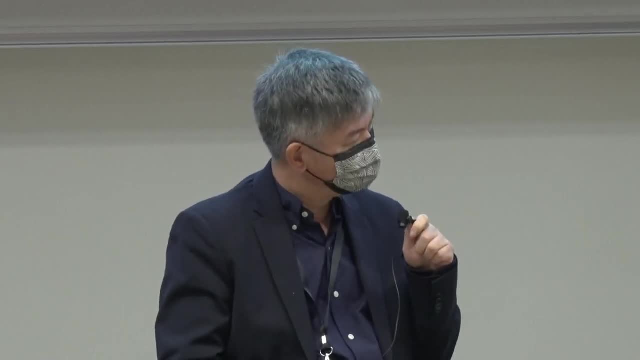 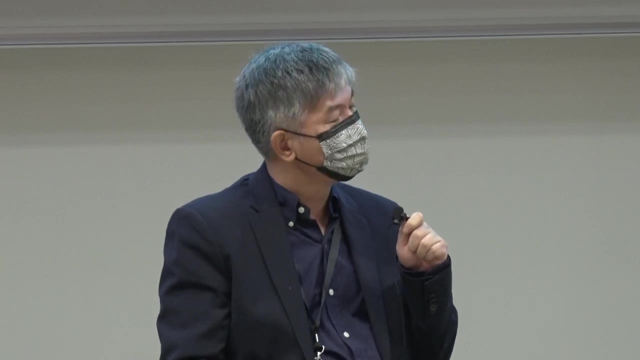 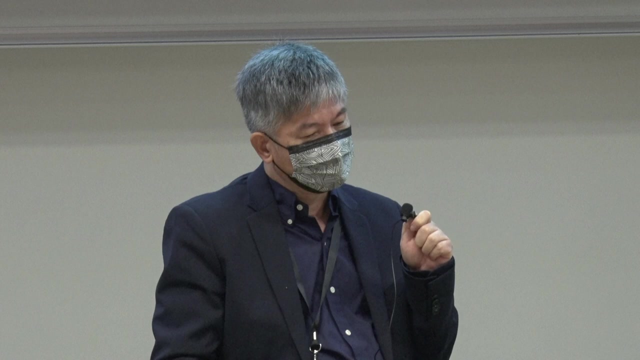 field, thank you. thank you very much, Emma. yeah, I think your question is about translational. yeah, through today's talk, you see, you know we are doing base, both basic research and the translational research, and I agree there's lots of space we can improve. for example, as a professor chair mentioned also the the. 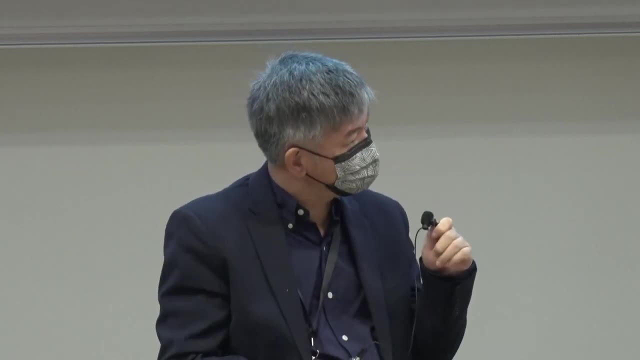 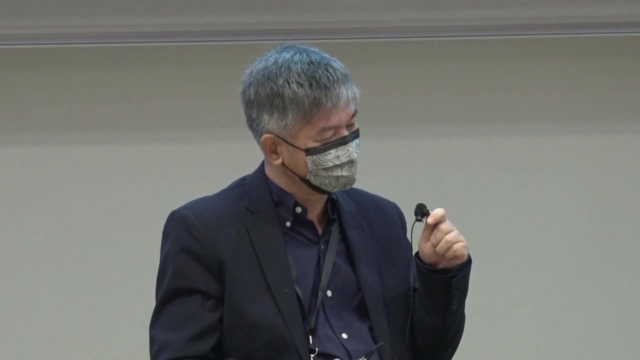 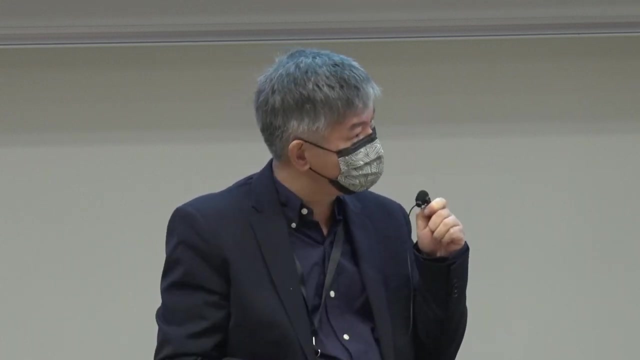 professor in mainland. every species, there's a value: the habitats, the species, the system- there's a value. biodiversity, there's a huge value. and also the. the last presentation about this anti-falling, so there's a lots of information about this anti-falling, so there's a lots of 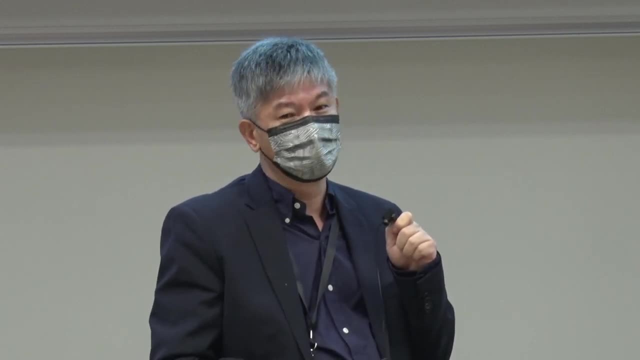 information about this anti-falling. so there's a lots of room a marine. you know room a marine. you know room a marine. you know research, biodiversity, global warming, as well as research, biodiversity, global warming, as well as research, biodiversity, global warming, as well as conservation. you know you can. 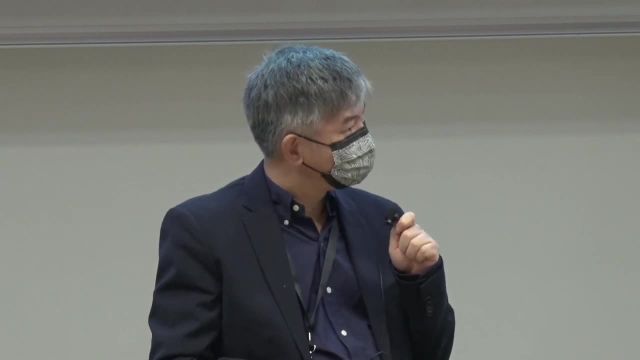 conservation, you know you can. conservation, you know you can create startup company or lots of create startup company, or lots of create startup company, or lots of potential okay. so I think young people potential, okay, so I think young people potential, okay, so I think young people certainly, you know you can get. 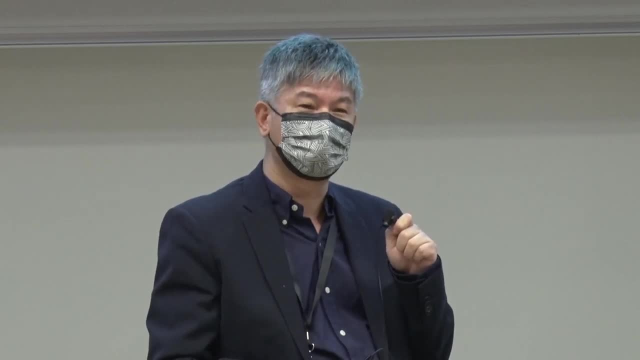 certainly you know you can get, certainly you know you can get interested in the research and the interested in the research and the interested in the research and the research and but also there's an research and but also there's an research and but also there's an opportunity to you, do you know, using 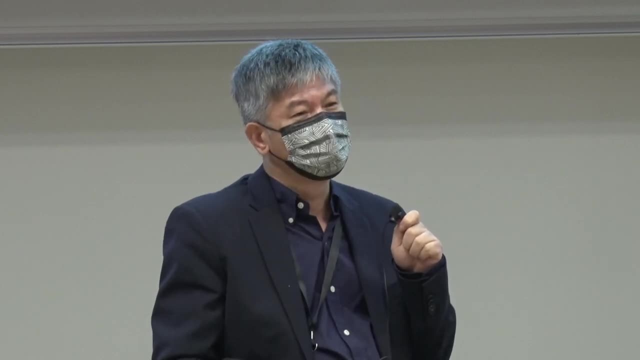 opportunity to you. do you know using opportunity to you? do you know using your knowledge to to you know? create your knowledge to to you know, create your knowledge to to you know, create either a company or productivity, either a company or productivity, either a company or productivity pro you know products. I think we need. 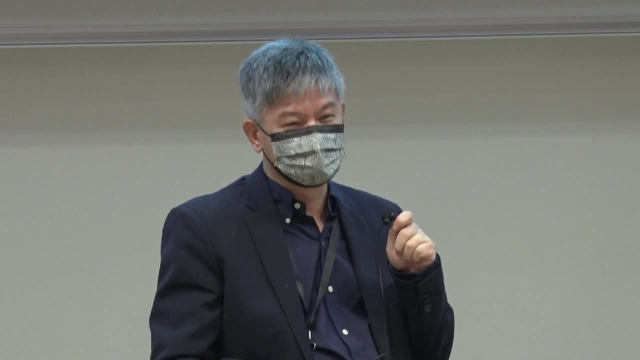 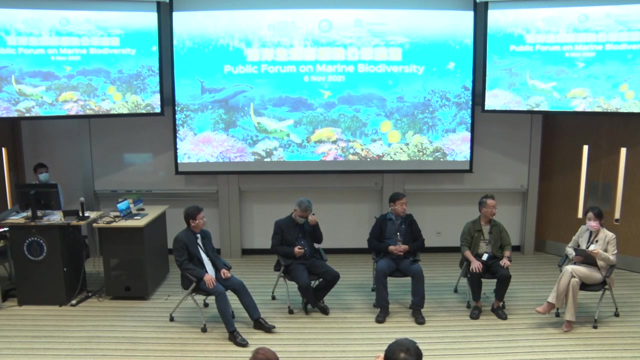 pro you know products. I think we need pro you know products. I think we need more people to come to this, more people to come to this, more people to come to this field. okay, yeah, thank you actually for the field. okay, yeah, thank you actually for the field. okay, yeah, thank you actually for the us co ocean decade initiative. the 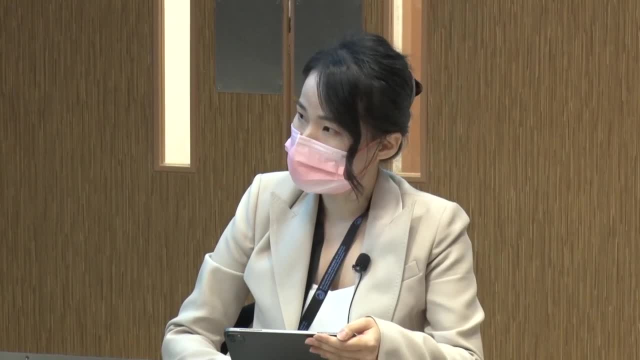 us co ocean decade initiative. the us co ocean decade initiative. the mission is the transformative ocean. mission is the transformative ocean mission is the transformative ocean science: solutions for the sustainable science, solutions for the sustainable science, solutions for the sustainable development, connecting people and the 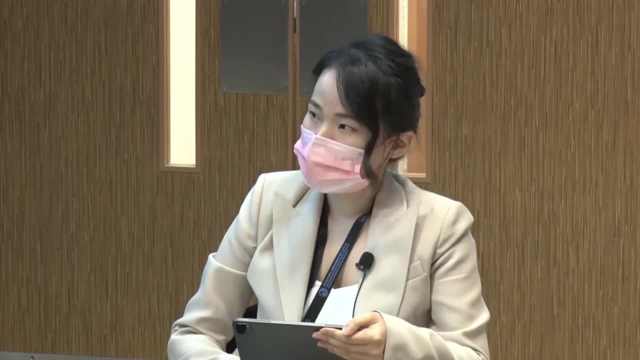 development connecting people and the development connecting people and the ocean. I agree with professor: there is a ocean. I agree with professor, there is a ocean. I agree with professor, there is a huge room here for our young scientists. huge room here for our young scientists. huge room here for our young scientists. now the question is to professor Cho. 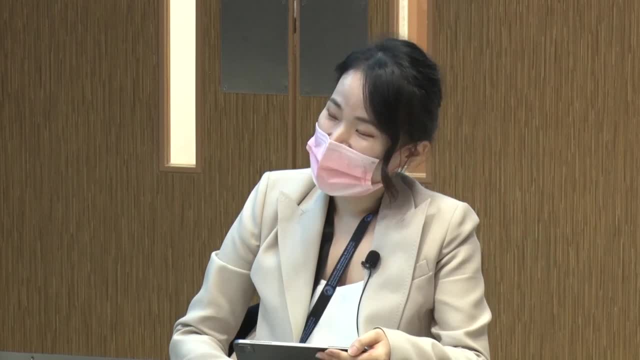 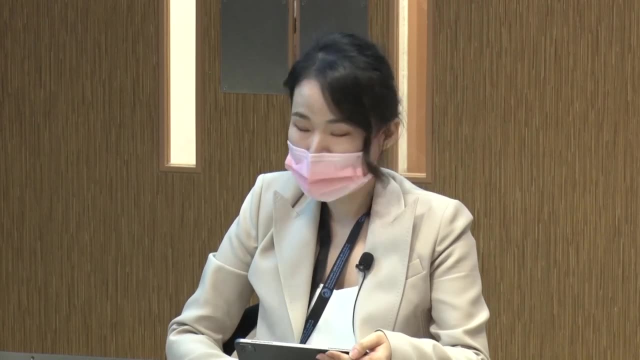 now the question is to professor Cho. now the question is to professor Cho also also also congratulations on your recent new. congratulations on your recent new. congratulations on your recent new species discovery professor chose team. species discovery professor chose team. species discovery professor chose team: discovered in Hong Kong water- our new. 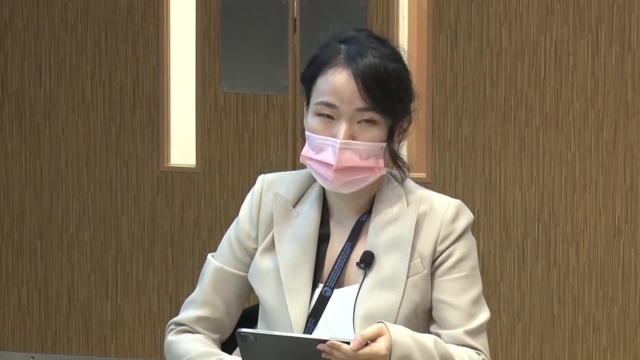 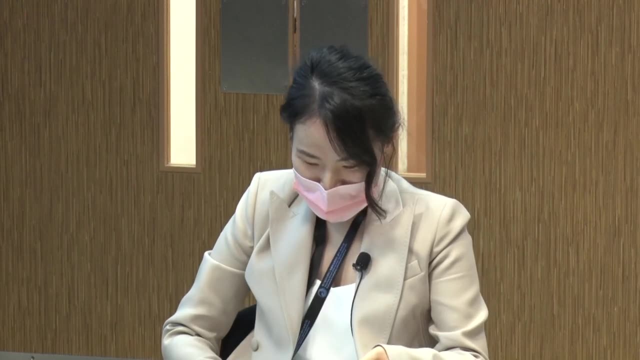 discovered in Hong Kong water, our new discovered in Hong Kong water, our new species of hard coral and the two new species of hard coral and the two new species of hard coral and the two new species of species of species of newly brunk right? yeah, so actually the 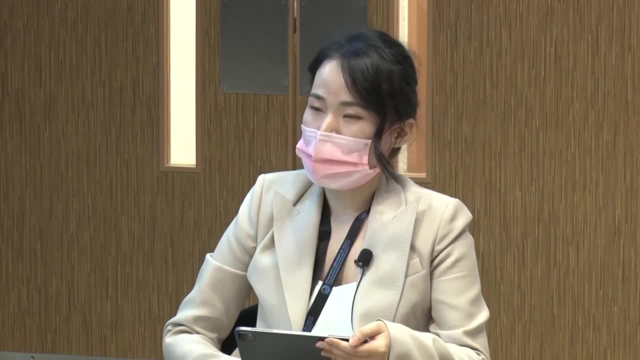 newly brunk, right? yeah? so actually the newly brunk, right? yeah? so actually, the discovery of the new species years are discovery of the new species. years are discovery of the new species. years are either vivid reflection of our Hong Kong either vivid reflection of our Hong Kong. 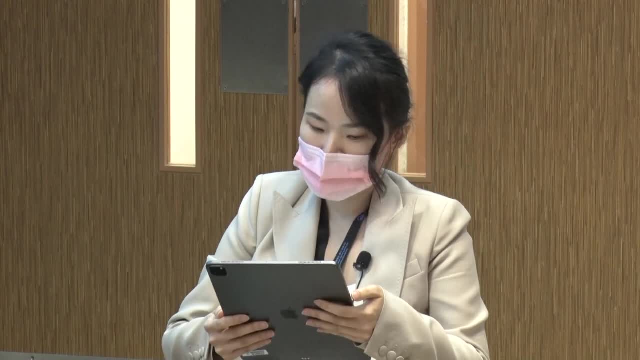 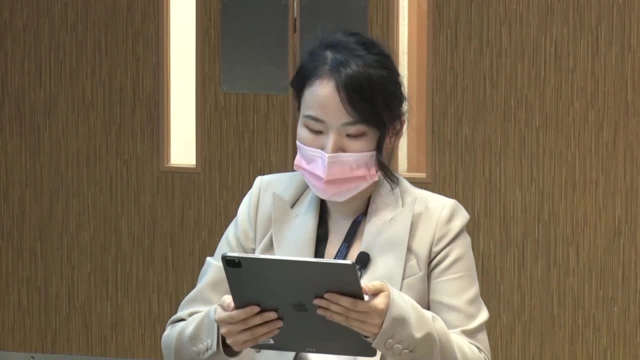 our original marine biodiversity and could you please share with more? could you please share with more? could you please share with more information regarding your journey of new information, regarding your journey of new information regarding your journey of new species discovery. thank you well I. species discovery. thank you well I. 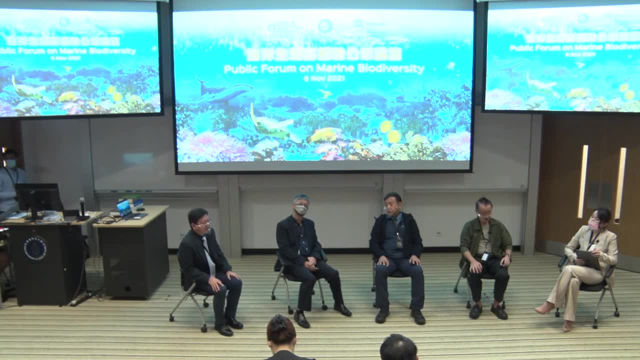 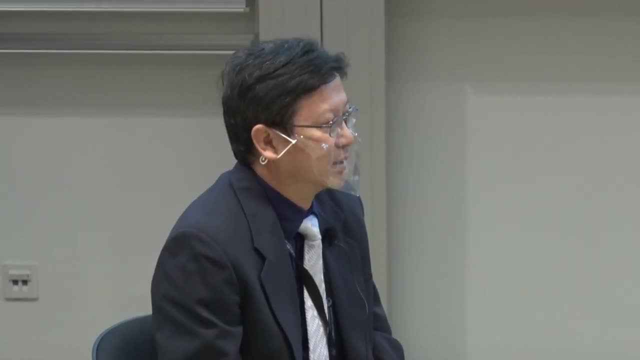 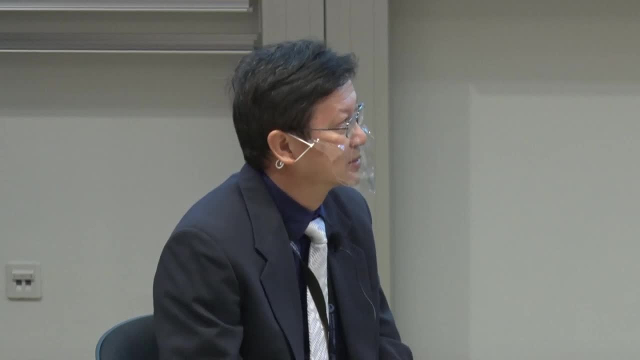 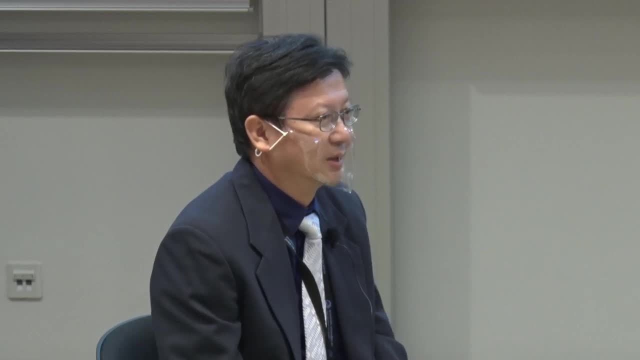 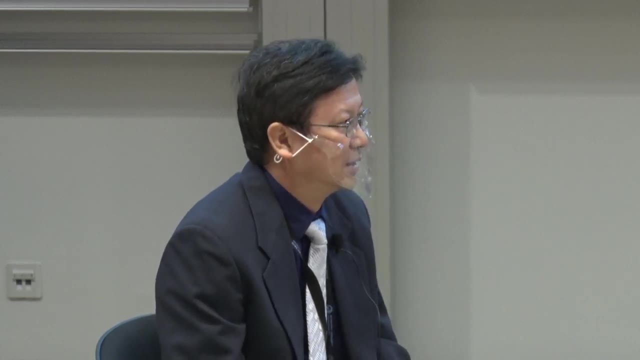 is different from the other species, but is different from the other species. but to do formal our taxonomy training, I'm to do formal our taxonomy training, I'm to do formal our taxonomy training, I'm sure, like sure, like sure, like buzzer joke in fish taxonomy you need. 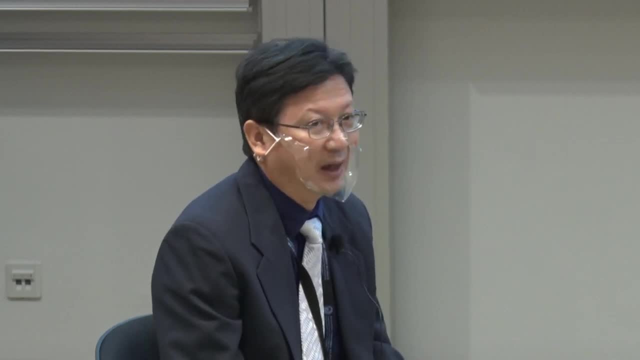 buzzer joke in fish taxonomy. you need buzzer joke in fish taxonomy. you need some training. and in the University I some training. and in the University I some training. and in the University I think it's a good place to train, think it's a good place to train. 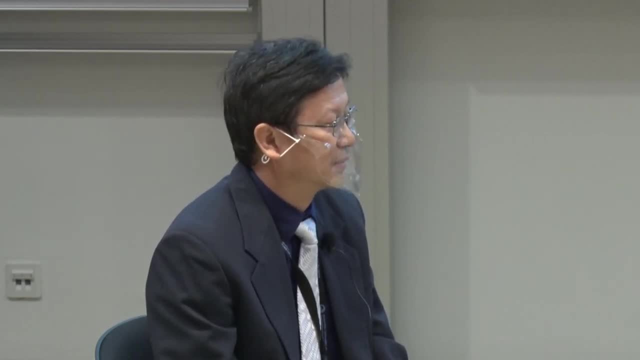 think it's a good place to train students to do taxonomy and, of course, students to do taxonomy, and, of course, students to do taxonomy, and, of course, you need to go to the field as well, and you need to go to the field as well, and you need to go to the field as well, and you need to go into the water and 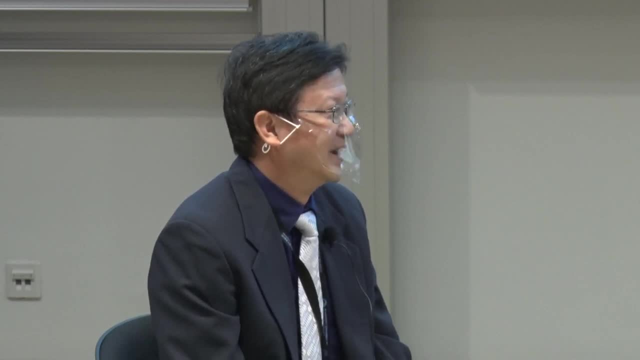 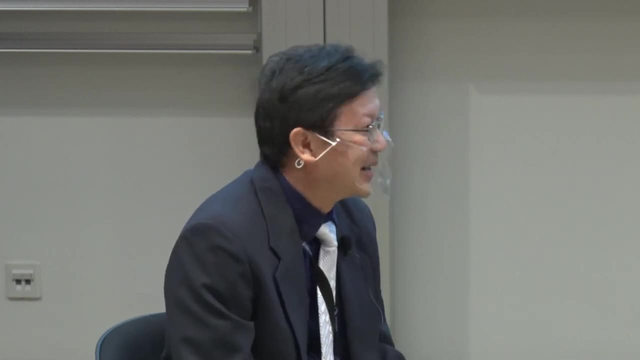 you need to go into the water and you need to go into the water and nowadays, a lot of professors are staying. nowadays, a lot of professors are staying. nowadays, a lot of professors are staying in the lab. but every time I go to the in the lab, but every time I go to the 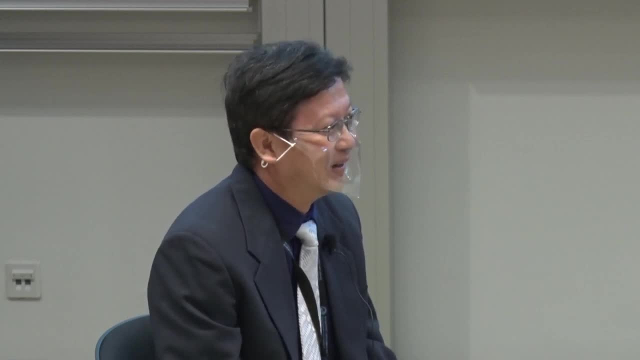 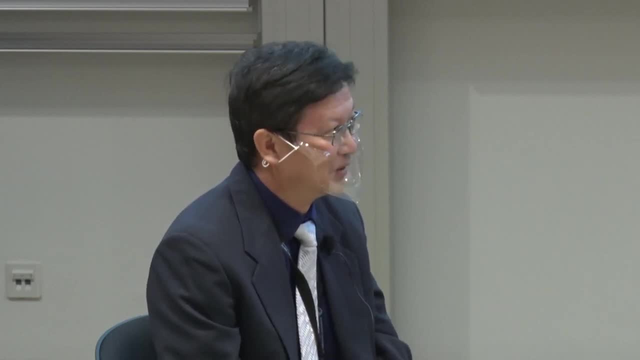 mud flat animals I see, and a lot of them mud flat animals I see, and a lot of them are new animals. so although Hong Kong is are new animals, so although Hong Kong is are new animals, so although Hong Kong is quite well explored, a lot of their even. 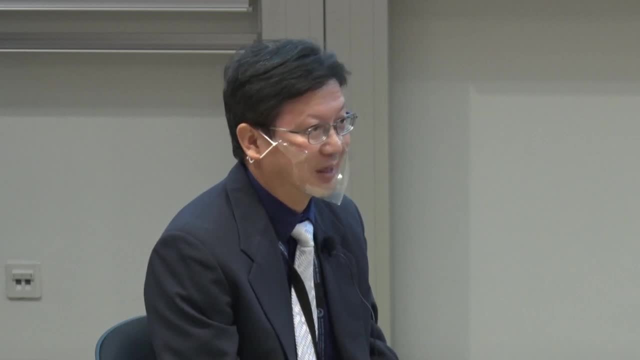 quite well explored. a lot of their, even quite well explored, a lot of their, even for corals, for example. a lot of divers for corals, for example. a lot of divers for corals, for example. a lot of divers. they see corals every day. they look at. 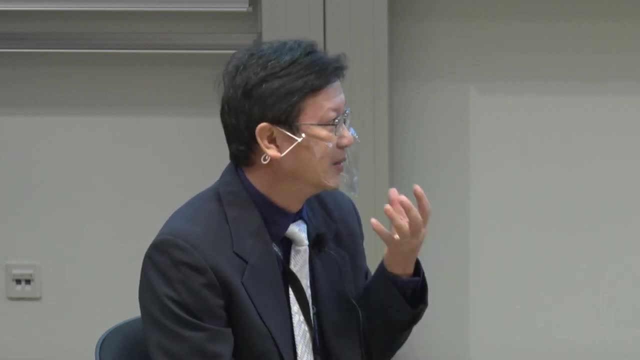 they see corals every day. they look at. they see corals every day. they look at the pretty a nudie branch every day. but the pretty a nudie branch every day. but the pretty a nudie branch every day. but they may not have the scale to identify. 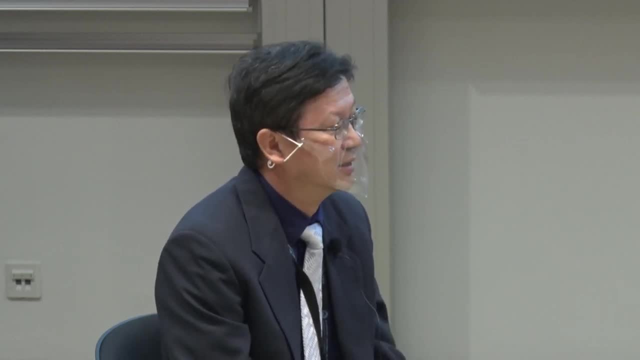 they may not have the scale to identify, they may not have the scale to identify them properly. so so, changing them properly. so so, changing them properly. so so, changing it's very important, it's very important, it's very important, thank you. training is the key for the. 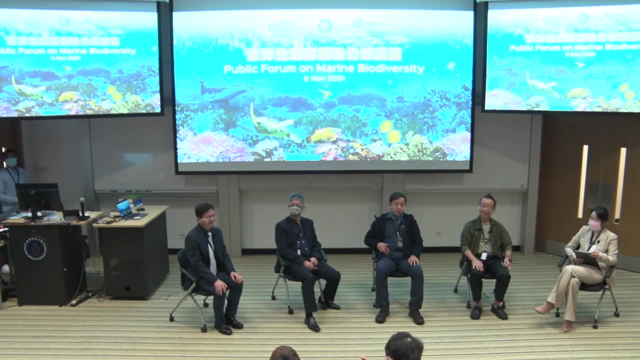 thank you. training is the key for the thank you. training is the key for the next generations, next generations, next generations. and people should have more, pay more, and people should have more, pay more and people should have more, pay more. attention on the marine biodiversity, attention on the marine biodiversity. 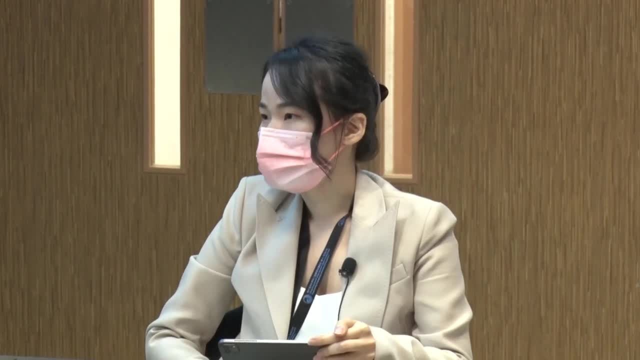 attention on the marine biodiversity. yeah, yeah, and also another way to do it: yeah, yeah, and also another way to do it: yeah, yeah, and also another way to do it is to collaborate with, is to collaborate with, is to collaborate with the amateur, the amateur, the amateur scientists. 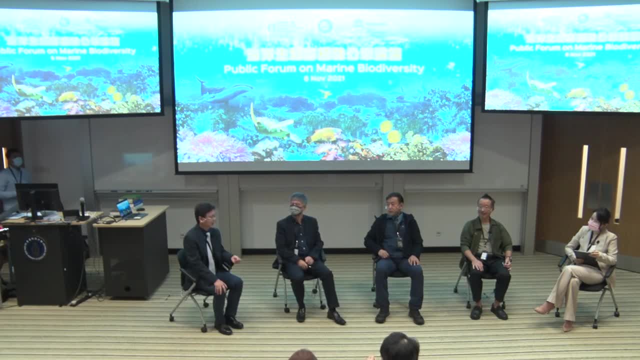 scientists, scientists, so they, so they, so they, if they have more time to look at, if they have more time to look at, if they have more time to look at what's going on in the field, and if what's going on in the field, and if what's going on in the field and if they have some new discoveries they want. 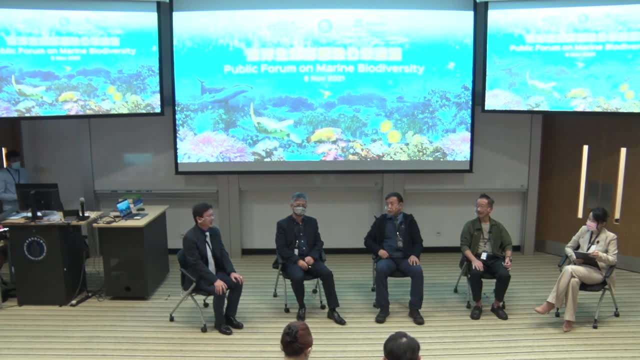 they have some new discoveries they want. they have some new discoveries they want to confirm, to confirm, to confirm. maybe they can contact, maybe they can contact, maybe they can contact experts, experts, experts to make some joint discoveries, to make some joint discoveries, to make some joint discoveries. yeah, 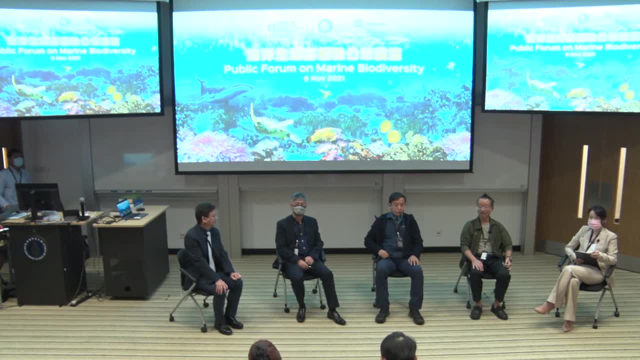 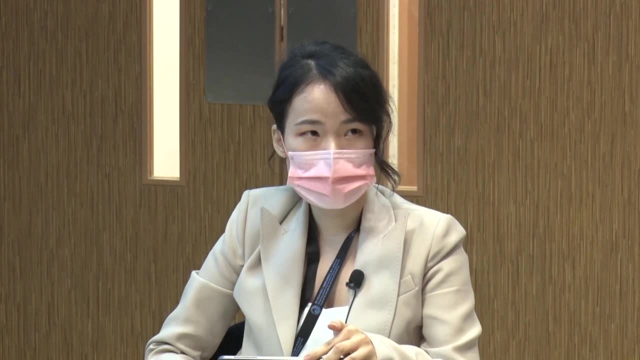 yeah, yeah, agree, totally agree, agree, totally agree, agree, totally agree, and, and, and, and also that we need to, and also that we need to, and also that we need to, we need to change our individual behavior, as we need to change our individual behavior, as we need to change our individual behavior, as well as the institutional. 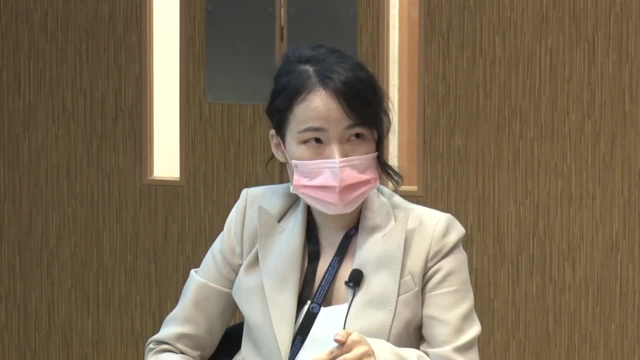 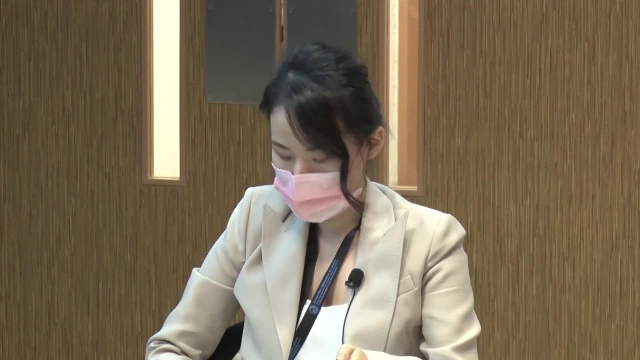 well as the institutional, well as the institutional behavior, behavior, behavior things. we still behavior things. we still have several minutes left. have several minutes left. have several minutes left. let's take another round of questions. let's take another round of questions. let's take another round of questions before we close this session. 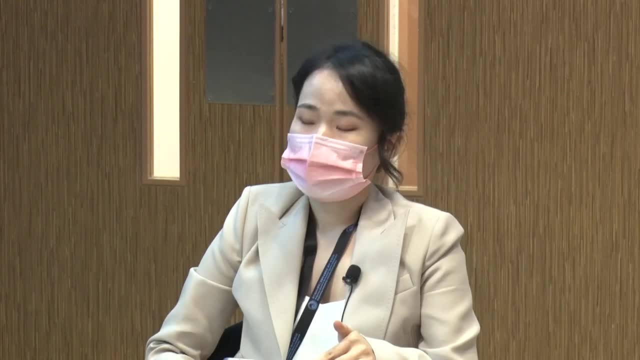 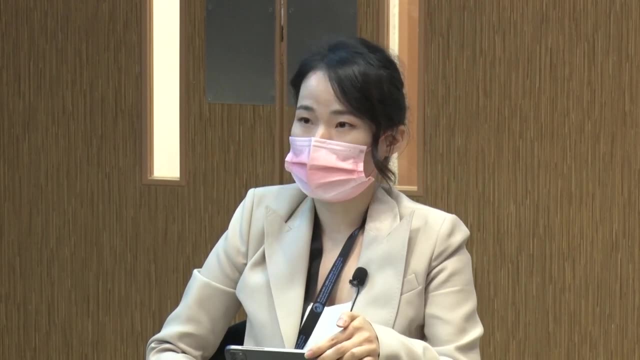 before we close this session. before we close this session, so our country is committed, so our country is committed, so our country is committed for the net zero target by the 2030, for the net zero target by the 2030, for the net zero target by the 2030, and also the carbon neutrality by the. 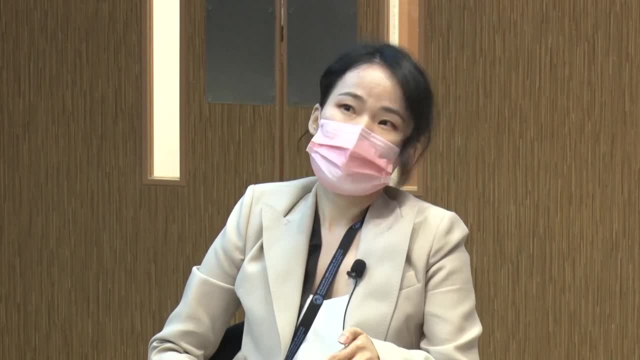 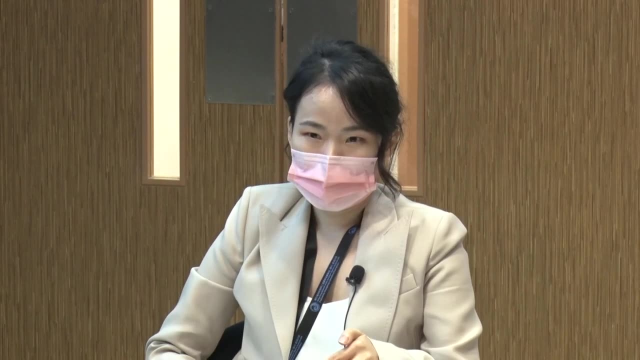 and also the carbon neutrality by the and also the carbon neutrality by the 20, 20, 20, 60., 60., 60.. our chief executive, mr our chief executive, mr our chief executive, mr miss carrie land, miss carrie land, miss carrie land also announced last year: 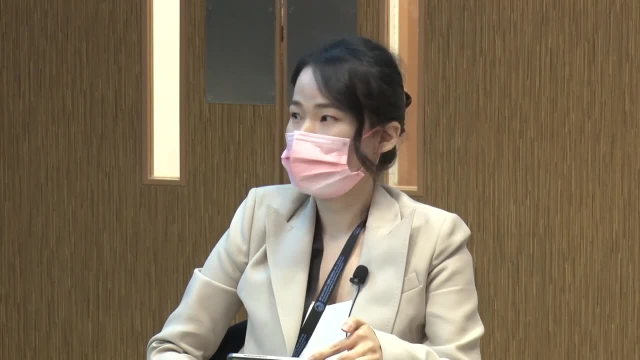 also announced last year, also announced last year: please, please, please, to the carbon neutrality by 2050, to the carbon neutrality by 2050, to the carbon neutrality by 2050. so the question is: uh, what is the link? so the question is: uh, what is the link? 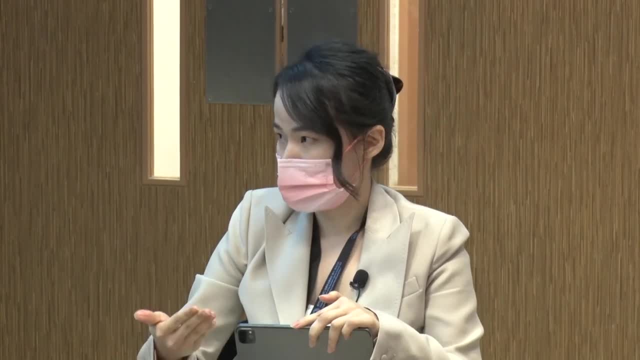 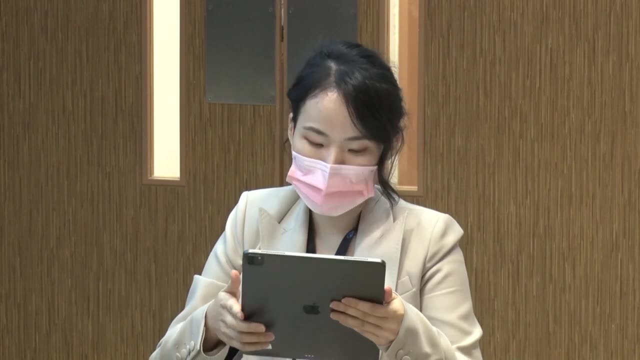 so the question is: uh, what is the link between carbon neutrality and the marine, between carbon neutrality and the marine, between carbon neutrality and the marine? biodiversity? biodiversity, biodiversity, as are the distinguished scholars here, as are the distinguished scholars here, as are the distinguished scholars here. so what's your opinion on the ocean? 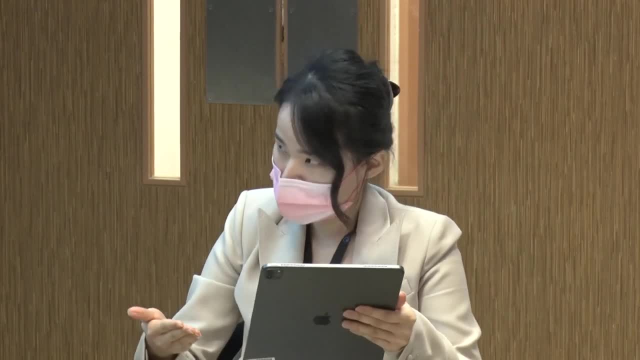 so what's your opinion on the ocean? so what's your opinion on the ocean? science venue chain. science venue chain. science venue chain: from problem identification to the, from problem identification to the, from problem identification to the knowledge application, knowledge application, knowledge application. so maybe start from professor thomas. 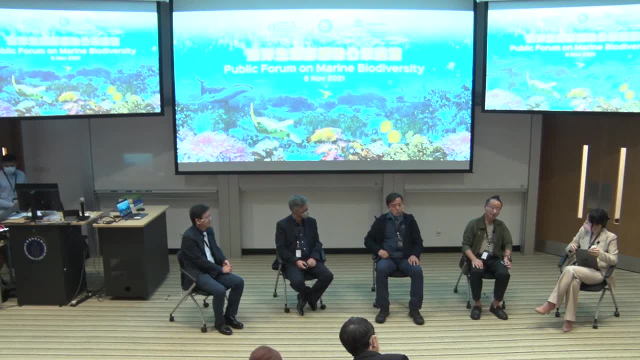 so maybe start from professor thomas. so maybe start from professor thomas. wong first, wong first, wong first: uh. yes, uh, yes, uh, yes, i will look at this from uh because i'm. i will look at this from uh because i'm. i will look at this from uh because i'm from a business background. i will look at. 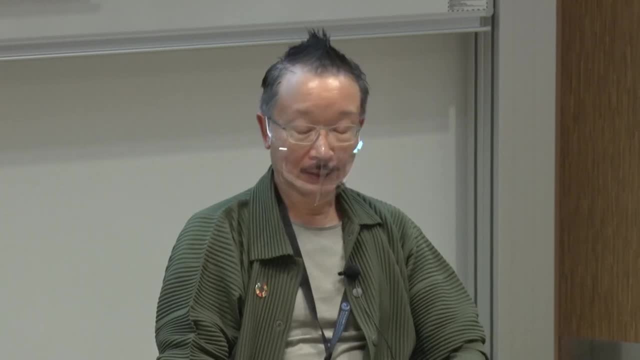 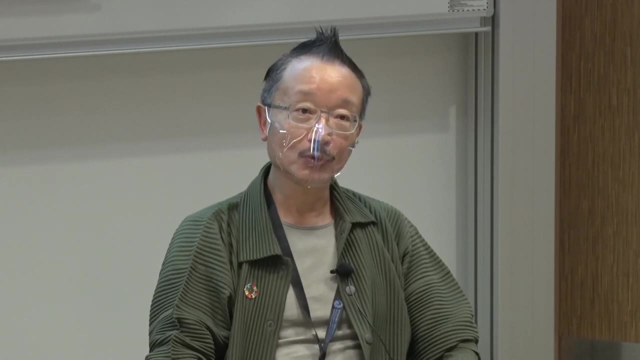 from a business background. i will look at from a business background. i will look at this more from a business, this more from a business perspective, this more from a business perspective than academic or scientific, than academic or scientific, than academic or scientific perspective. i think, as a businessman, we we. 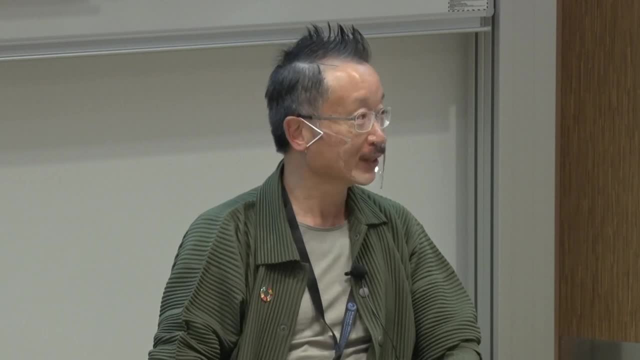 i think, as a businessman, we, we, i think, as a businessman, we, we understand, understand, understand, or, or, or, some of us understand that. some of us understand that some of us understand that the ocean is actually a very important. the ocean is actually a very important. the ocean is actually a very important climate regulator. 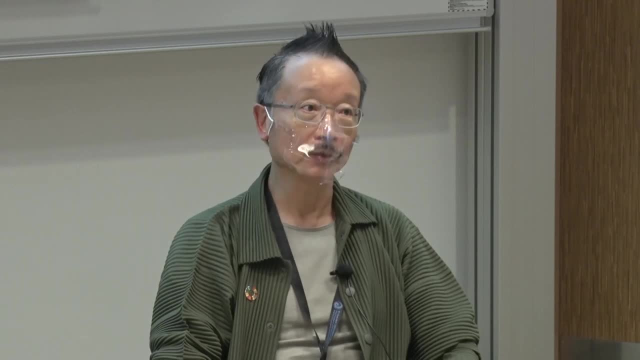 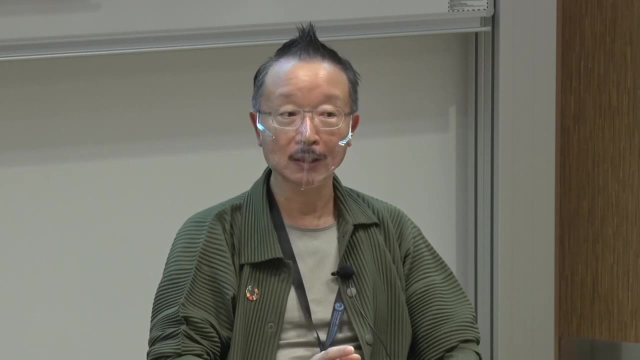 climate regulator, climate regulator, and they helps a lot with our and they helps a lot with our and they helps a lot with our carbons, carbons, carbons. so that's so, that's so. that's that's why, as a, that's why as a, that's why as a, as an individual or as a. 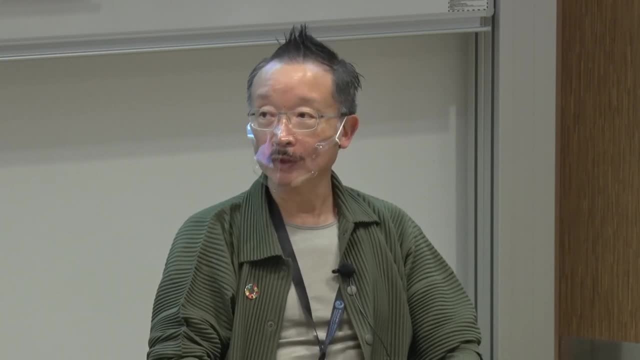 as an individual or as a as an individual or as a corporation, corporation, corporation. each and every one of us have to do our. each and every one of us have to do our. each and every one of us have to do our share and do our part. share and do our part. 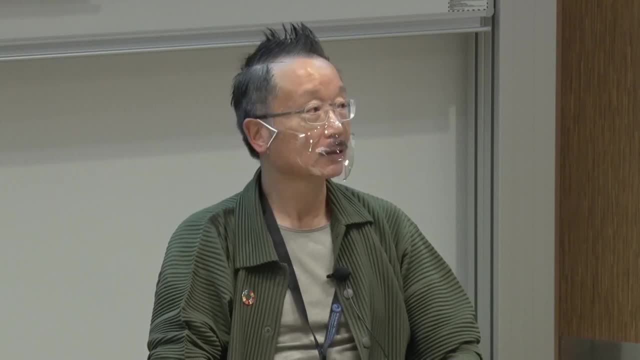 share and do our part, and we have to change our behavior. and we have to change our behavior. and we have to change our behavior. but to change our behavior, we must start. but to change our behavior, we must start. but to change our behavior, we must start with our mindset. 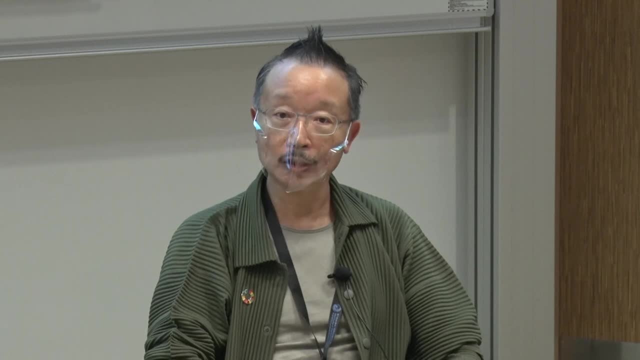 with our mindset, with our mindset so, for example, here with the uh, so, for example, here with the uh, so, for example, here with the uh, hkust, and with all these professors here, hkust, and with all these professors here, hkust, and with all these professors here, they have done a tremendous. 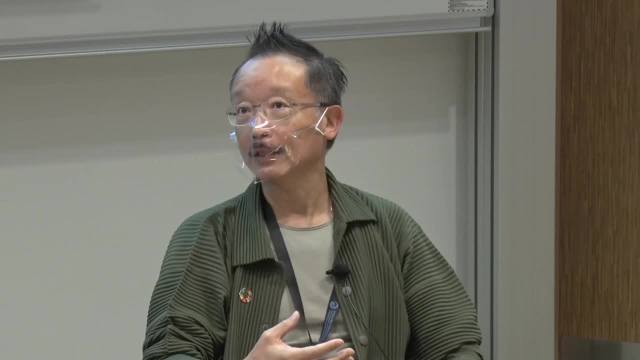 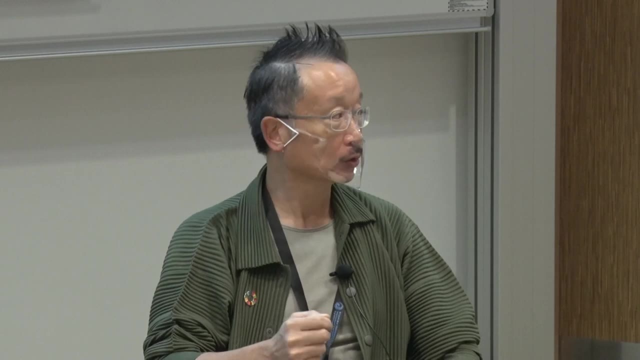 they have done a tremendous, they have done a tremendous amount of work on helping us to amount of work on helping us to amount of work on helping us to understand, understand, understand marine biodiversity and more marine biodiversity and more marine biodiversity and, more importantly, importantly, importantly, what we have to do and what we should. 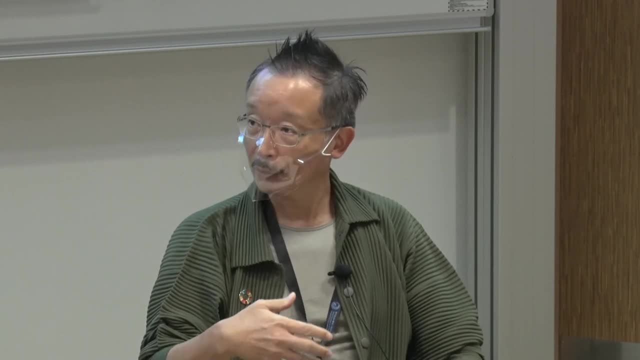 what we have to do and what we should, what we have to do and what we should do do, do so, so. so, after that, after that, after that, if we add on these, if we add on these, if we add on these recommendations, then we'll be helping. 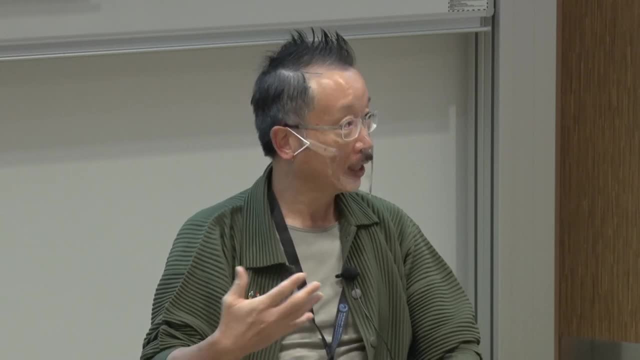 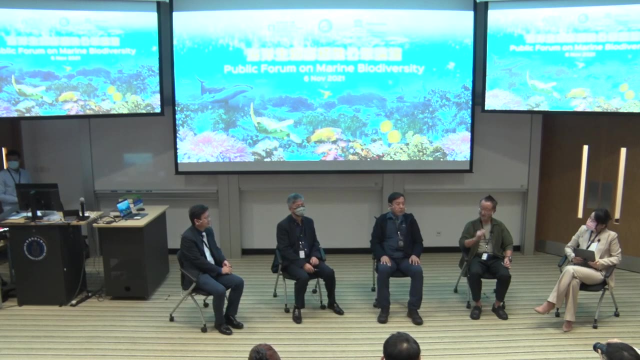 recommendations, then we'll be helping recommendations, then we'll be helping the ecosystem, helping planet earth and the ecosystem, helping planet earth and the ecosystem, helping planet earth and helping ourselves, helping ourselves, helping ourselves. thank you, thank you, thank you. uh, yes, uh, uh, yes, uh, uh, yes, uh, because, uh, i think conservation, this 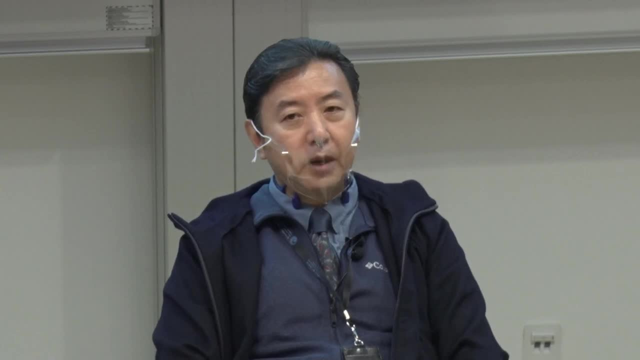 because, uh, i think conservation this, because, uh, i think conservation, this meaning is very, very broad. it's not meaning is very, very broad. it's not, meaning is very, very broad. it's not only the biodiversity, not only living, only the biodiversity, not only living, only the biodiversity, not only living organism, and also including, just like 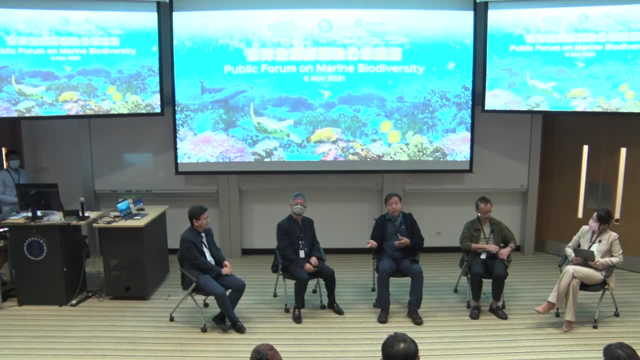 organism and also including, just like organism, and also including, just like artworks. you know, preserving artworks in artworks. you know preserving artworks in artworks. you know preserving artworks in museum, museum, museum, and also in my concept it's very uh and also in my concept it's very uh. 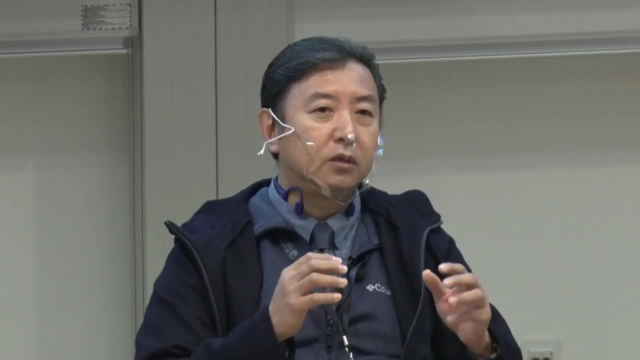 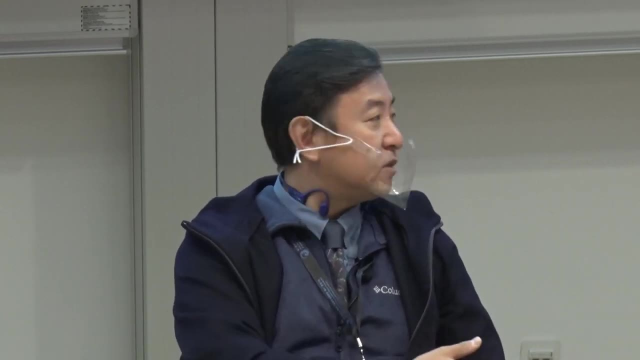 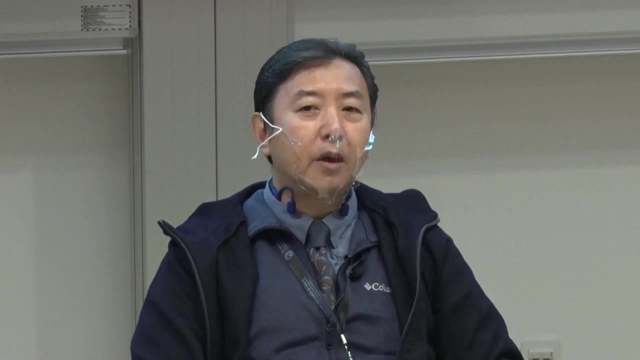 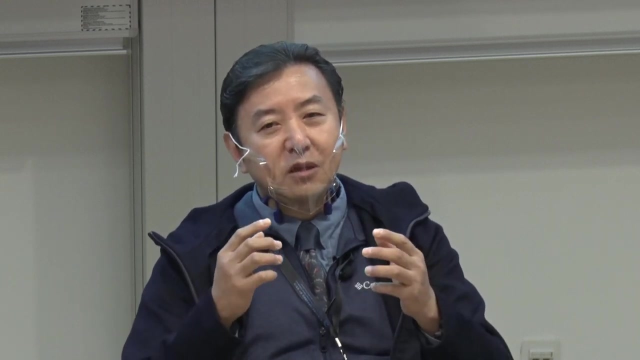 I think it's much more broad. I think it should be applied to our soul. It's very important Because- I'm very agree with Thomas- I think the conservation of our soul is about the human. It's a kind of species that, if we don't well educate it, 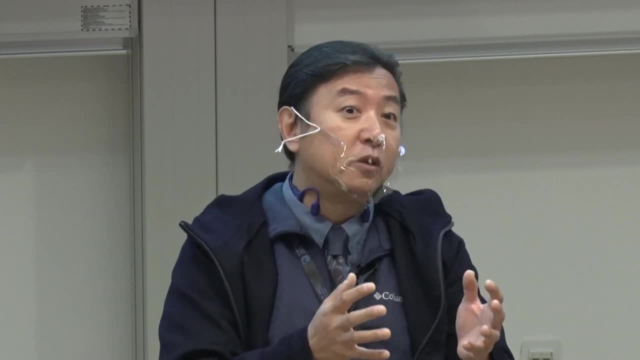 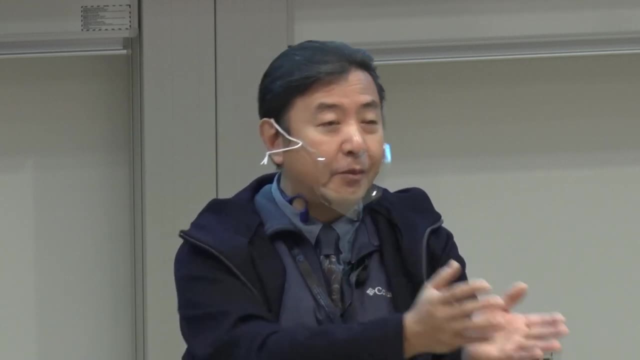 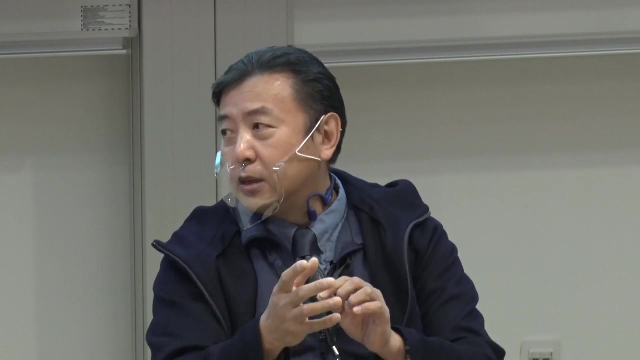 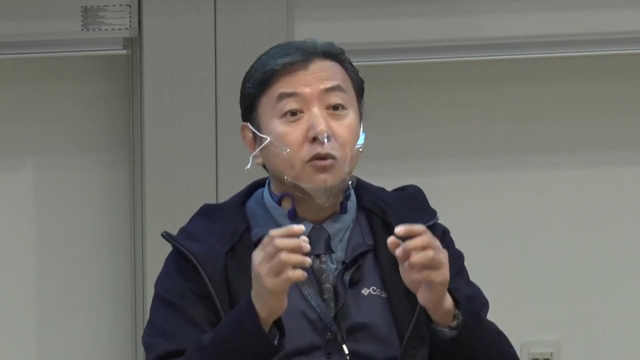 then we can't act very good. So maybe sometimes we are referring to some kind of carbon value or something, And this is only a kind of a reference. So I think we have to know more about the structure and function of nature And then also find out more and more indications. 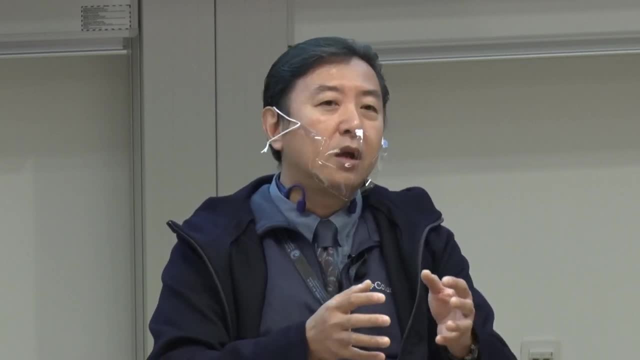 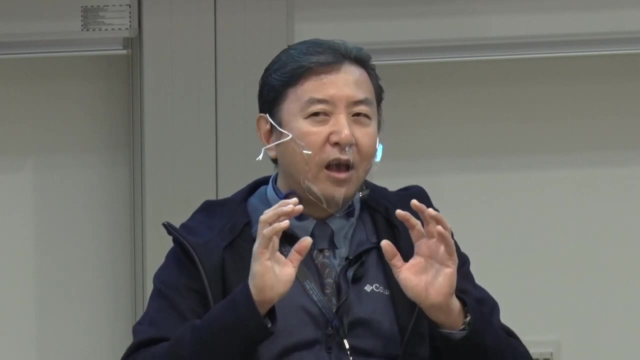 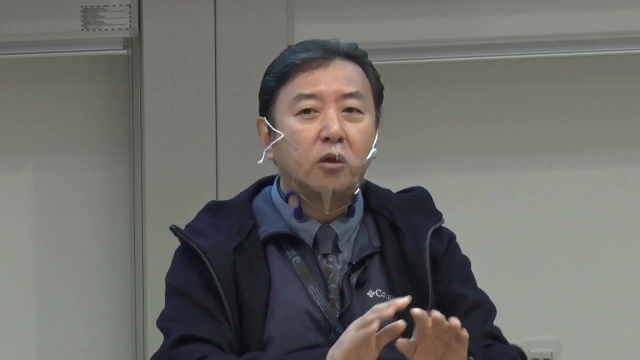 This is first, And then also more research and more education, And then, So hand in hand, And then I think we have to have more conservation of our soul. It's education, And then let them know the truth. It's not about the commercial. 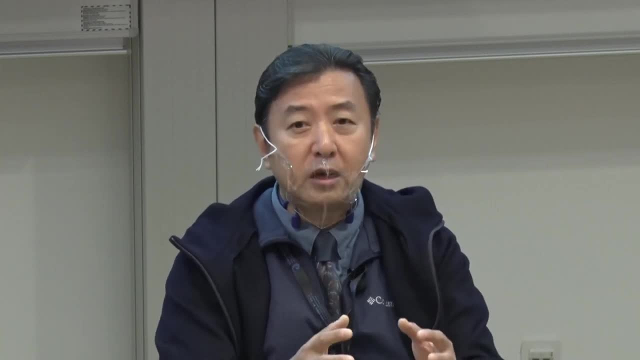 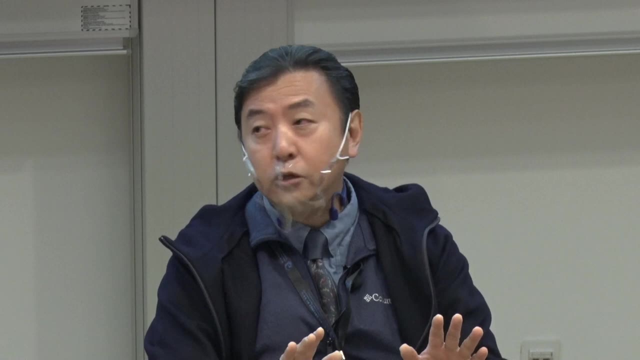 It's not about the cosmetics or something. It's truth And it's not selling. It's not about business. There's no business in nature. I think it's the only structure and function And we have to penetrate into it And then 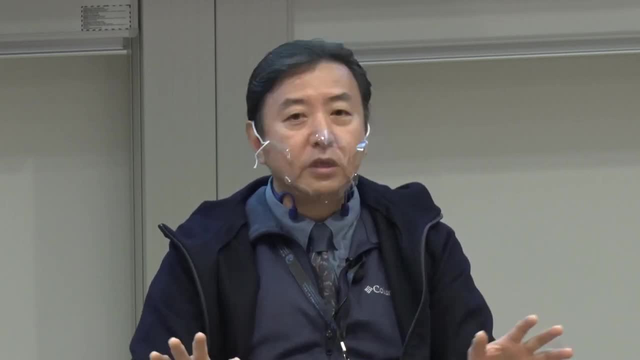 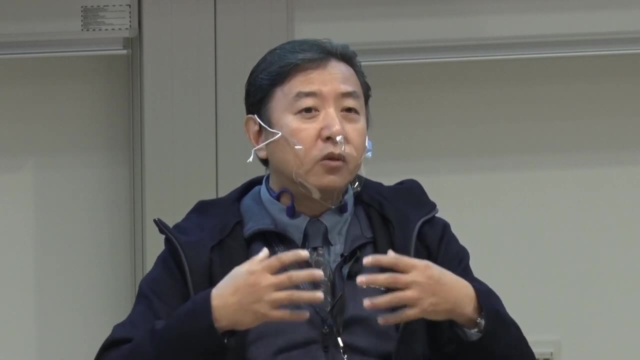 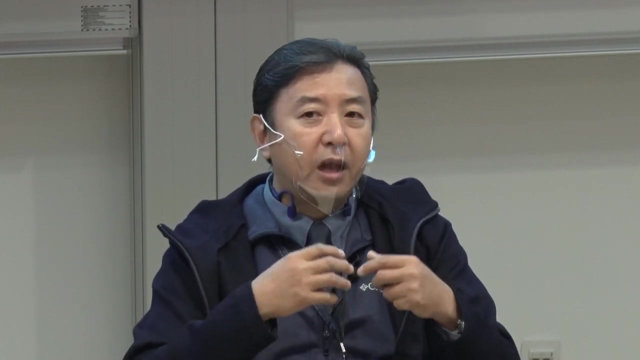 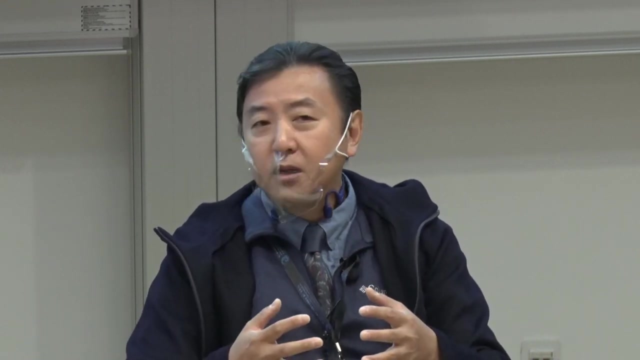 So let those students and all citizens also- It's all have to be educated, well educated- know the truth, And then I think all of our experts have a destination And then have a right to speak something to everybody. But we have to tell the truth. 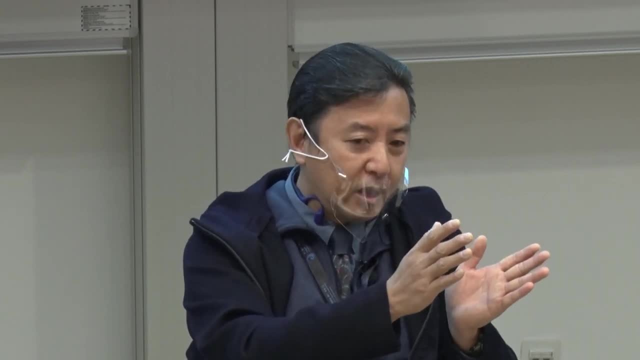 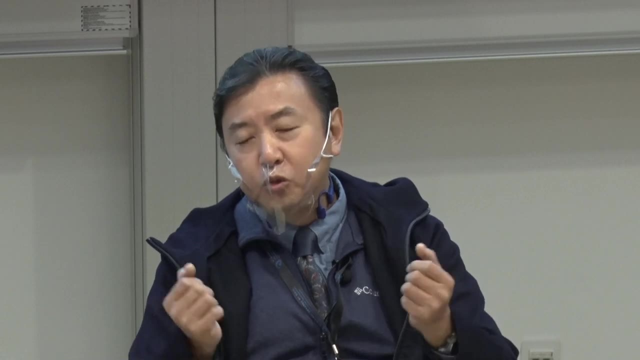 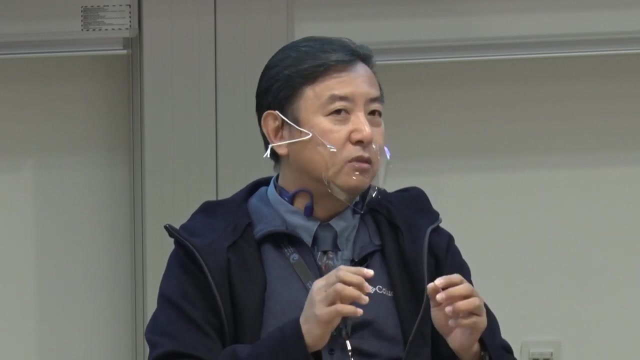 So this is about the first of all research, And then education And hand in hand with citizens and more people globally to do the conservation. This is the- I think it's much more important- And then we find out more indication at the same time, or so. 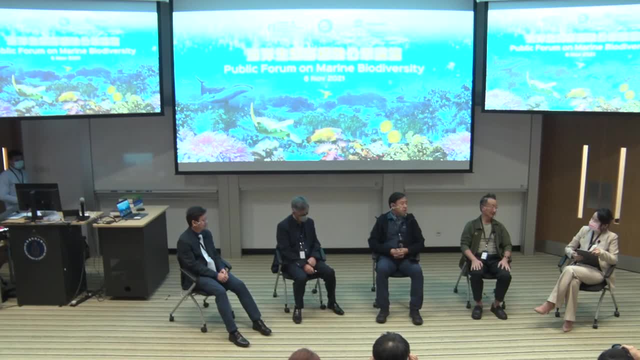 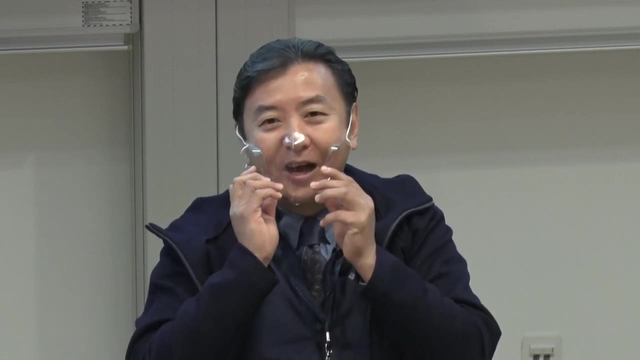 Yes, Because the climate change affect all of us on the global And we should work together, hand in hand, instead of talk for talk. And also, the education is not good, Not good, And then we'll- Our target species- will be eat up by the people. 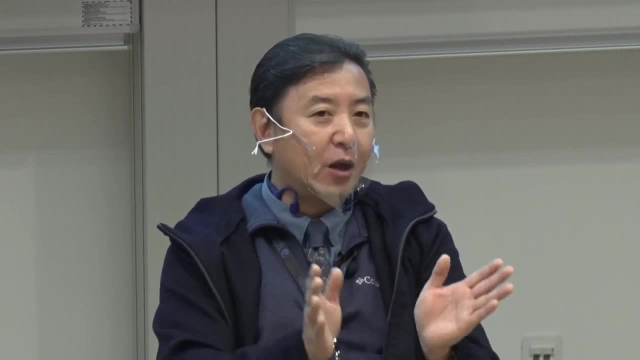 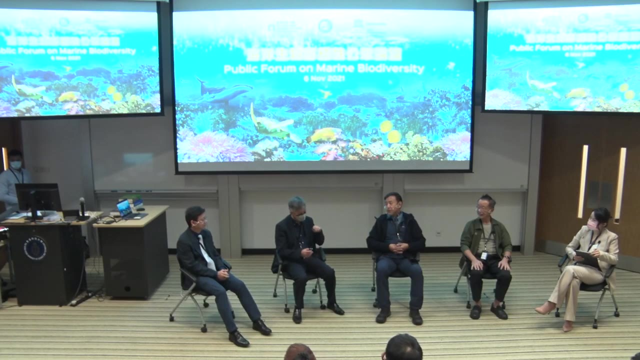 Also the consuming, how to consume, And then how many, how much is also the education. So this is all related to carbon. Yes, Professor Liu. OK, Maybe I add a little bit. You know we are talking about biodiversity and also climate change, right? 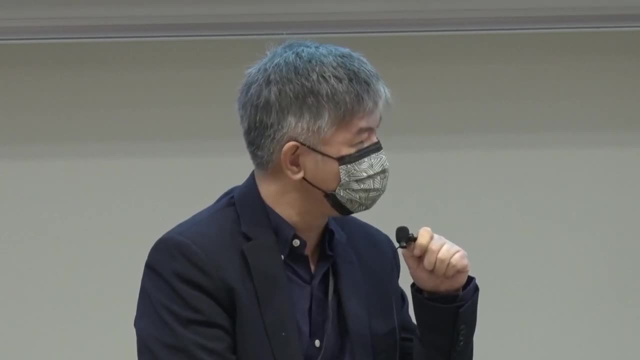 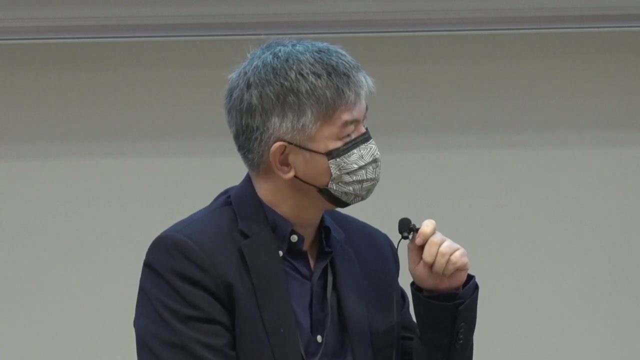 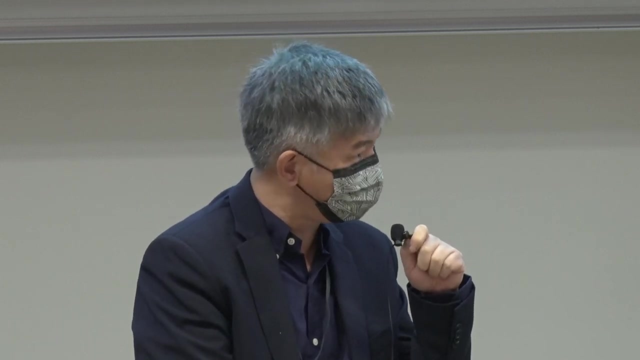 We are talking about COP 15 and the COP 26.. OK, So I think these two Are quite linked to each other. OK, On one hand, you know, global warming, climate change, can affect biodiversity, You know, like in ocean. 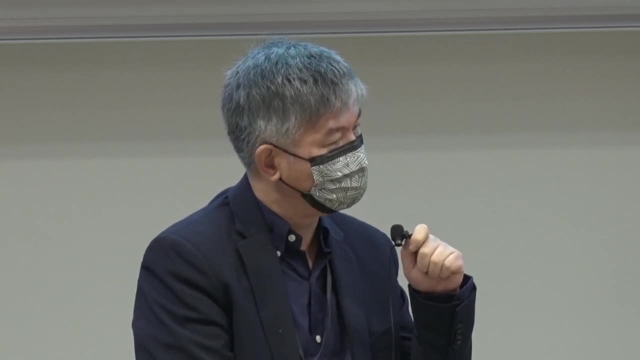 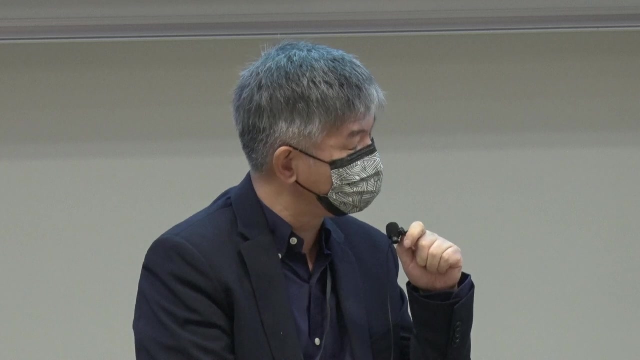 We have a warming ocean, We have oxygen depletion, We have ocean acidification. You know, all these can threaten the biodiversity And, on the other hand, you know this, biodiversity can also help to. you know the ocean, Yes. 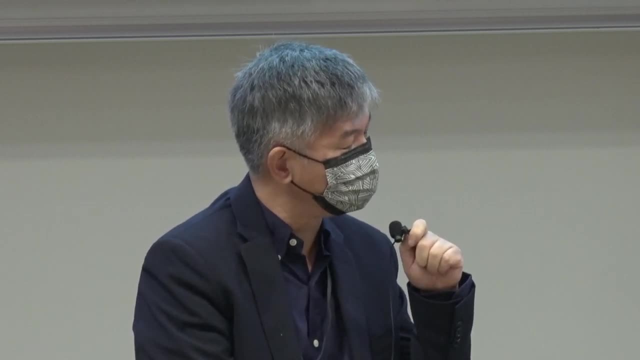 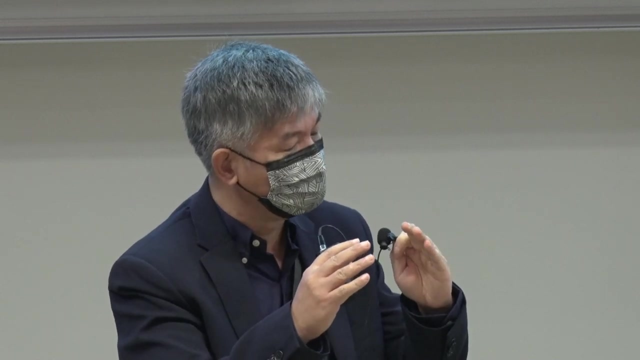 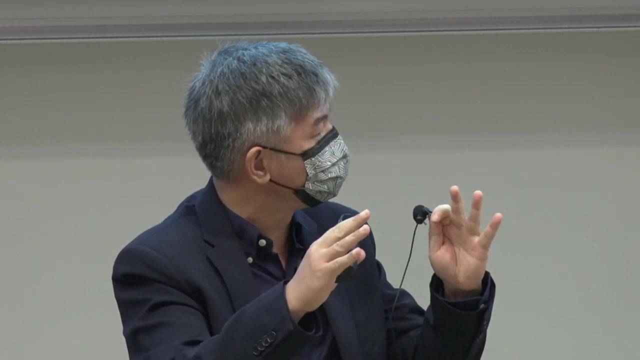 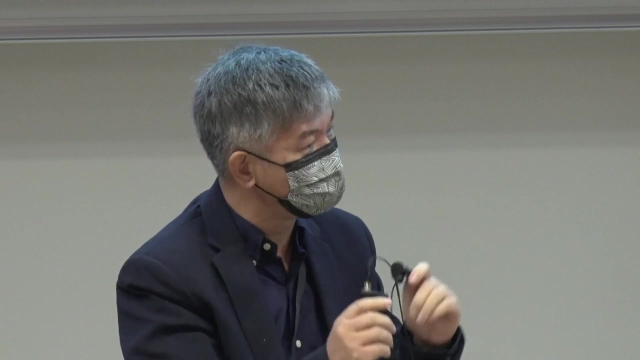 Yes, Yes, The ocean, the ecosystem fitness. you know the one more diverse kind of community ecosystem can resist. you know the change. OK, If you have a system with very few species, it will be very if you have some sudden change. 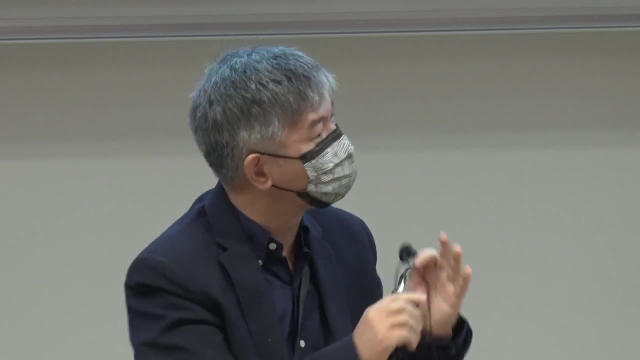 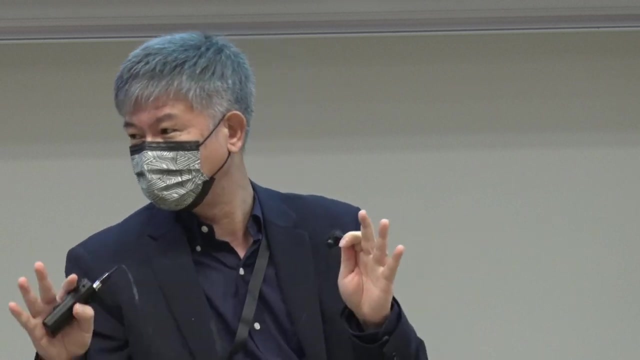 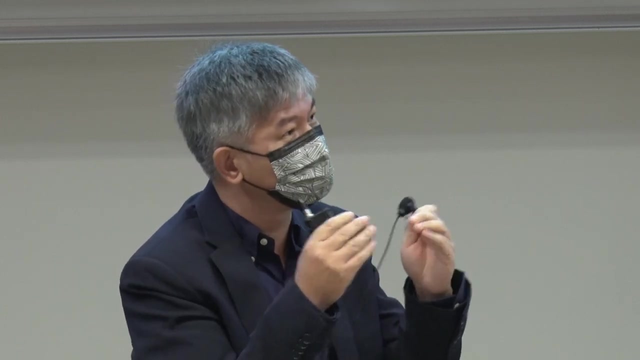 of the environment. it will, it will not, it will collapse. OK, This Some kind kind of theory. you know, a ecosystem with a more diverse species, there will be more resilience, okay, to the global change. so this, uh, i think the future, uh, research need to uh. 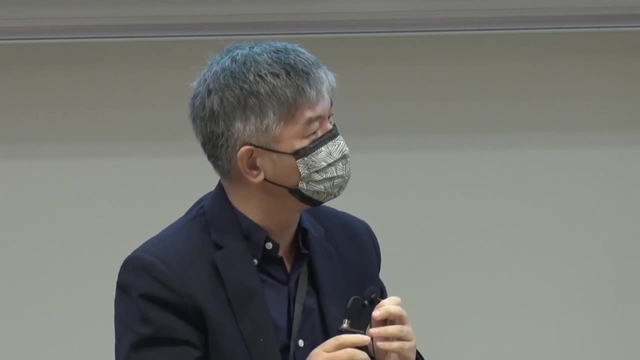 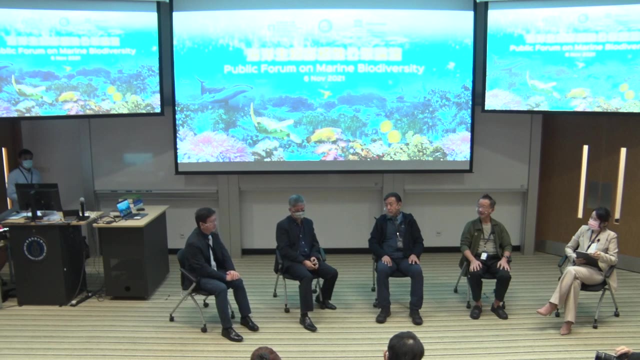 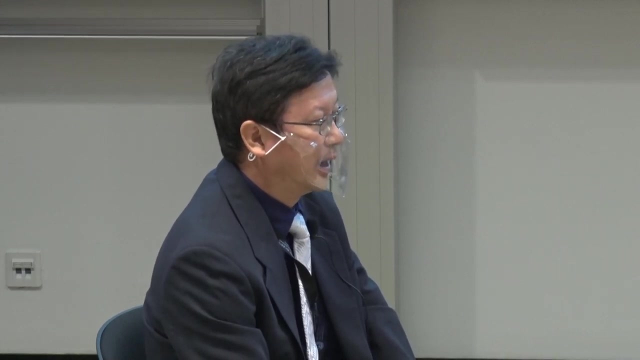 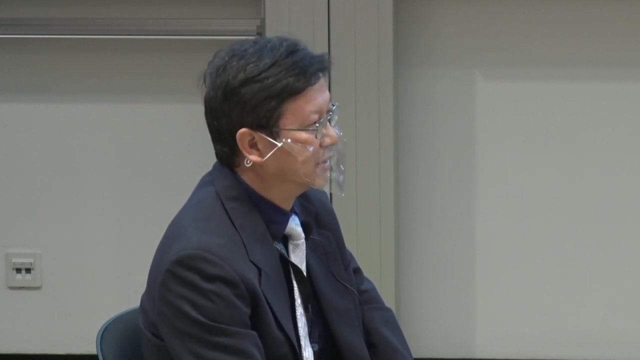 study the the interaction of of of these two topics. thank you, i also i agree with this point that with the knowledge about biodiversity we can make a better choice in our daily life. even everybody can contribute to reducing their carbon footprint can help achieve our carbon neutrality, of course. 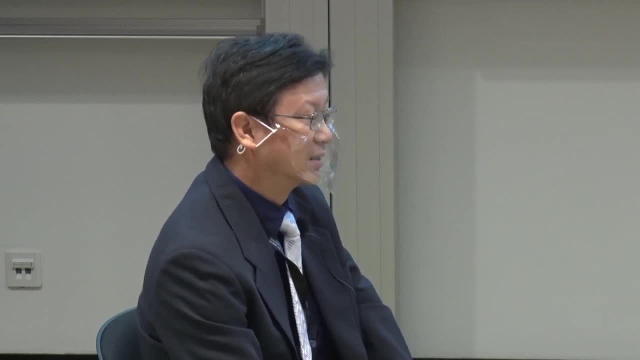 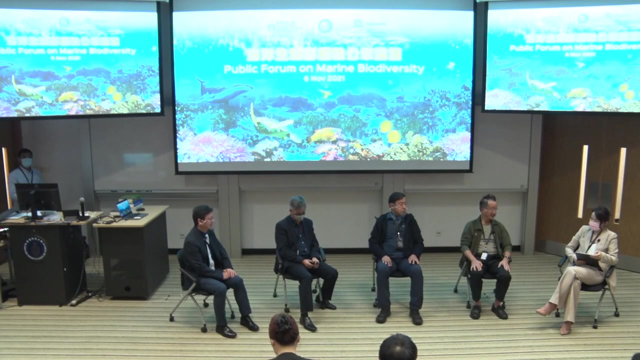 there's some, sometimes there's some conflict between conservation and development. so it's a society's decision to make, to determine whether, for example, a project should go ahead, whether we should compensate enough for the loss. so okay, thank you all very much for your insight, for sharing for our on-site participants. 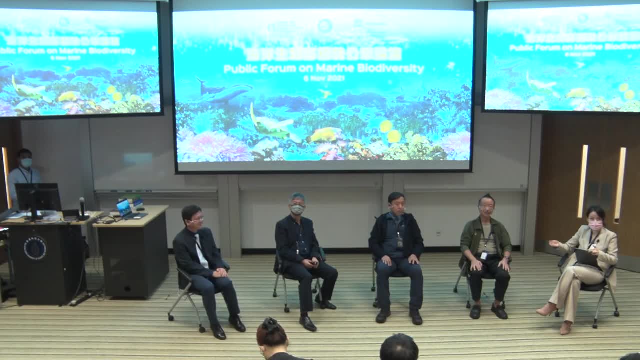 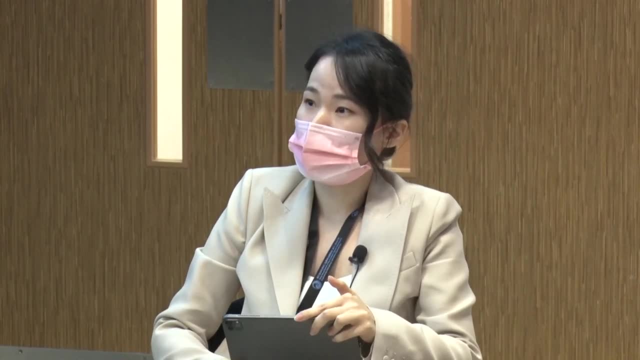 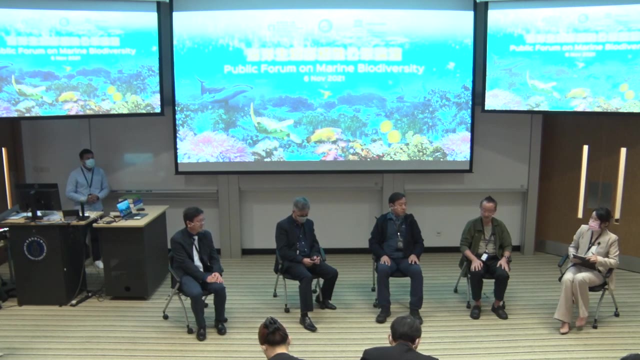 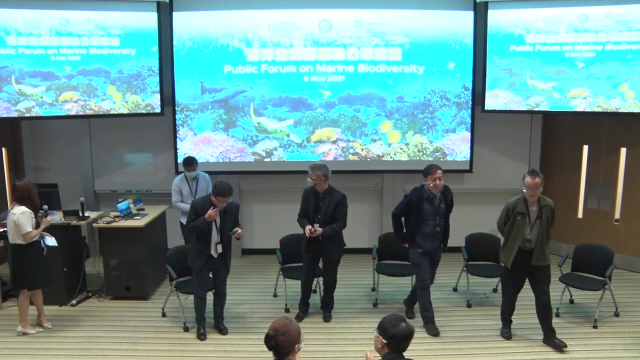 so you can continue the dialogue with our invited speakers after the q a session. so, since the time is limited, so i will pass the time to our mc again to continue the forum. so thank you all very much to the q a session. so, thank you, please visit it. thank you, thank you. 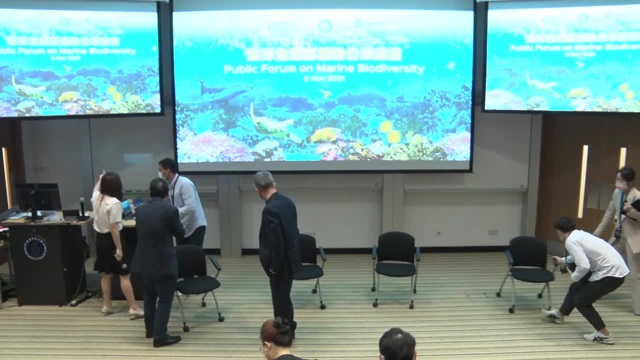 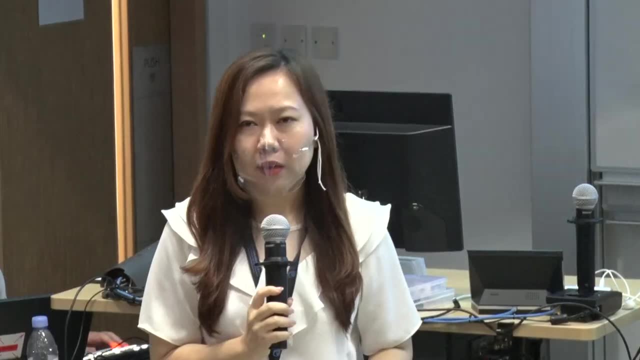 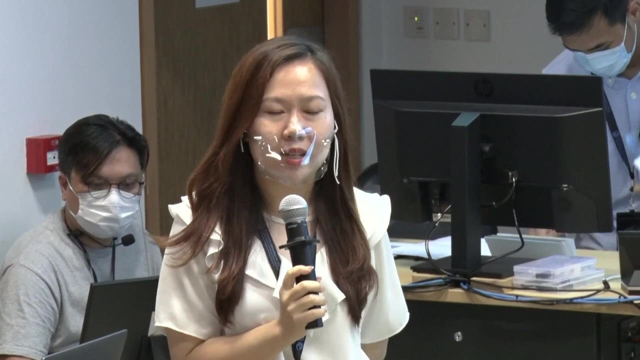 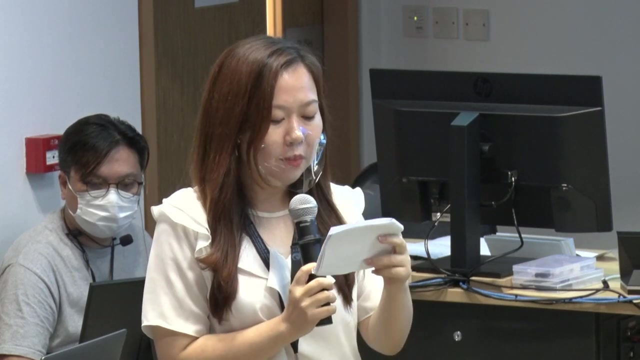 thank you, okay. um. before the closing remark and certificate presentation session: um, here you can see the qr code of the feedback form of today. hope you enjoy today's event. so, um to express our special gratitude to all guest speakers, may i now invite professor qian pei yuan and professor karen jean to present the thank you certificates and so. 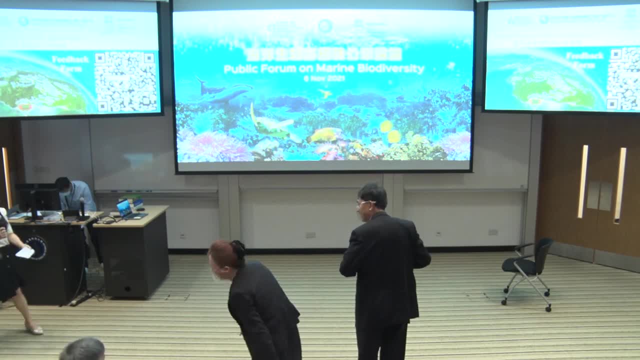 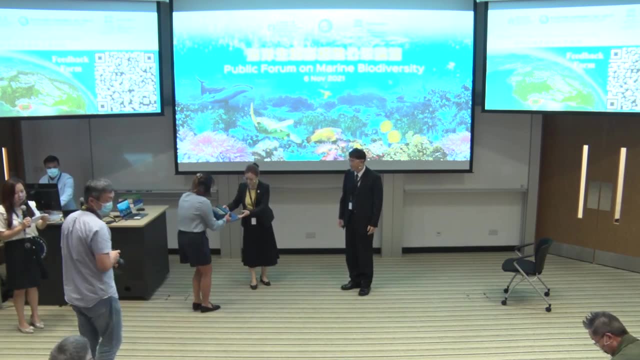 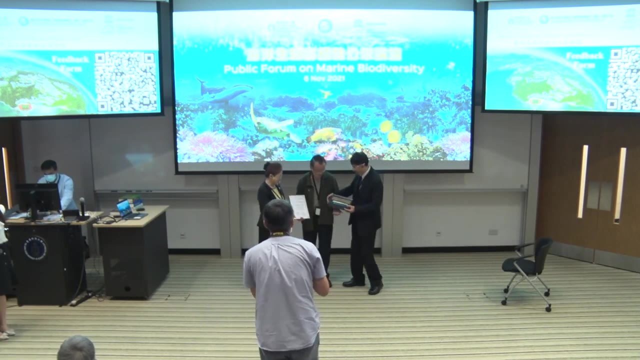 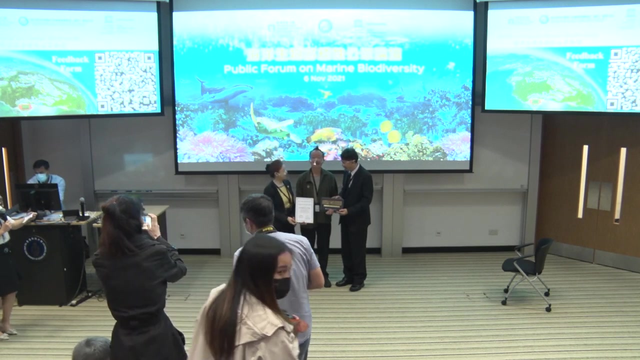 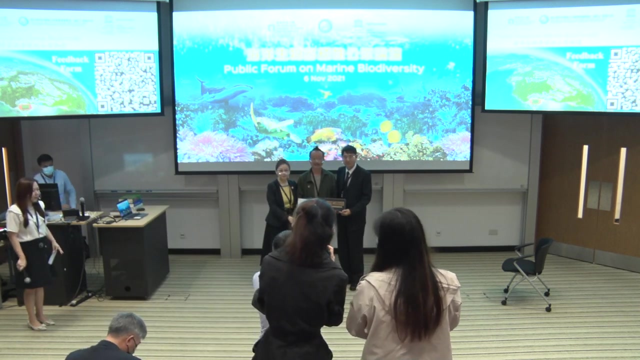 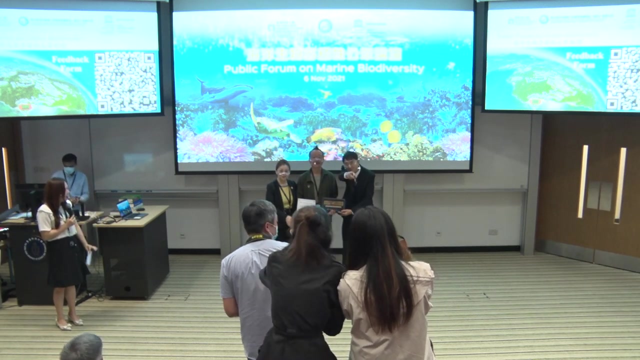 veneer to all of our guest speakers. please come forward. okay, the first guest speaker, professor thomas wong. please come forward to receive the thank you certificate and souvenir and have a photo with them. okay, help me. okay, professor wong, please remain on the left hand side. 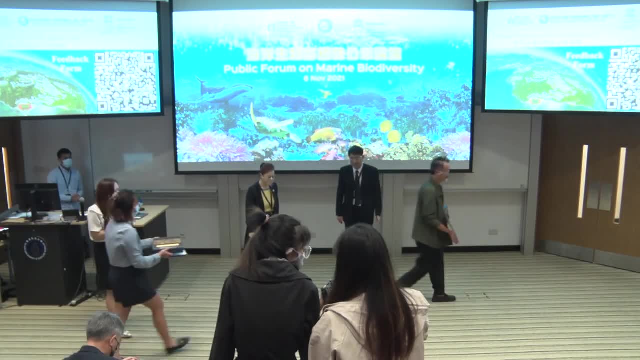 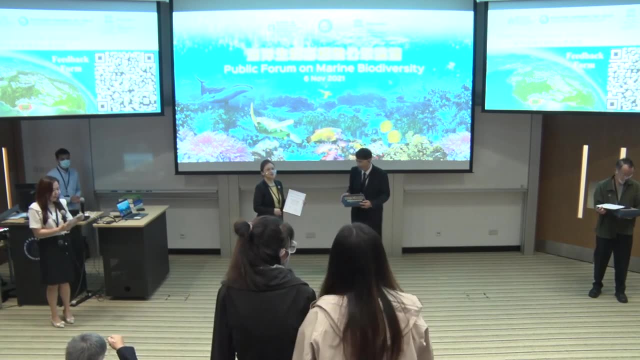 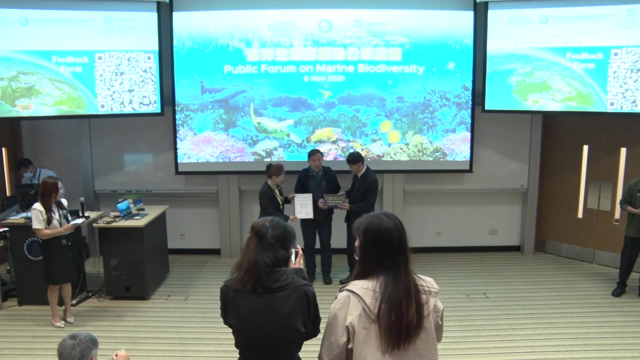 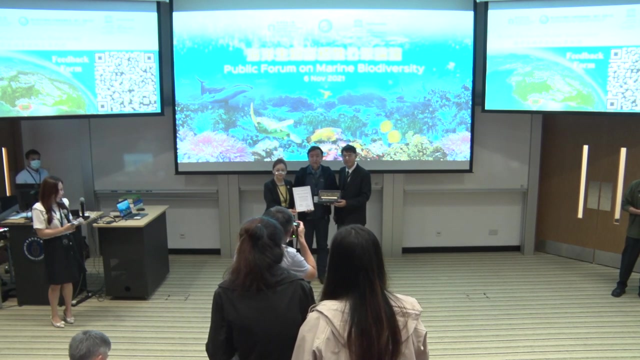 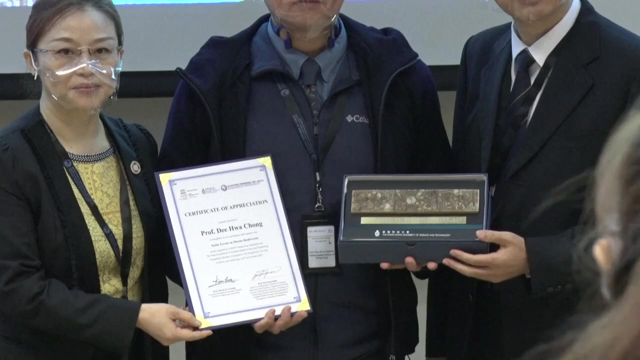 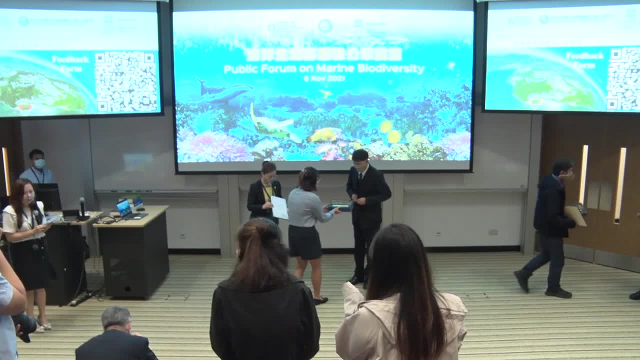 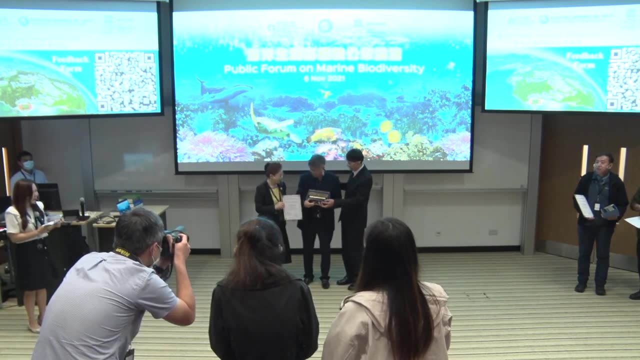 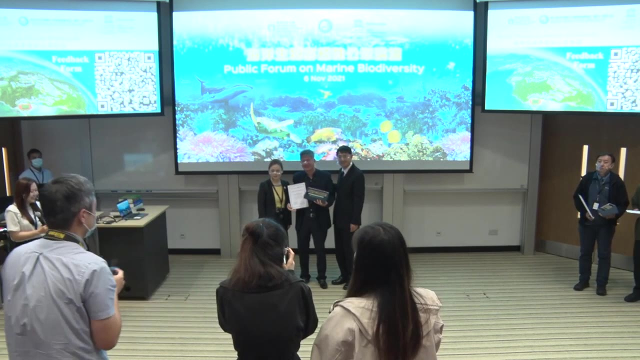 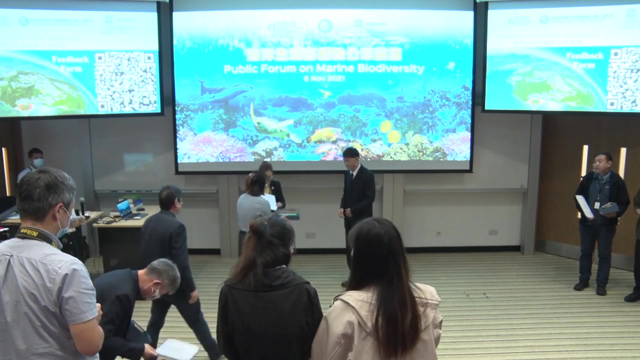 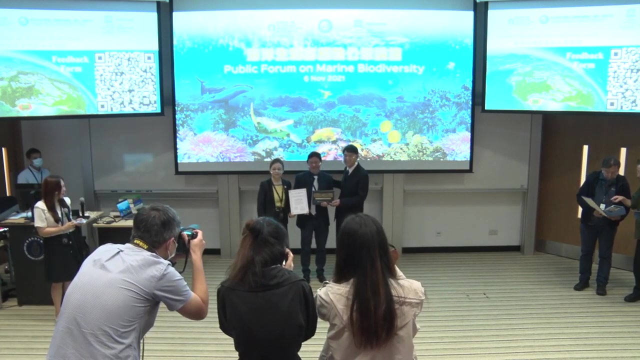 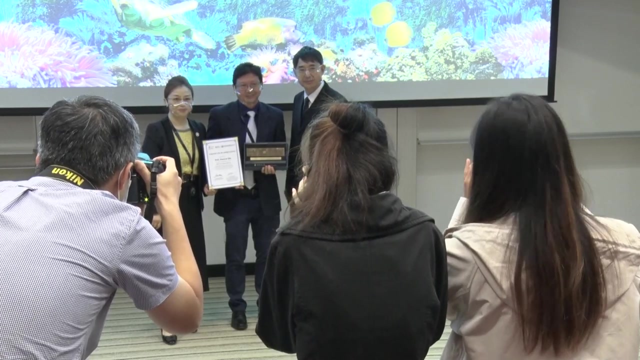 and the next guest speaker, professor liu huangbin, please come forward. thank you, thank you, come forward, welcome. Okay, last but not least, Professor Qiu Jianwen, please come forward. Okay, please remain, and all the guest speakers: please come forward and have a group photo. 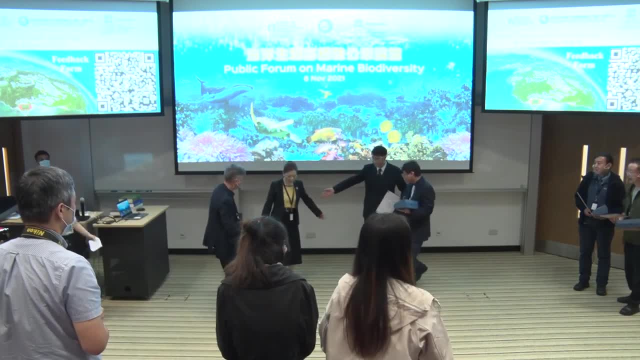 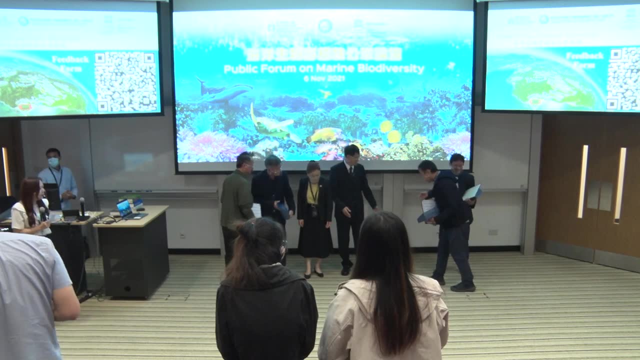 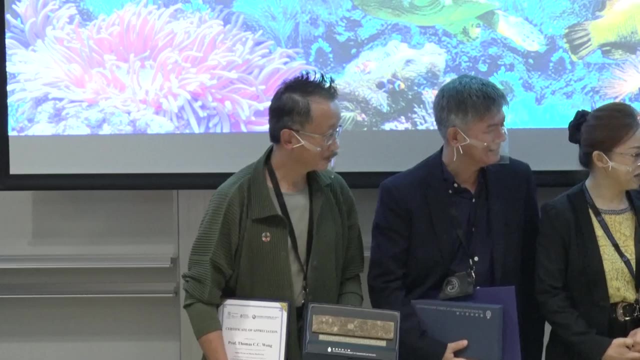 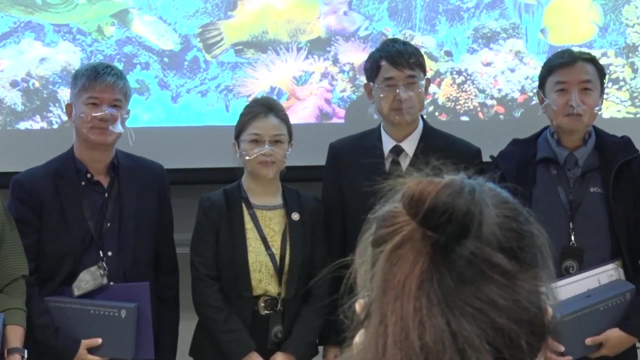 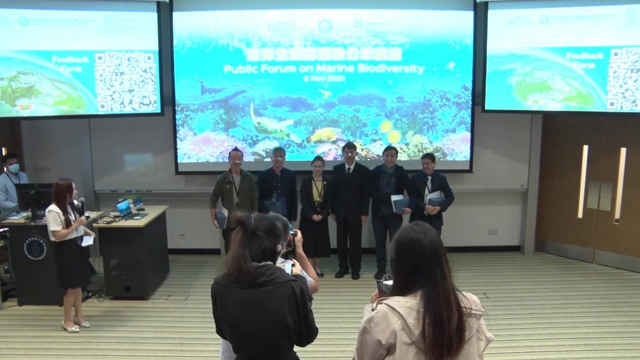 with Professor Qian and Professor Zheng. Yes, let's take a group photo together. Okay, thank you very much, Professor Qian and Professor Zheng, and Professor Jianwen- Okay, thank you, Professor Qian and Professor Zheng, please remain, and all the guest speakers please. 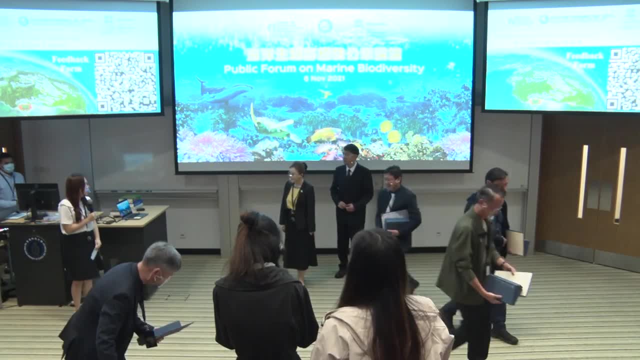 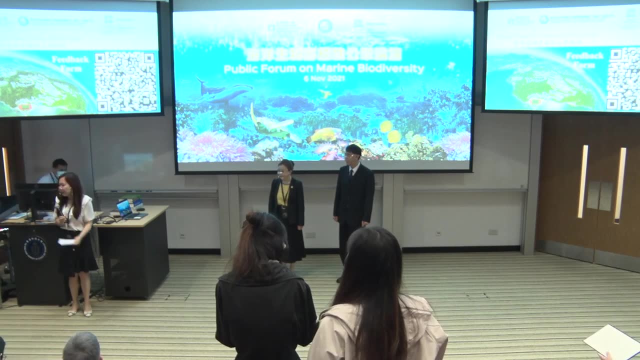 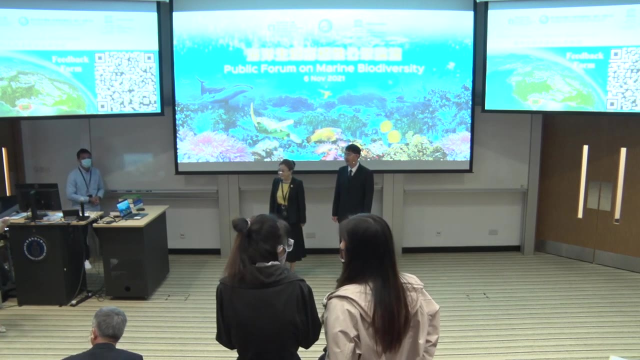 be seated. To appreciate our sincere gratitude for the Hong Kong branch team, we wish to present a certificate of thank you to all of them. Start to Hong Kong branch. Yes, As we know, the Hong Kong branch of Southern Marine Science and Engineering, Krundall-Naboratchikwancho. 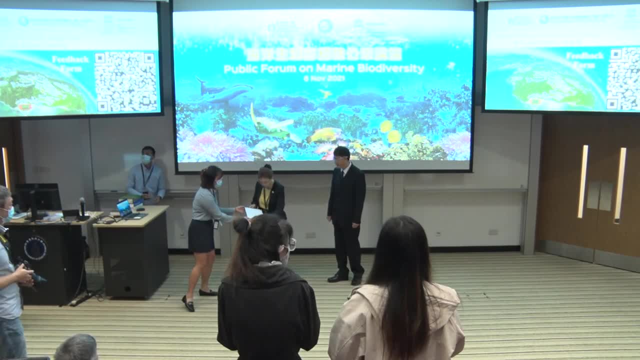 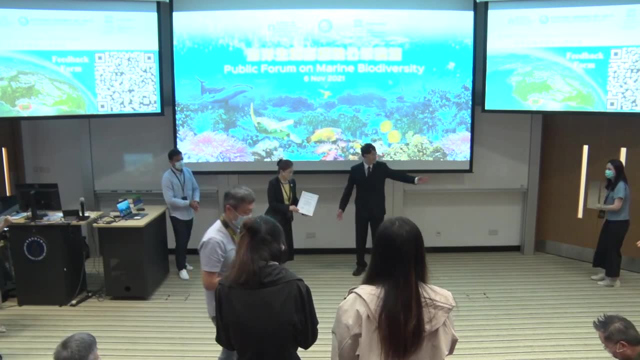 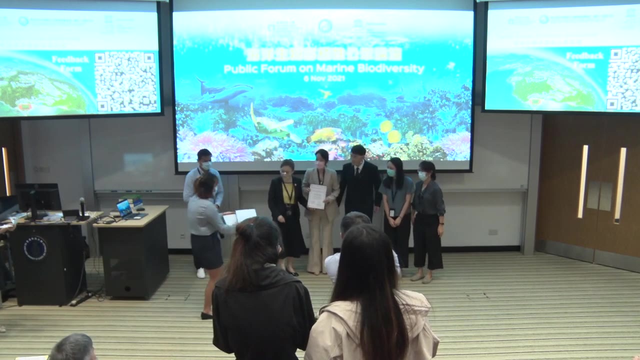 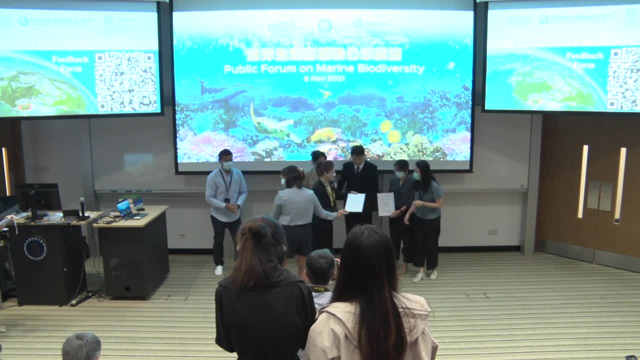 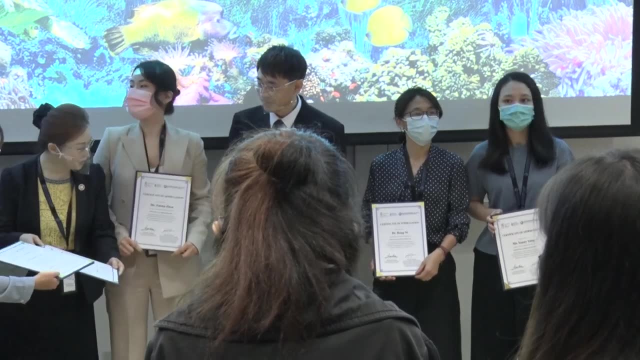 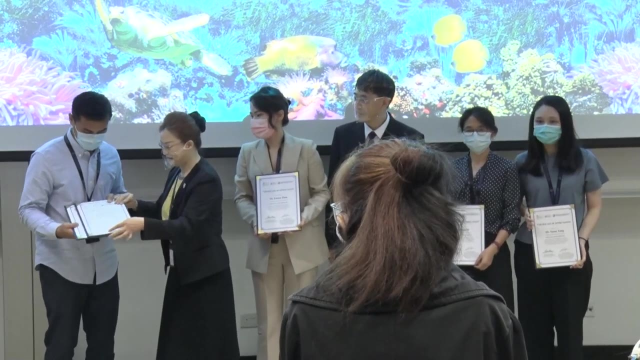 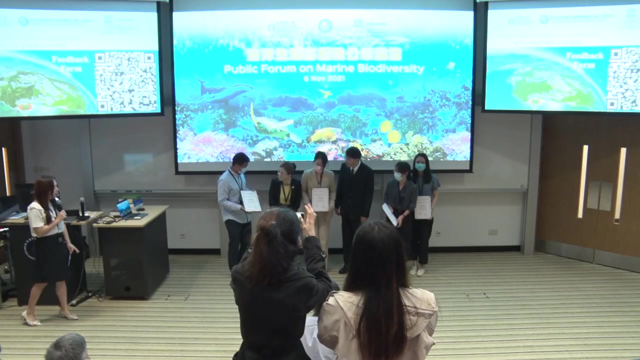 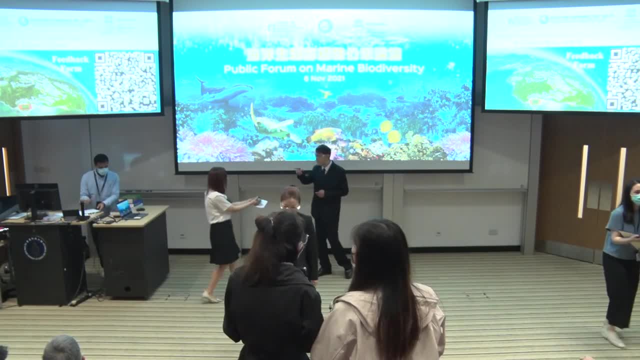 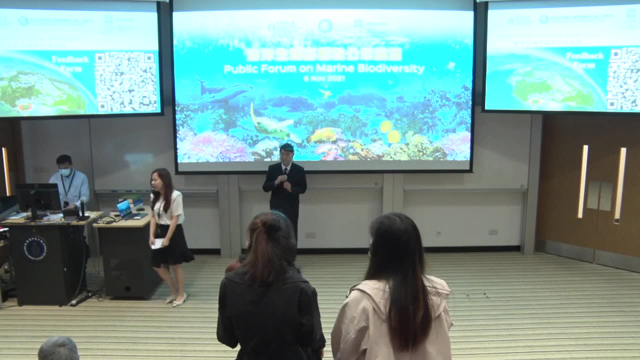 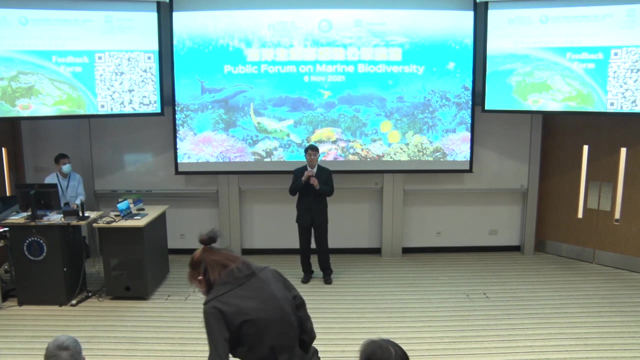 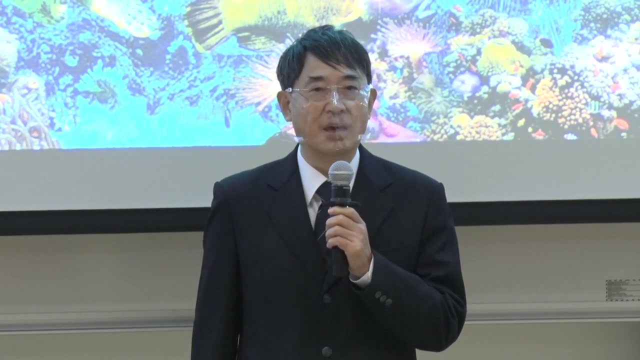 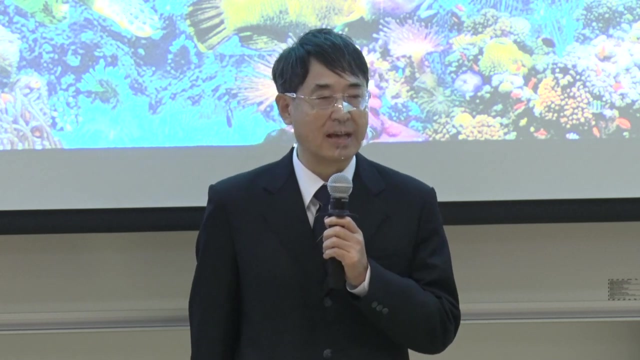 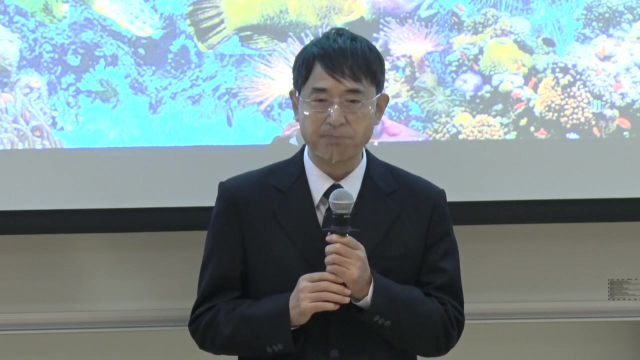 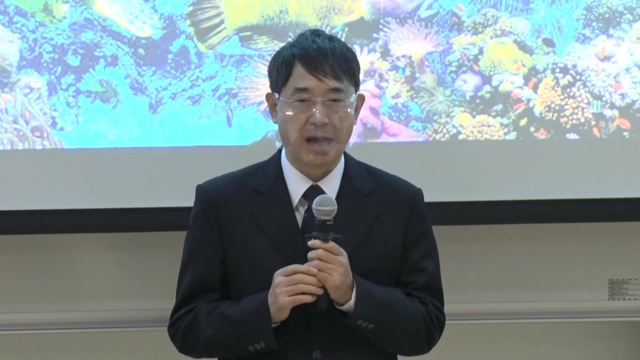 Hi, closing remarks for today's event. Well, so the really exciting afternoon time passed very fast. on behalf of the organization organizing the body of this public forum, that means the Hong Kong branch of Southern Marine Science Engineers, Guangdong Laboratory and also the UNESCO of Hong Kong. 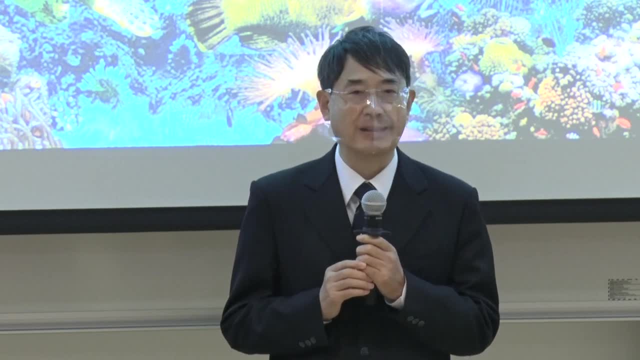 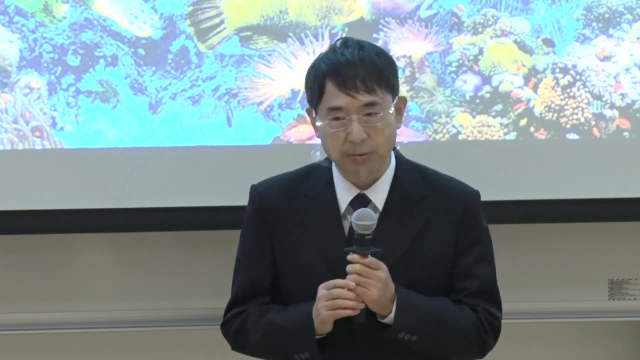 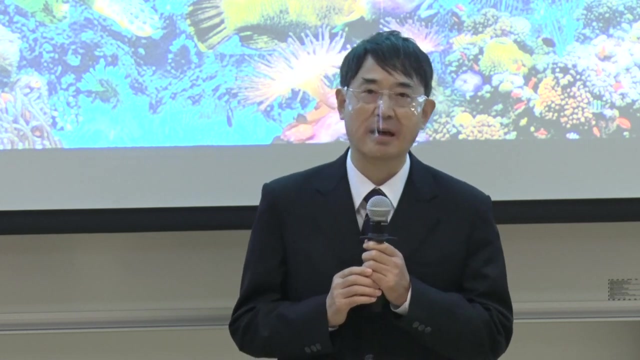 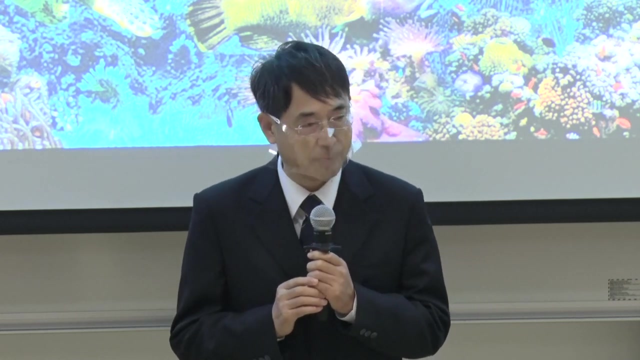 I'd like to thank all of you for attending this public forum on marine biodiversities. I also really want to thank all the distinguished speakers for today's public forum. Their talks definitely enriched our knowledge on marine biodiversities, As Mr Ng pointed out. 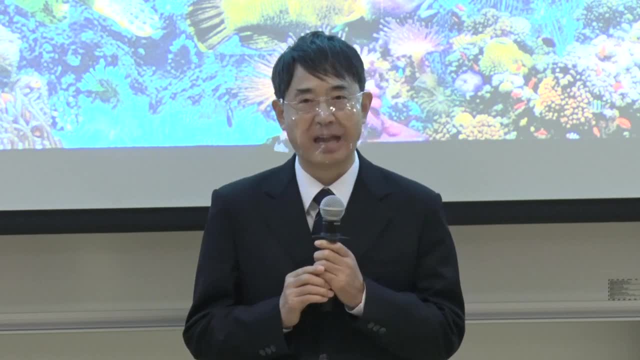 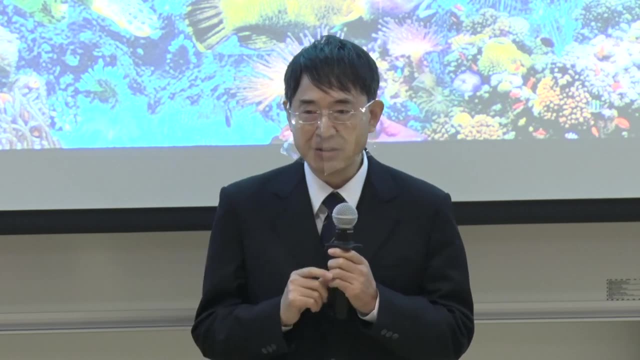 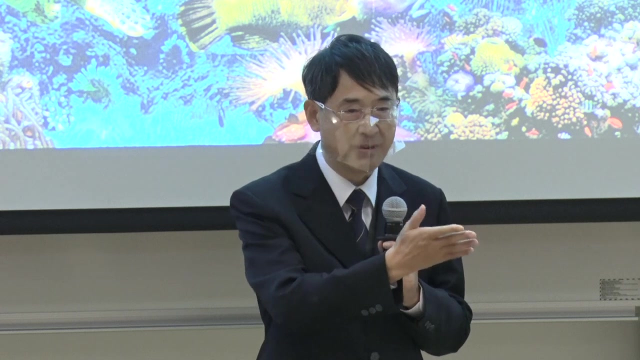 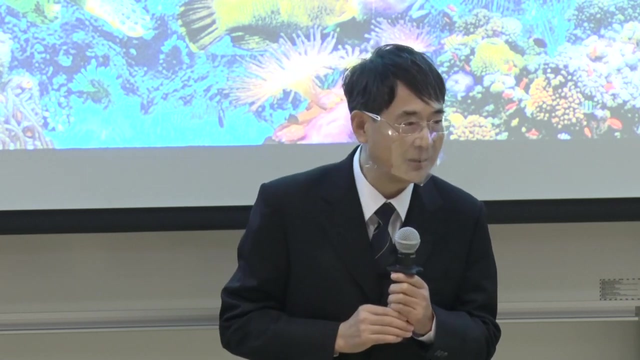 regarding the biodiversity protections, there are a number of issues. First of all, do we have the desire to know what's up there? Secondly, as some of our guest speakers pointed out, do we know what they're doing there in terms of ecological? 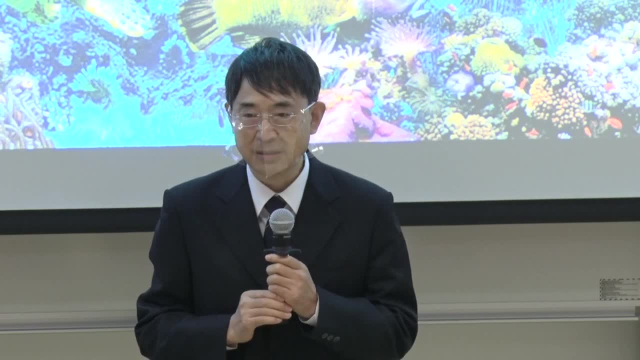 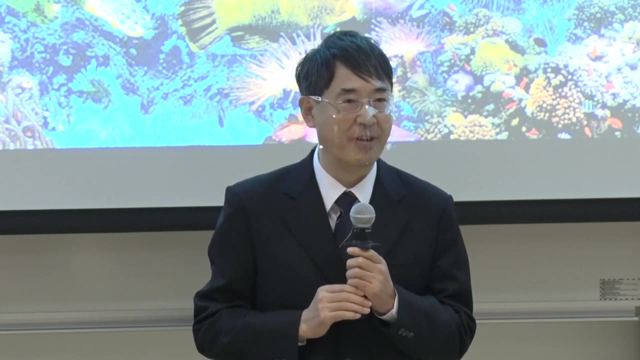 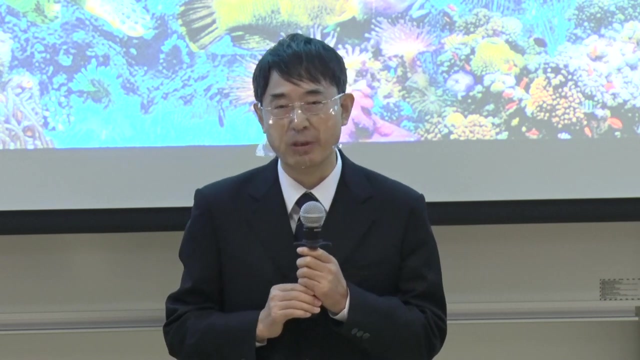 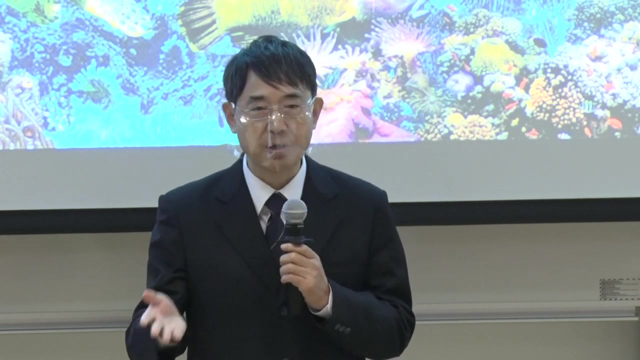 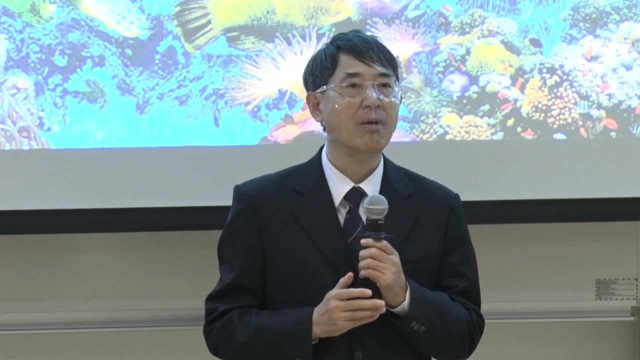 function and service. My impression is overall, Hong Kong is very, very rich in marine biodiversity, But there are still huge knowledge gaps. There are lots of species, regardless of the fish, all the worms, all other marine organisms We still do not know. 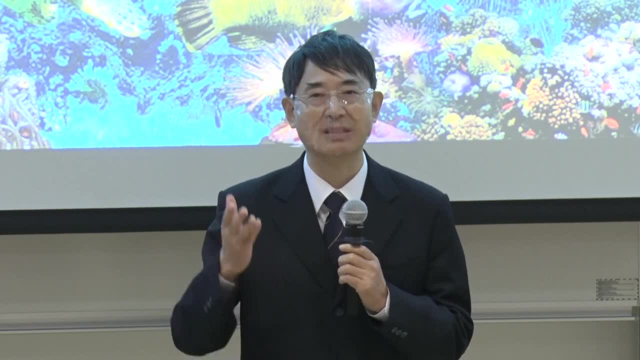 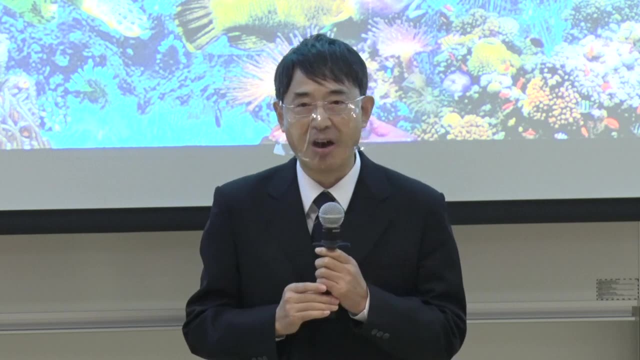 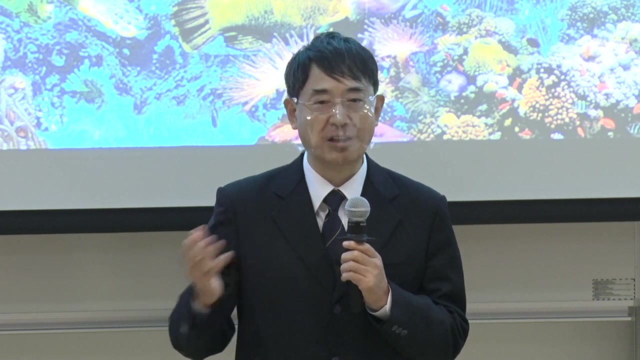 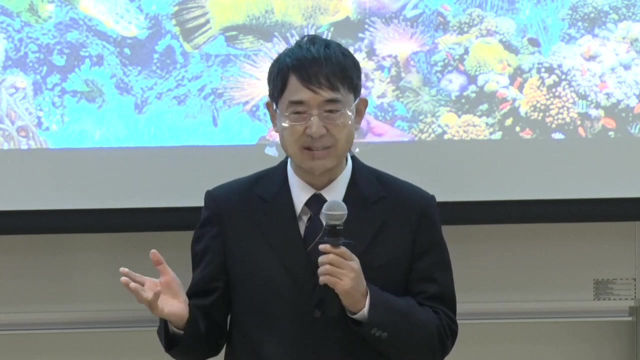 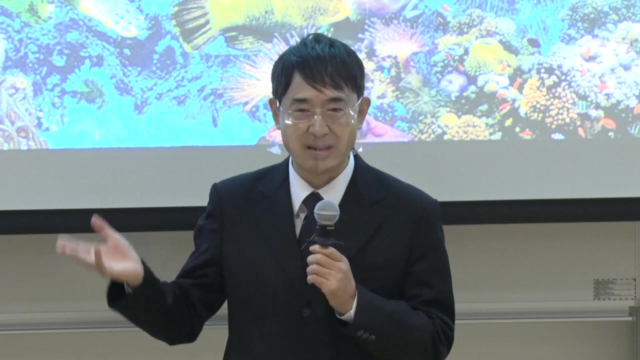 many of the species in terms of taxonomy, in terms of their ecological functions, But overall, as Mr Ng pointed out, when Hong Kong society is talking about the environment, lots of times people even don't mention about marine systems. So we tend 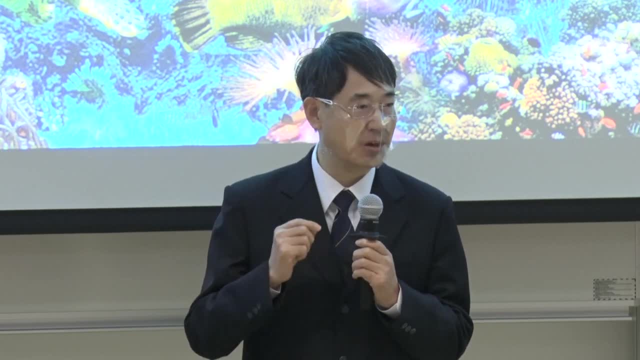 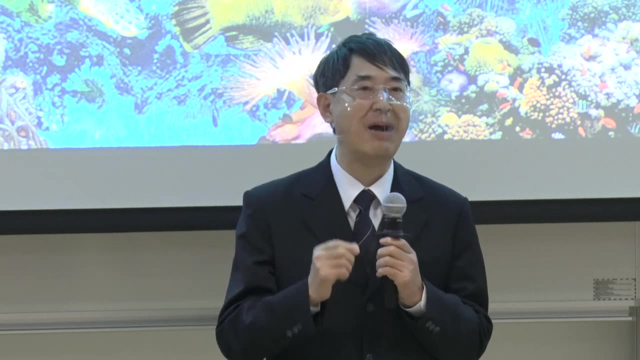 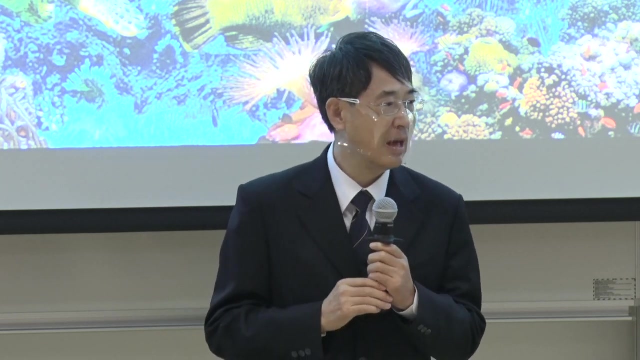 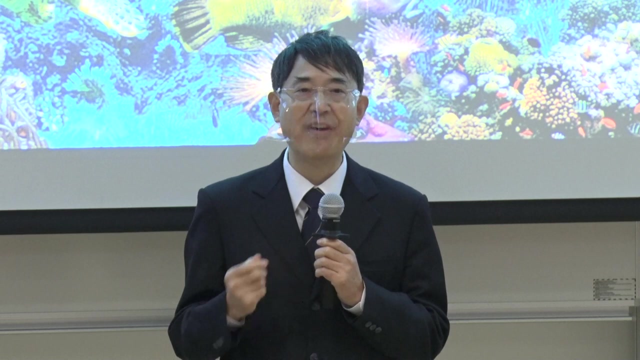 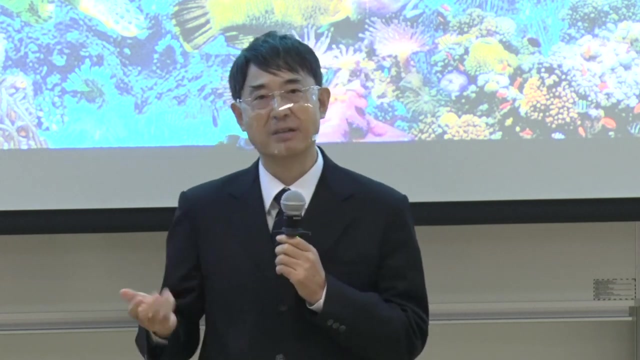 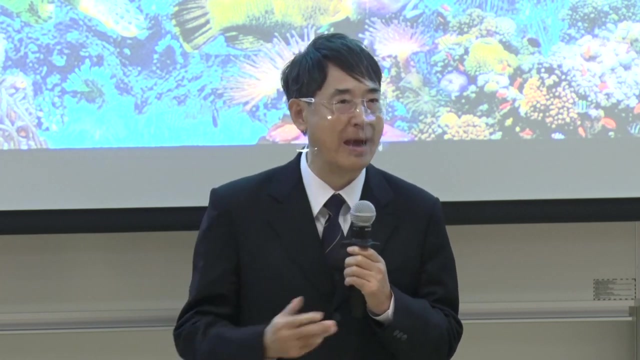 to forget about it, But Hong Kong is surrounded by waters. When we're talking about our environment without considering the ocean, also the marine, how can we address the so-called environmental issue here? So we're facing challenges Without understanding ocean betters. 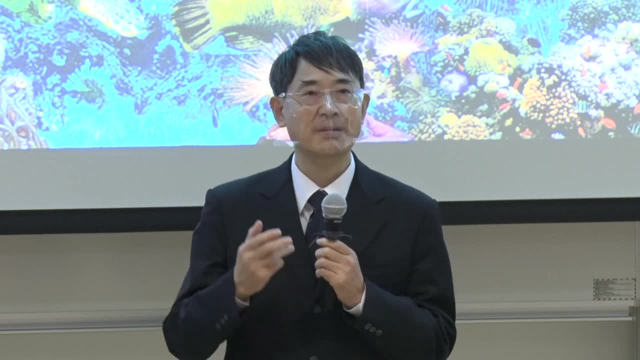 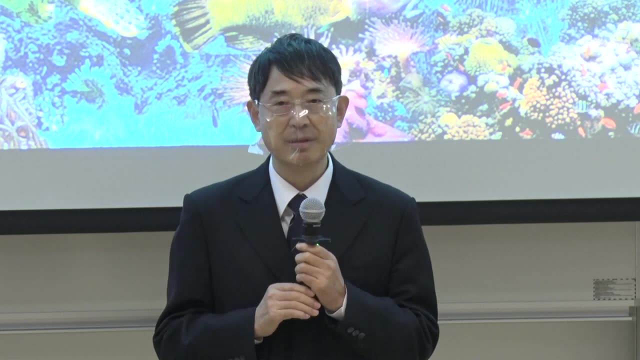 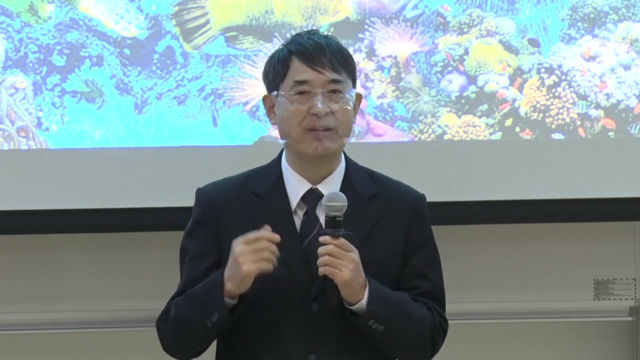 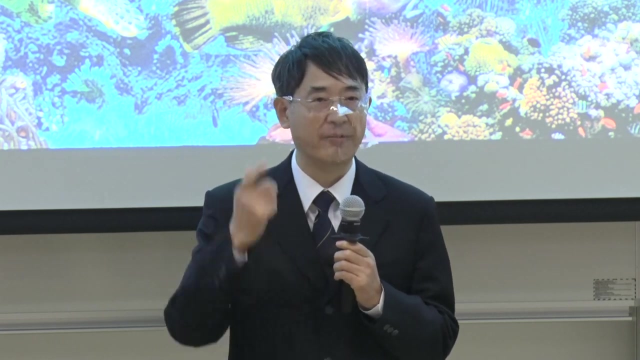 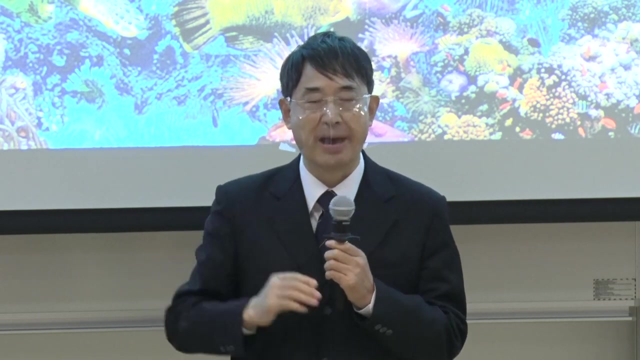 you know, we cannot really find a proper solution to deal with our problems. So biodiversity is the key word for today's public forums. You and I, we are all the citizens of the planet. We share the richness of the biodiversity. But, more importantly,